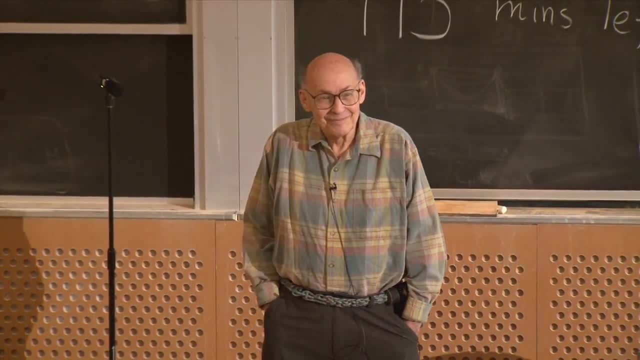 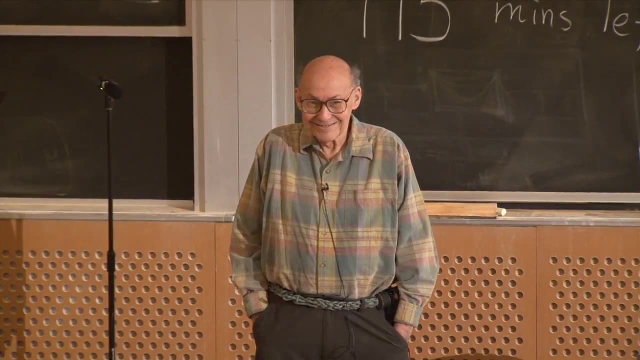 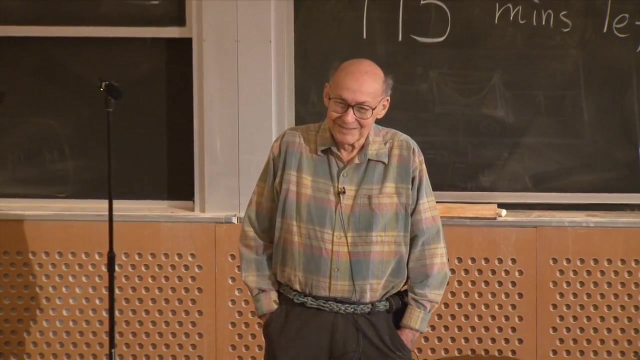 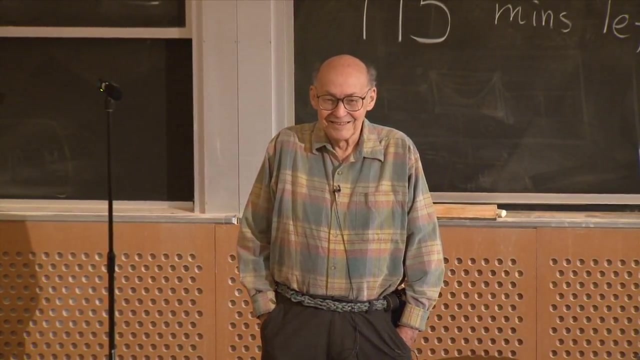 What do you think AI people should work on next? Do you know what question I was going to ask you before you said your question? Oh, OK, I was going to ask you: what kind of questions do you think that AI people should be asking right now? 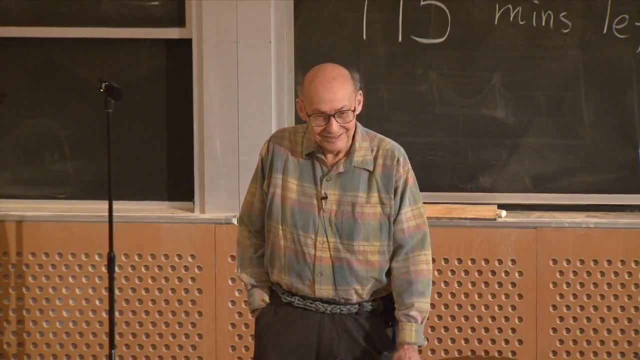 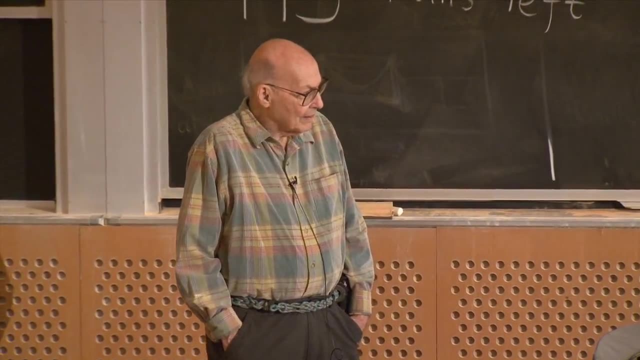 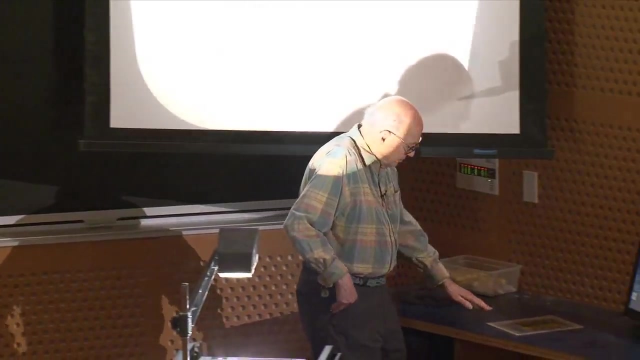 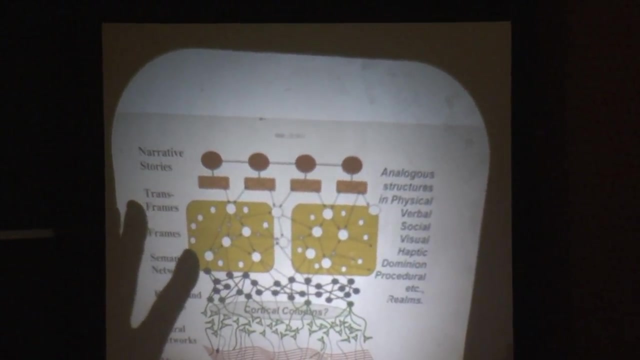 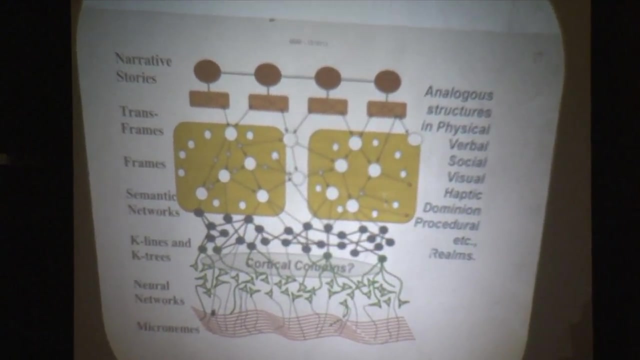 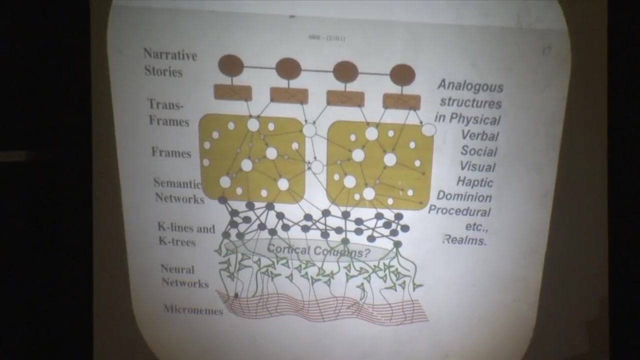 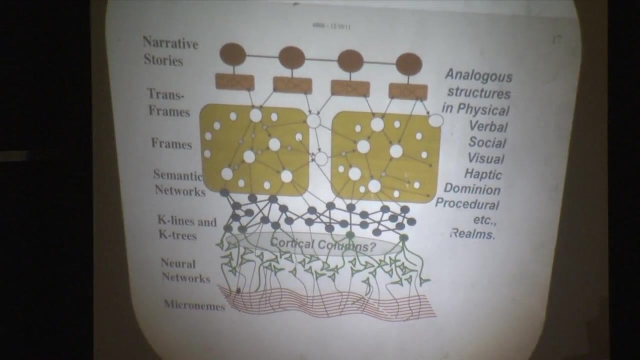 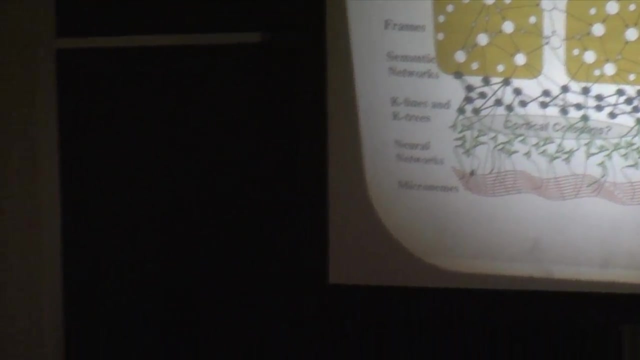 That's right. Anybody have a meta question? One good question is: I could focus it better But Or make it bigger. Is that enough layers? It's possible that I got the idea from Sigmund Freud, who wrote about 30 books. 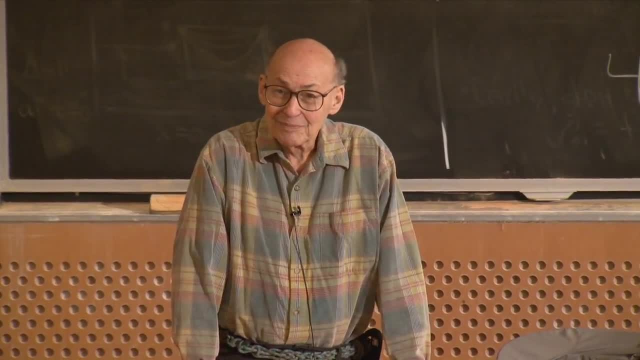 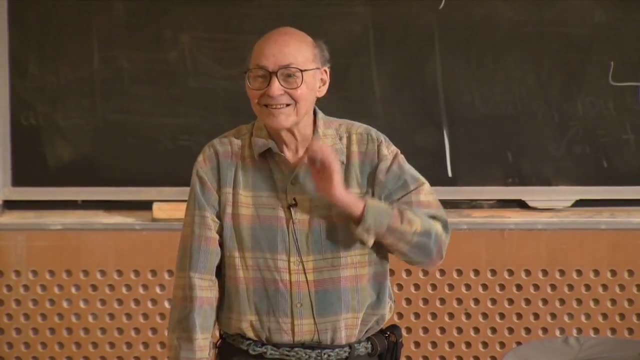 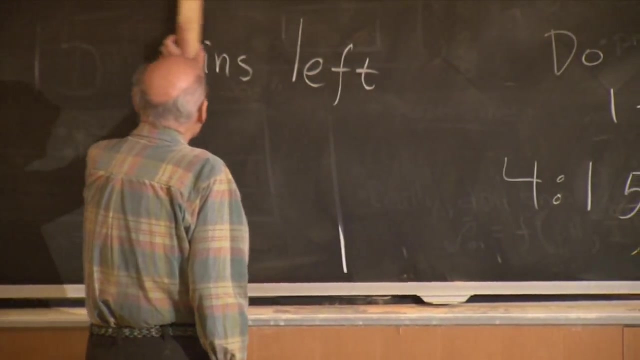 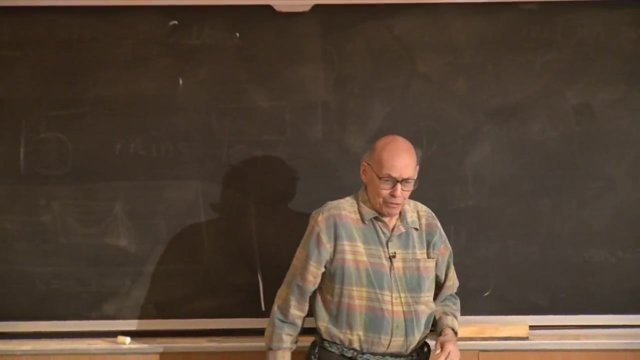 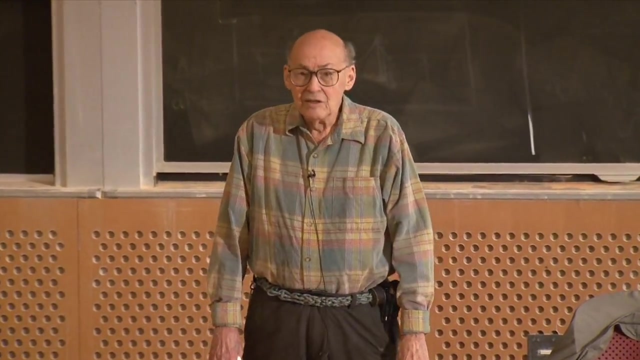 Who knows what Sigmund Freud's three layers were. Sure, Id ego superego. Right here Id ego superego. Freud wrote about 30 books. I know because I had a graduate student once who decided to quit computer. 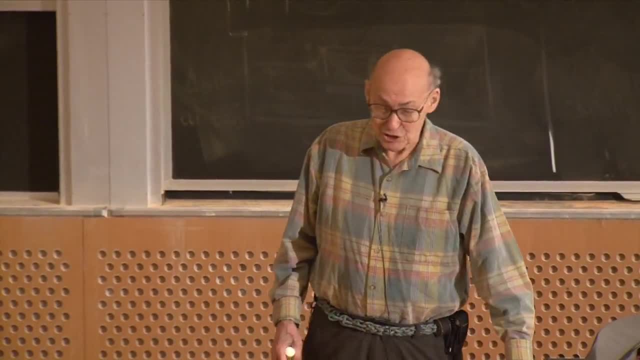 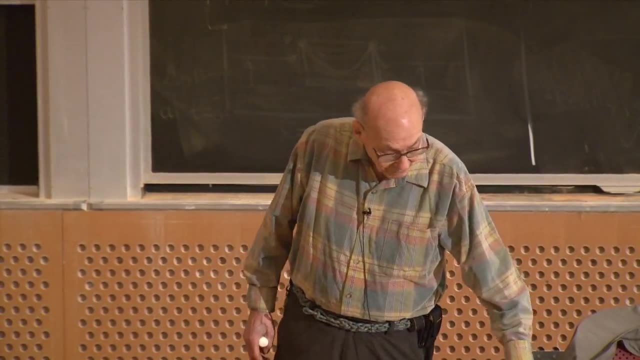 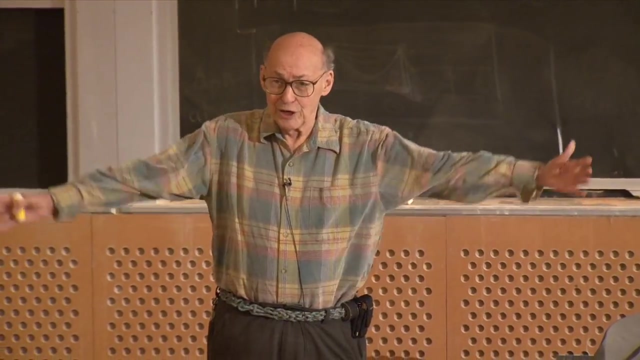 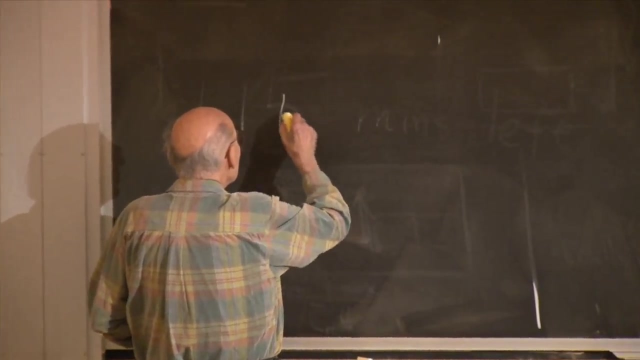 science and go into emergency medicine. He had an MD which he wasn't using And he suddenly got fed up with computer science. So he sold me his set of Freud books, which is I don't know if he is going to be using them, but 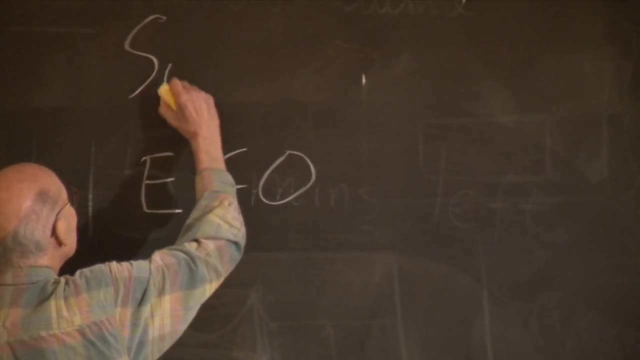 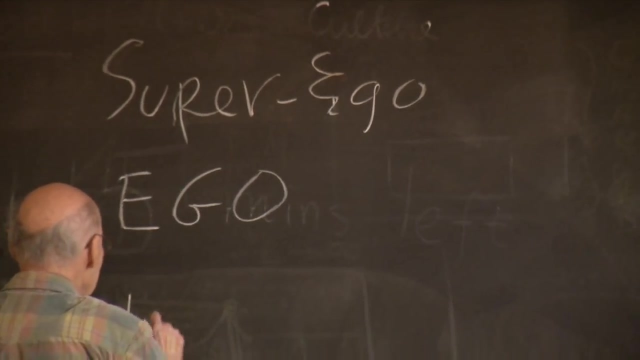 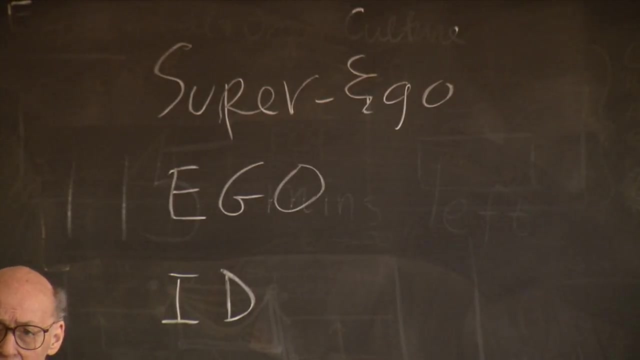 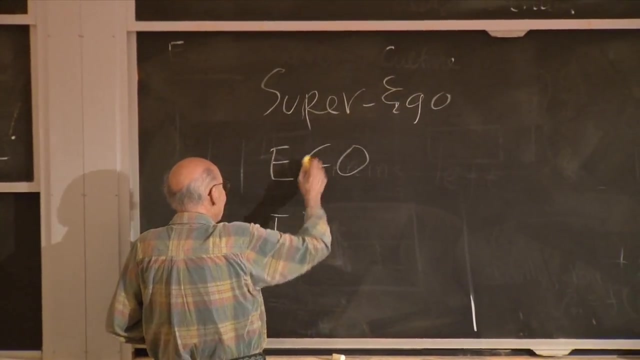 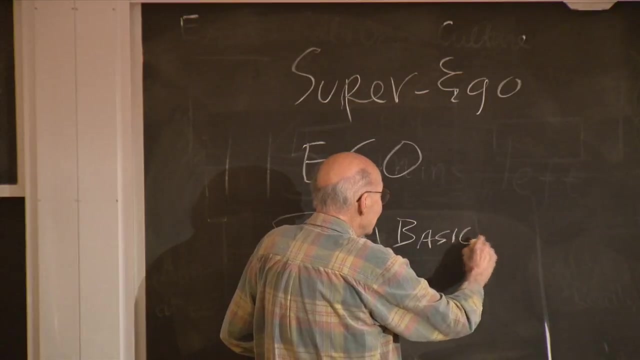 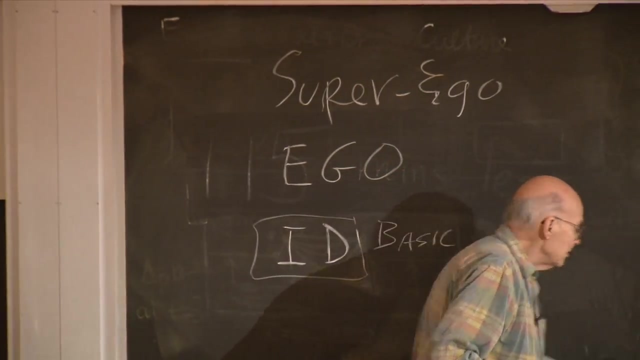 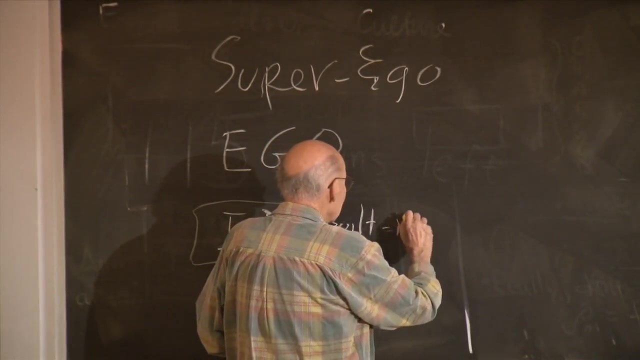 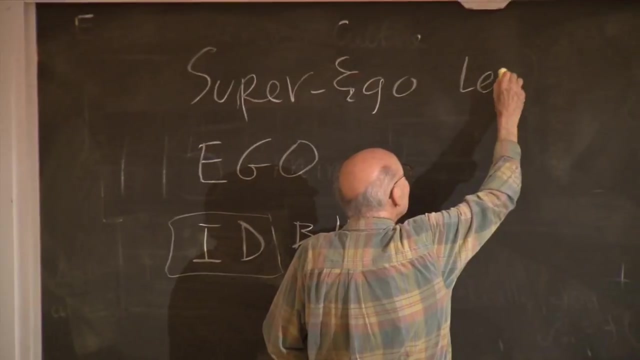 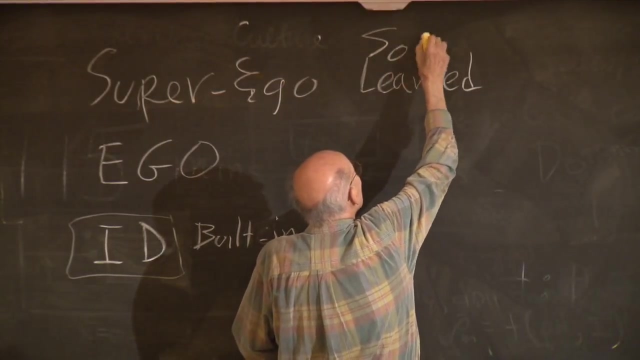 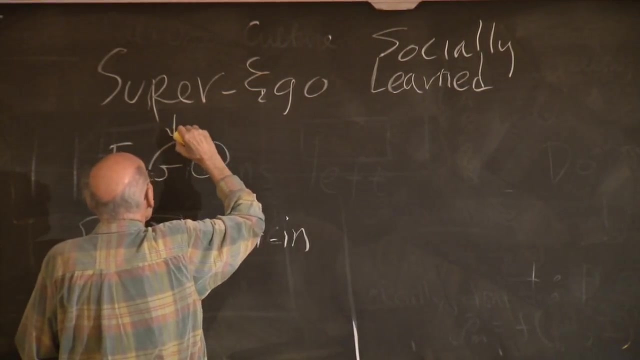 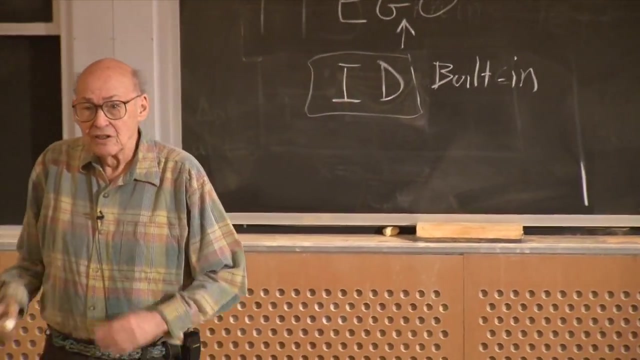 But. But in Freud's vision these don't seem to be a stack. But there is this thing which is basic instincts- I shouldn't say basic, maybe to a large extent built in And this is learned socially. And I think the nice thing about Freud's concept. 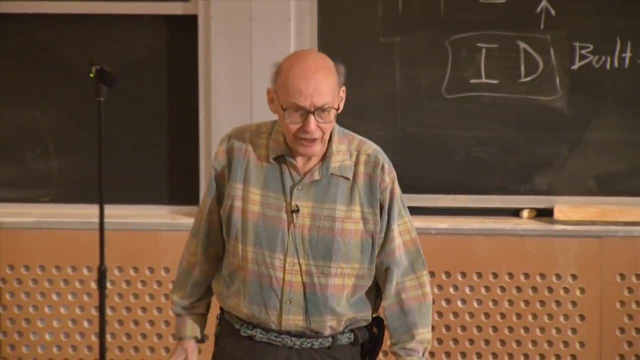 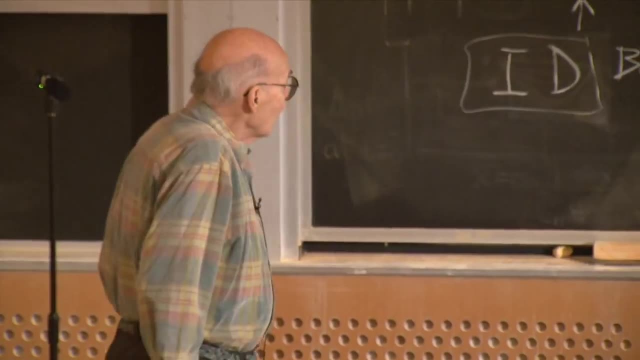 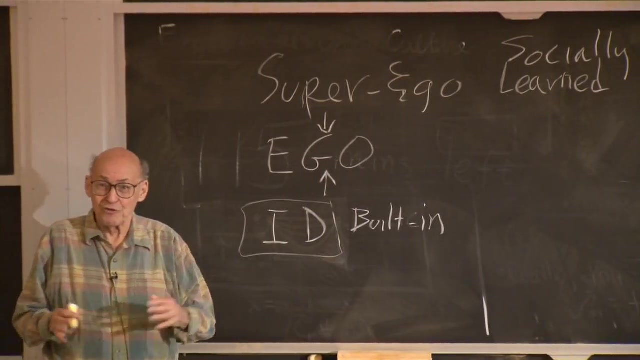 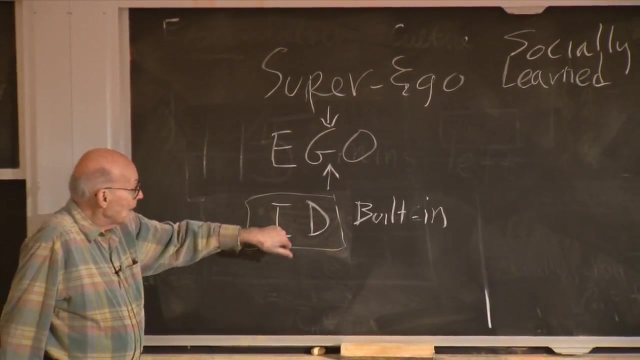 which, as far as I know, doesn't appear much in earlier psychology, is that these conflict. And when a child grows up, oh, A lot of what we call civilization or socialization or whatever, comes from taking the built-in instincts which 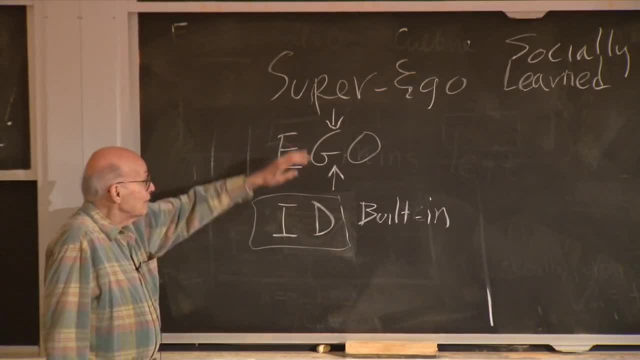 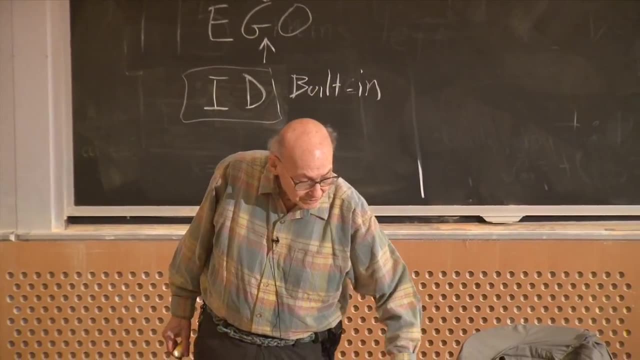 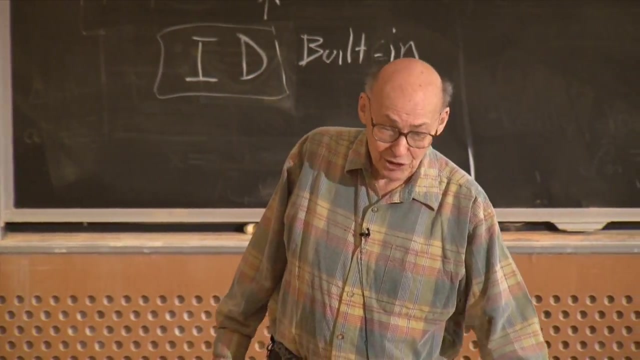 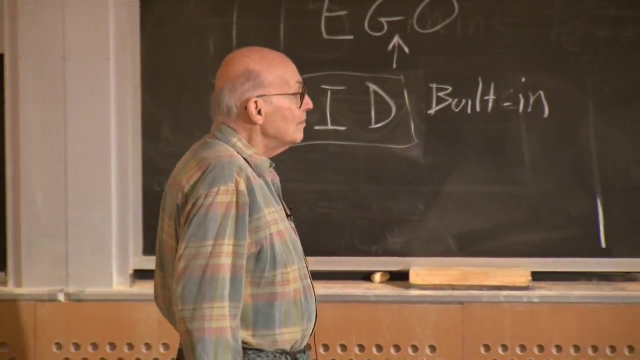 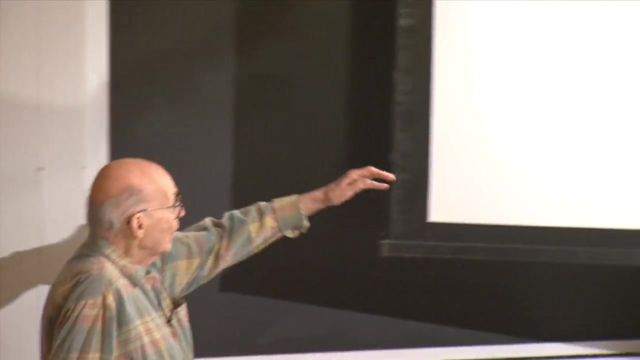 is, if you see something you like, take it and the social constraints that say you should negotiate, And if you want something someone else has, you should fool them into wanting to give it to you or whatever. So in fact, when I make this big stack of mechanisms, 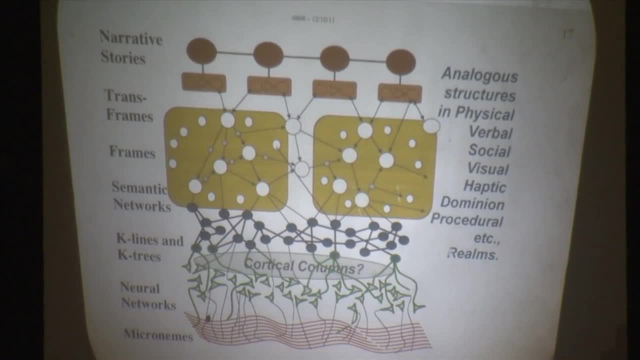 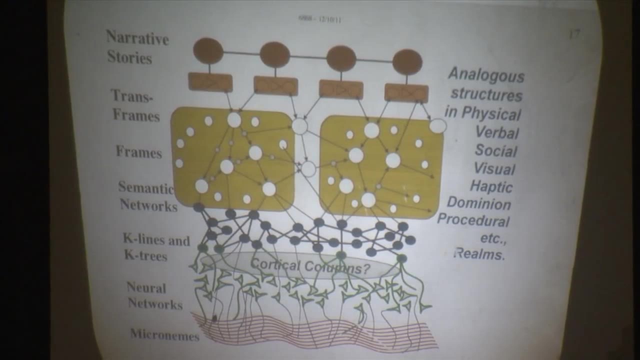 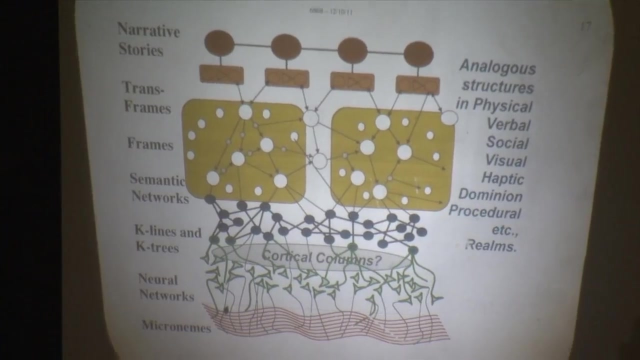 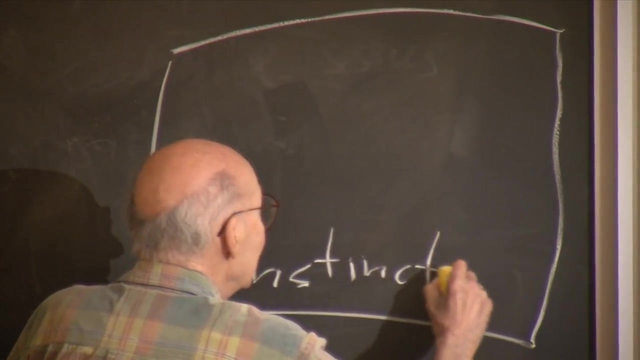 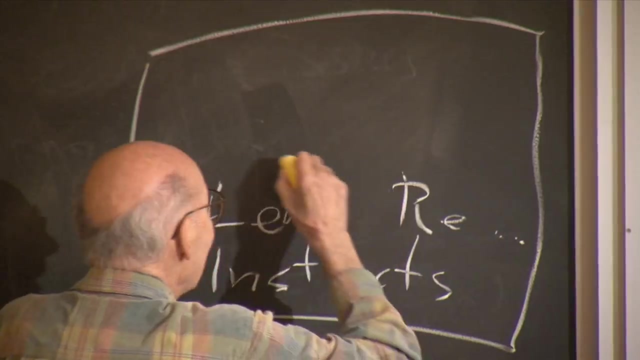 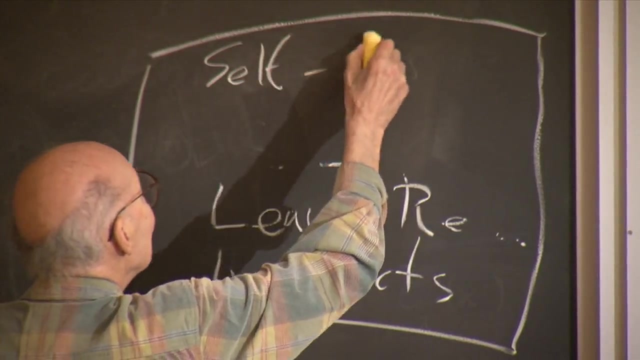 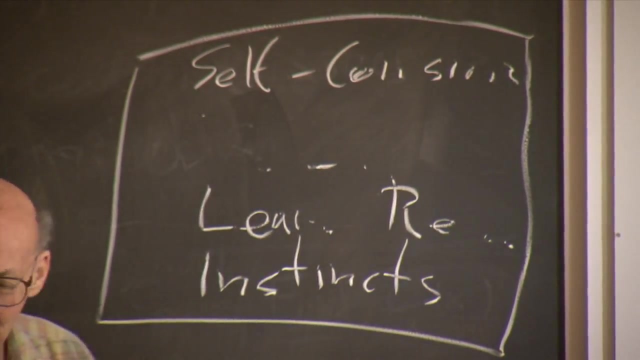 that really well. that's actually not the, The organization that the book starts to develop chapter by chapter, which was instincts, learned reactions and so forth, up to self-conscious. What's the next to top layer? Self-idealism. 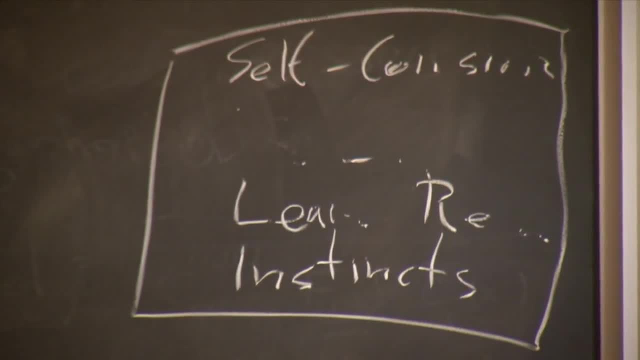 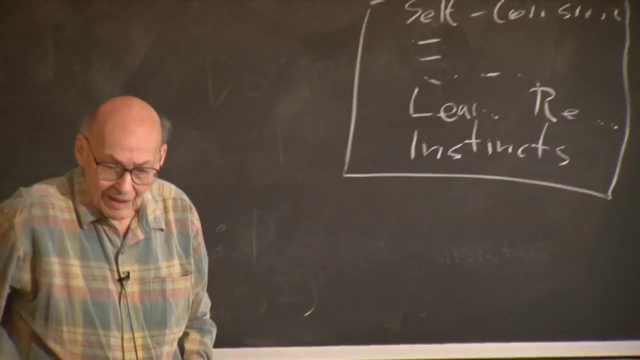 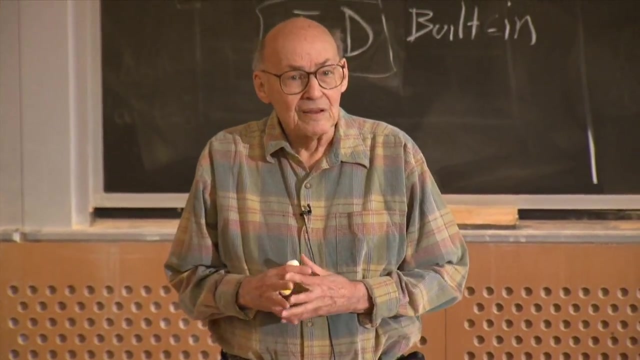 MARVIN MINSKY- What I've forgotten: Self-idealism. MARVIN MINSKY- Yeah, I guess, so It's hard to tell. The reason I had six layers is that, unlike what people do when making theories in science is. 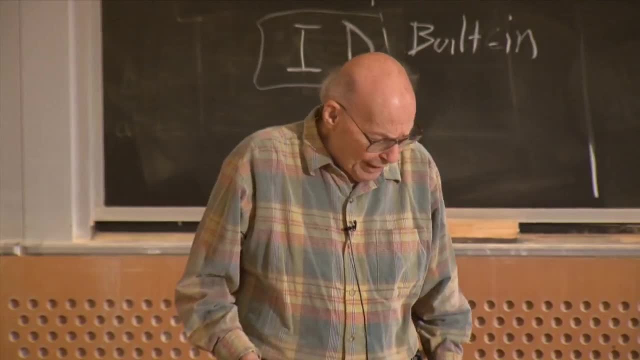 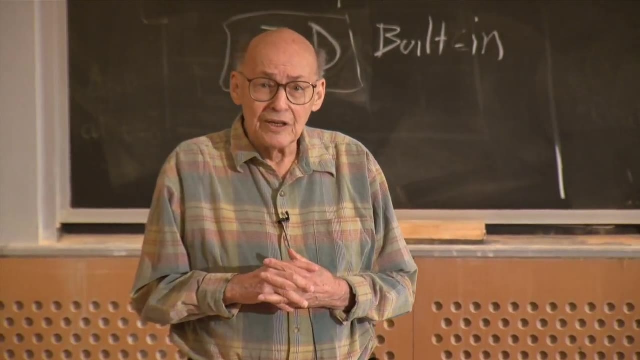 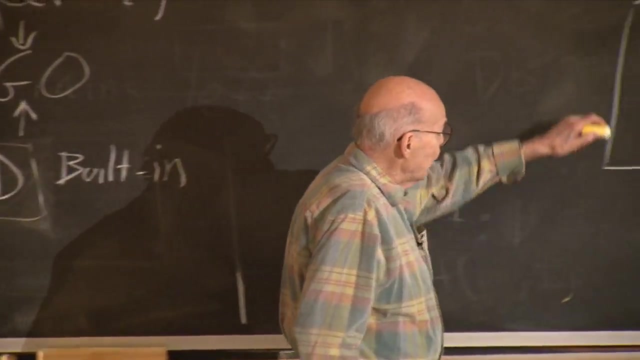 I assume that whatever ideas I have, they're not enough. That is, instead of trying to reduce the mind to as few reactions, as few mechanisms as possible, I think you want to leave room If your theory is to live for a few years. 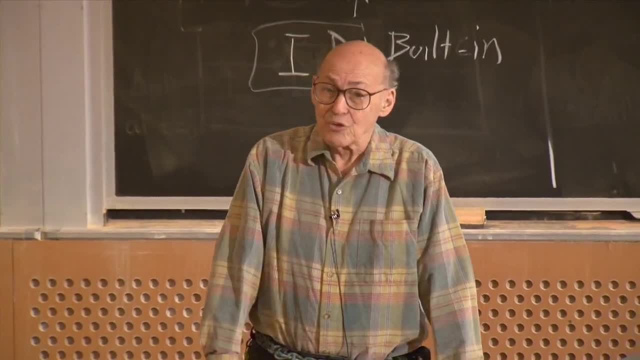 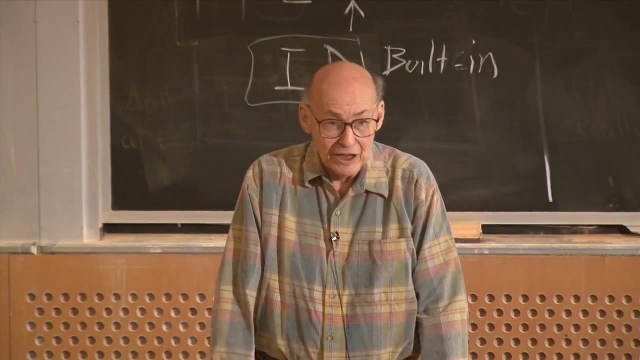 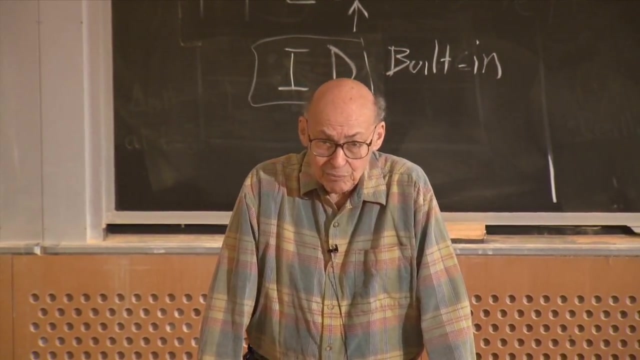 you want to leave room for new ideas. So the last three layers, beginning with reflective thought and self-idealism, are the three layers: Self-reflective and the ideals. It's hard to imagine any clear boundaries And at some point when you make your own theory. 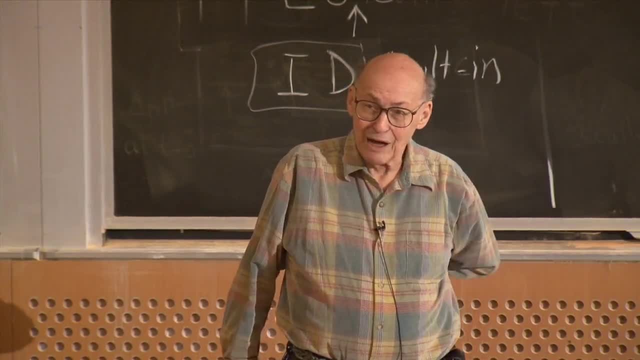 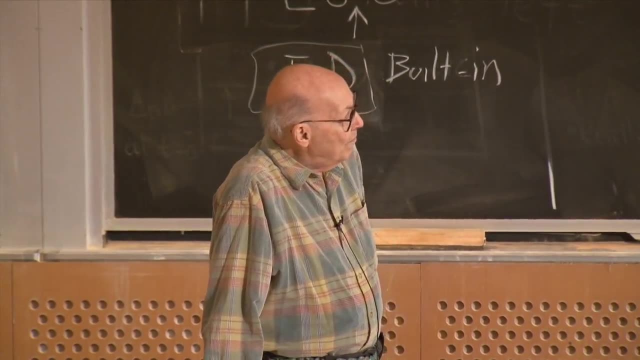 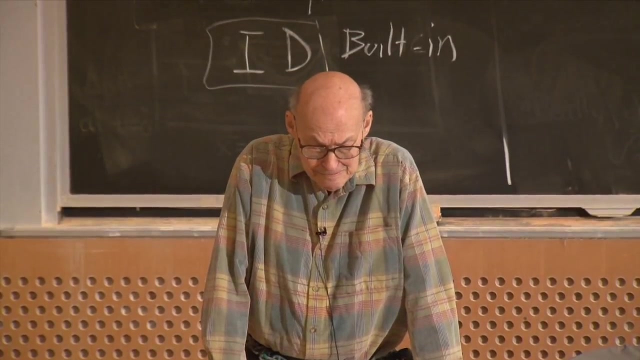 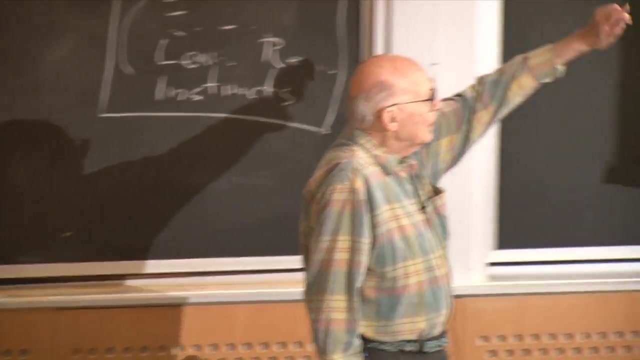 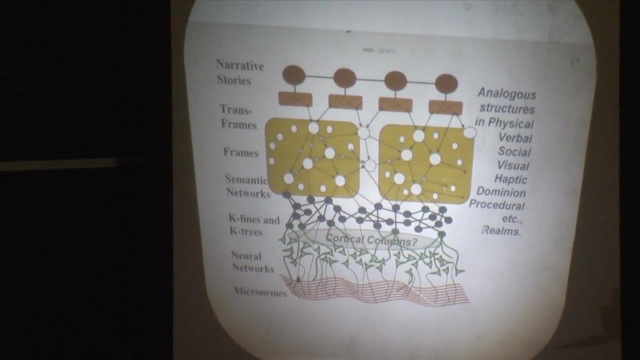 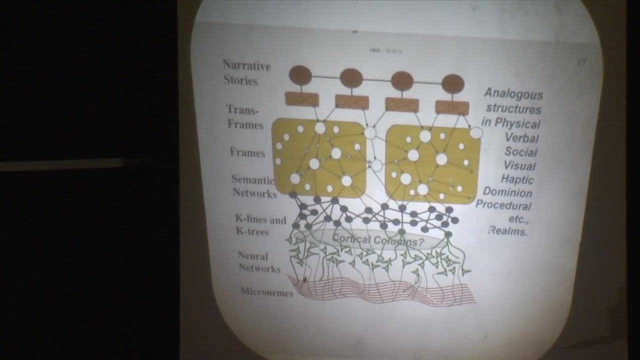 maybe you can squeeze it into these extra boxes that I have. A little later in the book, another hierarchy appears, And that's this is imagining as a functional diagram to show how knowledge or skills or abilities, or whatever you want to call them- the things that people do. 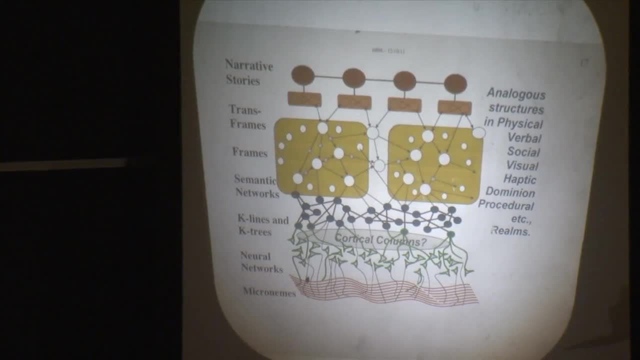 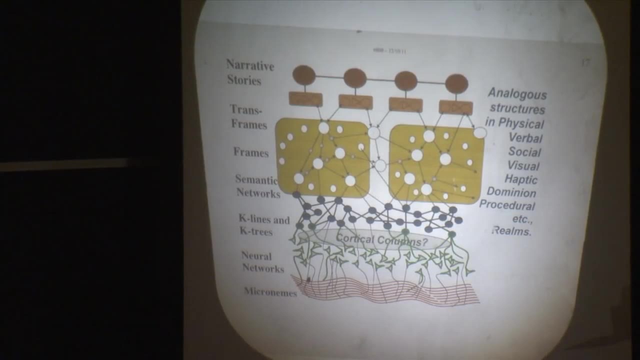 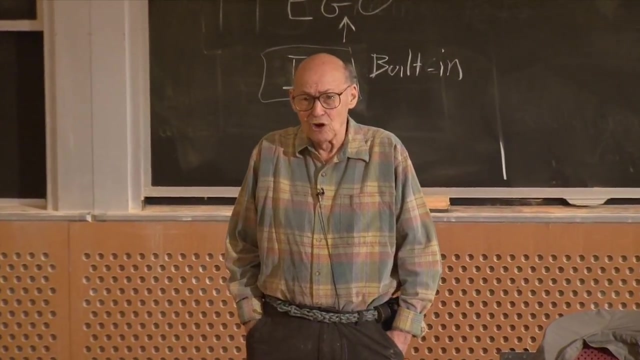 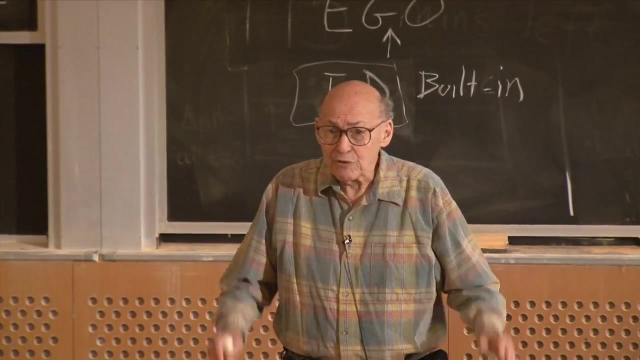 might be arranged, And as far as I know- I don't know, Because virtually every psychologist in the last 100 years has suffered from physics envy- They want to make something like Newton's laws. The result has been that, except for the work of people, 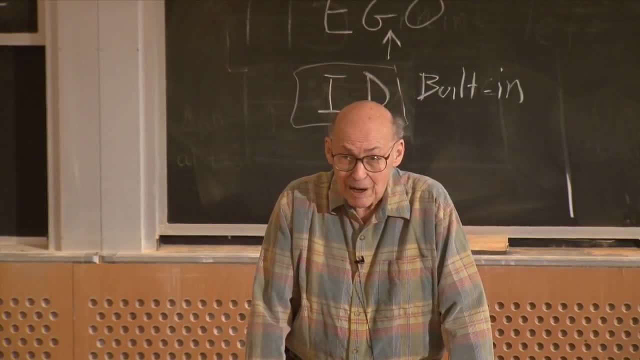 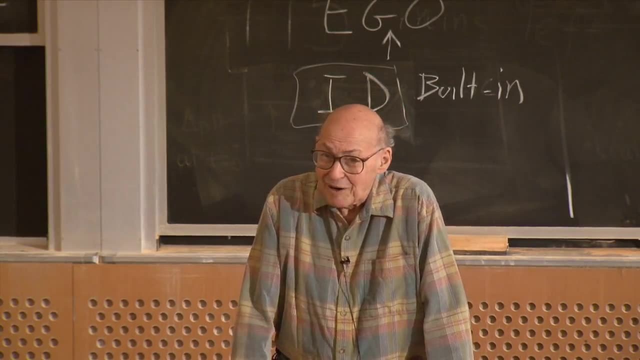 like Newell and Simon and other pioneers who started research in artificial intelligence. there's no way to make something like that, And that's what I'm trying to get at. And that's what I'm trying to get at, And that's what I'm trying to get at. 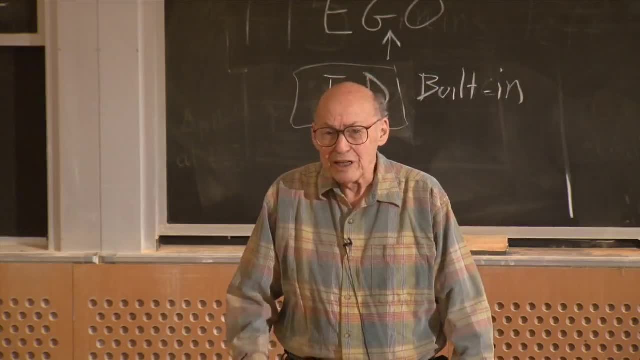 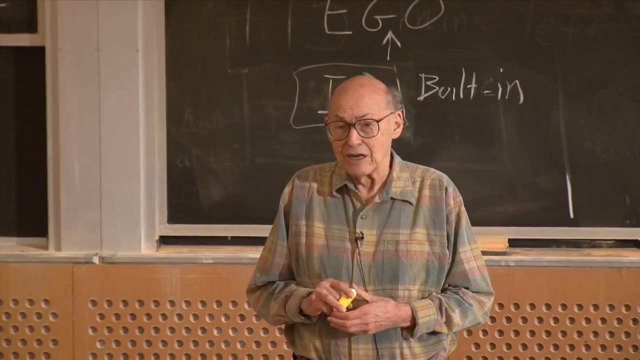 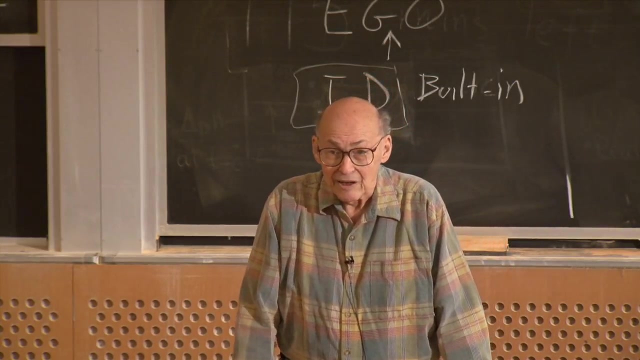 You've heard me complain about neuroscientists, But there's pretty much the same complaint to be leveled against most cognitive scientists who, for example, try to say: maybe the entire human mind is a collection of rules, And if-then rules. 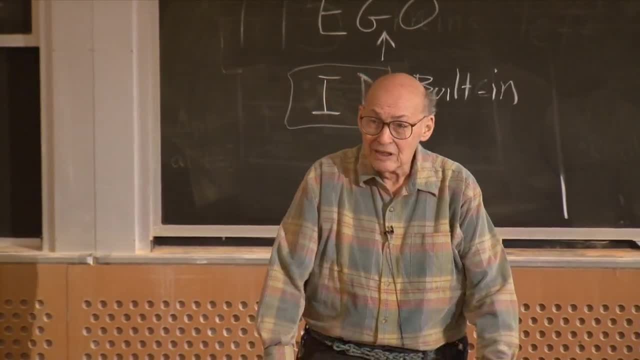 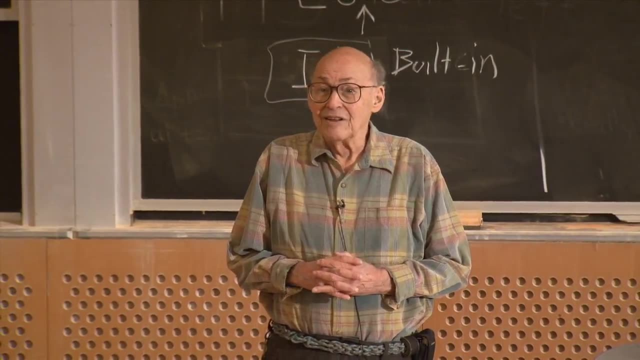 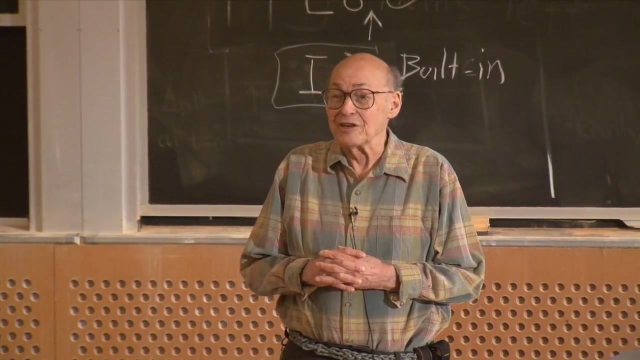 Well, in some sense you could make anything out of if-then rules, But I don't know. But the chances are, if you try to make a learning machine that just tried to add rules in some beautifully general fashion, I suspect the chances are it would learn for a while. 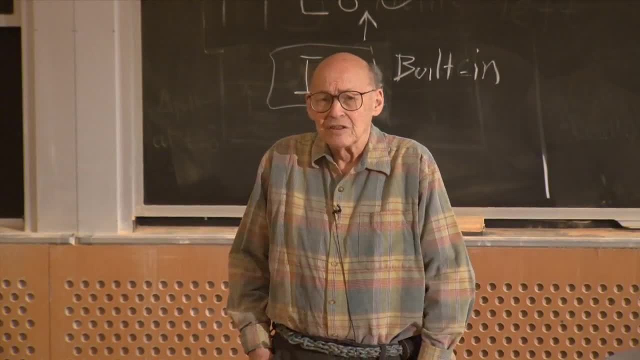 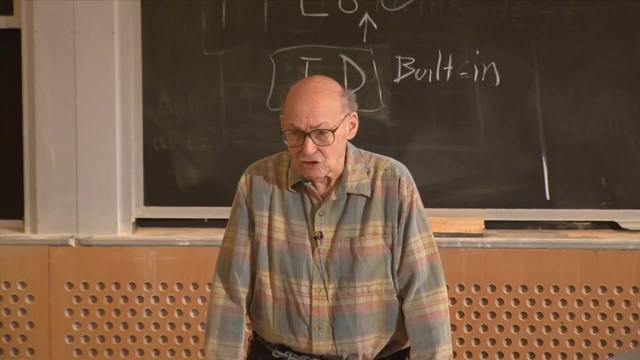 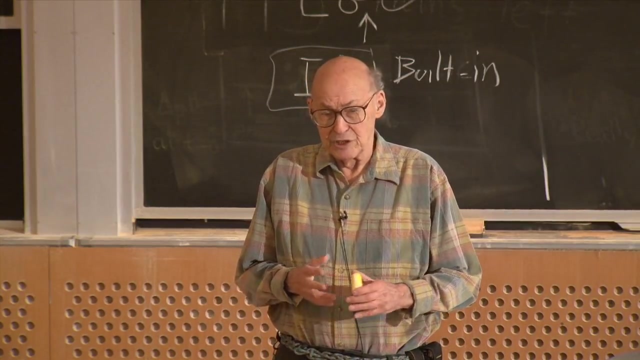 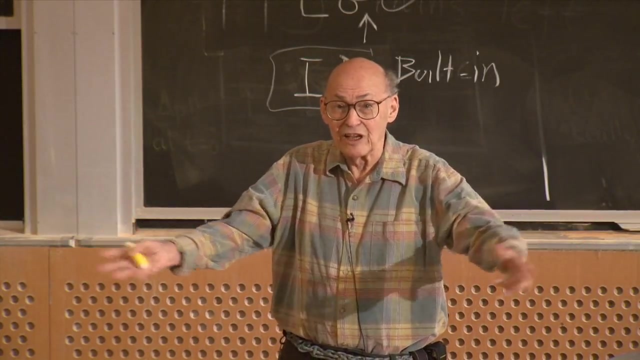 and then get stuck, And indeed that's what happened maybe five or six times in the history of artificial intelligence. Doug Lenat's system called AM, automated mathematician, was a wonderful PhD thesis And it learned arithmetic completely by itself. He just set up the thing biased, so 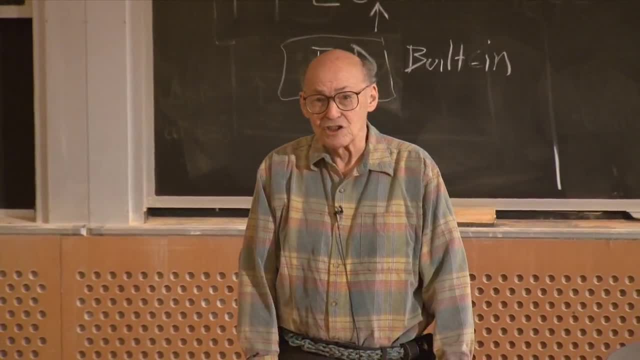 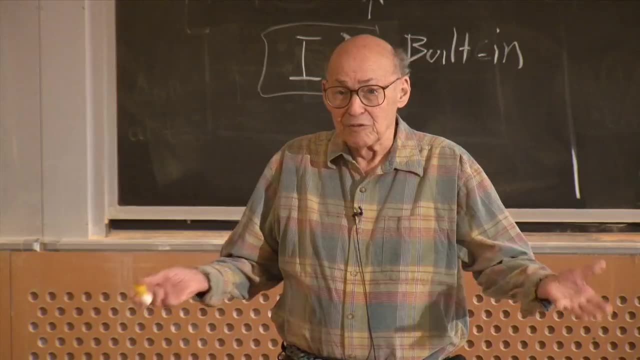 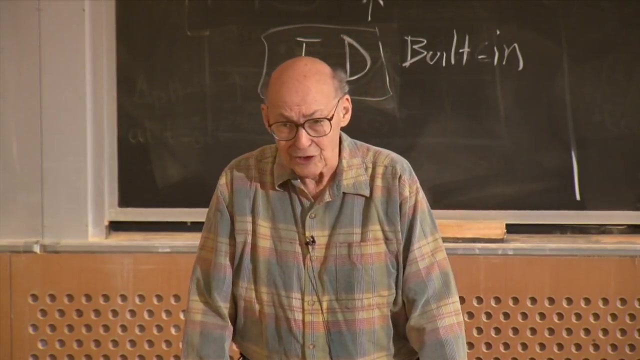 that it would have some concept of numbers like 6 is the successor of 5, and stuff like that, And it fooled around And And discovered various regularities. I think I mentioned it the other day- It first developed the concept of number. 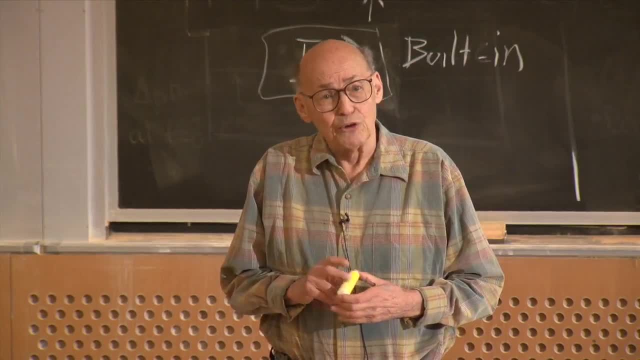 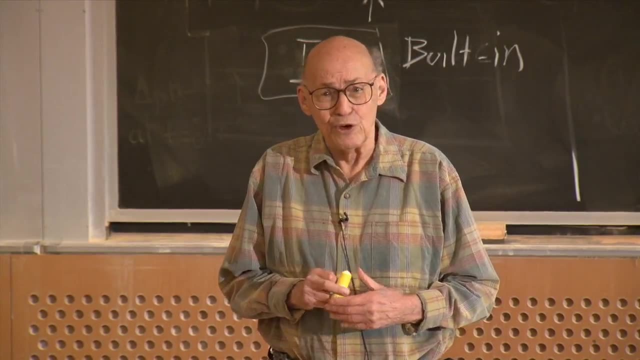 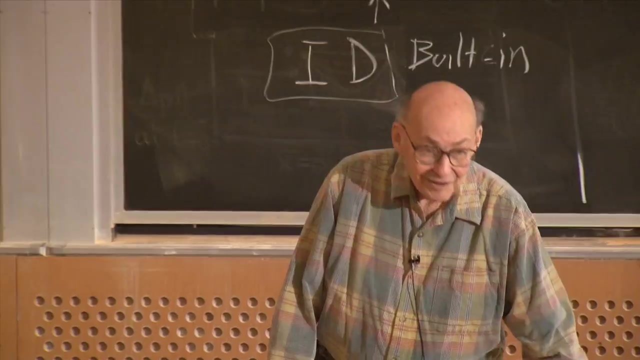 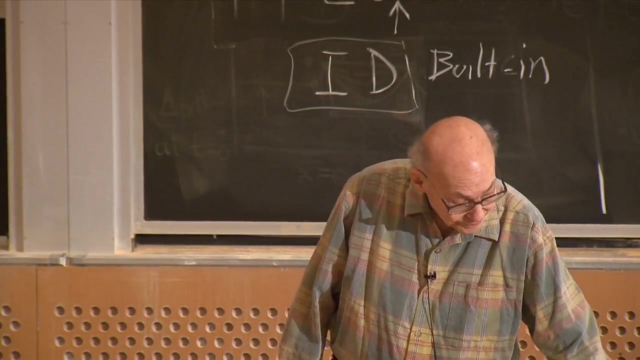 which wasn't very hard, because he wrote the whole thing in the AI language called LISP. How many of you know LISP? That's a lot In looking at the biographies of the late John McCarthy. all week there were lots of attempts by the writers. 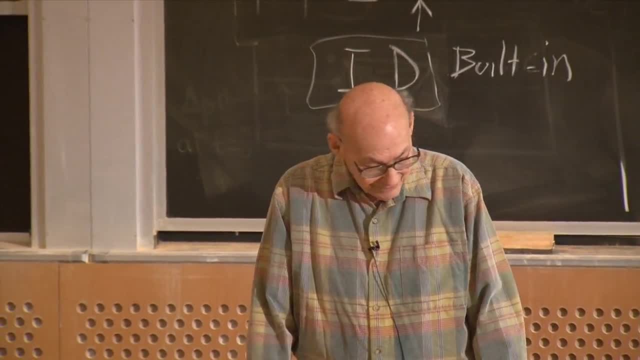 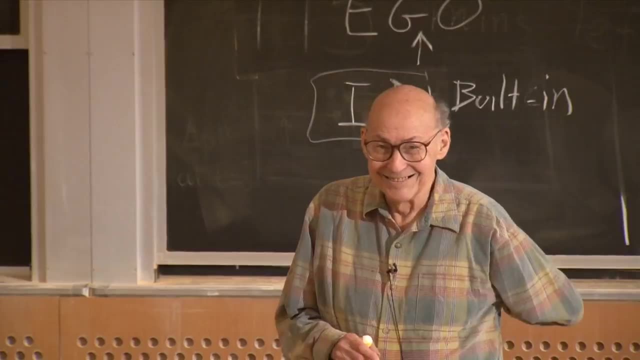 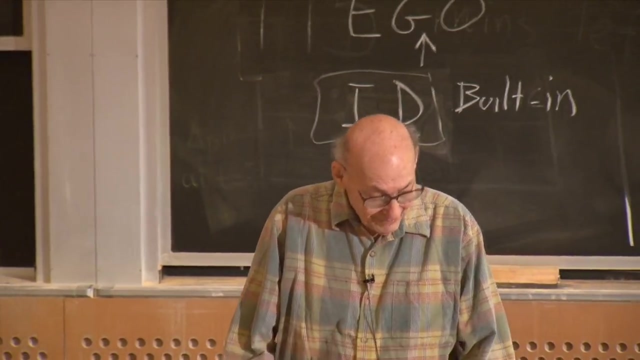 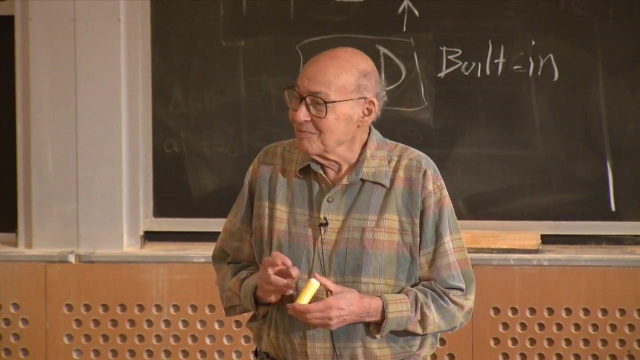 to say what LISP was. The tragedy is. you probably could have described it exactly in a paragraph. It's because it's saying that each structure has two parts and each of those has two parts, And I don't remember seeing any attempt. 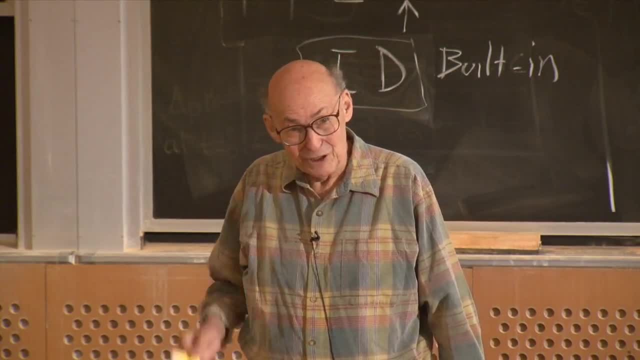 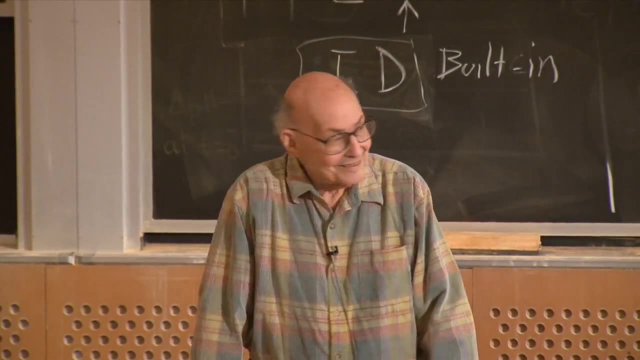 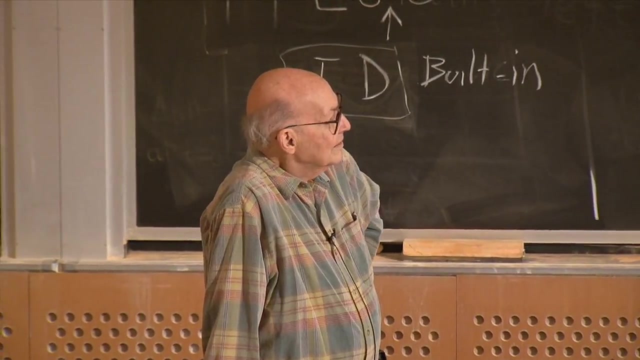 to say something about this programming language. Yes, How do you imagine the layers interact with each other? MARVIN MINSKY- Those, Yeah, those and those the six layers. MARVIN MINSKY- I think they're layers of organization. 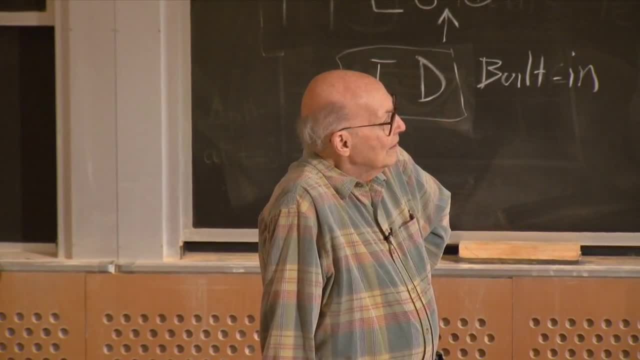 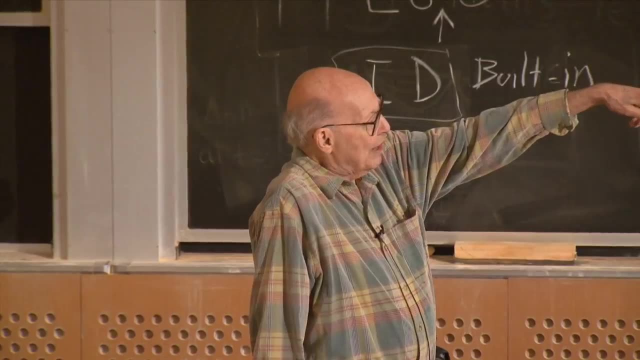 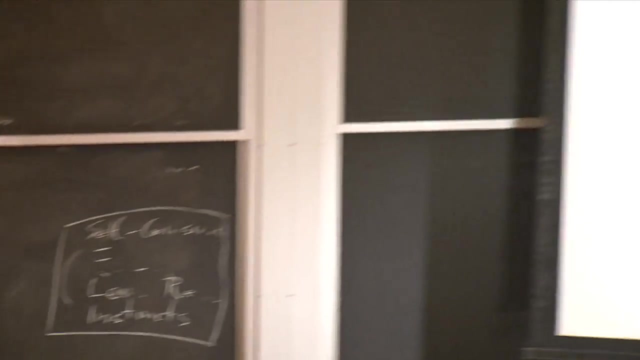 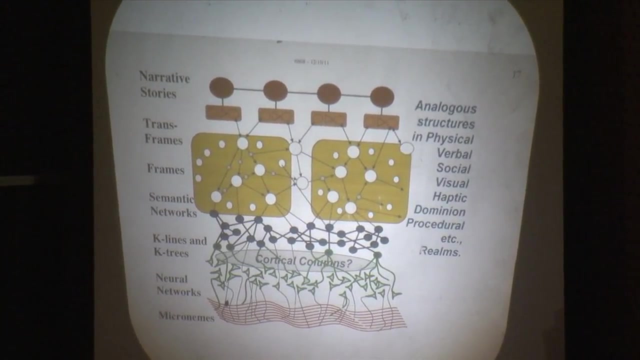 I think they're layers of organization. But yes, because the trans frames. a trans frame is made of two frames. But then if there were a neuroscientist who said: oh, maybe when you see an apple and you're hungry, you reach out and eat it. 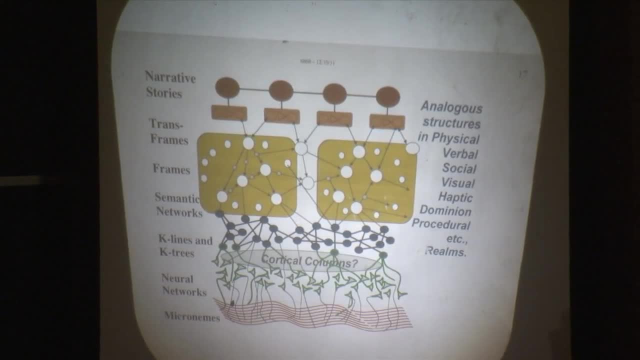 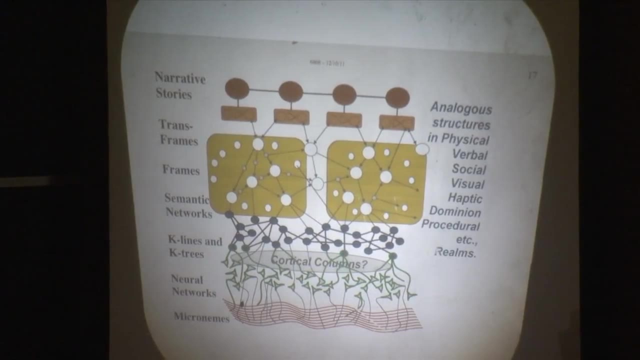 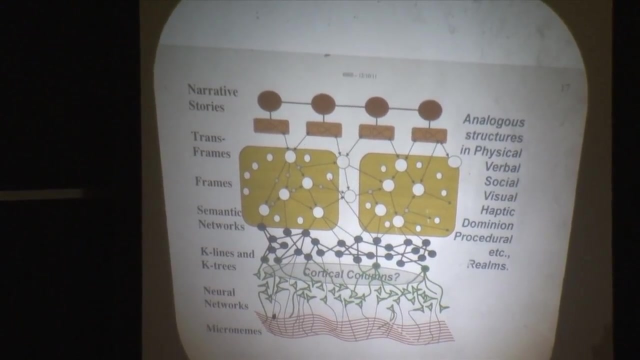 MARVIN MINSKY- Yeah, MARVIN MINSKY- So So you could think of that as a simple reflex: if this, then that. Or you could say: if I'm hungry now and I want to be not hungry, what's a possible action? 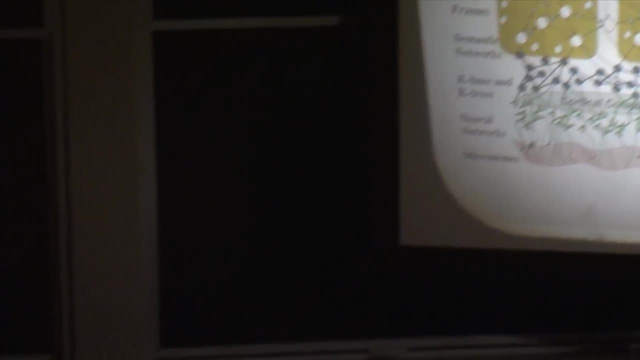 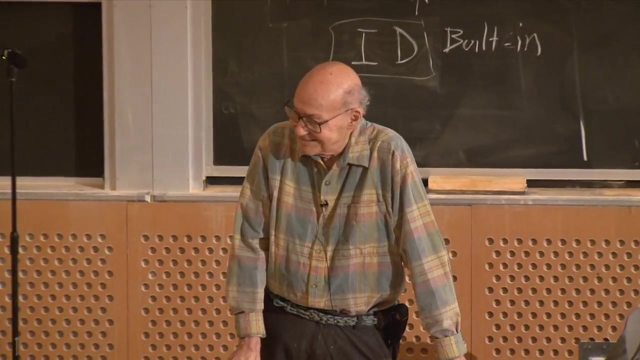 could I do, And that action might be: look for an apple or yes. So I was teaching my class on the day that McCarthy passed away, and then I was explaining, And then I have. I had some students in the class who weren't even computer scientists. 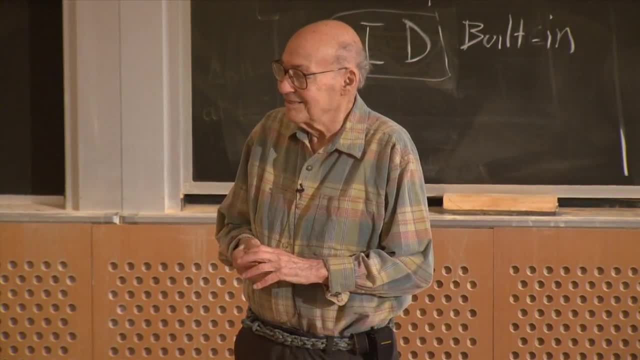 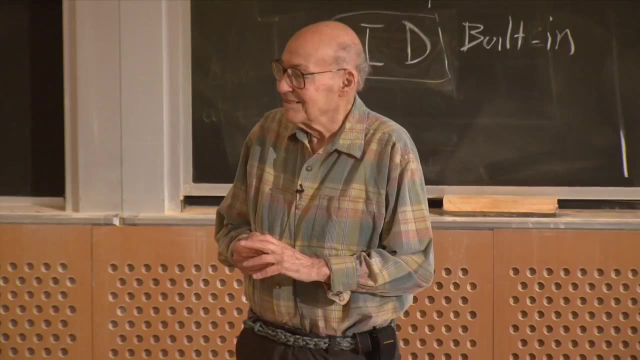 And so I was thinking about the same problem, which is, how do I explain what Lisp was? And I remember, and so I said well before that there were languages like Fortran that manipulated numbers. Lisp was the fourth first language to manipulate ideas. 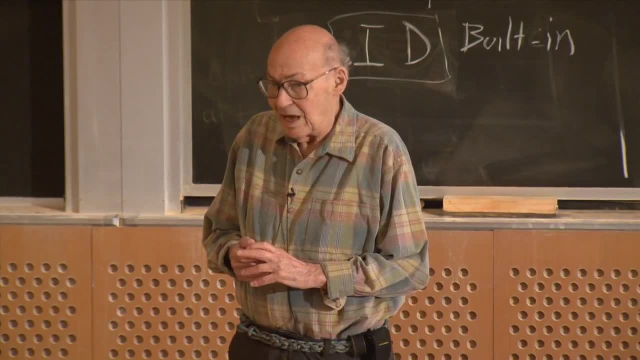 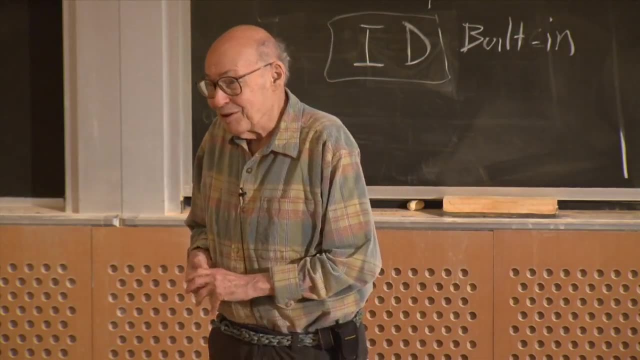 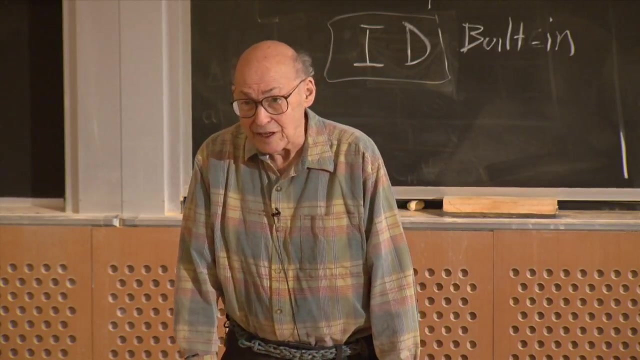 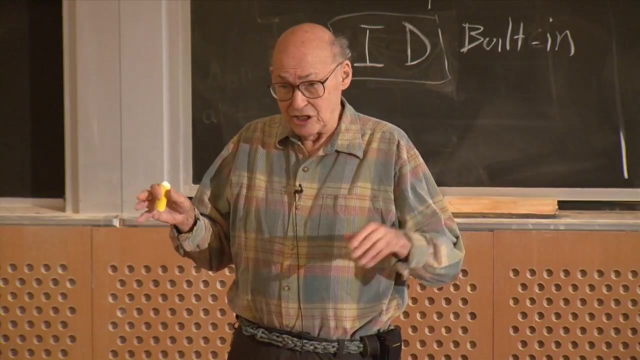 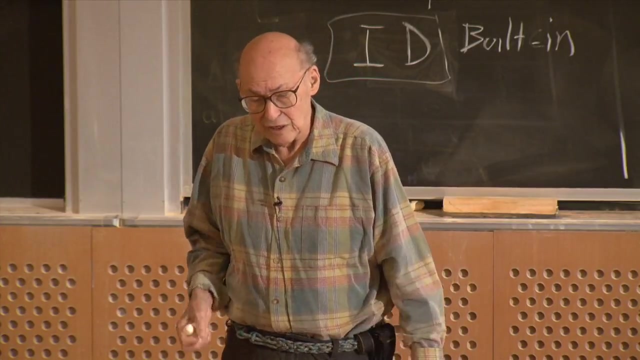 MARVIN MINSKY- Mm-hmm, Yes, it can manipulate representations of. yes, it's manipulating the ideas that are represented by these expressions. And one thing that interests me is another analog between psychology and modern cognitive psychology and computer science or artificial intelligence. 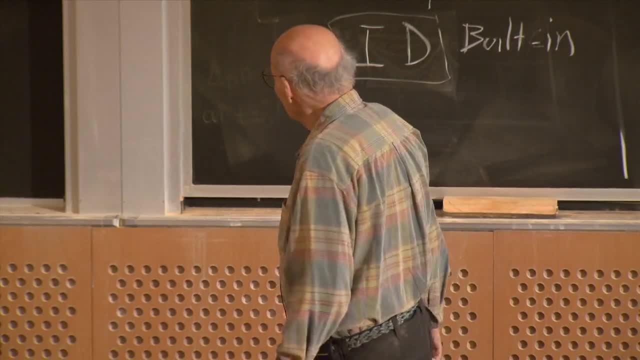 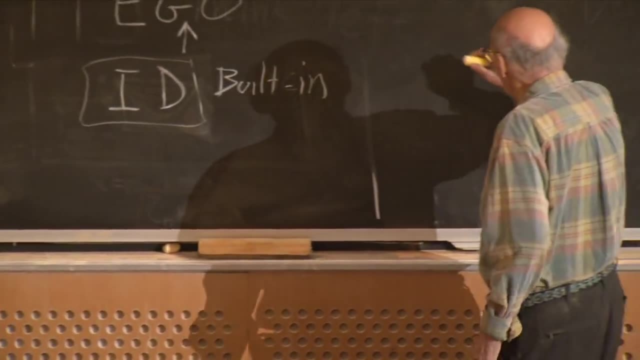 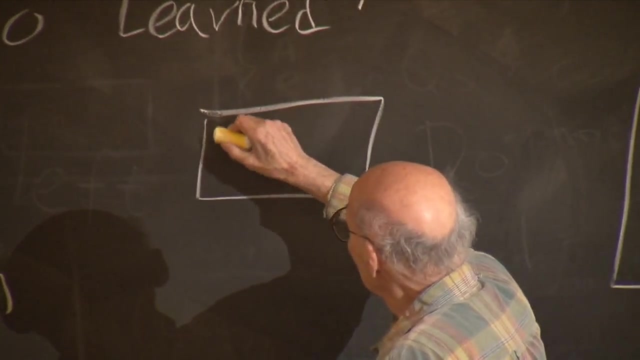 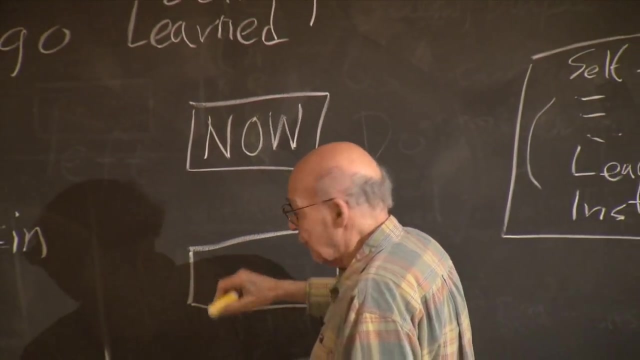 is the idea of a goal. where? what does it mean to have a goal? And you could say It's a piece of machinery which says that if there's a situation, what you have now, and if you have a representation of some future thing. 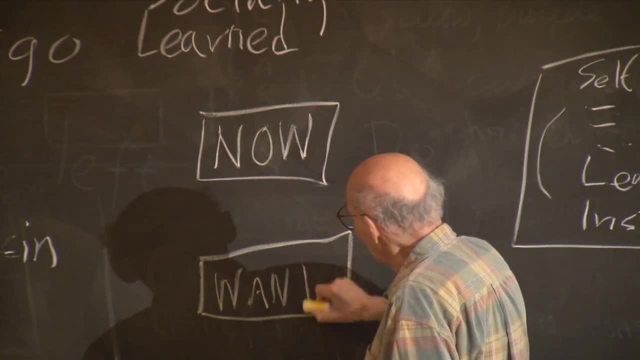 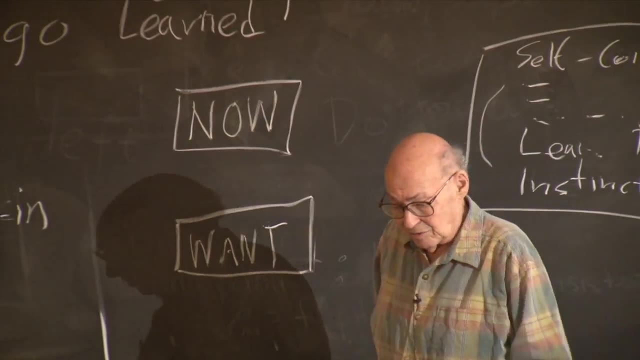 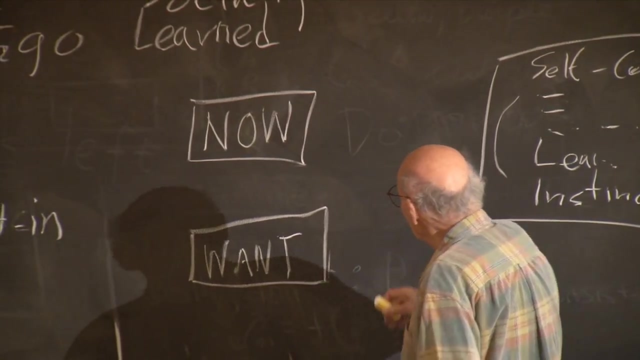 what you want. So, of course, at any time you're in a situation that your brain is somehow representing Maybe five or 10 ways, not just one. But what does it mean to have a goal? And what it means is to have two representations. 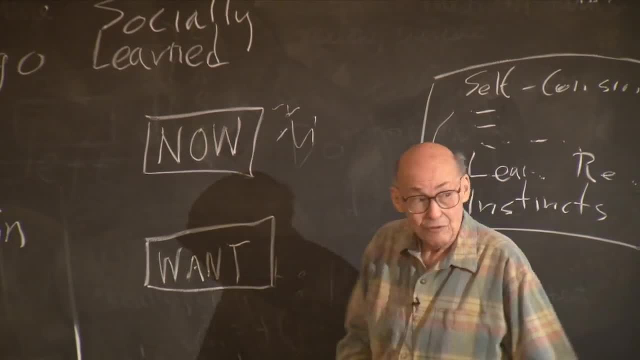 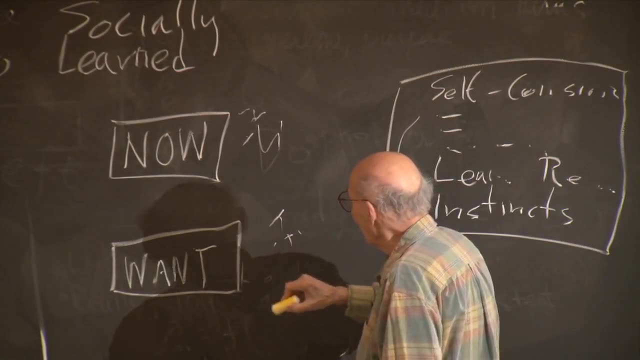 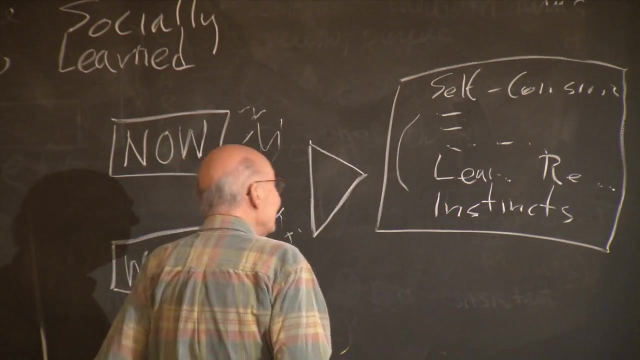 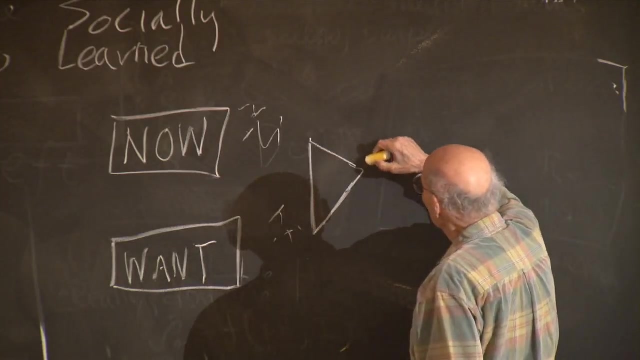 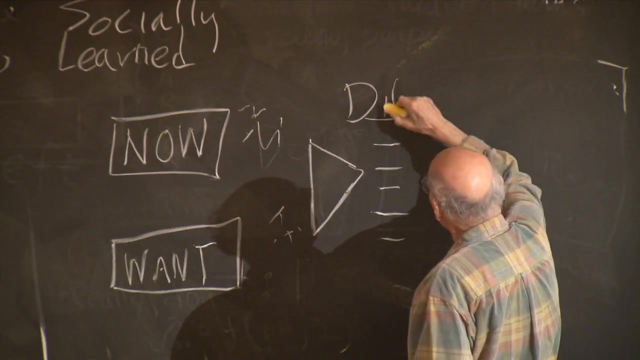 One is a representation you've made of some structure which says what things are like now, And the other is some representation of what you want, And I don't think I need that. And the important thing is: what are the differences? And instead of saying what's the difference, 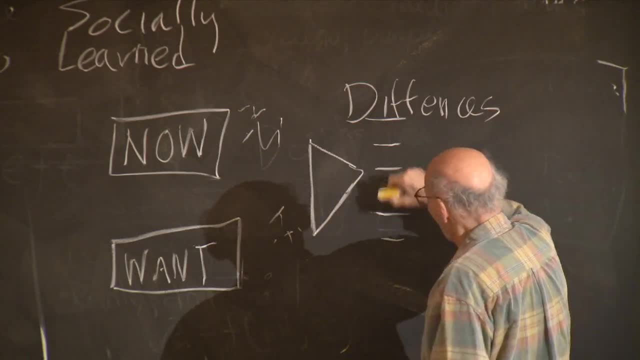 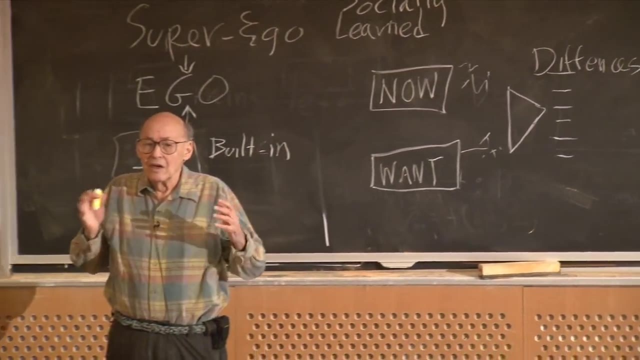 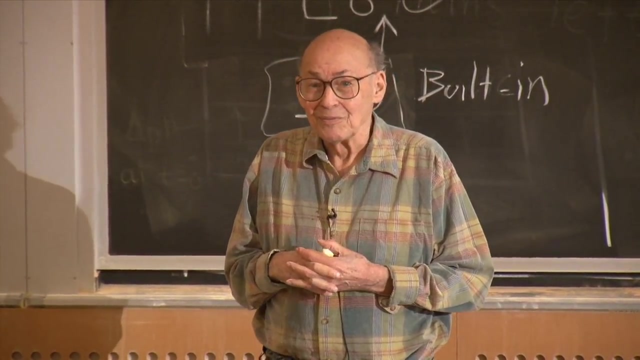 maybe it's good to say what are the differences. So what does it mean to have a goal? It means to have some piece of machinery turned on. You can imagine a goal that you don't have, right Like I can say what's David's goal? 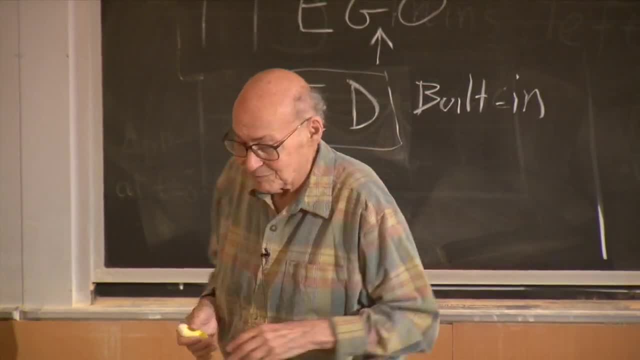 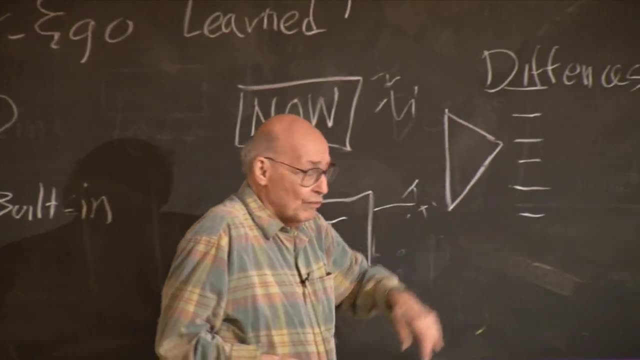 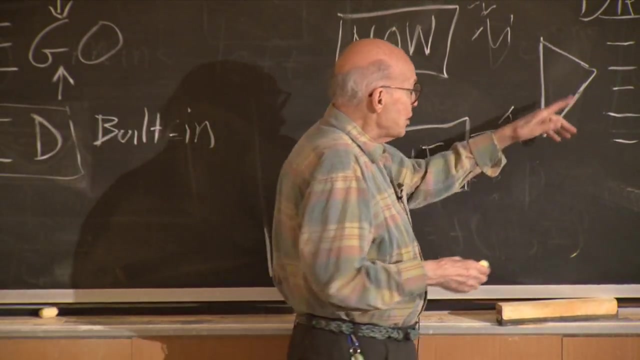 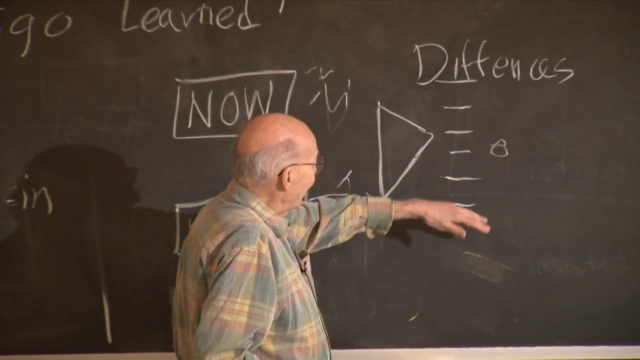 It's to get people to go to that meeting. So what you want is to minimize the differences between what you have and what you want, And so there has to be a machinery which does what: It picks out one of these differences and tries to get rid of it. 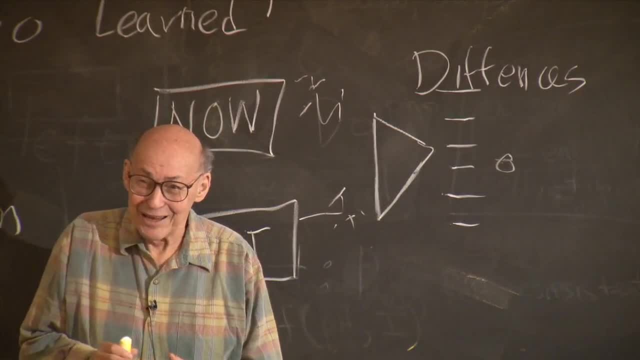 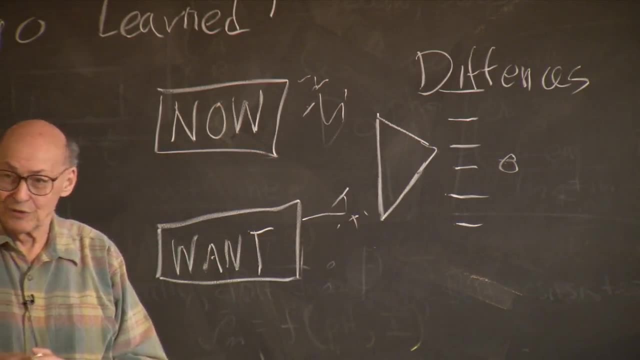 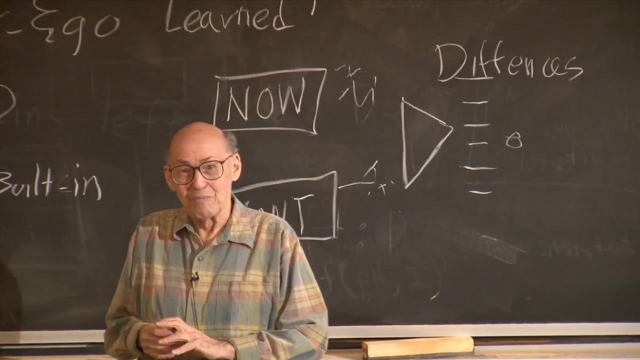 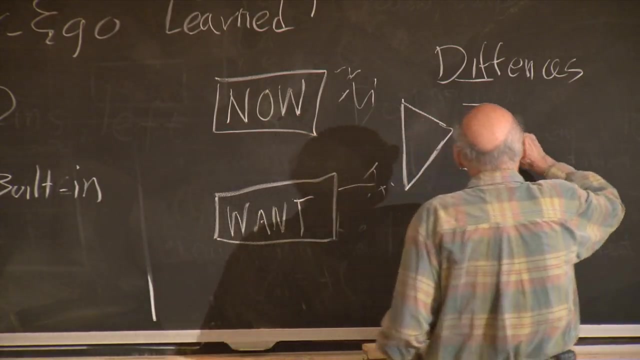 And how can you get rid of it? There's two ways. The good way is to change the situation so that difference disappears. The other way is to say, oh, that would take a year. I should give up that goal And I'm digressing. 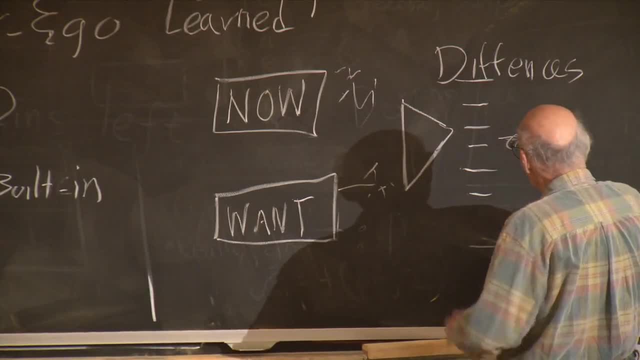 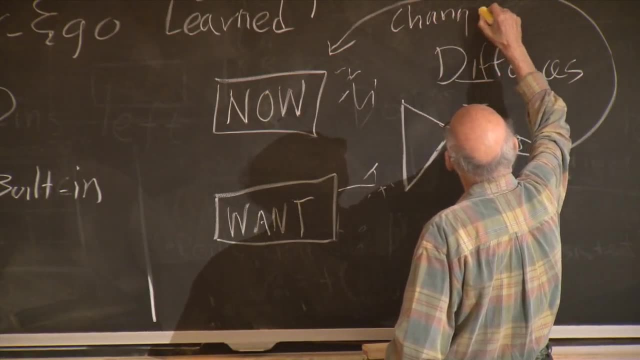 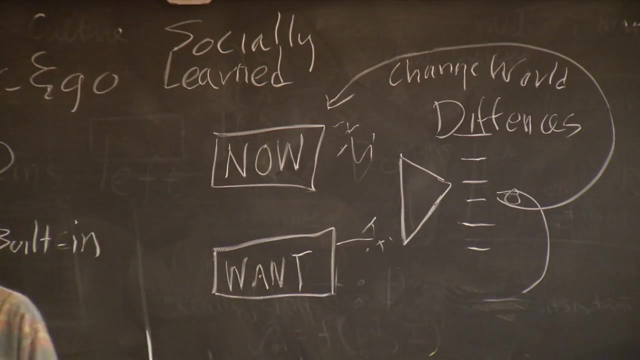 So you want something that removes, and I'm going to give up that goal. The feedback has to go this way: Let's change the world and get rid of that difference. So well, how do you get rid of the difference? That depends on: maybe you have a built-in reflex, like 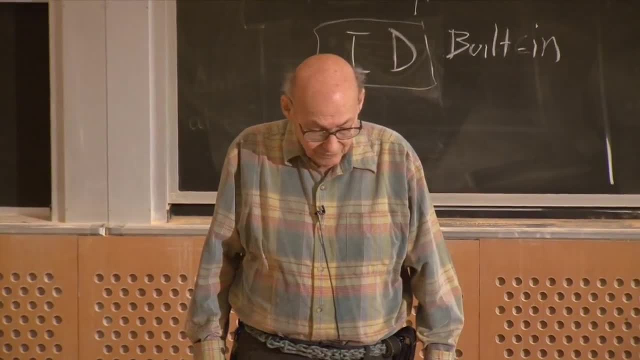 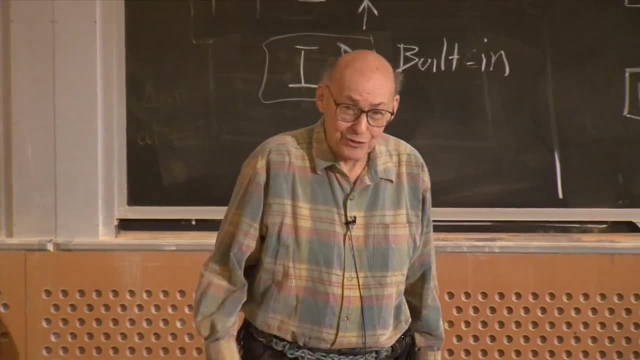 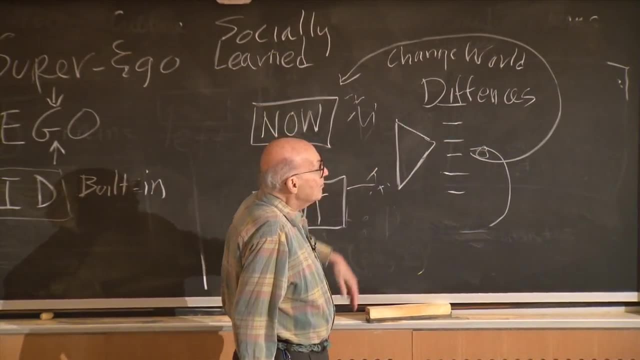 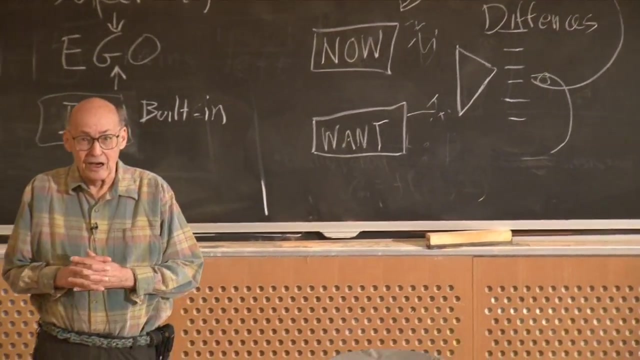 something senses it and tells you to breathe. So you've got built-in things And the question is, how do you represent these sorts of things? And in fact, I think I got a lot of this idea from the PhD thesis of Patrick Winston, who 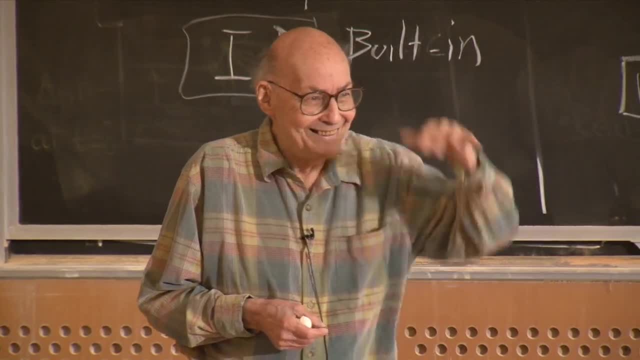 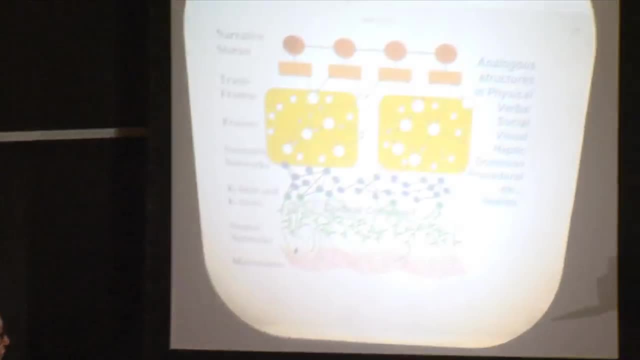 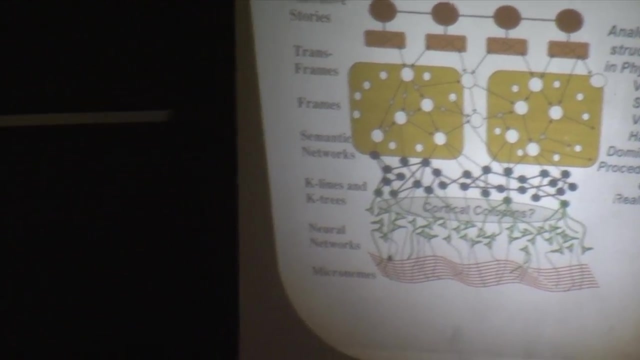 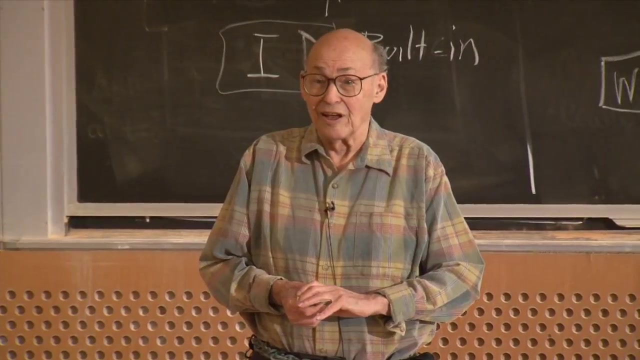 was here a minute ago. But the question is, how do you represent what you want And how do you represent what you have? And I think the big difference between people and other primates and reptiles and amphibians, reptiles, fish. 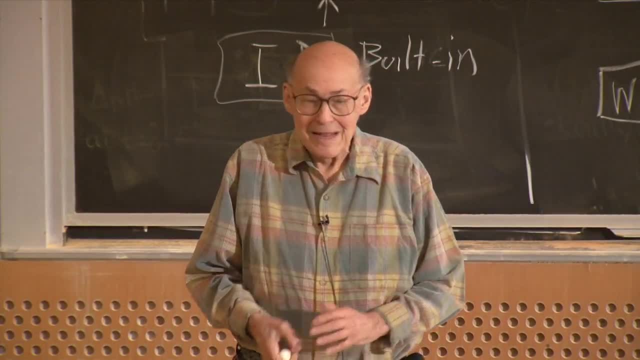 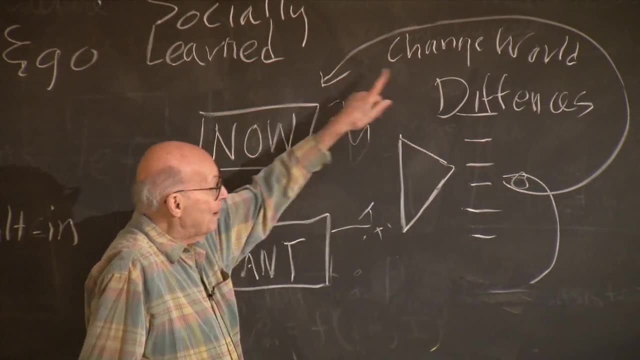 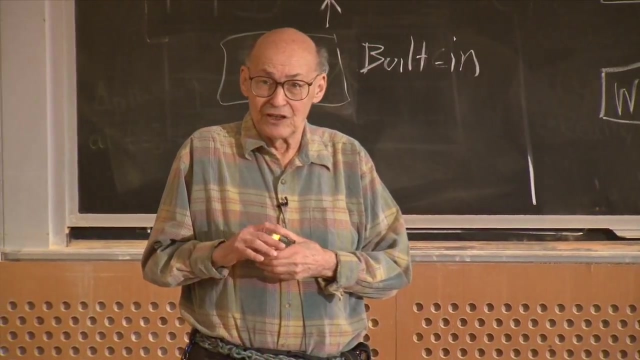 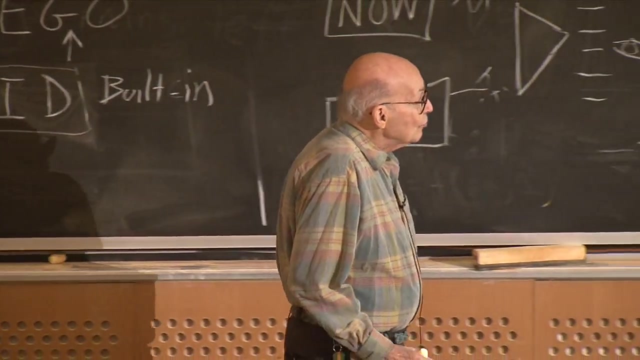 and going back to plants and so forth, is that we have these very high level, powerful ways of representing differences between things, And this enables us to develop reflexes for getting rid of the differences. So this is what I think might be a picture of how 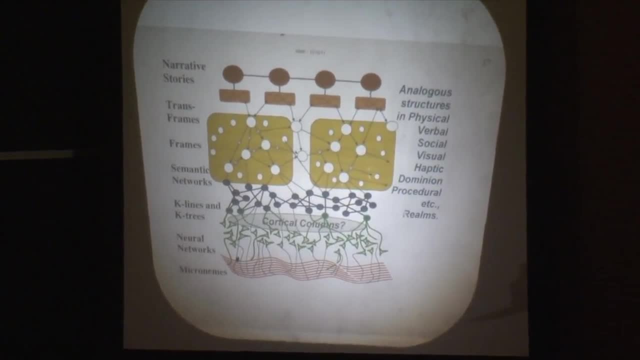 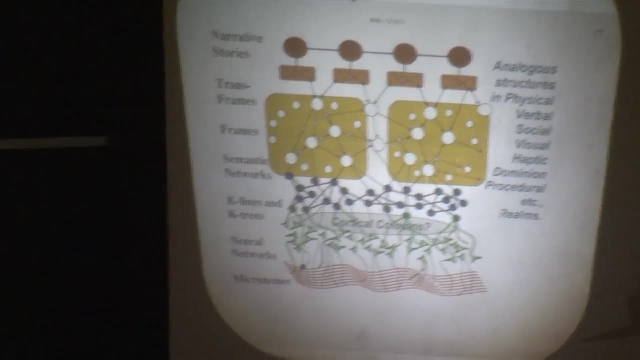 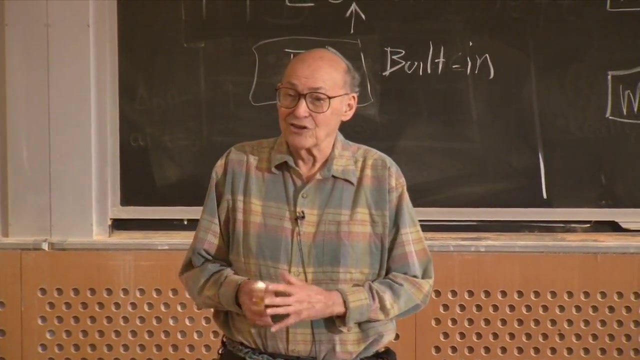 the brain is organized, And at every level. these things are made of neurons. But you shouldn't be looking at the neurons individually to see how the brain works. It's like looking at a computer and saying, oh, I understand that. All I have to do is know a great deal about how. 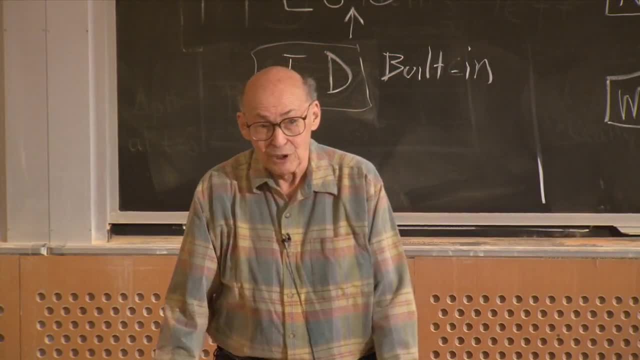 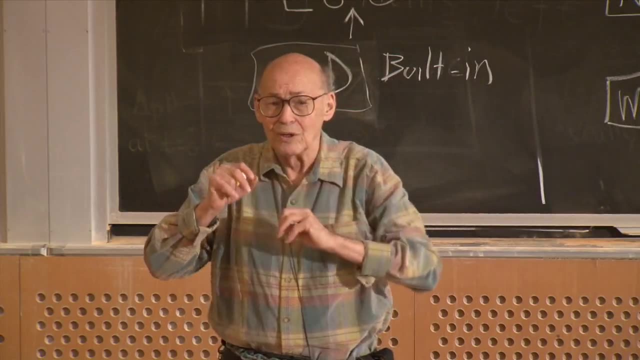 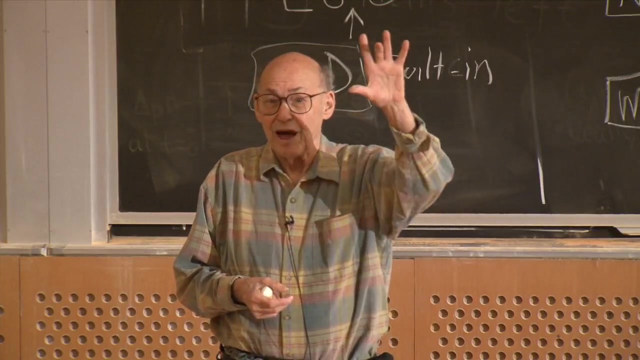 each transistor works. The great thing about a computer is that it doesn't matter how the transistor works. The important thing is to recognize. oh look, they usually come in pairs, Or really four or 10 or whatever called a flip-flop. 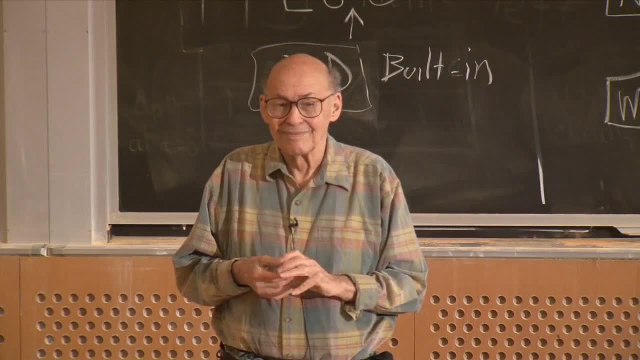 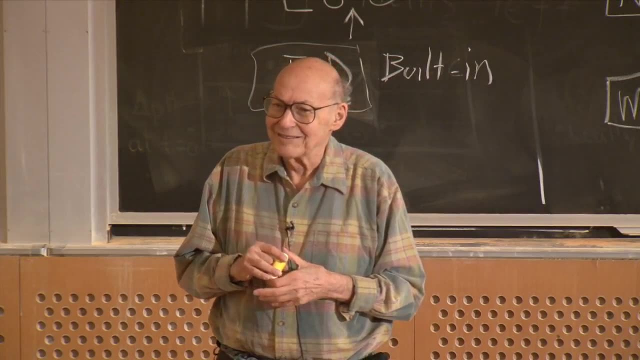 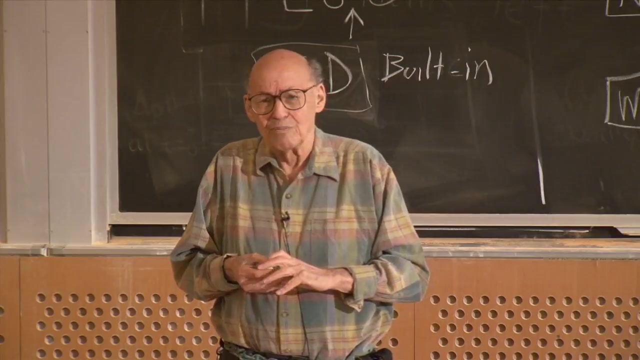 And do you ever see a neuroscientist saying: where are the flip-flops in this or that? It's very strange. It's as though they're trying to develop a very powerful computer without using any concepts from computer science. It's a marvelous phenomenon. 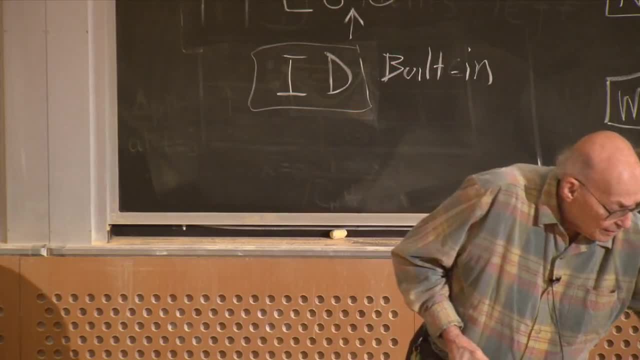 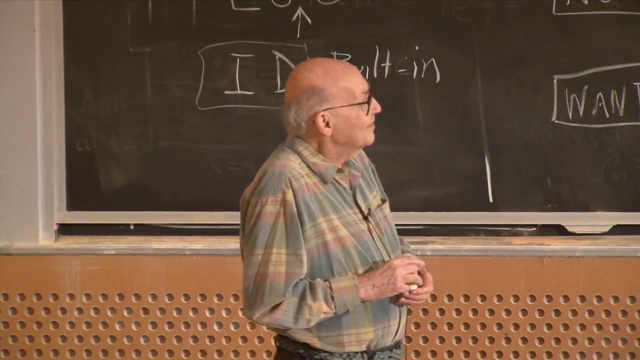 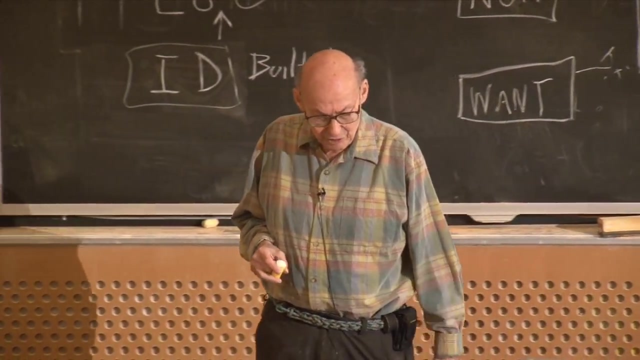 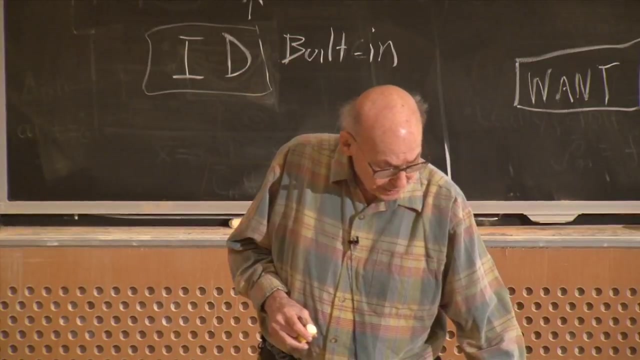 And You have to wonder: where did they grow up And how did they stay? isolated? In biology departments, I think, biology departments Or psychology departments. Well, I started out in biology pretty much, And then I ran across these early papers, one of which 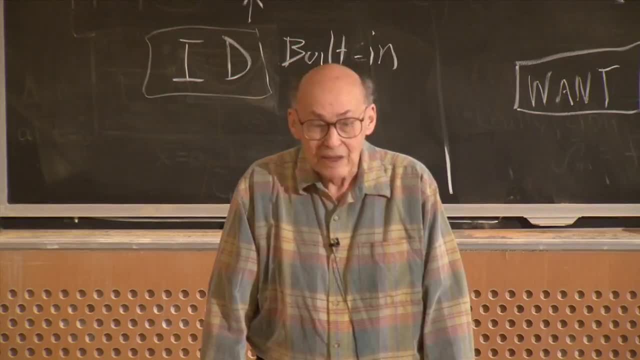 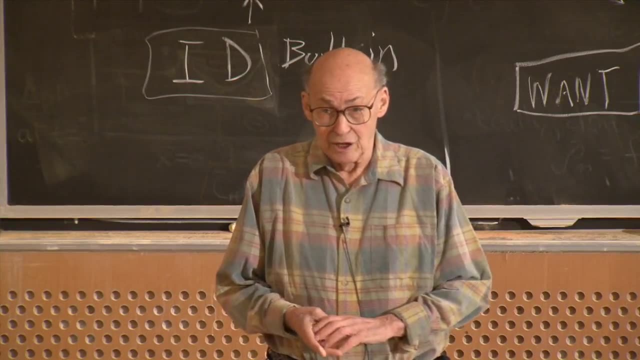 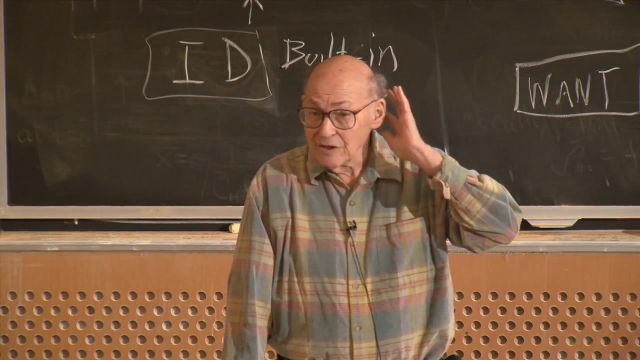 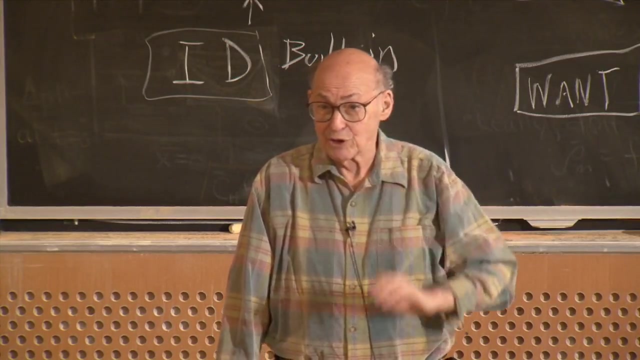 was by Letvin. It was a paper by McCulloch and Pitts and people like that. In the early 1940s the idea of symbolic neurons appeared. It had first appeared in 1895 or so with the paper that Sigmund Freud wrote but couldn't get published. 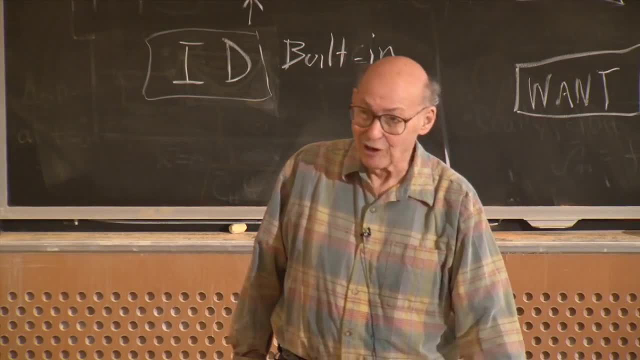 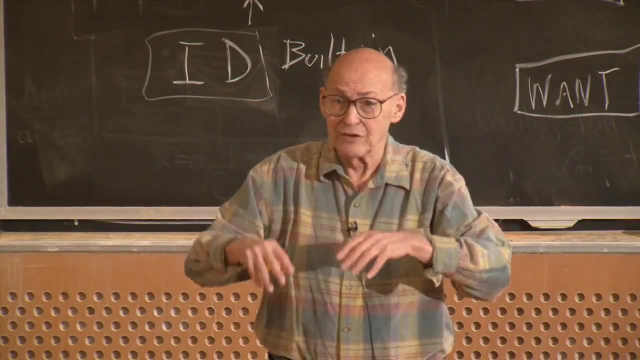 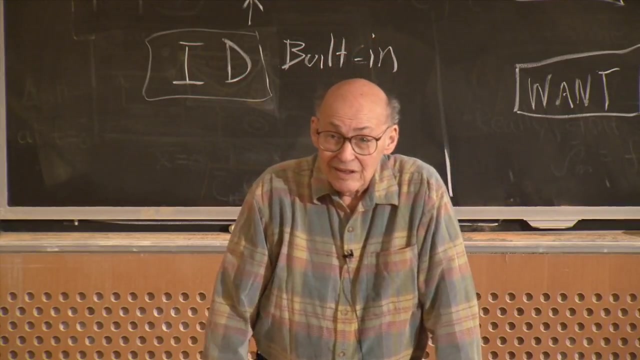 I think I mentioned that called Project for a Scientific Psychology And it had the idea of neurons, The idea of neurons with various levels of activation, And sometimes you would have a pair of them and one would be inhibiting the other, And so that could store some information. 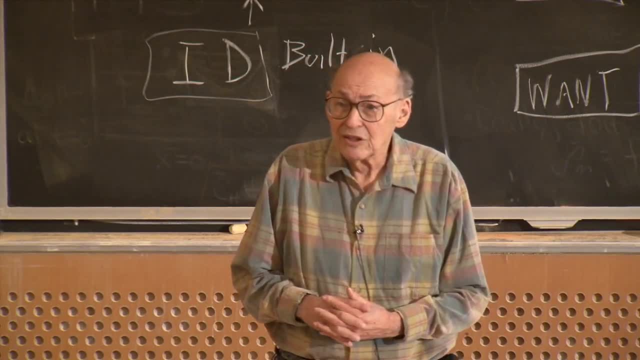 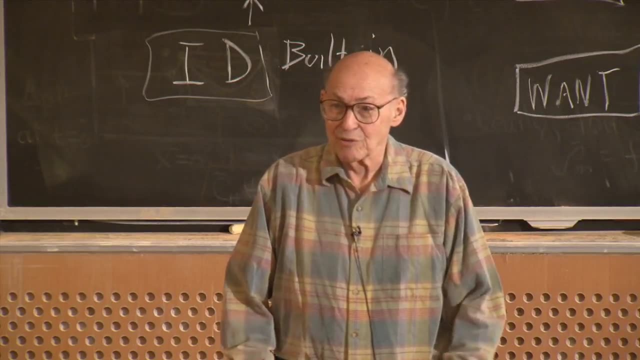 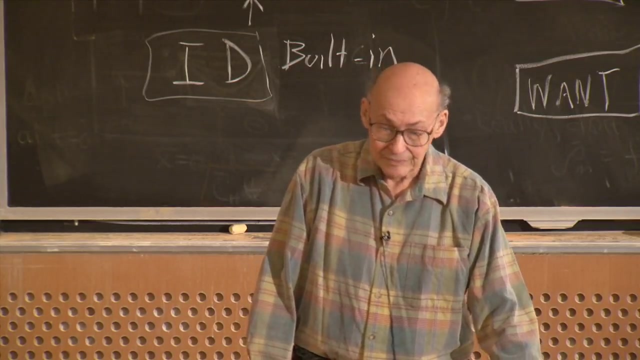 And he's not very explicit about how these things might work, But as far as I know, it's about the first attempt to have a biological theory of information processing at all, And he was unable to get it published. Yeah, Marvin, Yeah. 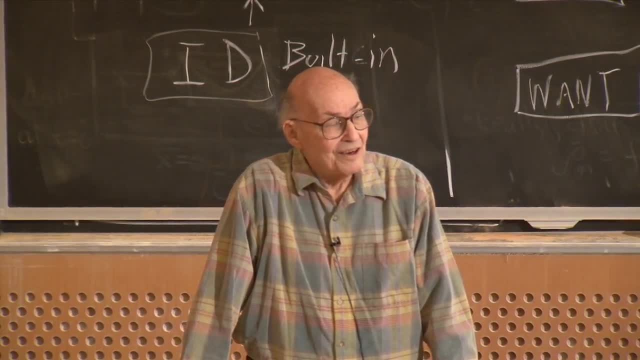 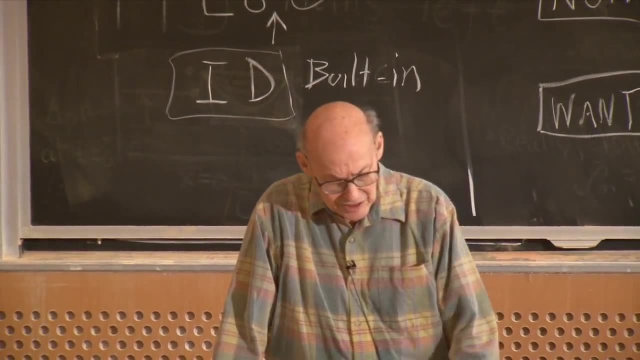 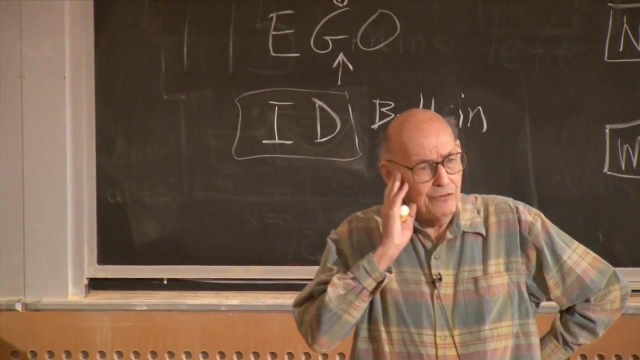 I want to interrupt a little bit, Since McCarthy did this. just the idea. do you have any summary reflections on the stuff that he did or his contributions? MARVIN MINSKY- There are a lot of things that he did And I noticed that none of the obituaries. 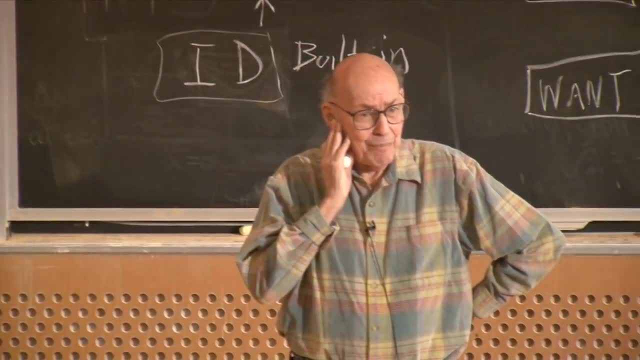 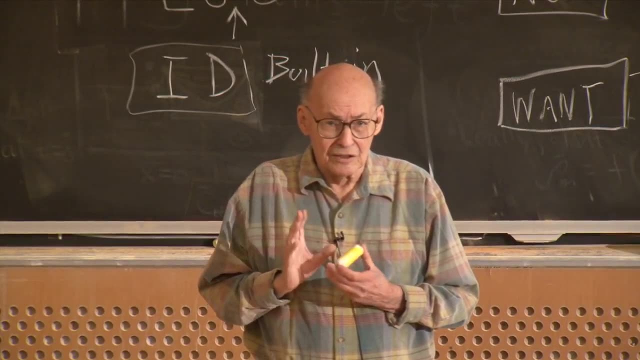 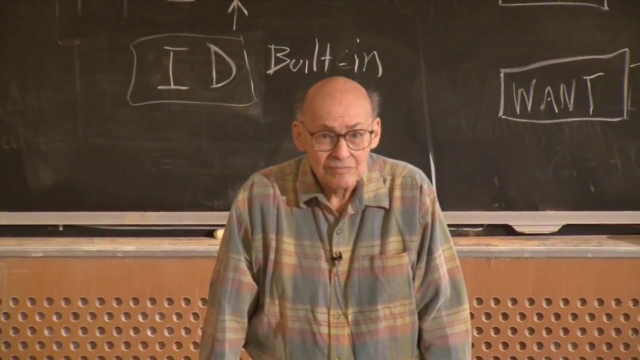 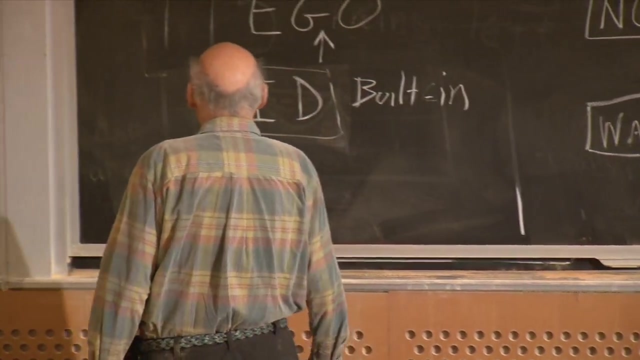 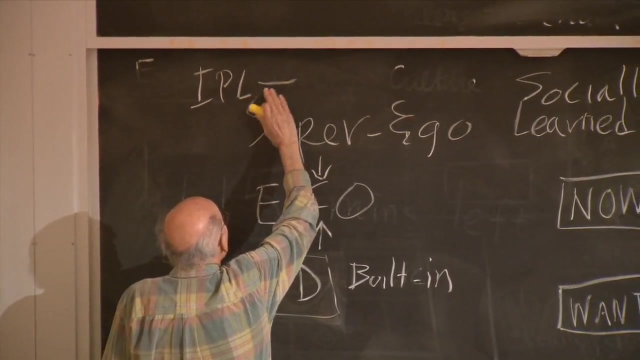 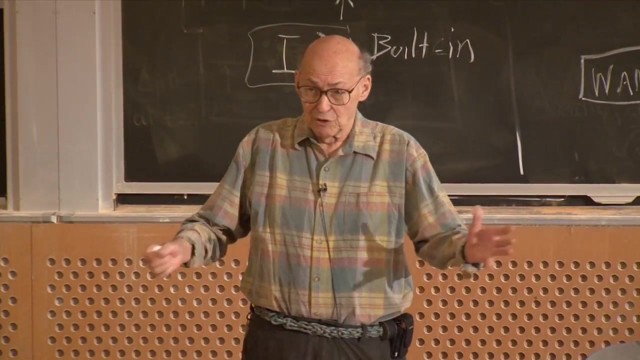 actually had any background. What had happened is that Newell and Simon had started to make- they had struggled to make programs that could do symbolic logic And they made a language called IPL, And IPL was a language of very microscopic operations. like you have several registers. 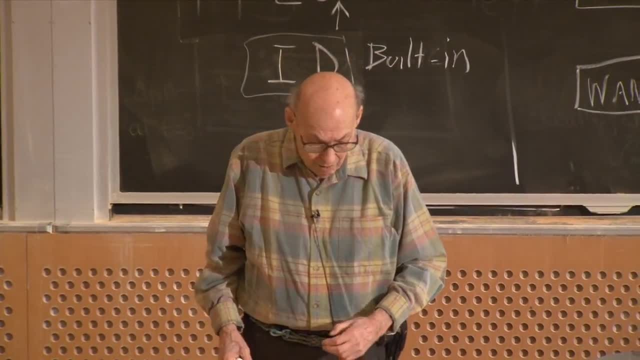 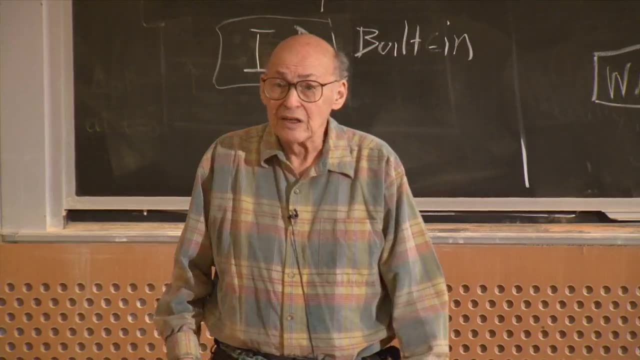 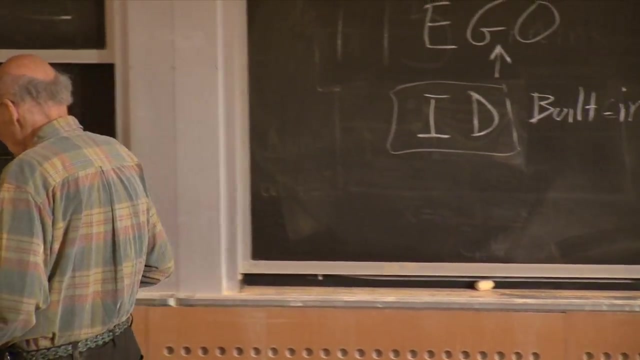 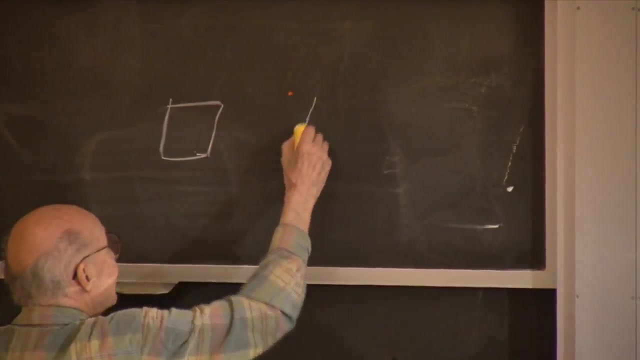 Put a symbol in a register, perhaps do a piece of arithmetic on two symbols, if they're numbers. If not link up, You could sort of make registers artificially in the memory of the computer And you could take two or three registers and you could. it had instructions. 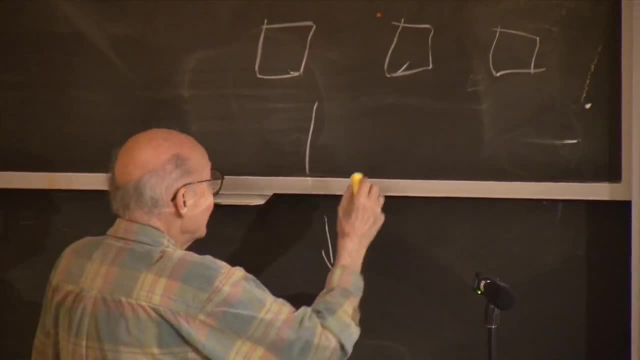 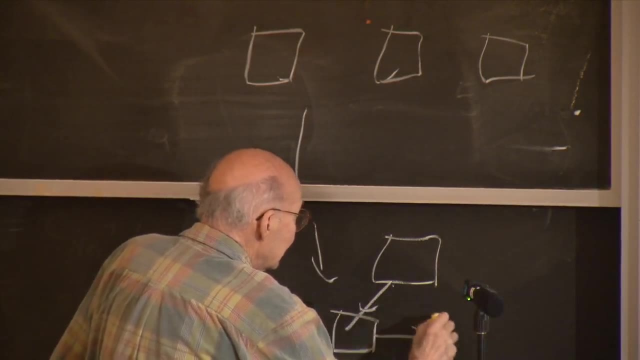 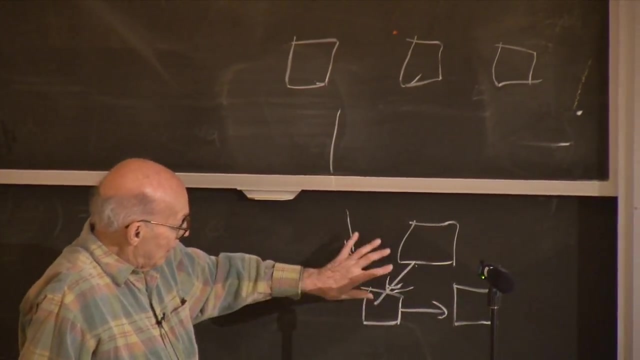 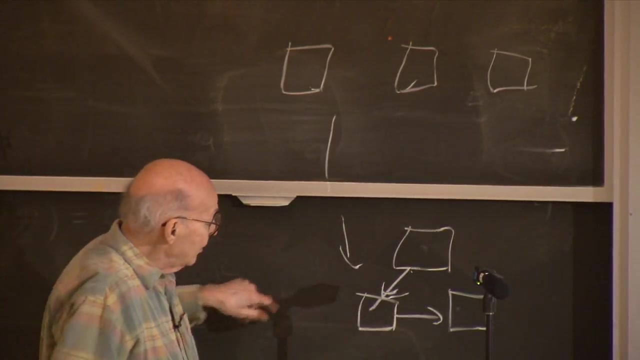 for making lists or trees, So you could arrange these in a way that. so here are the three things, And this is just a simple list, but I've drawn it as though these two were subsidiary to that. Of course, that depends on what program. 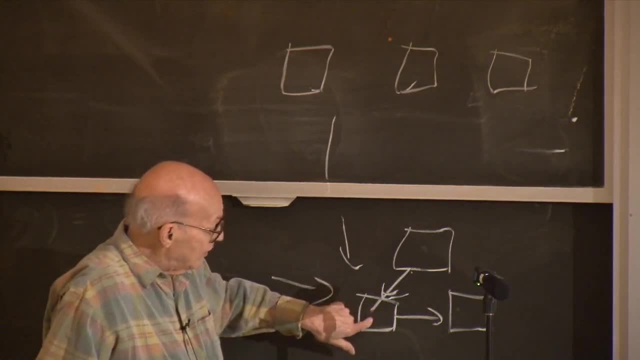 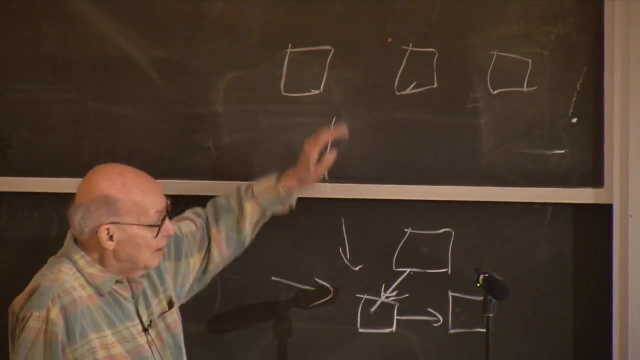 is going to look at this, And you could have a program which can say: here are two arguments for a function, And it doesn't matter what order they're in, It just depends on how you wrote the function. So Newell and Simon had written a programming language which 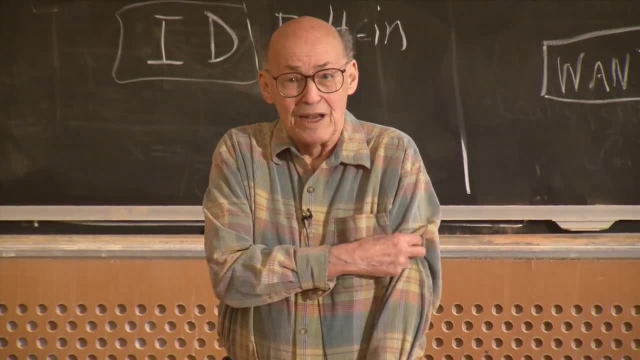 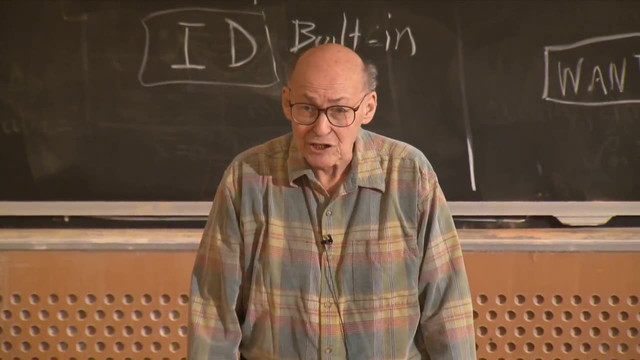 said: put something in a register, link it to another register and then perform the usual arithmetic operations. In fact, what they were doing is mostly performing logical operations, Because if you're going to do something, you're going to have to do something. 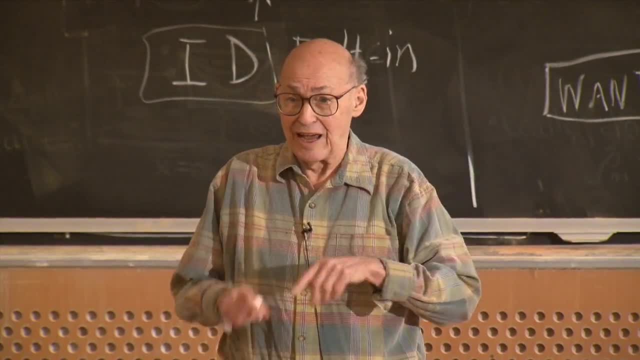 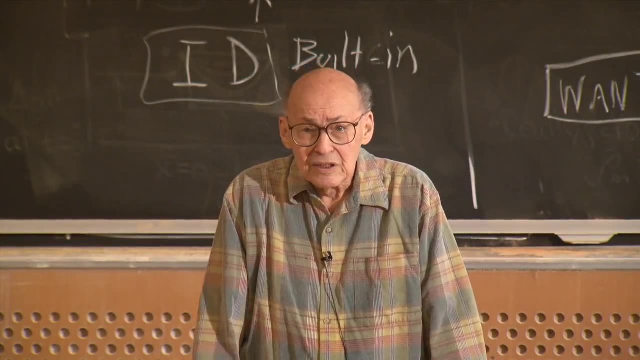 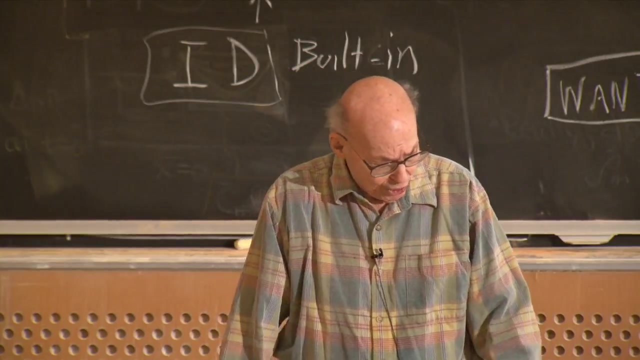 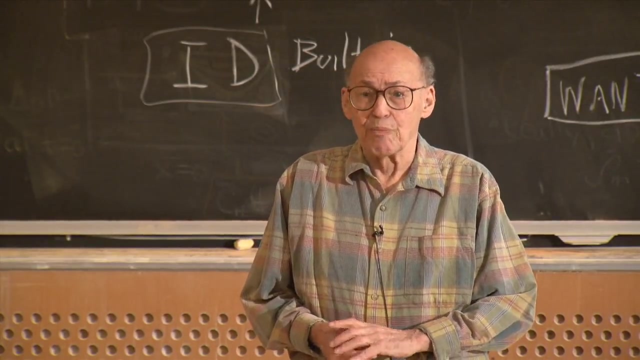 And of course even the early computers had ANDs and ORs and XORs and things like that. Try to remember what they were using for. So Newell and Simon had written a program that could deal with Boolean functions and prove little theorems about you know. 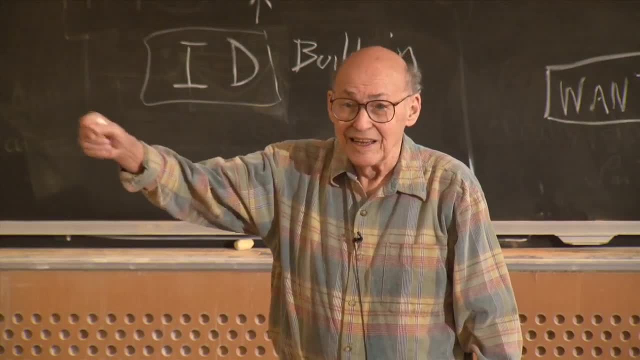 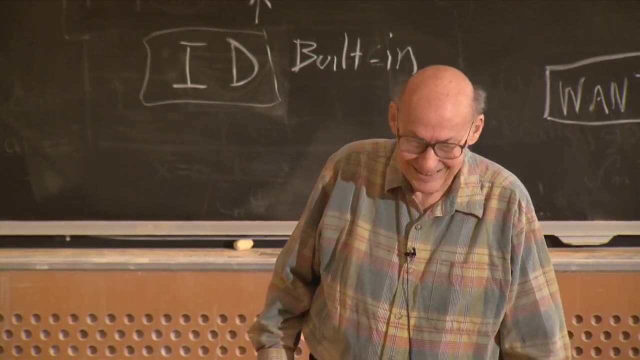 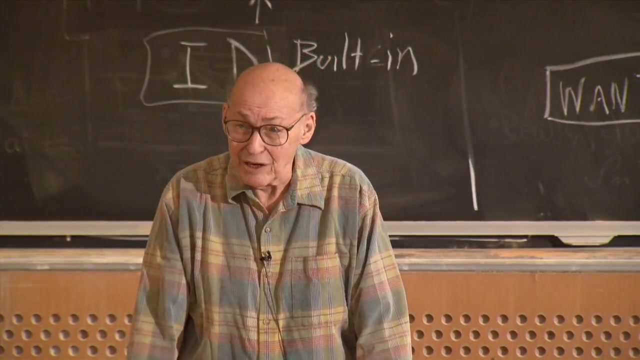 what functions are in them. So this is kind of where the point is: Not a OR not B. Is that wrong? I forget Should have more knots. Anyway, they wrote this beautiful but clumsy thing made of very simple logical primitives. 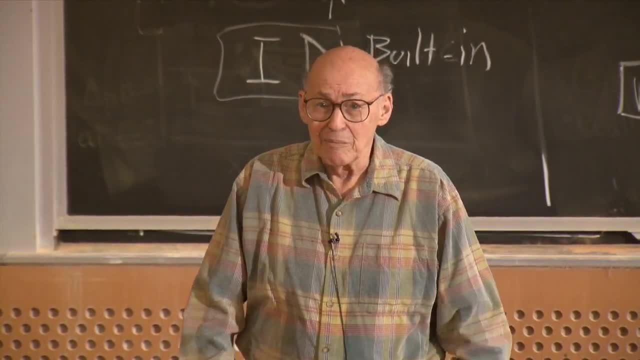 McCarthy. at the same time, IBM had spent 400 man years writing a program called. There was a program called UCI, There was a program called And there was a program called. I had to write a program called I-B-A. And I had to write a program called I-B-A And there was a program called I-B-A And they said you should write one, And you've got to write one, but you should write one. And there was one beautiful little thing that's going to happen. 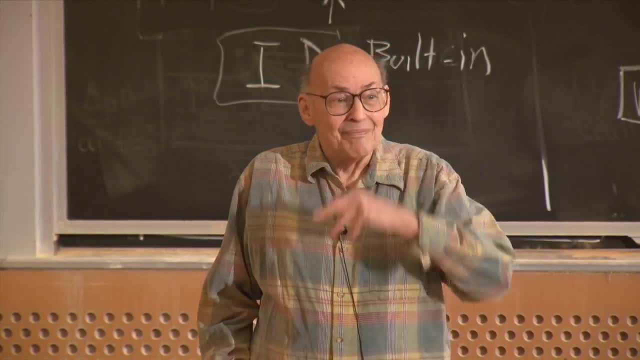 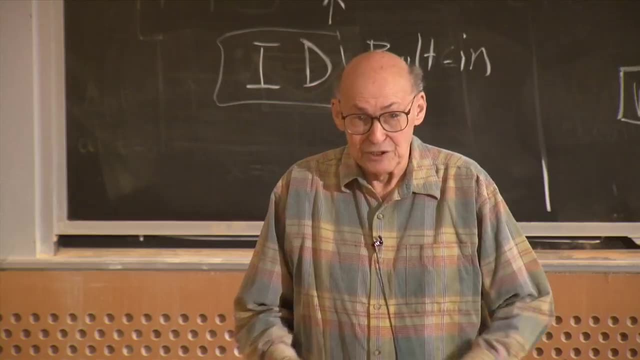 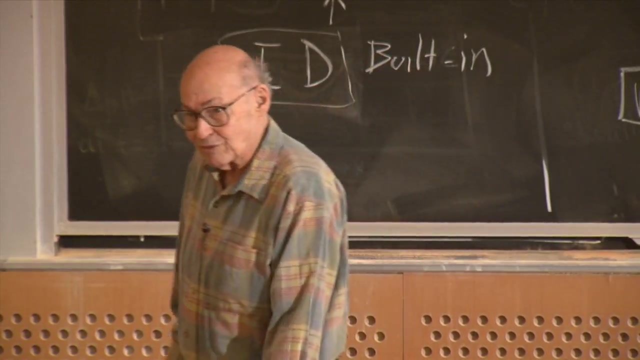 Fortran 1 or Fortran- I'm not sure that people had serial numbers on programming languages yet, because we're talking about the middle 1950s And McCarthy had been thinking about how would you make AI programs that could do symbolic reasoning. 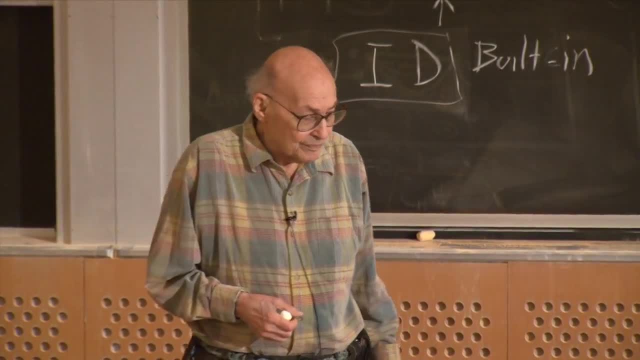 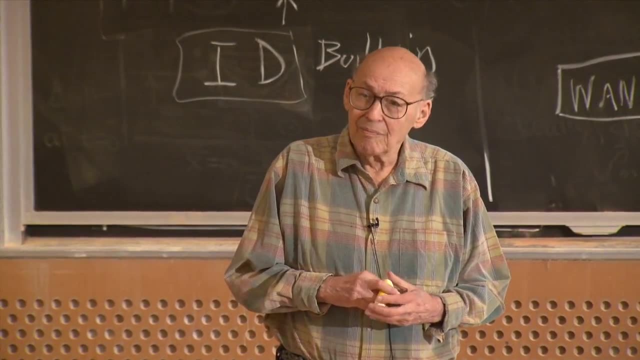 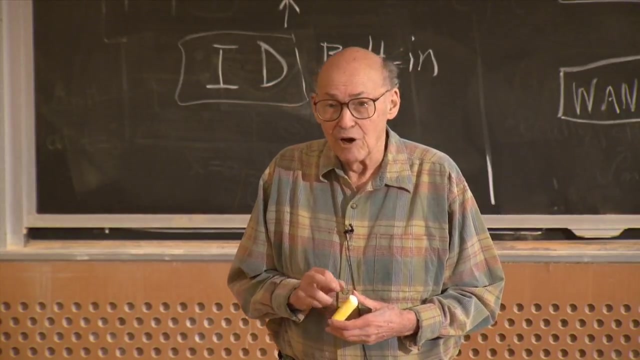 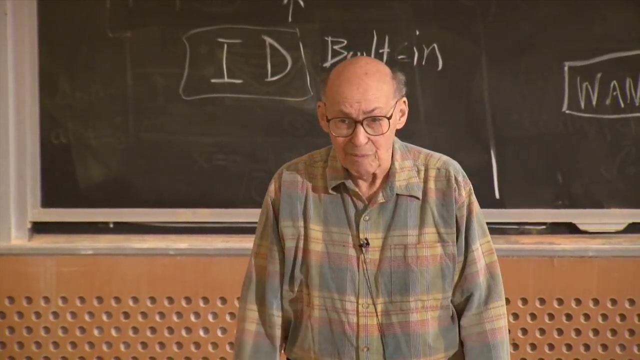 And he was indeed particularly interested in logic Backtrack. In fact, Newell and Simon had got their program to find proofs of most of the theorems in the first volume of Russell and Whitehead's Principia Mathematica, which is a huge two-volume book from about 1905,. 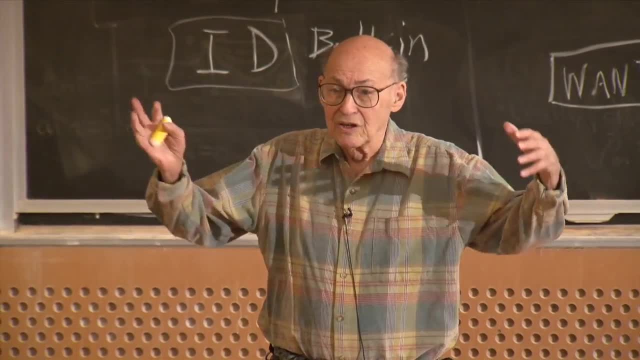 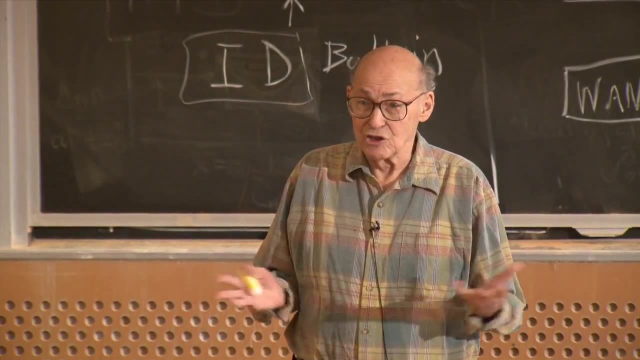 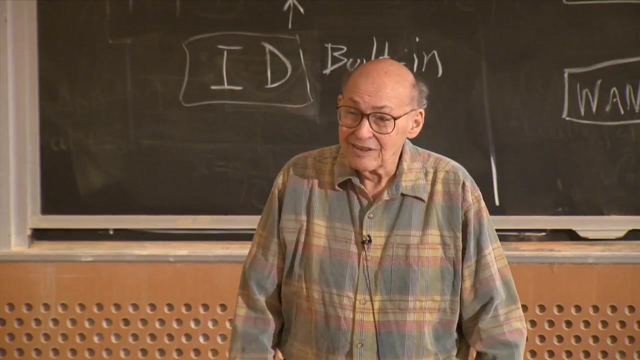 I think, which was the first successful attempt to reduce mathematics to logic And they managed to get up. They got up to calculus and show that differentiation and integration can be expressed as logical functions of variables. It's a great tour de force because you had to. 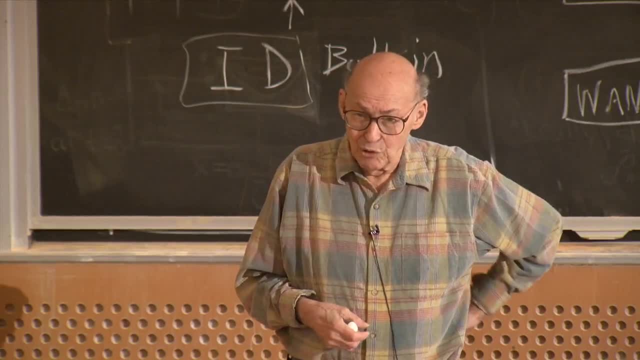 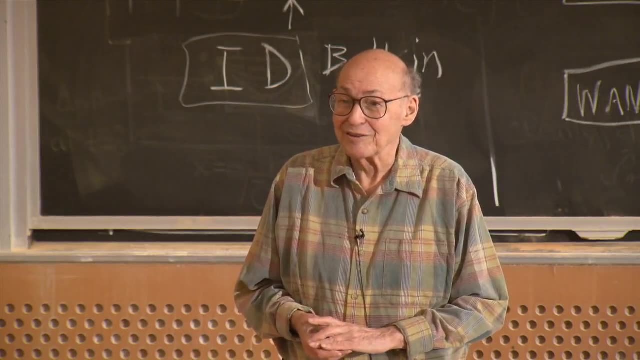 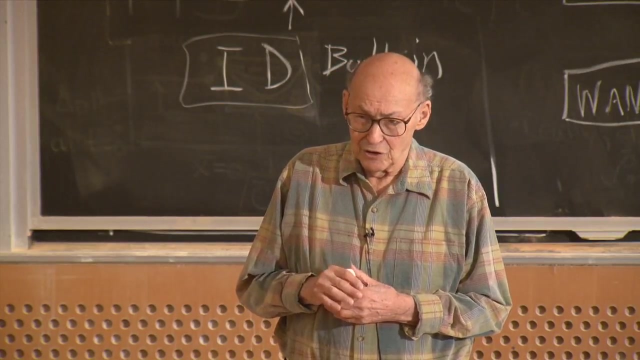 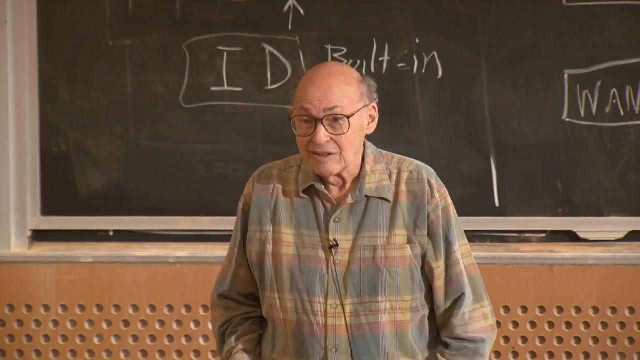 Because logic itself barely existed. Boole and a few others had- including Leibniz had- invented Boolean algebra-like things. Frege and others had got predicate calculus with there exists and for all. And that stuff was just appearing And Russell and Whitehead wrote this huge book. 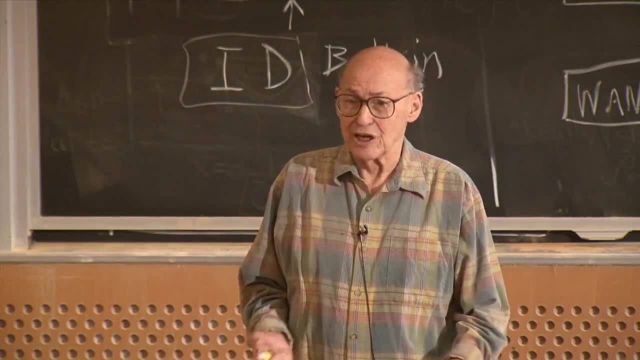 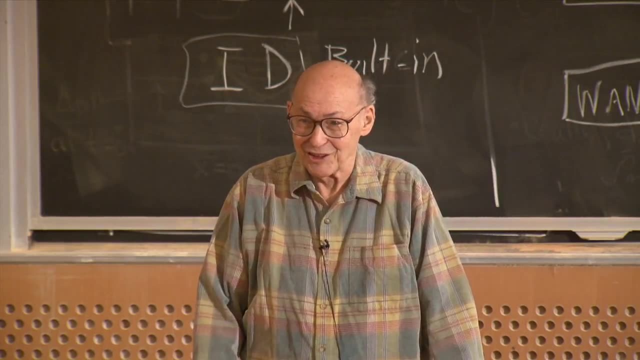 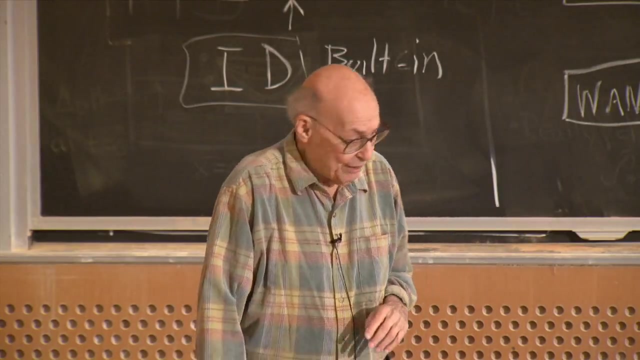 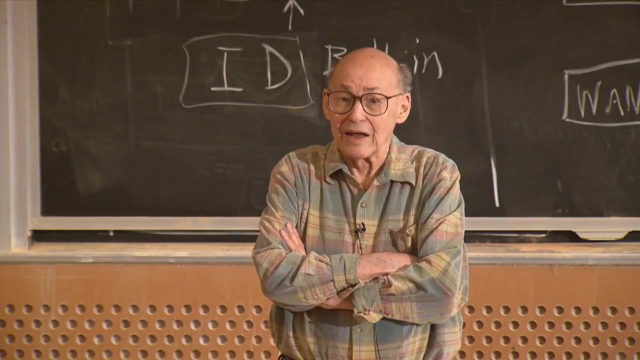 which got all the way up to describing continuous and differentiable functions and so forth. The first volume was huge and just did propositional calculus, which Aristotle had done some of also. Anyway, McCarthy looked at that and said: why can't there be a functional language like Fortran, that 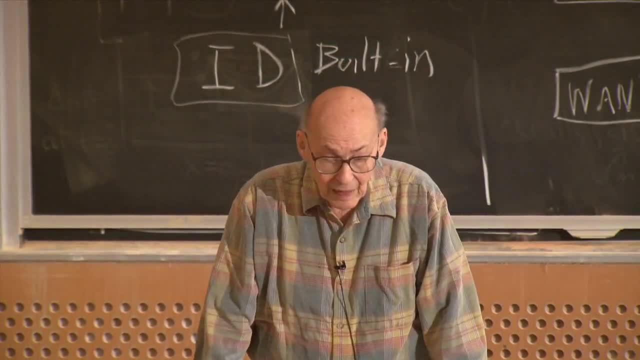 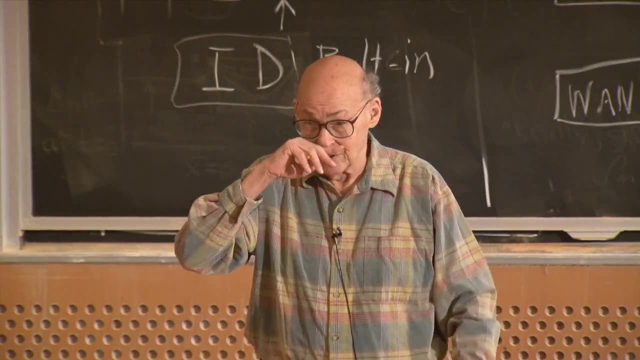 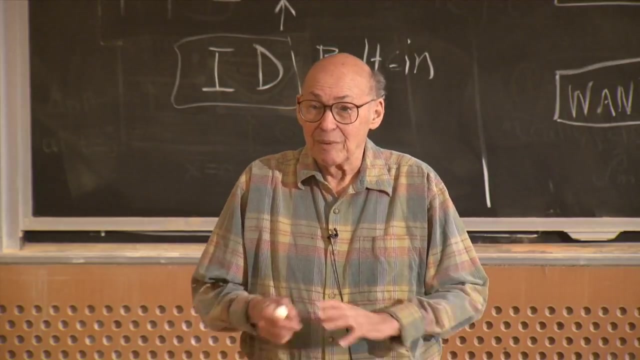 can do symbolic reasoning And pretty much all by himself. he got the basic ideas from Lisp. They're built on the Newell and Simon experiment, But he basically converted the MARVIN MINSKY, MARVIN MINSKY, MARVIN MINSKY. 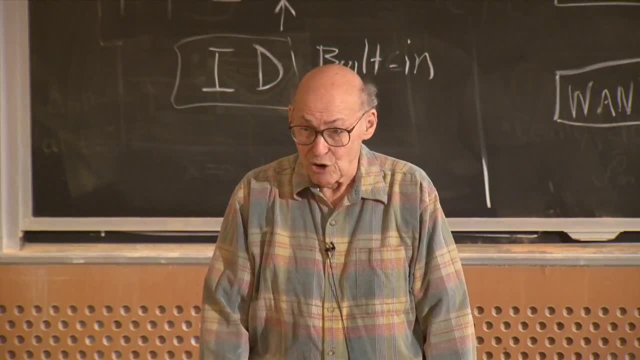 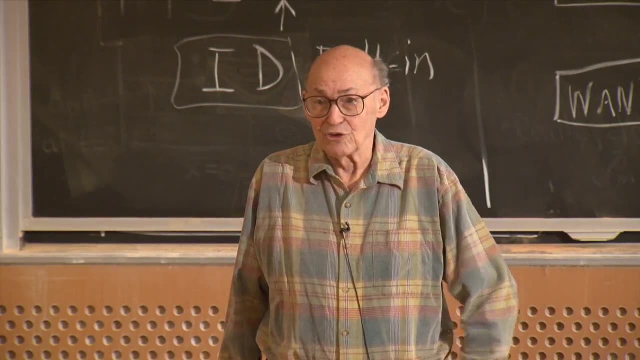 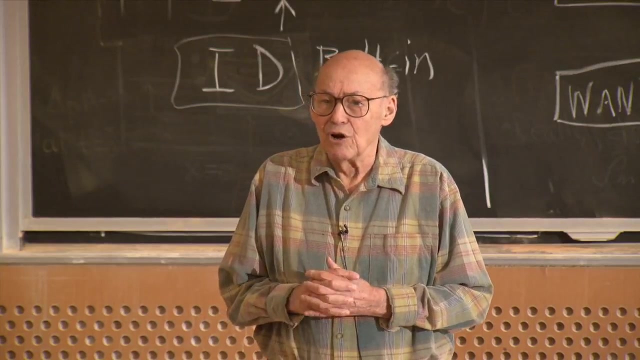 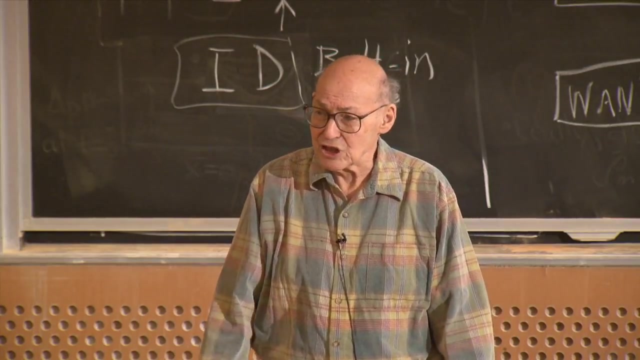 symbolic system into something like Fortran, which was only able to manipulate numbers, into Lisp, which was able to manipulate arbitrary symbols in various ways. If you want to know more about that, you can find McCarthy's home page at Stanford, just by. 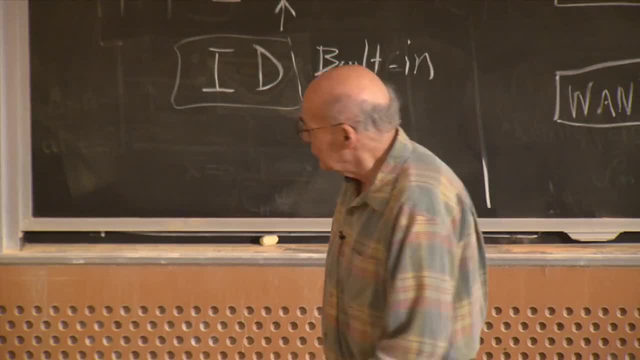 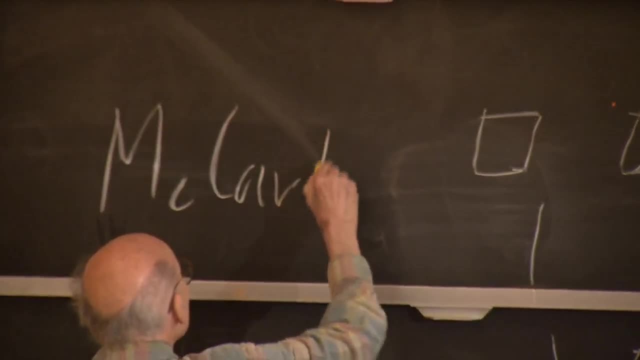 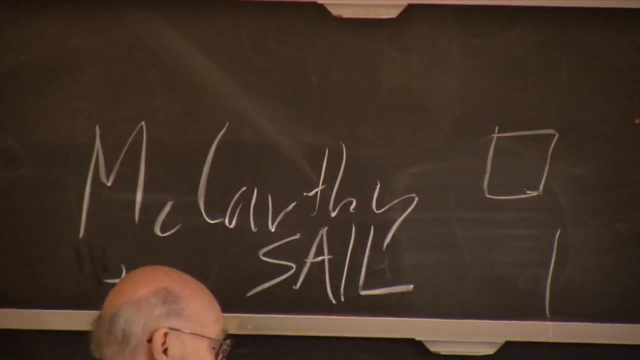 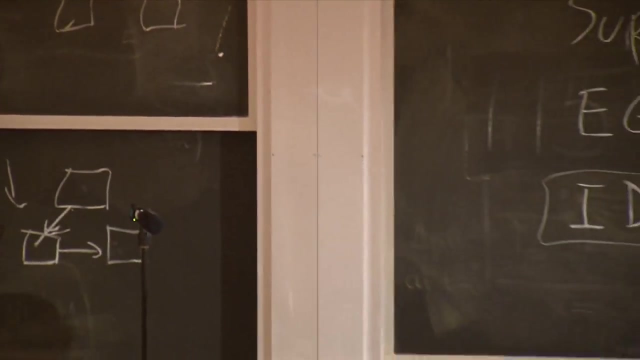 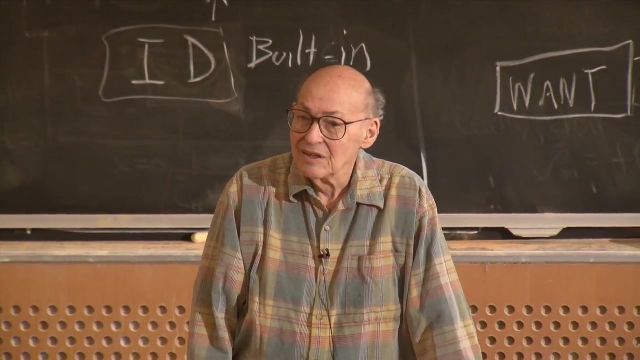 I think if you Google, search for McCarthy and SAIL- SAIL is Stanford Artificial Intelligence Laboratory- and you'll get his home page And there's a 1994 article about how he invented Lisp. Yes, Right after you started talking about Lisp, you jumped over and you said: 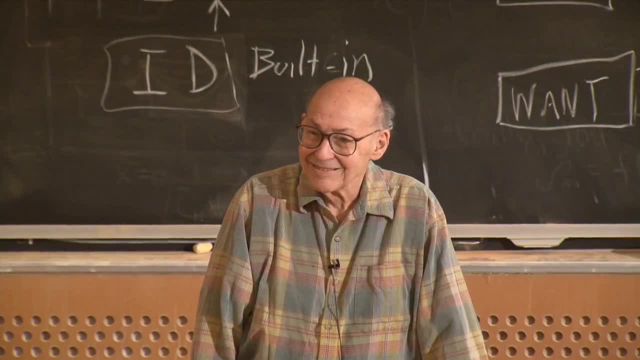 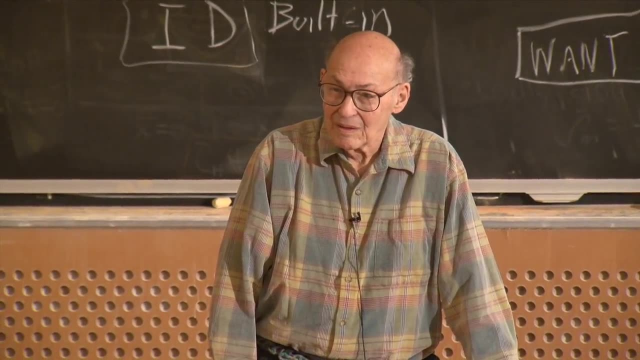 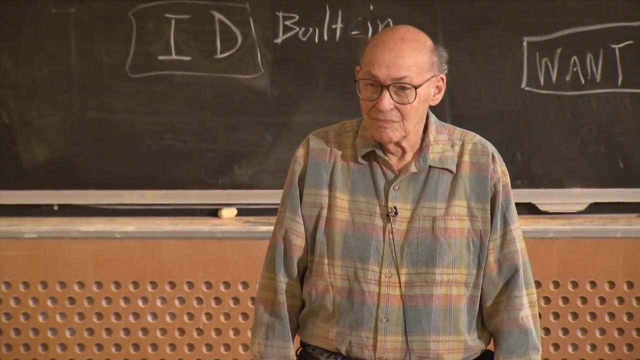 here's the now and the want, which is the current state and the desires, And I think you were going for some kind of analogy between the symbolic evaluation available in Lisp and what conscious entities do. However, one of the most beautiful things about Lisp- 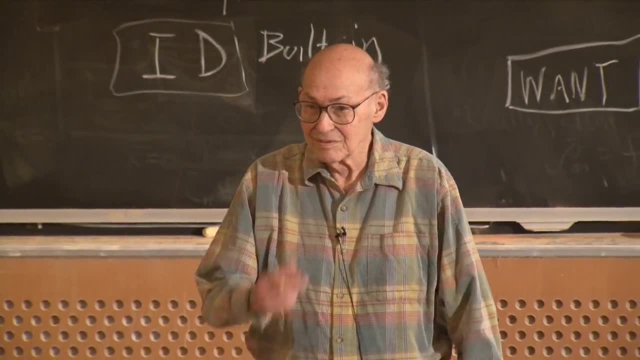 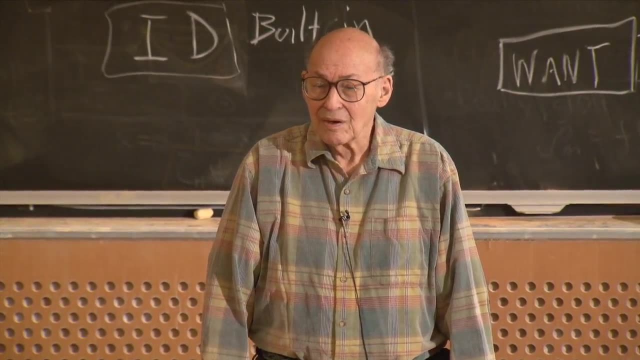 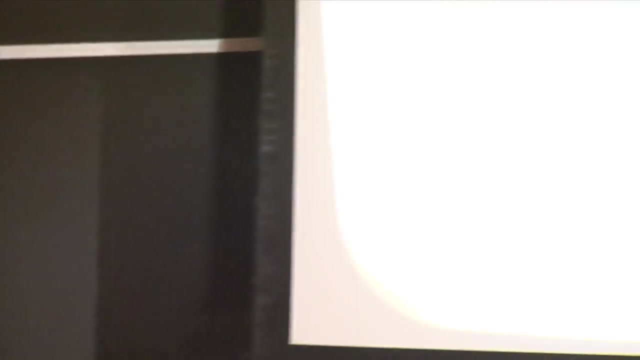 is the homo-iconicity, the fact that you have things such as macros. What is there in the conscious entity that is equivalent to the macro Macros? Yeah Well, each of these levels is. each of these levels are ways of combining things at the previous level. 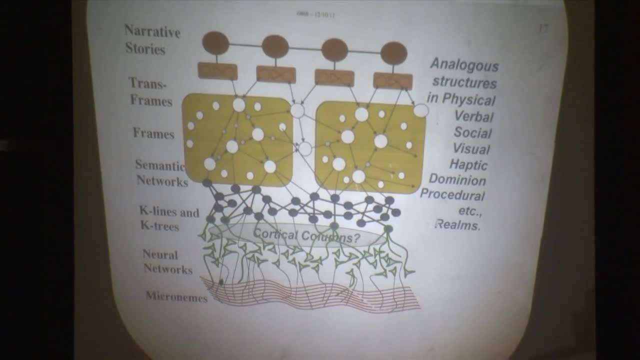 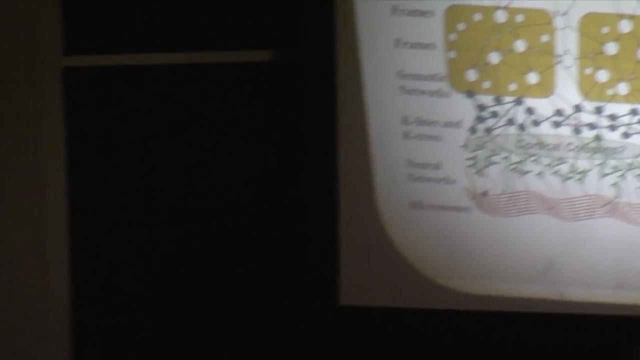 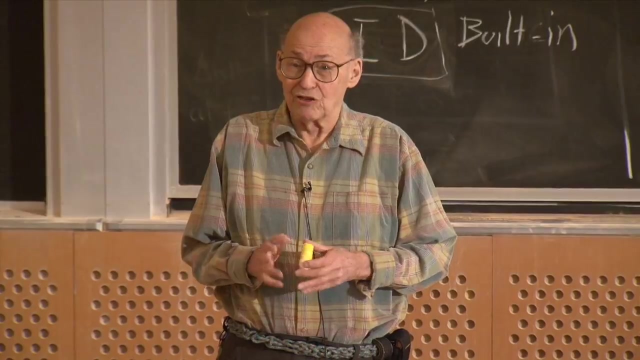 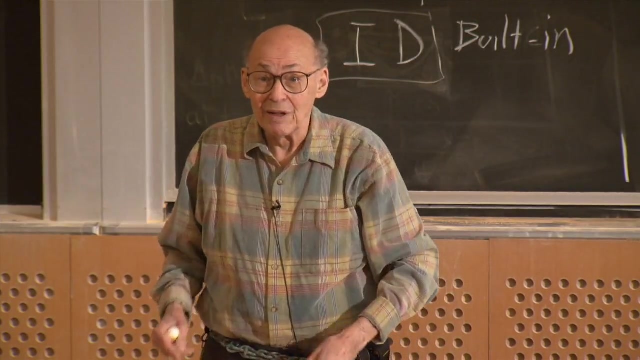 so that the way I drew it at the top. there are stories where you what's a story? You mention some of characters in a typical story. then you say: and here's a problem these characters encountered, and here's what Joe did to solve the problem. 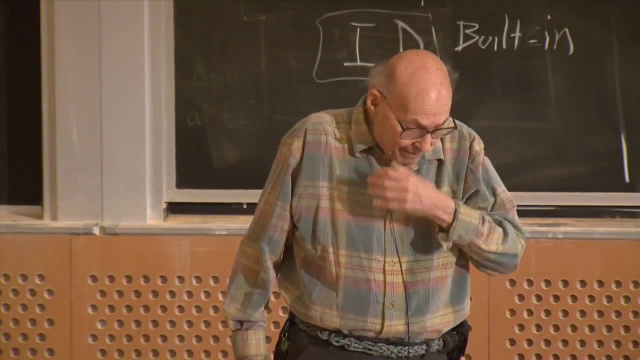 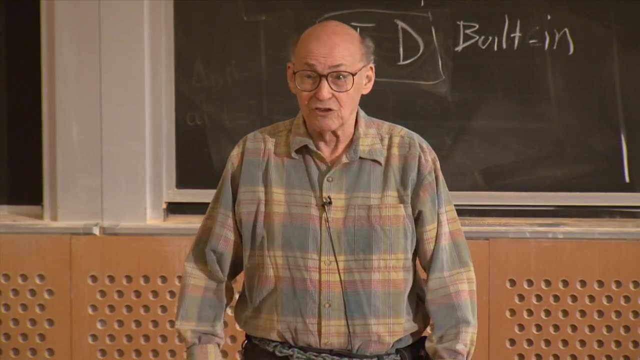 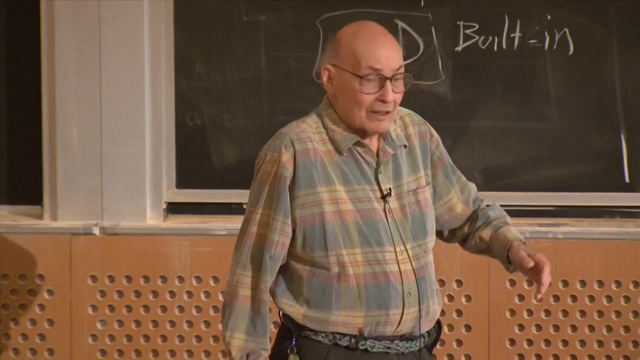 but it didn't work. and here are the bugs. And the reason it didn't work is that Mary was in the way, so he killed her and then blah, blah, blah. And so that's what stories are. If you just write a series of sentences, it's not a story. 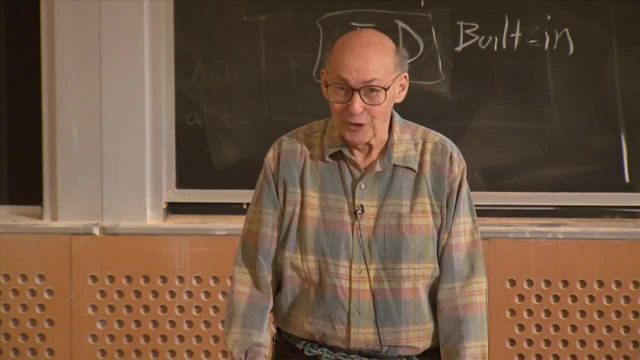 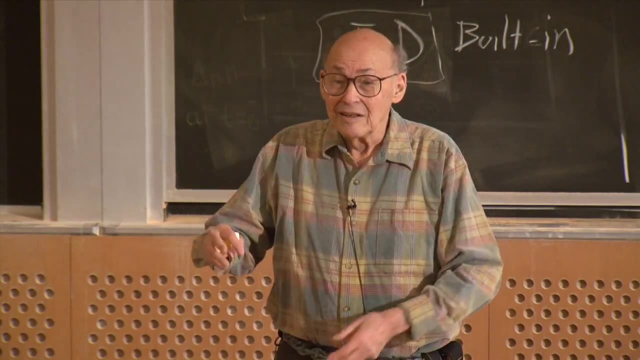 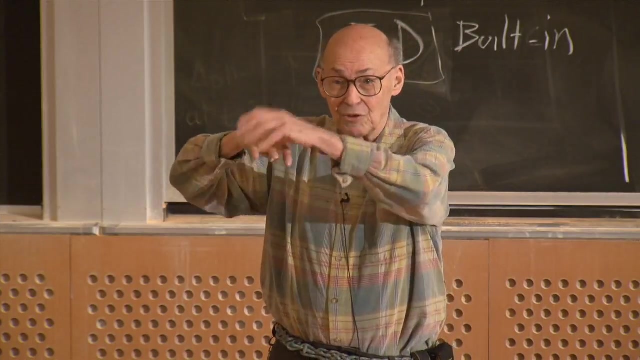 even though the New Yorker managed to make those into stories for about a period of 20 years. But a typical story introduces a scene and it introduces a problem, and then it produces a solution. but the solution has a bug And then the rest of it is how you get around that bug. 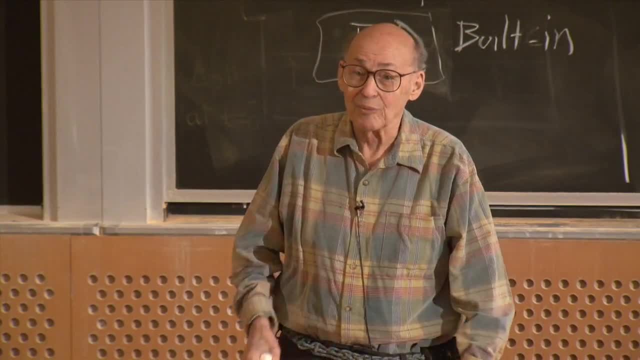 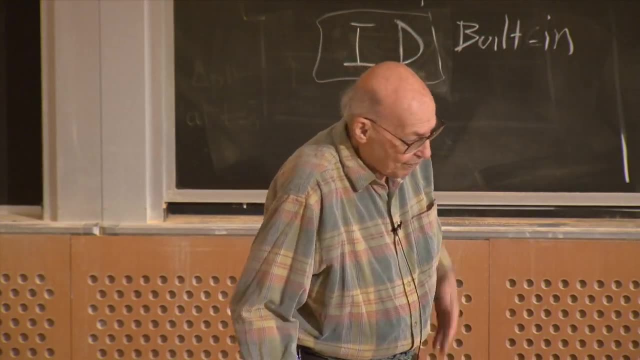 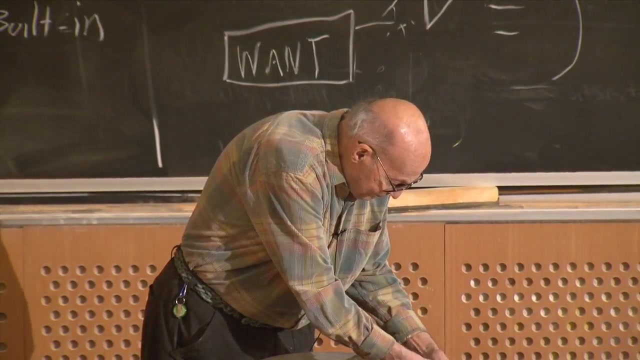 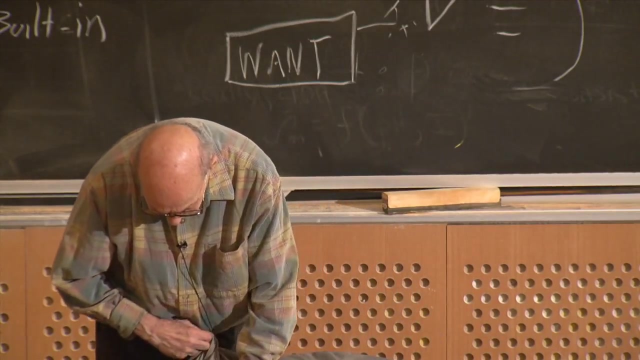 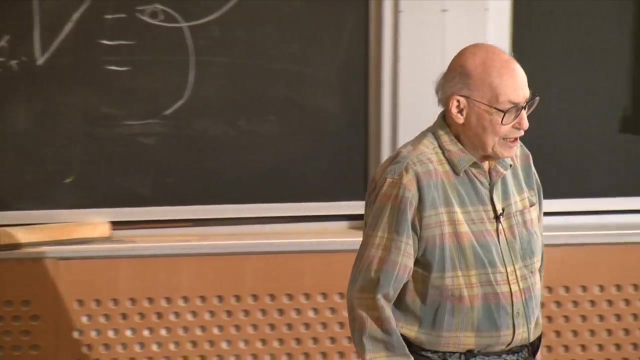 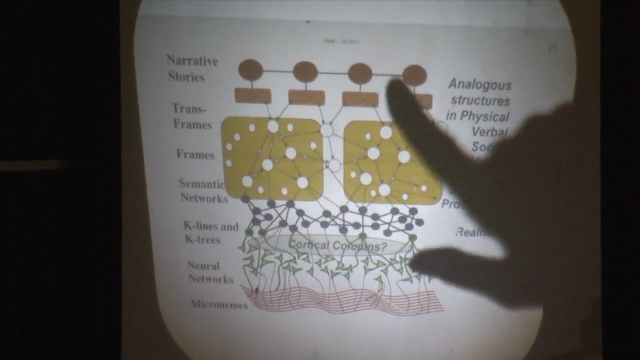 and how you maybe change the goals in the worst case. But so a story is a series of incidents. I wonder if I brought my death ray. Looks like I didn't. Oh, But you don't need it with this. You have to be here. 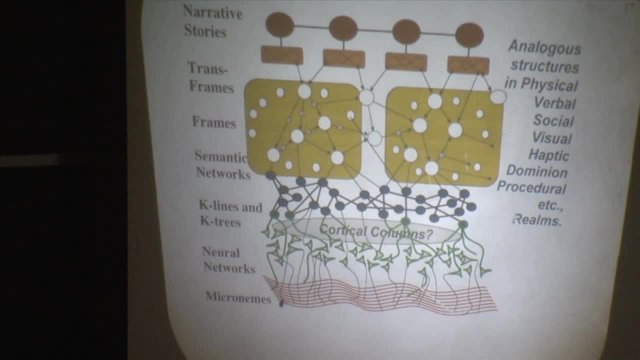 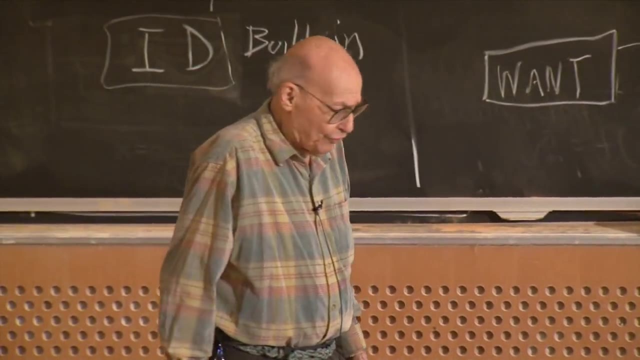 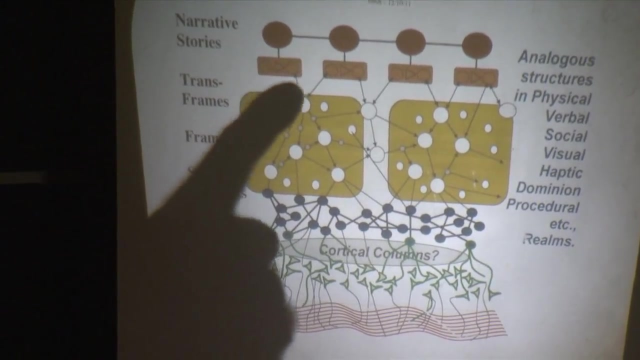 Anyway, but what's a story made of? Well, there are situations and you do something and you get a new situation. So what's that? Well, this thing I called a trance frame, which is a pair of situations, And OK, so what's an individual situation? 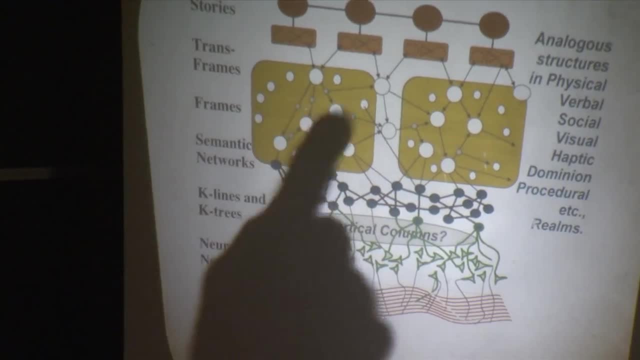 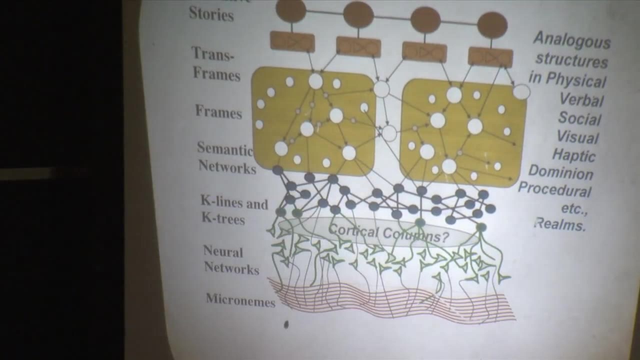 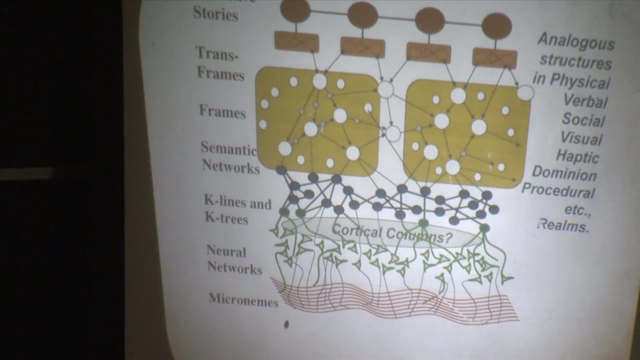 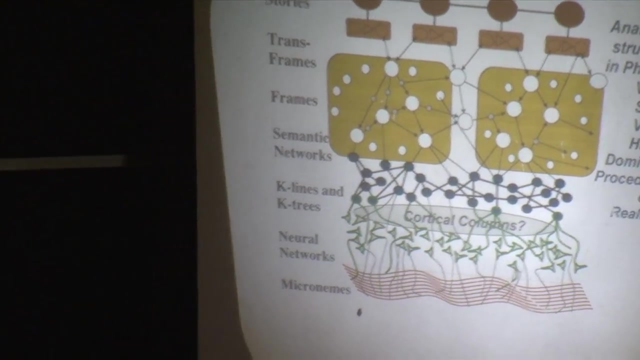 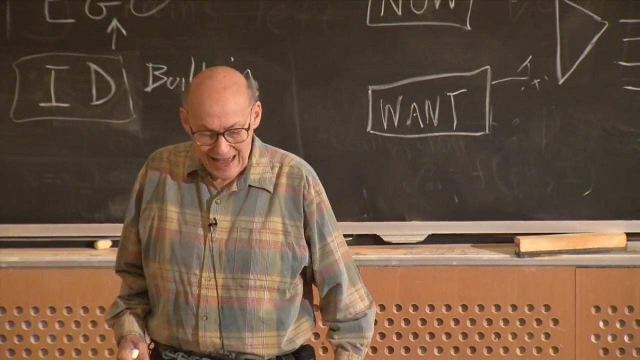 Well, it's a big network of nodes and relationships And I'm not sure why I have semantic networks down here rather than here, but Oh well, a frame is a collection of representations that's sort of stereotyped or canned. that might have. 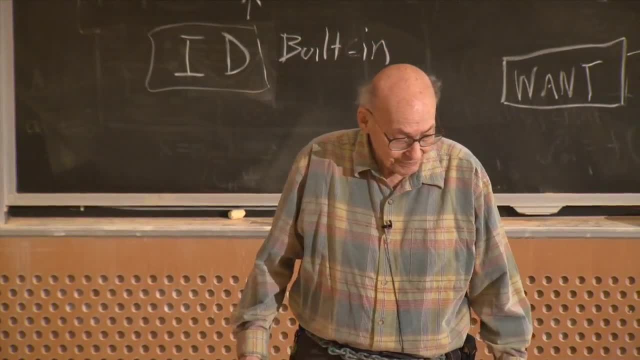 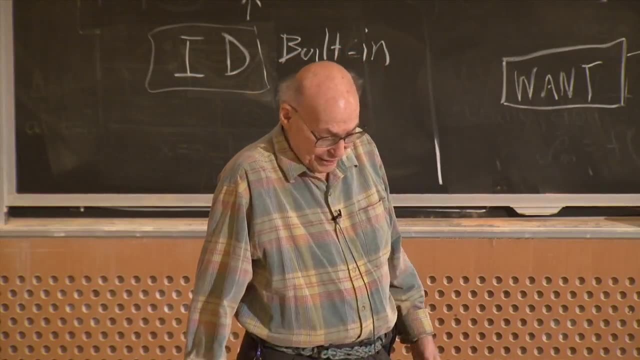 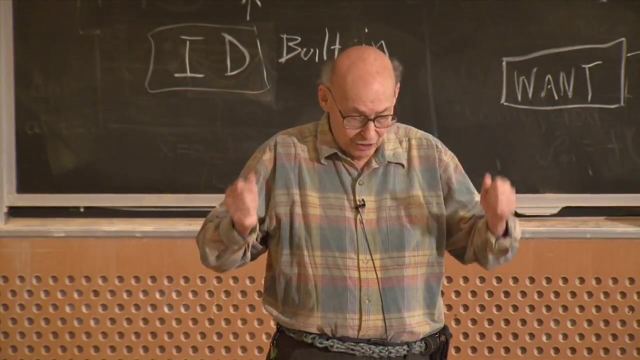 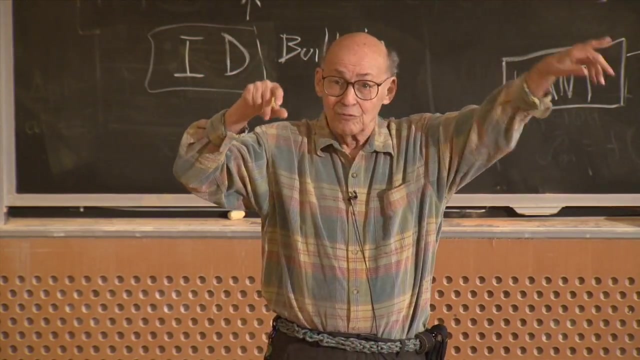 a single word like oh, just about any word breaking something. If I say John broke the X, you immediately say oh, that's a trance frame. Here's an object that had certain properties, parts and relationships and it's been replaced. 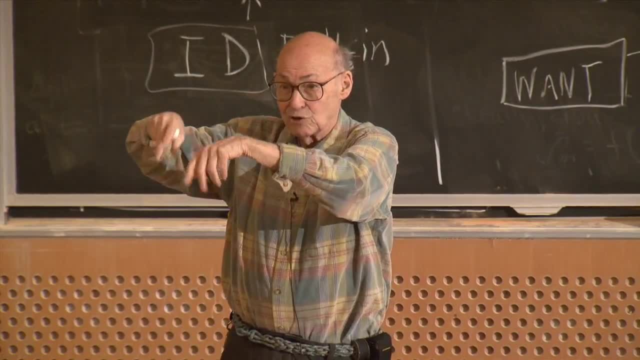 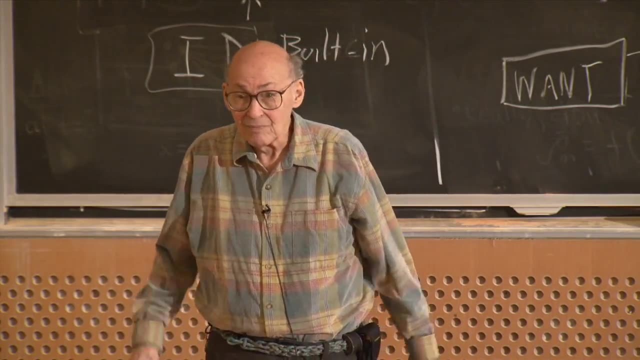 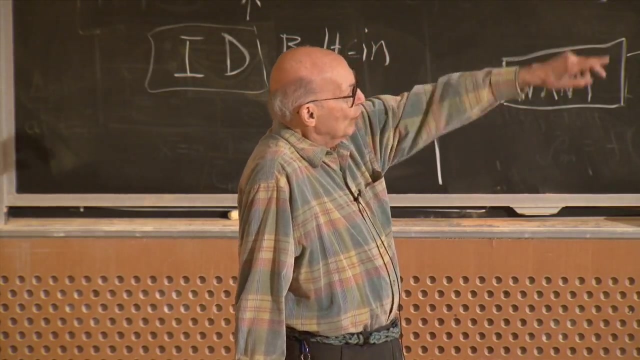 by this thing which has most of the same objects except, but different relationships, or one of the objects is missing and has been replaced by another frame, and so forth. So one question is: what's the relation? So this is a picture of cognitive representations. 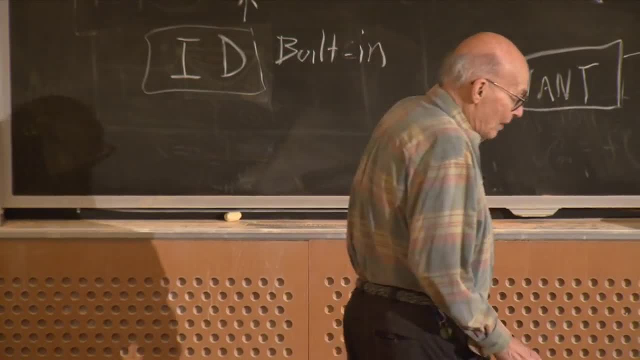 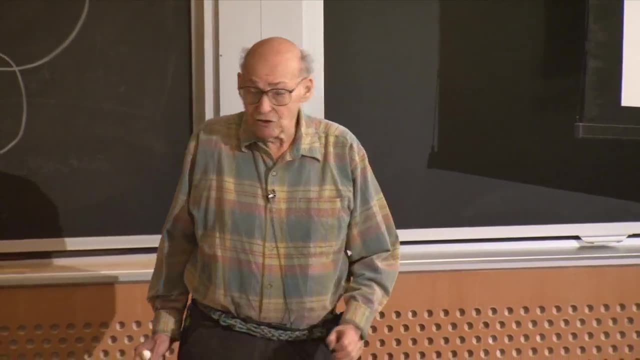 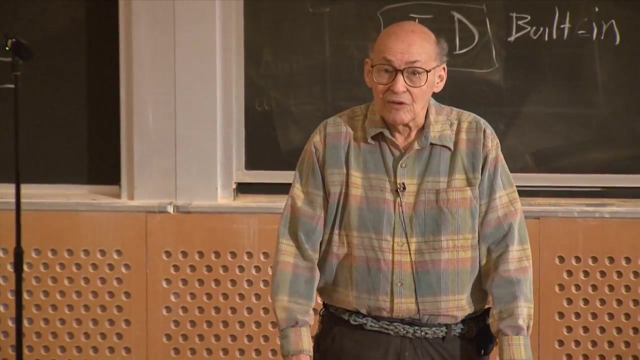 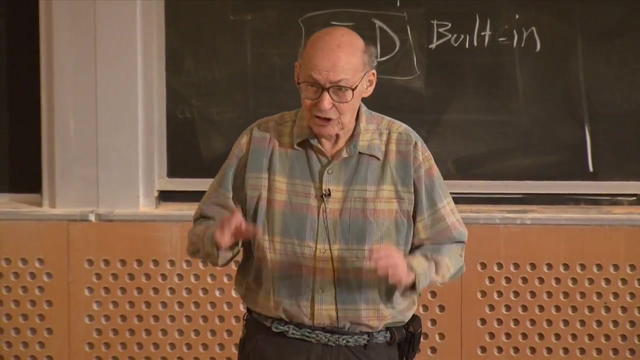 Everything is made of little parts And in the society of mind I described the idea of K-lines. which is what's a K-line? It's an imaginary structure in the nervous system which is there's really two kinds. There's a sort of perceptual K-line. 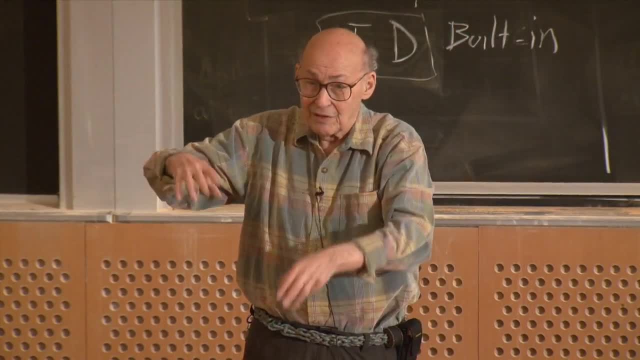 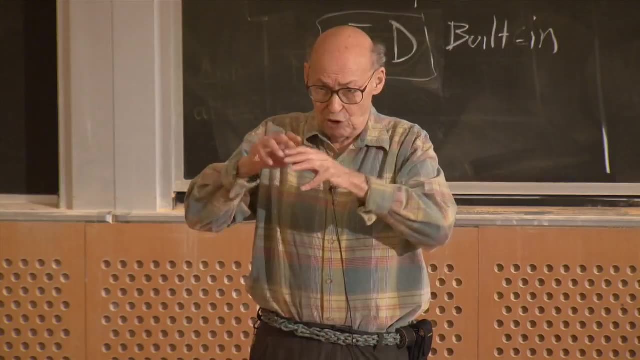 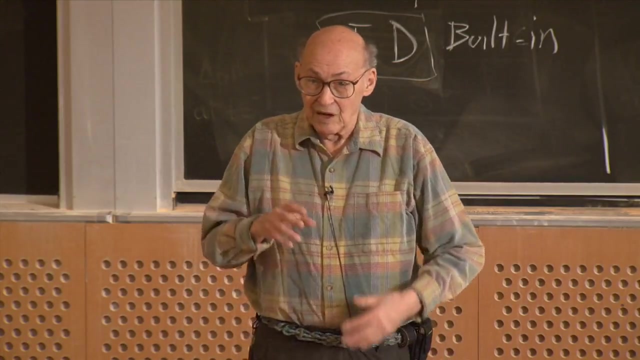 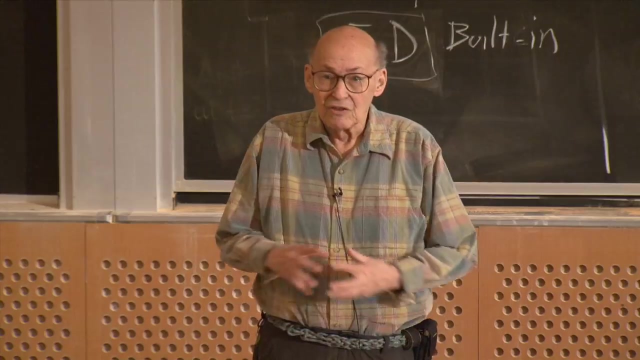 which is something that recognizes that, say, 10 features of a situation are present, And if these are all present, then a certain bunch of neurons or neural activity goes on. And on the other hand, when you think of something like a word, suppose I say microphone. 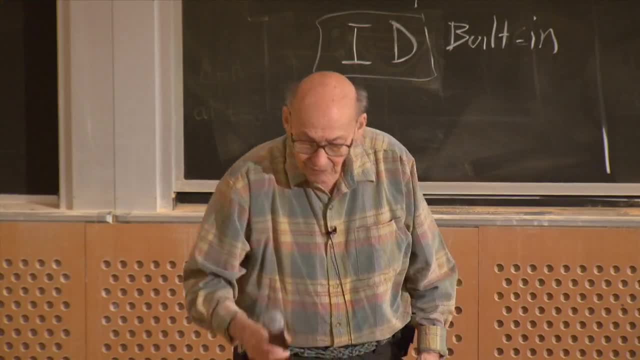 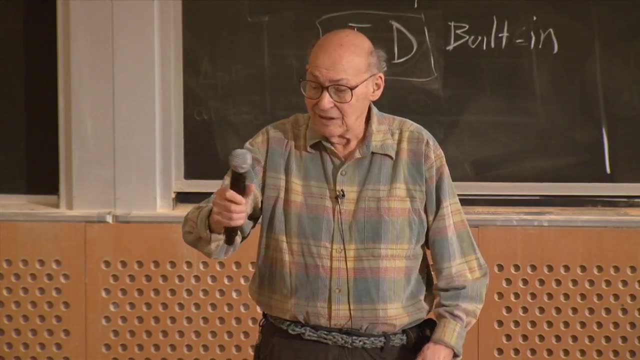 then you're likely to think of something that has a business end, which collects sounds, And it has a stand, or maybe it has a handle, And if you're an engineer you know that probably it has a battery or a transmitter or a wire. 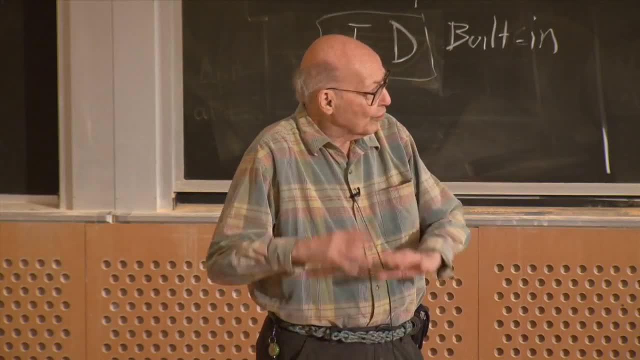 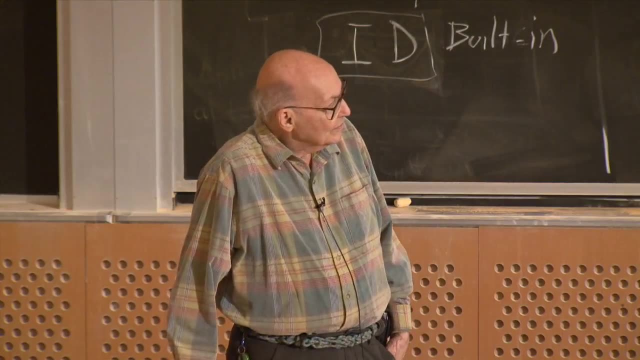 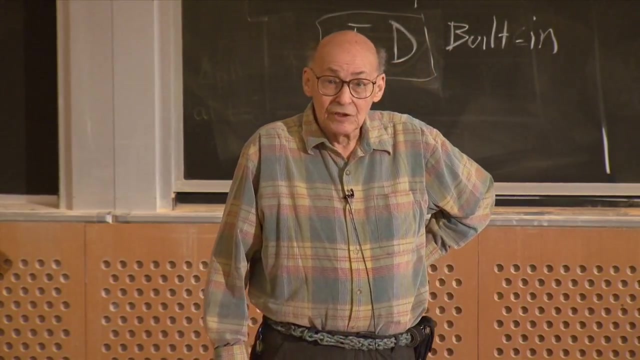 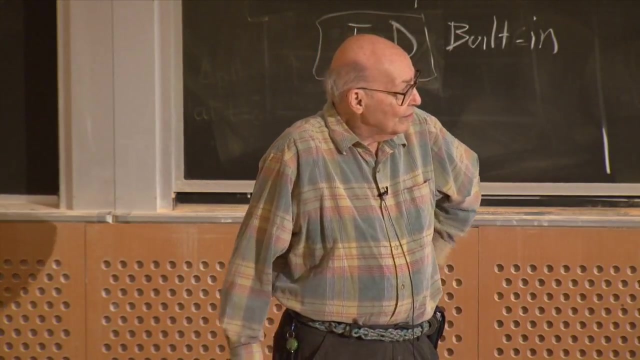 So those are the things that I call frames or K-lines, And anyway, chapter 8 of the Emotion Machine talks about that And there's a lot of detail in the old book, The Society of Mind, about what K-lines and things. 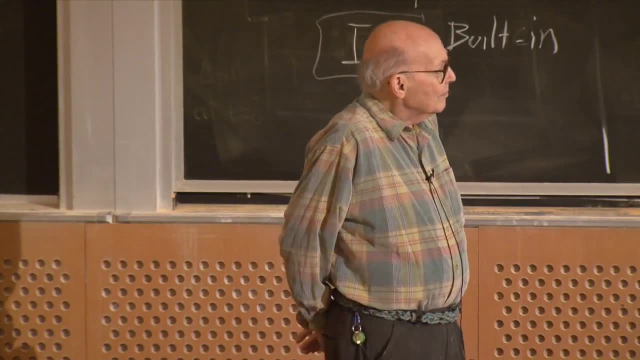 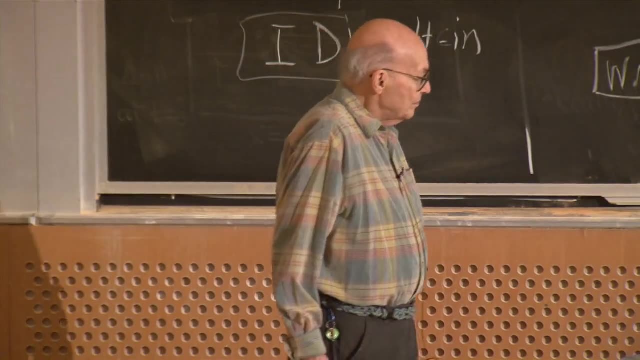 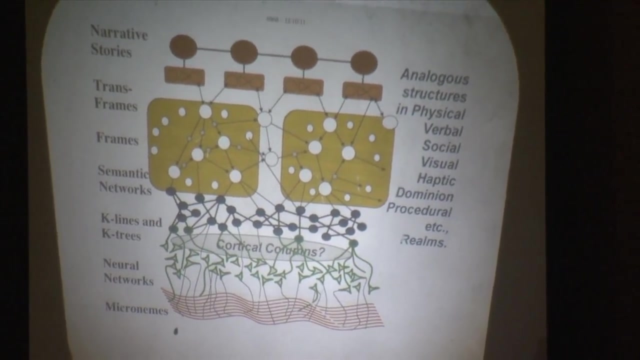 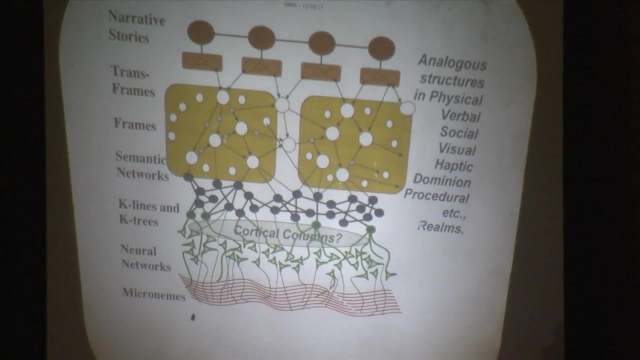 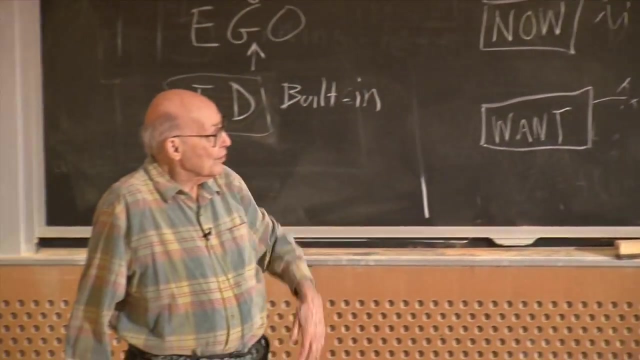 like that could be made of. Now, whatever those are, and as far as I know, no matter how hard you look, you won't find any published theories of what in the nervous system is used to represent the things above that sort of midline. 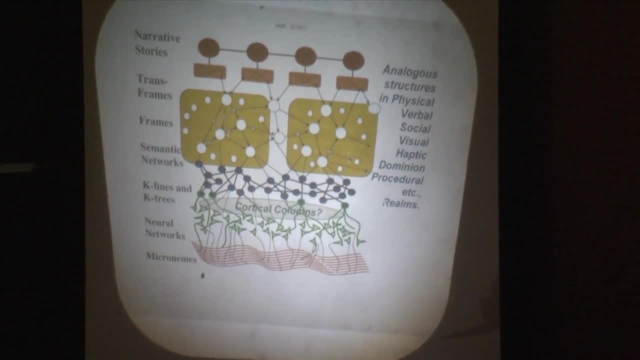 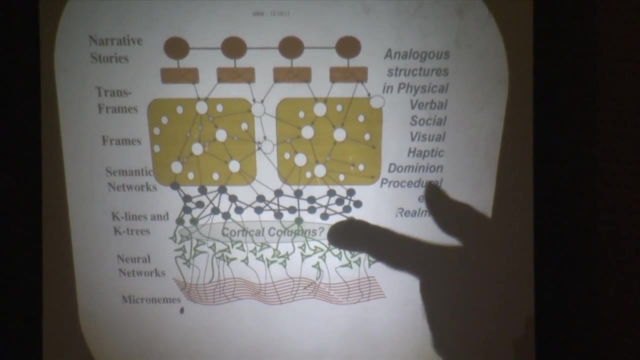 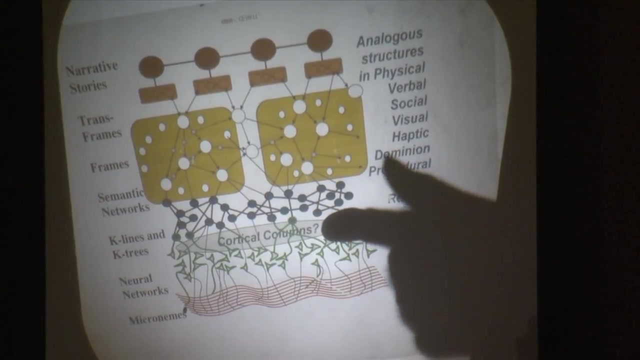 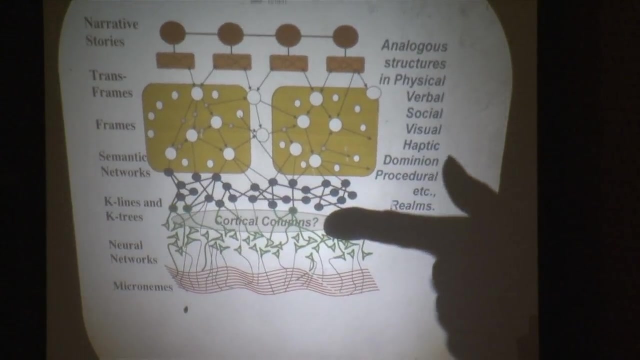 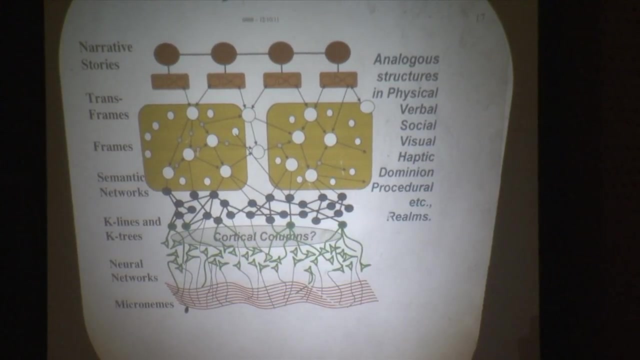 there, Cortical columns. I suspect that almost everything that the human brain does, that fish and those lower animals- or earlier animals- I should say I'm not sure that higher and lower makes any sense- are probably symbolic processes where it probably does more harm than good to have. 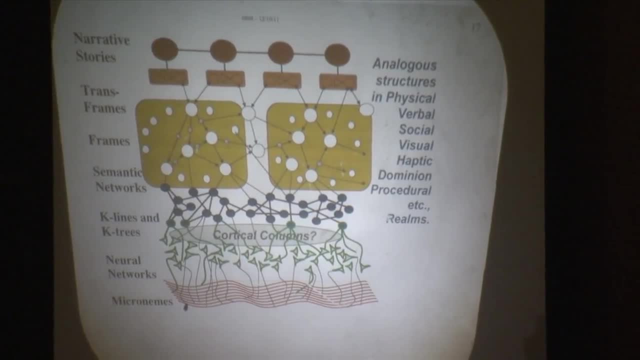 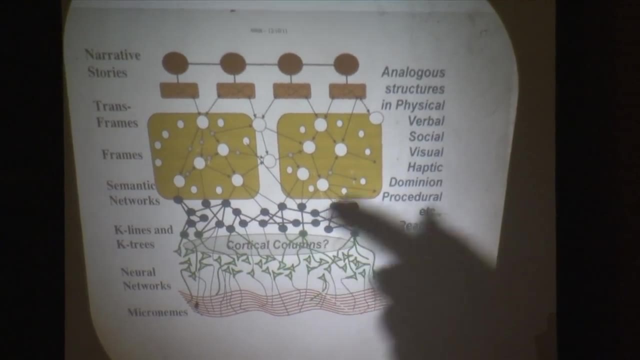 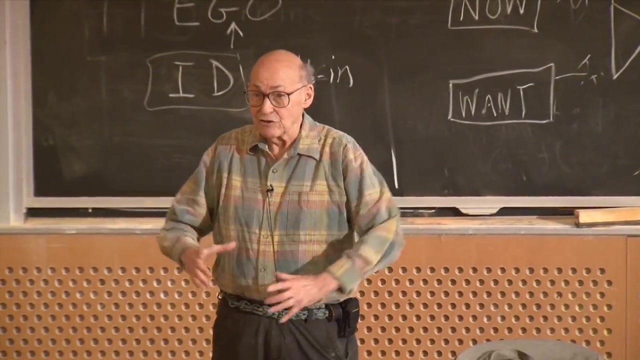 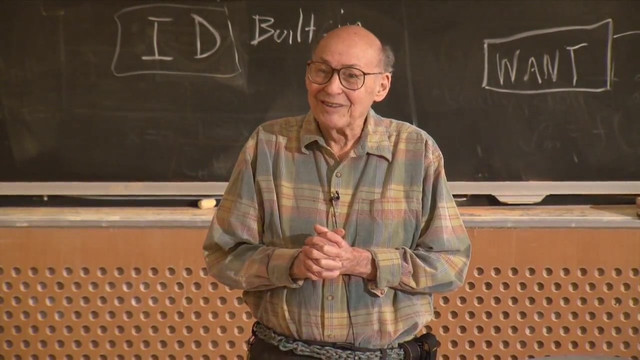 elaborate theories of what's the physiological chemistry of neurons, But at some point we want to know what in fact the brain is made of. The cortical column has a few hundred brain cells arranged And there are several projects around the world trying. 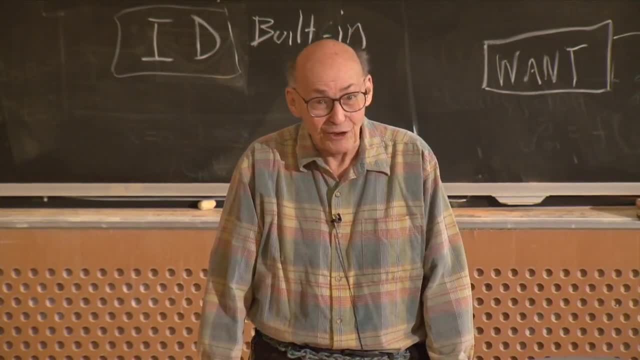 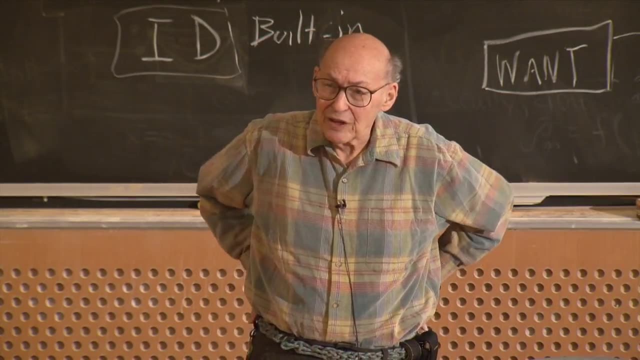 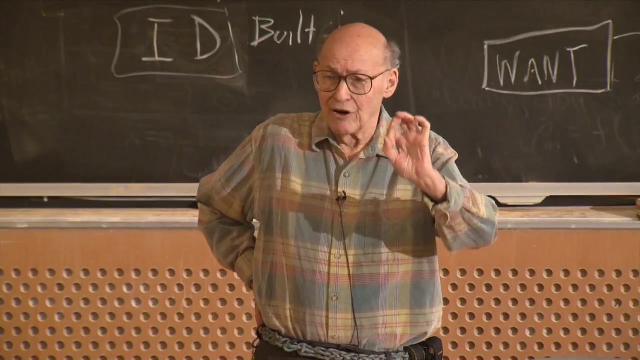 to take electrons, Microscopes and pieces of mouse brain or cat brain and make a huge connection matrix. The problem is that the electron microscope, even the electron microscope pictures, still aren't good enough to show you at each synapse what is probably going on. 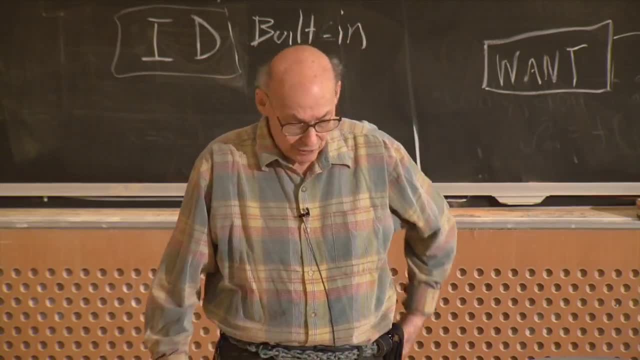 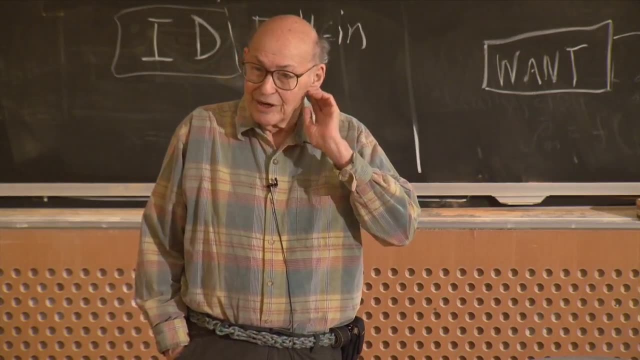 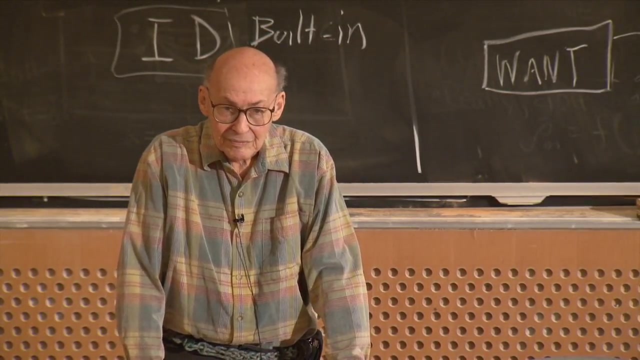 Eventually people will get theories of that and get slightly better instruments, And I'm not sure that the present diet grams that they're producing are going to be much use to anyone. Yes, It's a nice question. This question might be a little bit difficult. 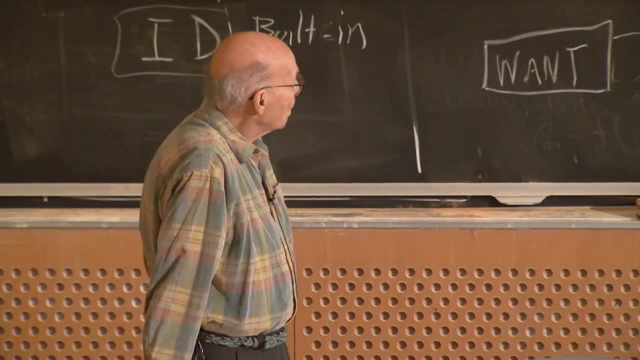 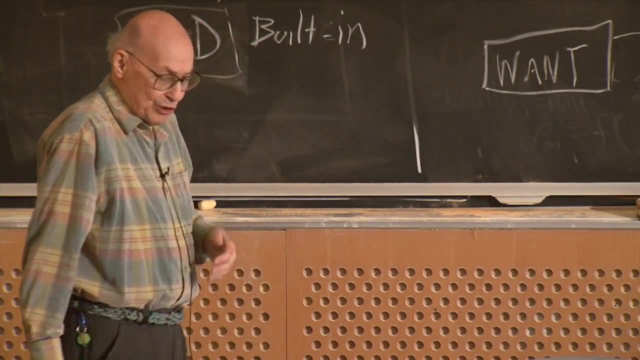 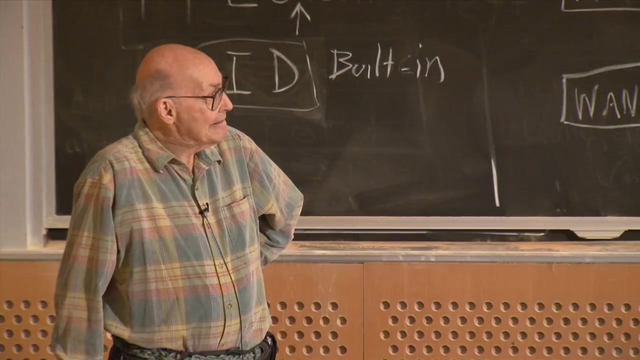 So I'm going to start from the goal being a difference between now, this, now state and the desired state. How do we reduce the difference? Yeah, Yeah, How do we get the difference? And so now I'm going to also, I'm 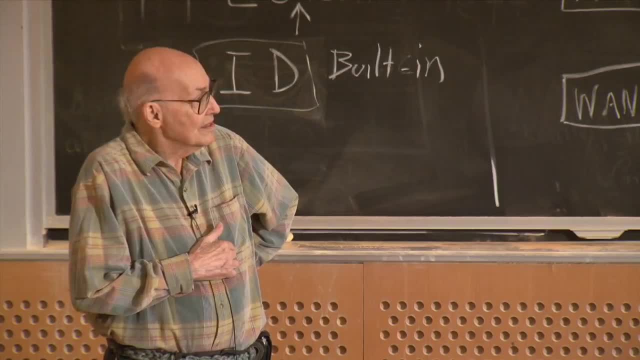 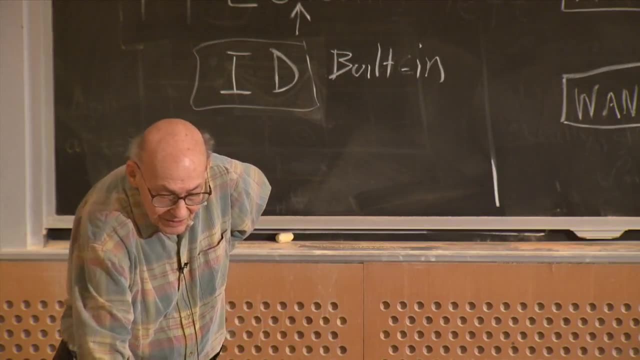 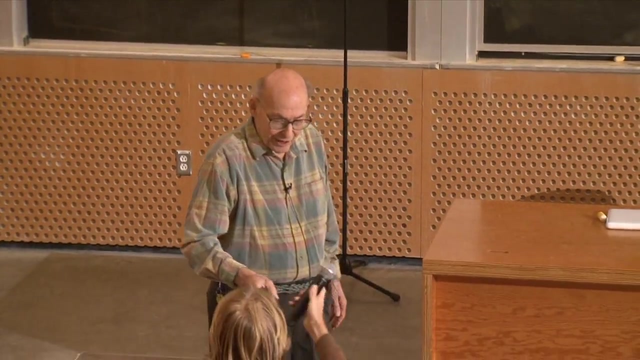 going to also take the fact of the animals being different, And I'd say that one of the biggest big differences is that we, as people, we cannot describe these differences. It actually is only good for the recording. OK, So we can describe these differences. 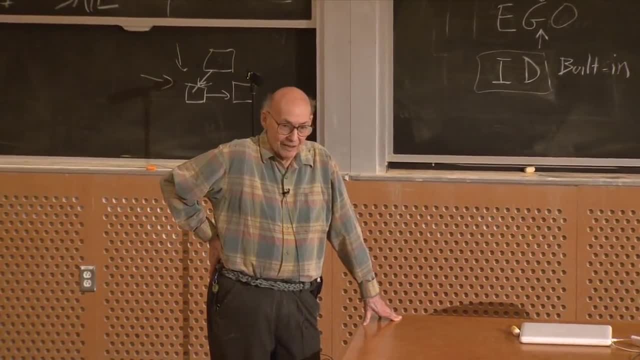 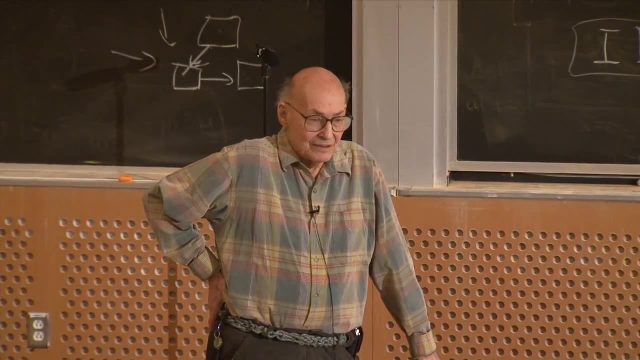 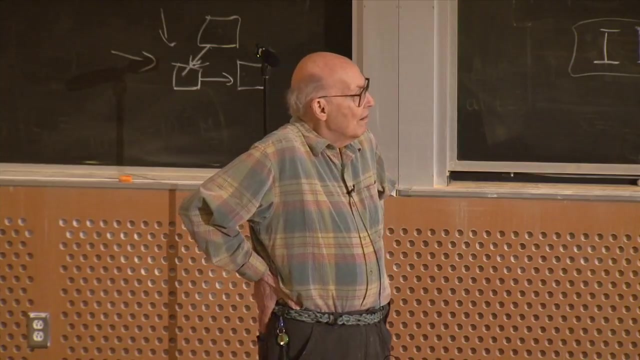 and talk with them, talk about them with other people, without having to act on them. Yeah, Yeah, Yeah, We can't do that. We can't expect to act on those goals or hypothetical goals. So if everything that has to do with goals 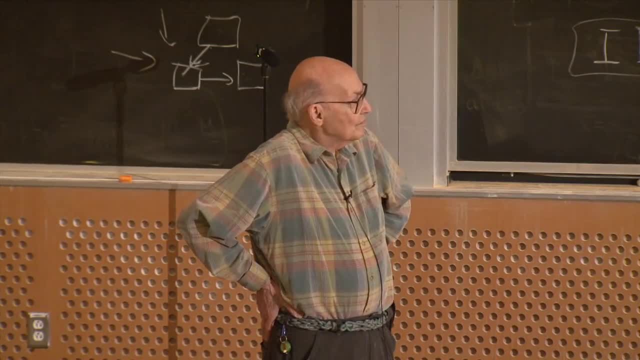 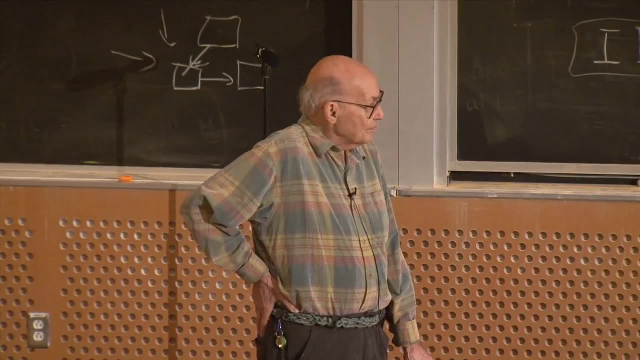 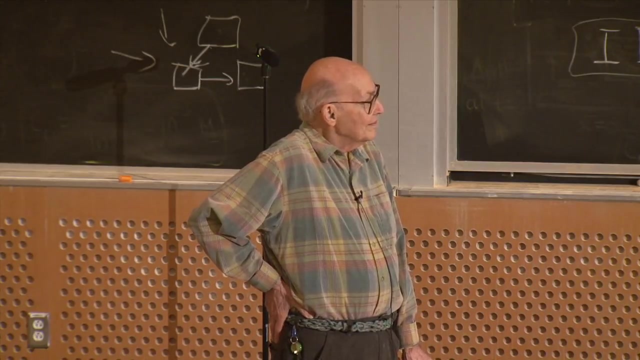 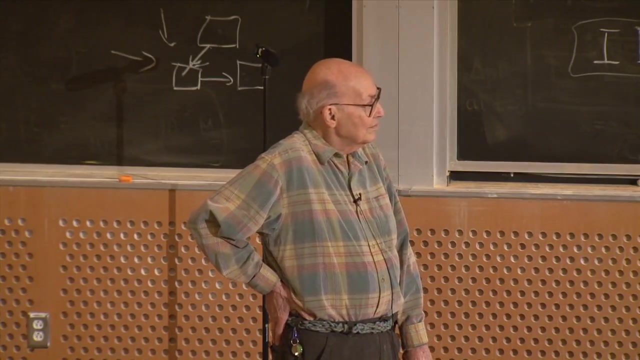 is represented with a complex structure like this one and I want to implement it in a computer. well, I can. just for every hypothetical case that has to do with solving a certain problem, I can just make more copies in the memory. then I don't know how convenient it is to postulate that there is like a huge memory data bank. 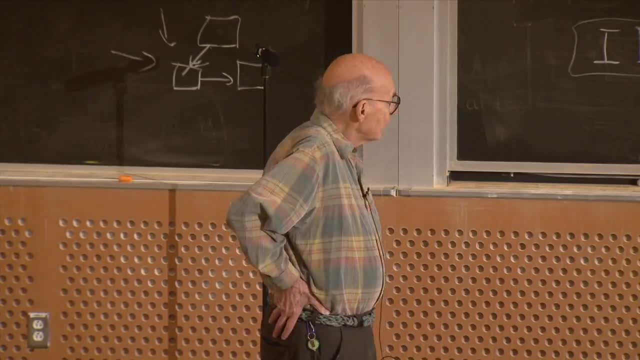 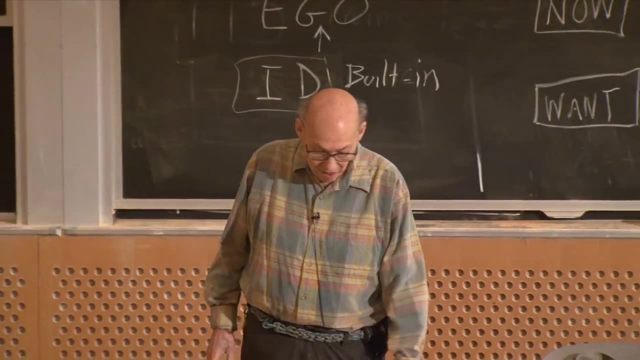 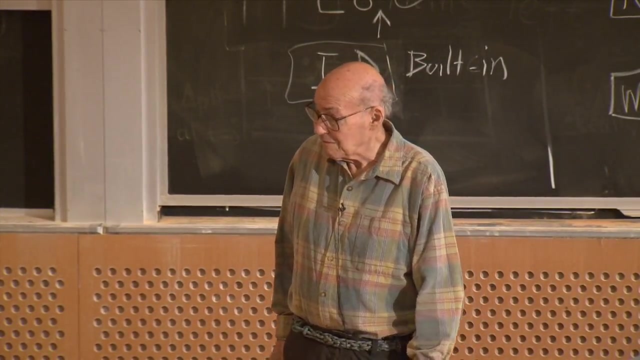 where you can make copies of everything that's going on, or if you have to assume some kind of a huge collection of pointers and acting on those pointers. So this is just a random point and I'd like to hear if you have any ideas on this. 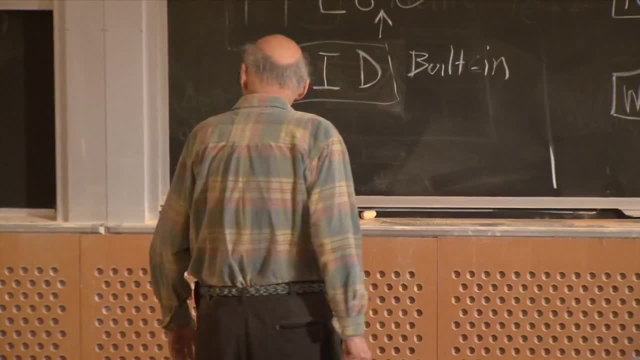 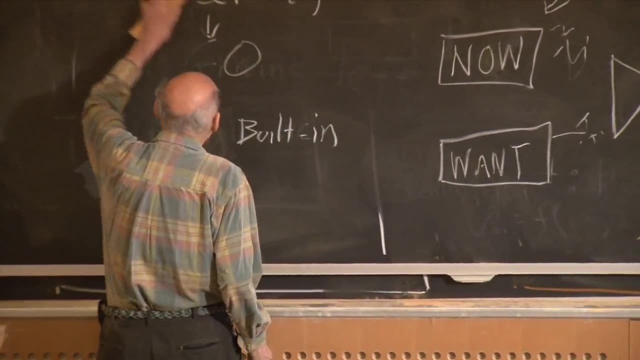 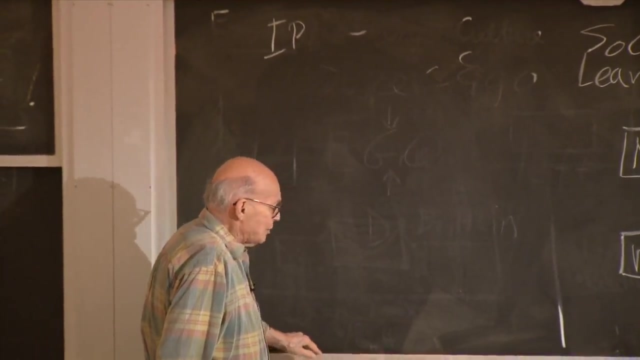 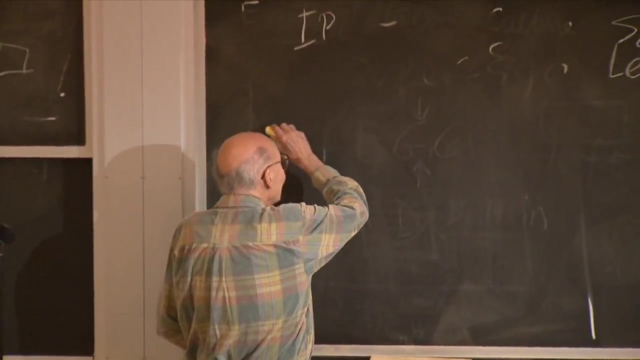 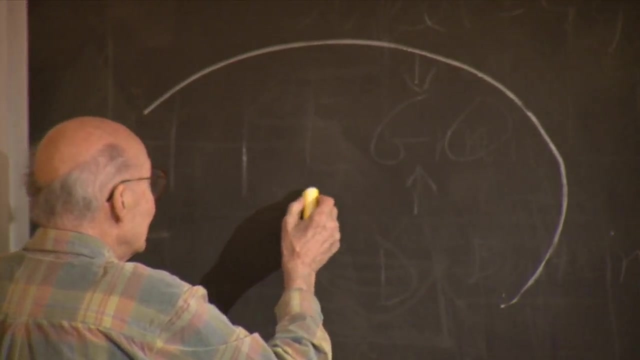 That's an important question, Thank you. We know quite a bit about the fundamentalism, the functions of some parts of the brain, and so, if you, I don't think I've ever tried to draw a brain, but there's a structure called the amygdala. 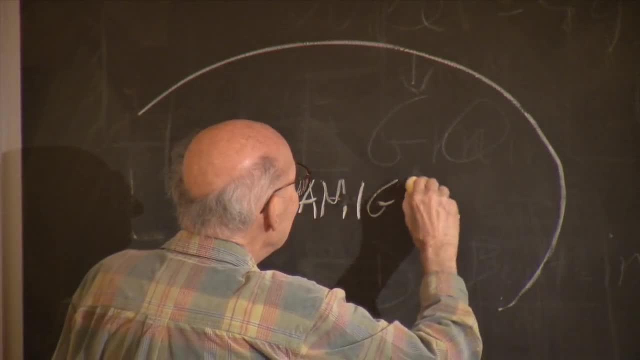 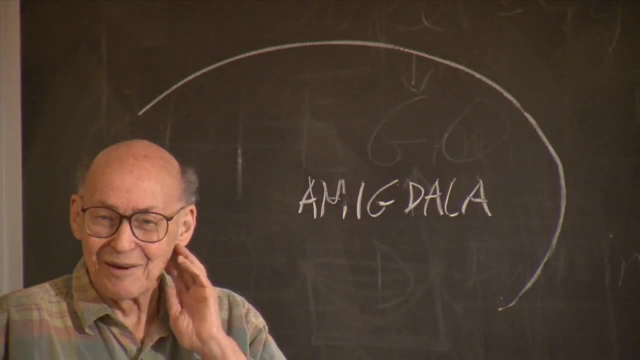 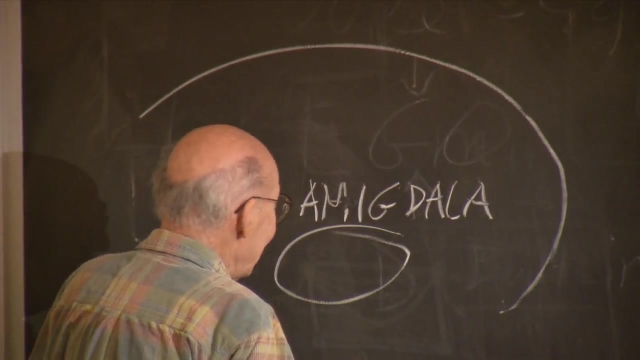 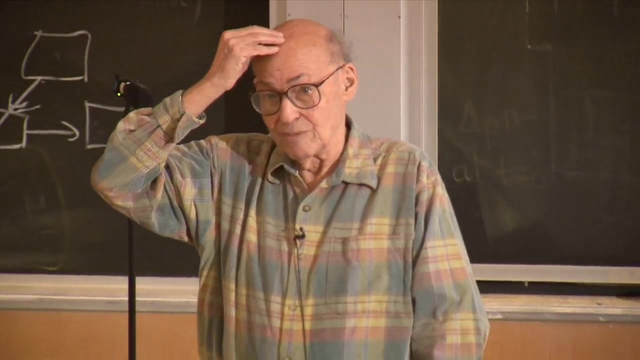 How do you spell it? I believe that means almond-shaped. Is that right? Anybody have a Google handy And that's down here somewhere and it has the property that it contains the short-term memories. So anything that's happened in the last couple of seconds. 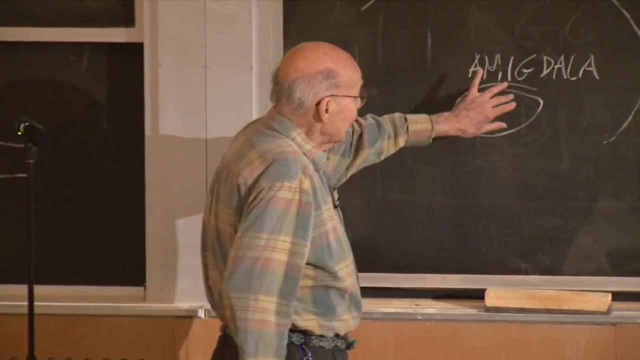 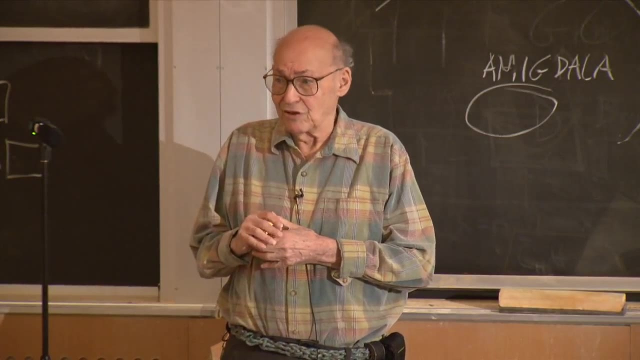 is somehow represented here in a transient way, and everything that's happened in the last 20 minutes or so leaves traces, and everything that's happened in the last 20 minutes or so leaves traces. and everything that's happened in the last 20 minutes or so leaves traces. 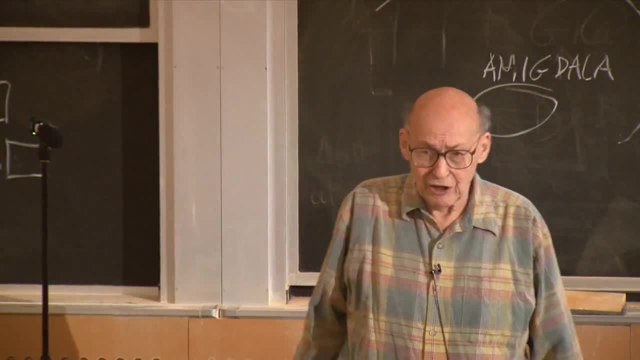 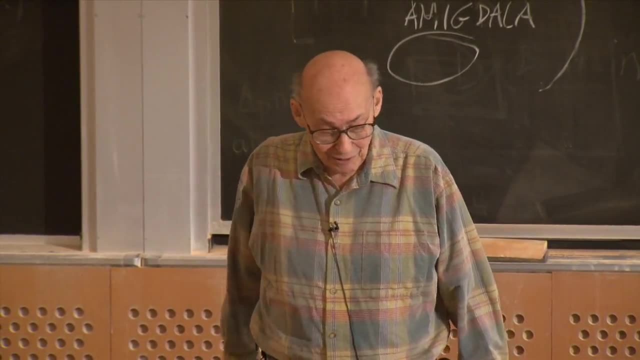 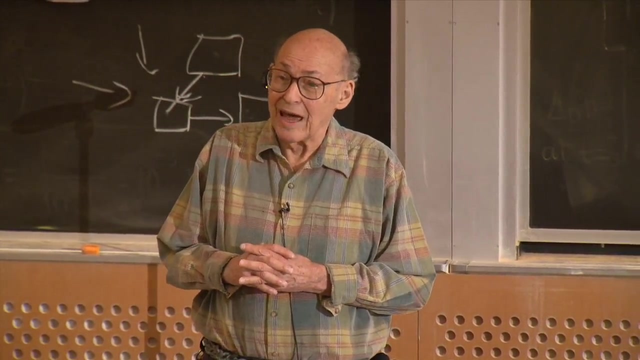 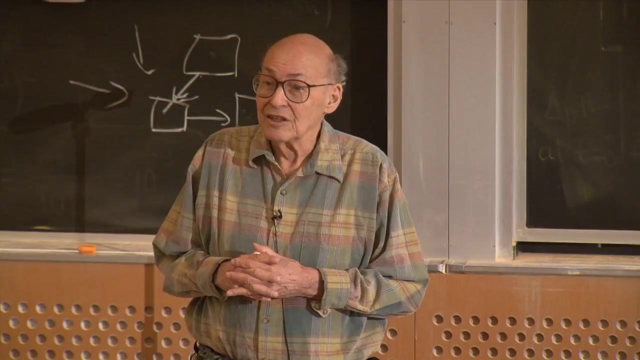 in the amygdala, so that if somebody's in an automobile accident or is knocked out by a real powerful boxing punch, then when you wake up later you can't remember anything. that happened in about 20 minutes or a half hour before the trauma. 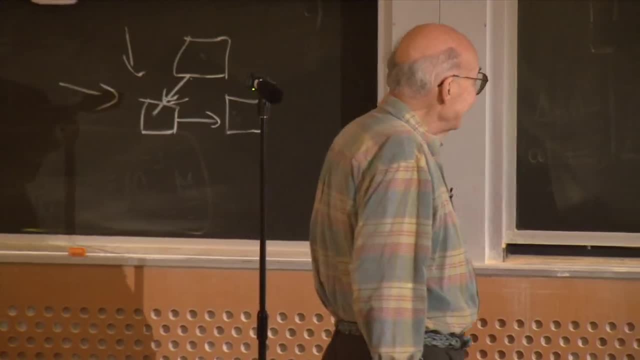 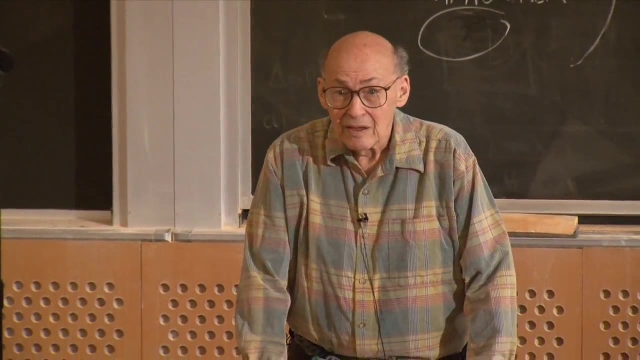 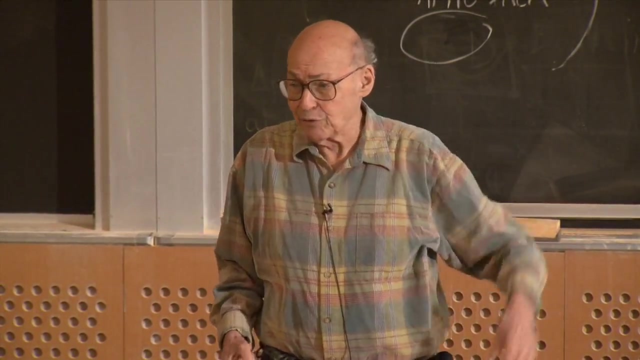 So that's a very good experiment to try, and there's a lot of evidence that this happens, because the memories of the last half hour or so are stored in the conjecture is in a dynamic form. Maybe there are huge numbers of loops of neurons. 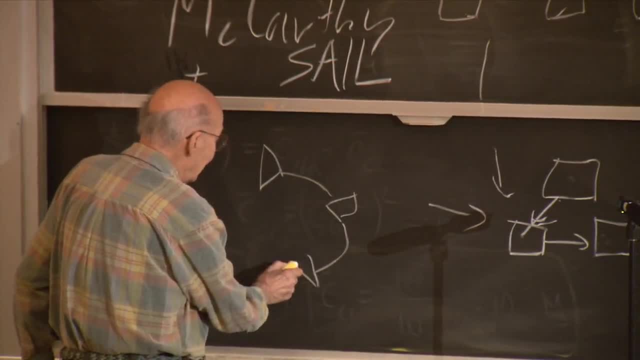 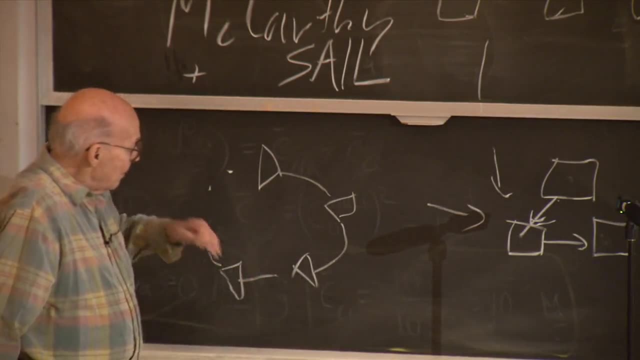 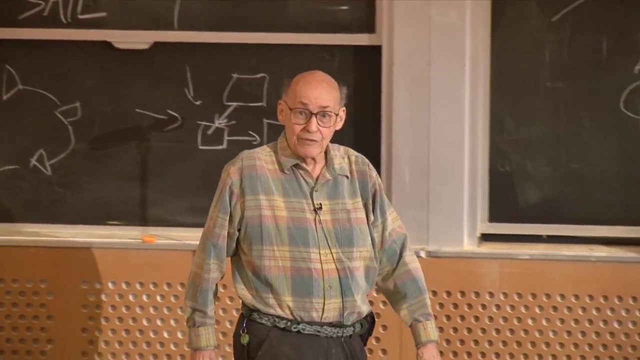 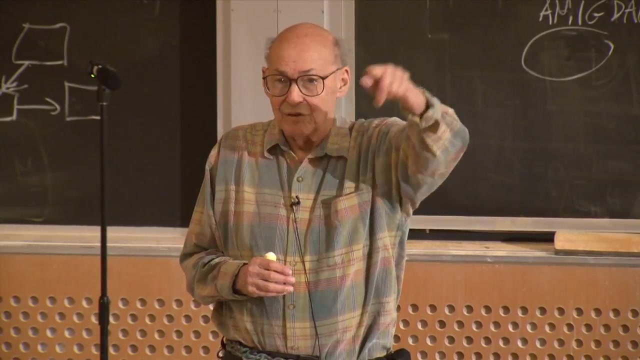 connected in circles or circle, Anyway, nobody really knows. So if you have a bunch of neurons connected in a big circle, maybe 20 or 30 of them, then you can probably put 10 or 20 bits of information in the form of different spaced pulses. 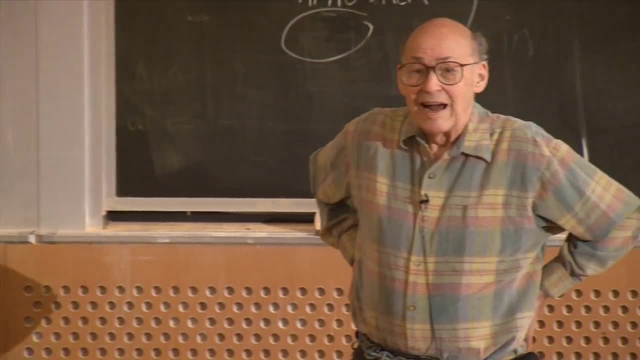 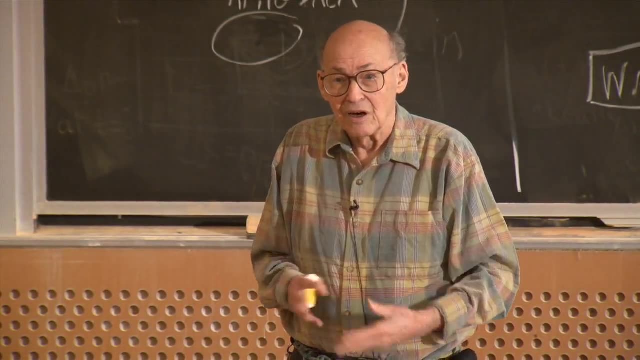 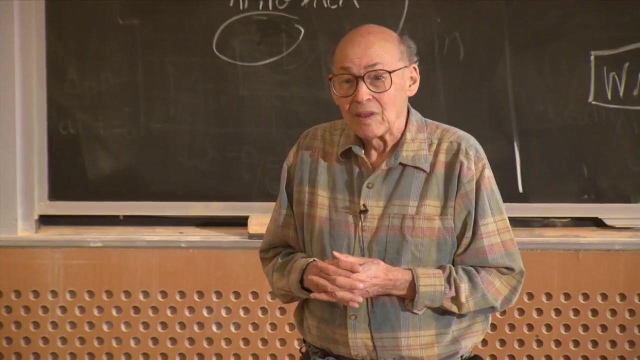 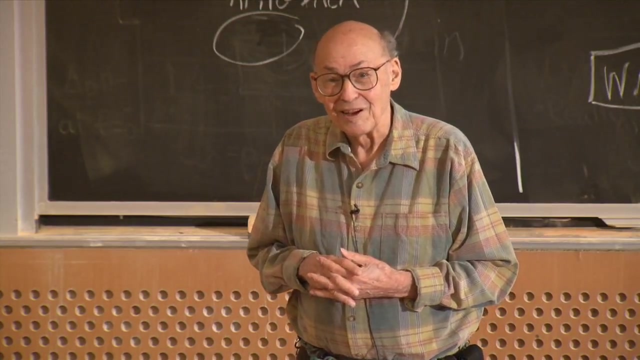 and a great mystery would be: how does the brain manage to maintain that particular pattern of pulses for 10 or 20 minutes, And then no one knows where it goes after the 20 minutes. but if a person gets enough sleep that night, then it turns out that it's no longer in the amygdala. 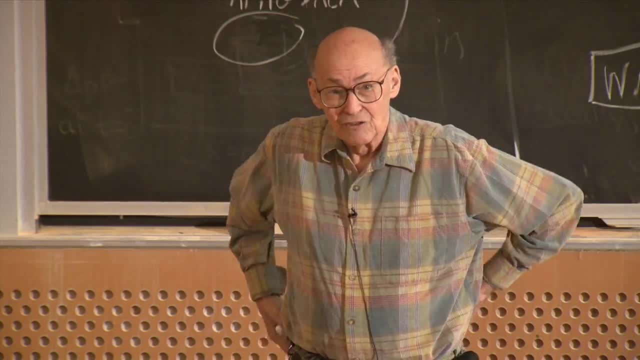 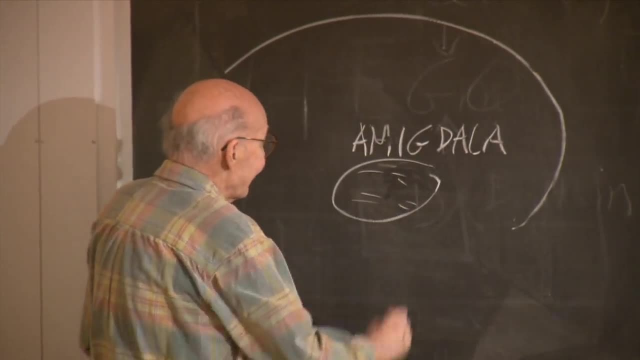 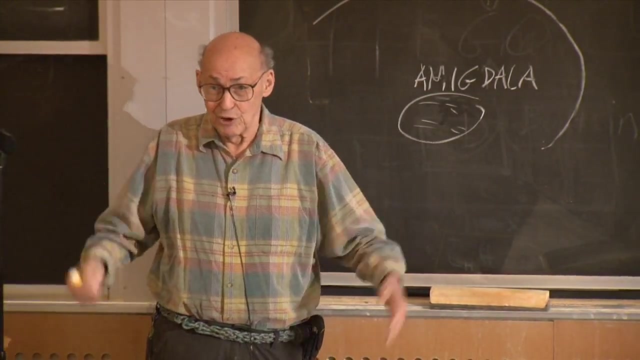 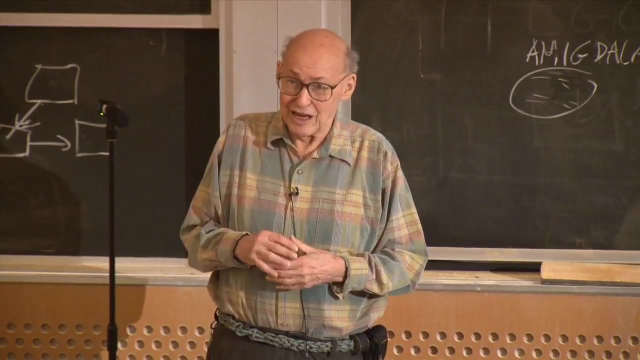 and it's somewhere else in the brain, And so one question is if there's all this stuff stored here and you might think of it as what's happened in the primary memory Every computer starts out with. maybe just the first computers had just two or three registers. 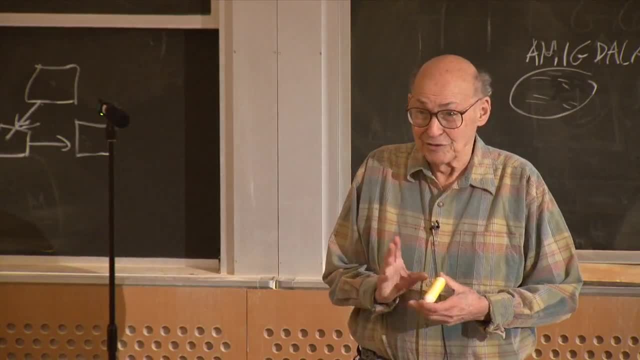 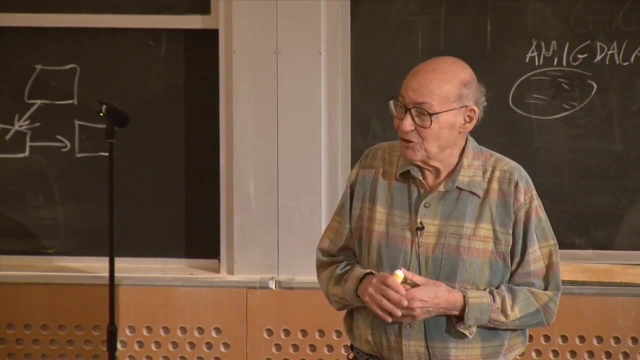 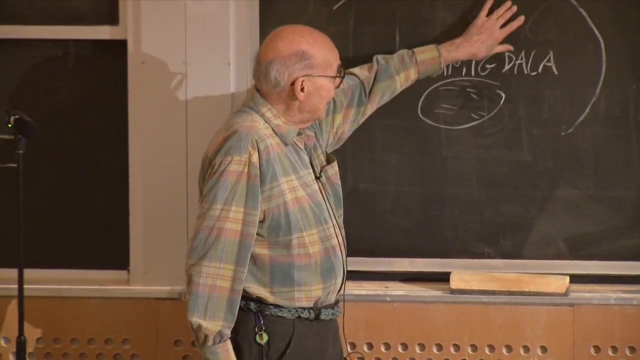 Then they got 16 and 32.. And I imagine how many fast registers are there in a modern computer. I haven't been paying attention, Maybe 64,, maybe whatever, But anyway they're gone. but the next day, if you've gotten some sleep, you can retrieve them. 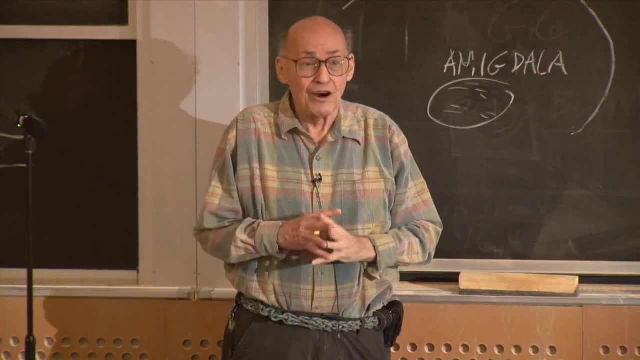 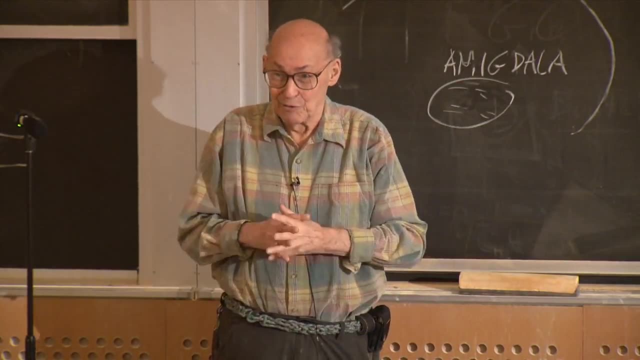 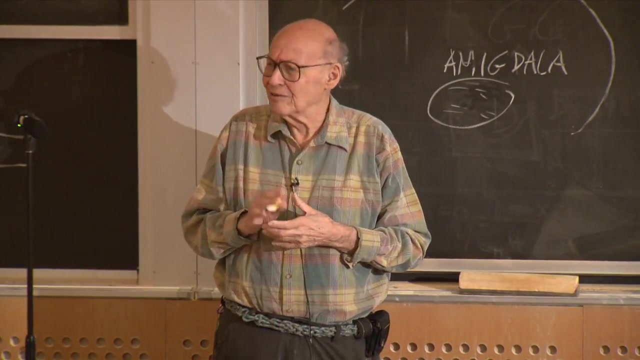 Somehow they're copied somewhere else. As far as I know, there is no theory of how the brain decides where to put them and how it records it, and so forth. Something very strange about this big science lacking theories, isn't there? What would you do if you were in a profession? 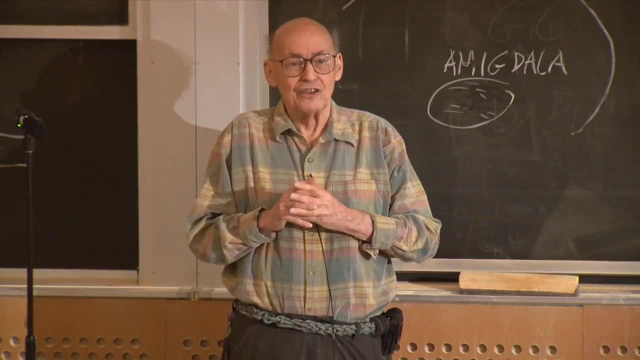 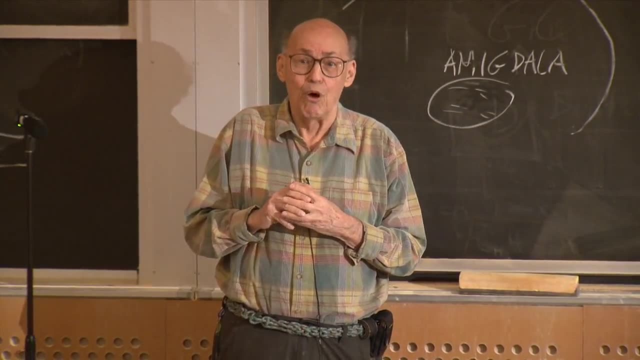 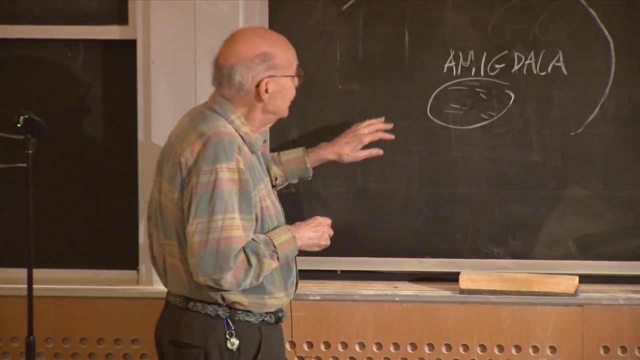 where they're talking about dozens and dozens of mechanisms which clearly exist, and you say: how do you think that works? And they say: well, I don't know. None of my friends know either, so I guess it's OK. So we don't know how it picks a place to put them. 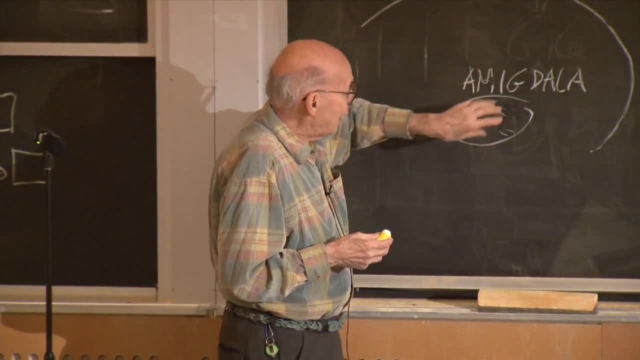 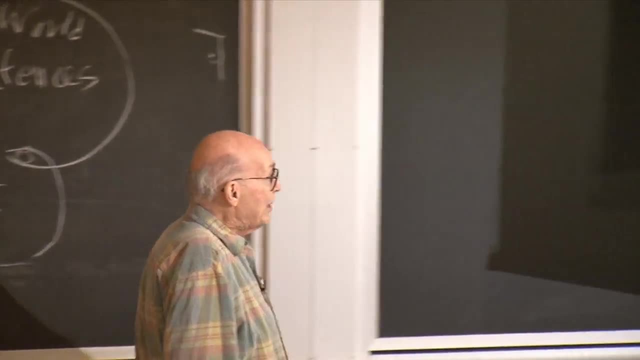 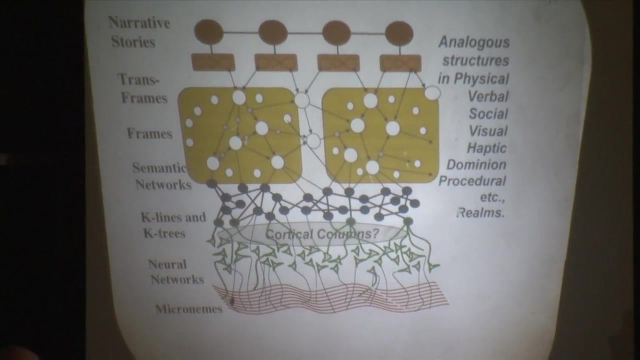 and we don't know how, when you ask a question, it gets back there so that you can reprocess it and talk about it, But anyway, so I made up these theories that things are stored in the form of K-lines, And there's a lot of discussion in the Society of Mind. 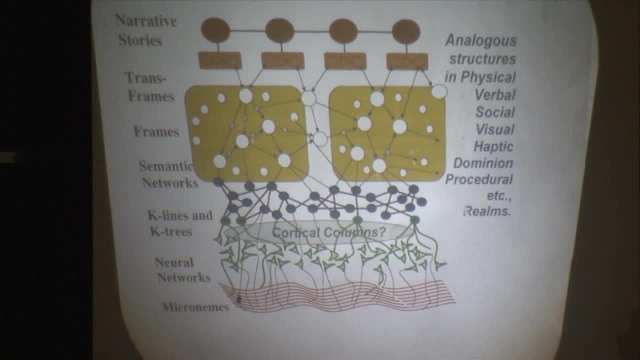 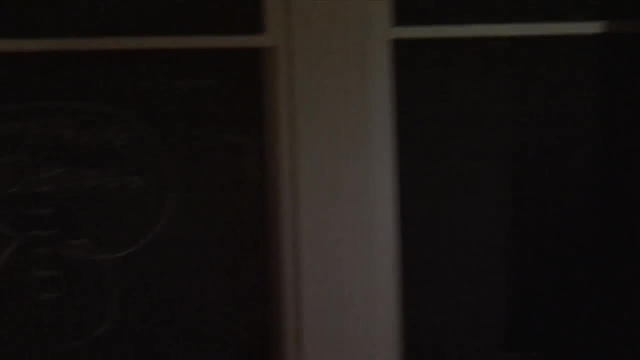 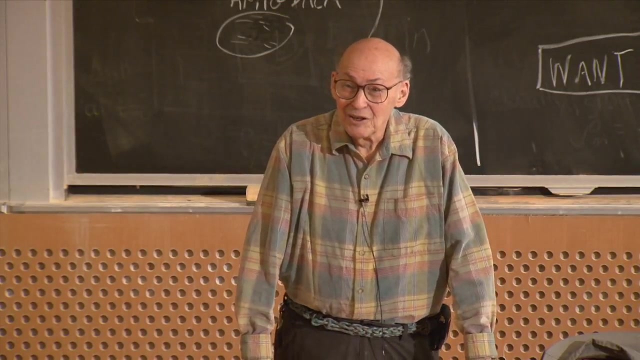 about how K-lines probably have to work and so forth. And if you look at the Society of Mind in Amazon, you'll find this enraging review Bye A neurologist named Robert Restack, who says he introduces these undefined terms called K-lines. 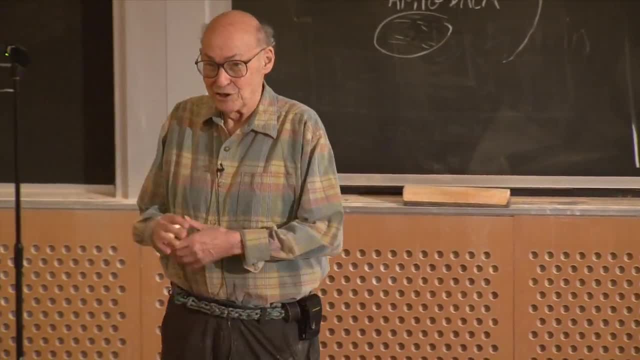 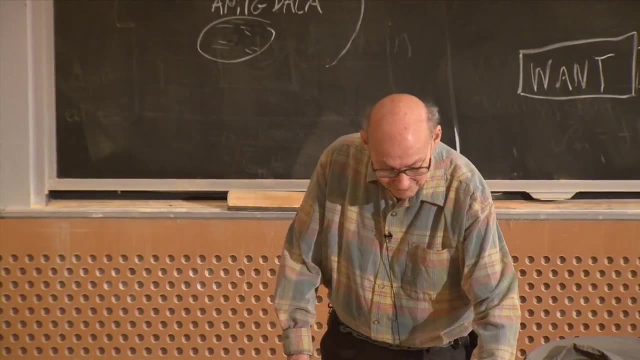 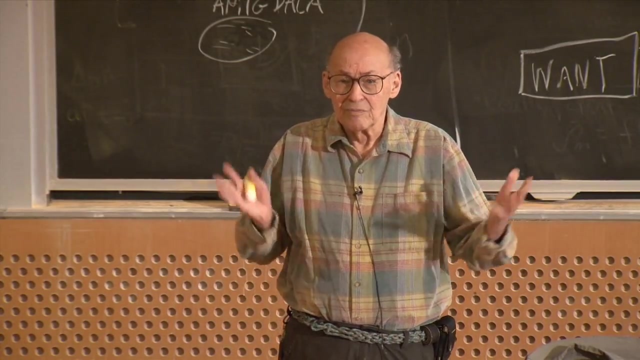 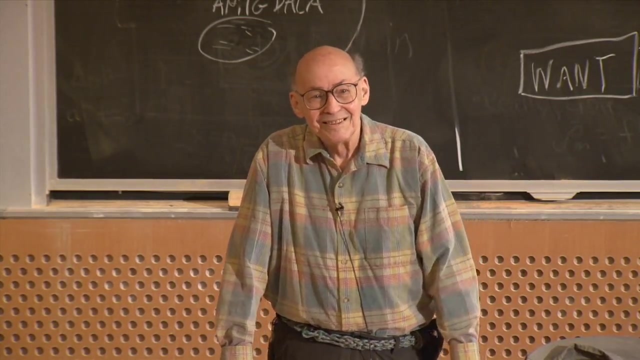 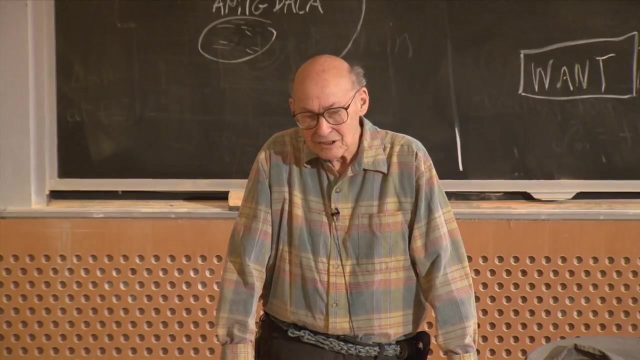 and paranomes and things like that, of which there's whole chapters in the book. So that's my favorite review of the explaining the problem of getting neuroscience to grow up. Yes, Who had a question? Yes, So one thing that provokes me is: how do you think? 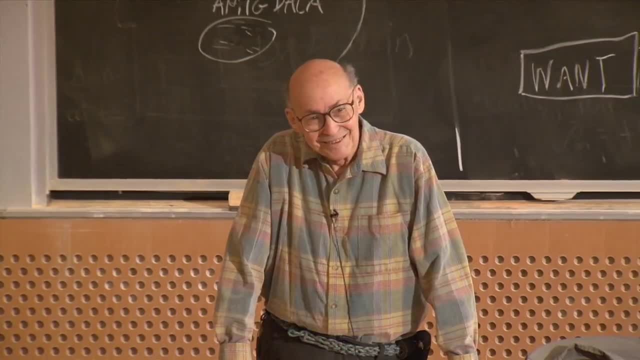 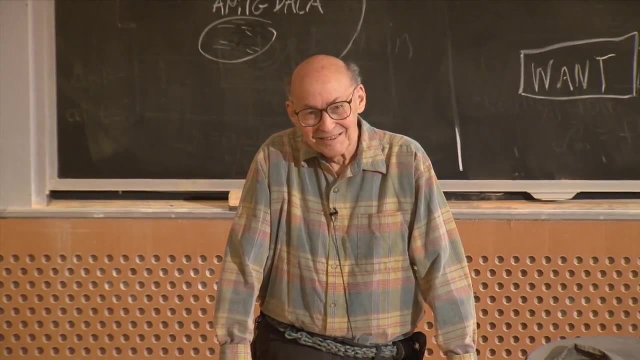 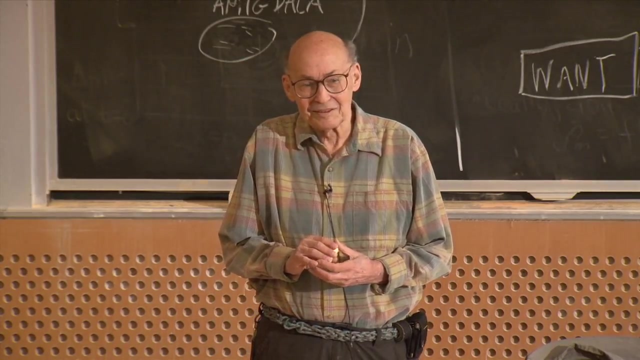 the brain decides to do things. How do they decide what to do, did you say Well, say you want to relate a story, but hundreds of things happen. how do you select what to tell and what not? to Right, Right. 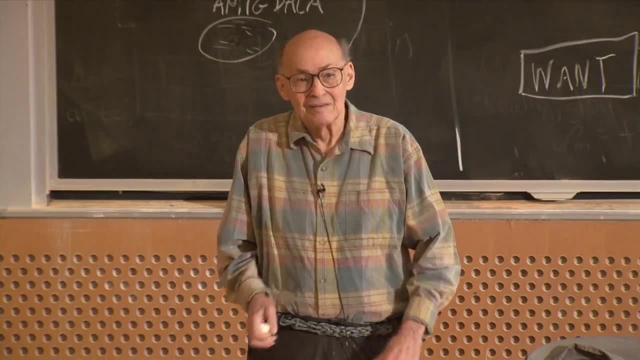 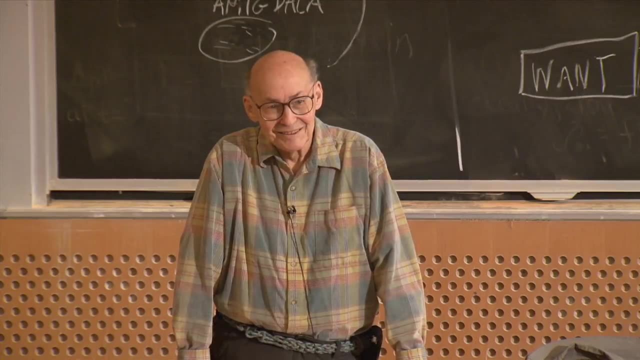 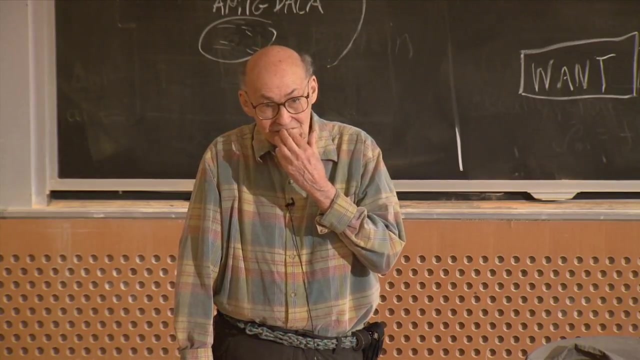 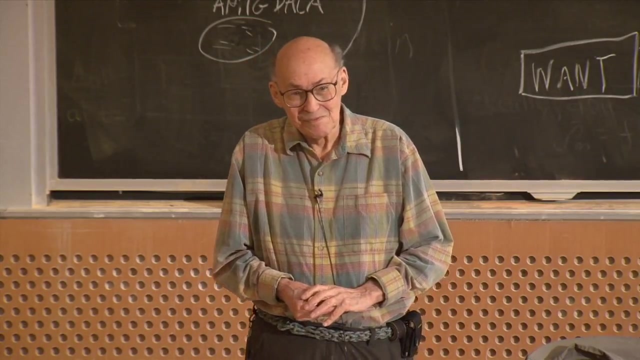 So it seems like you need some sort of intentionality behind it. but how do we learn to do that in the first place? almost When you describe a goal, you describe what's going on now and what's the thing you want, But then how do you decide which few things to be considered? 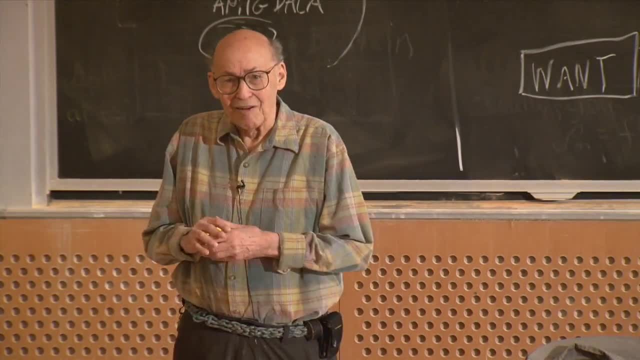 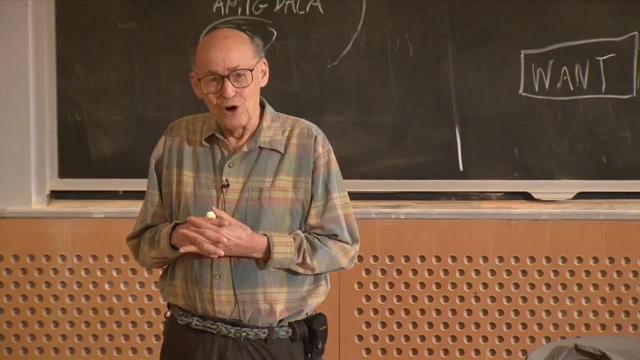 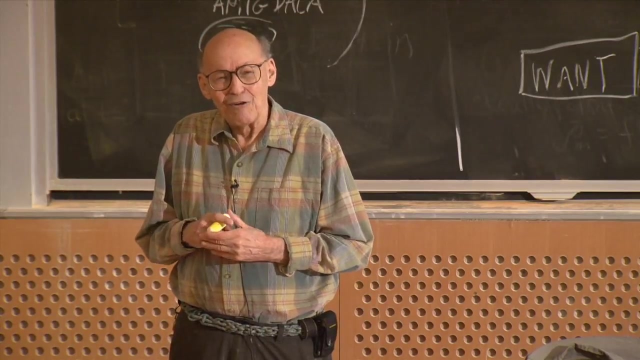 Oh, you're asking a wonderful question, which is, after all, if I were to talk to you for an hour about your goals, you could tell me hundreds of goals that you have. So the question is: how do you pick the one that you're? 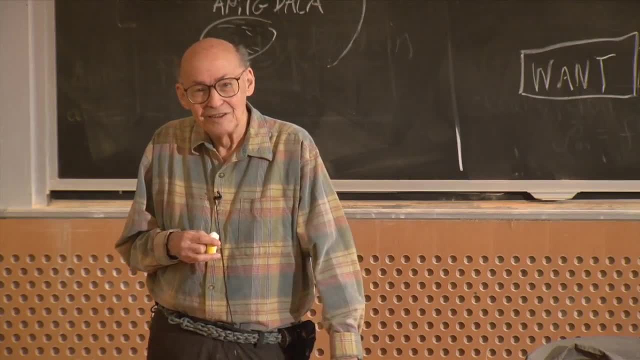 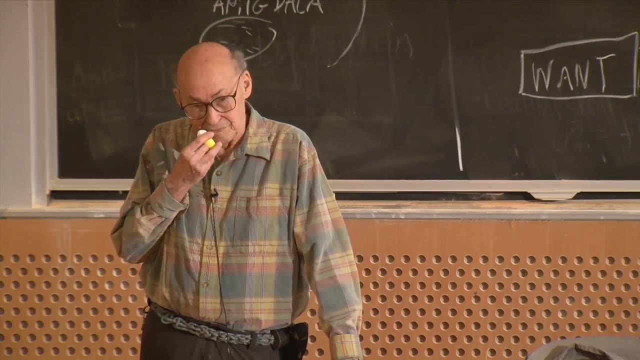 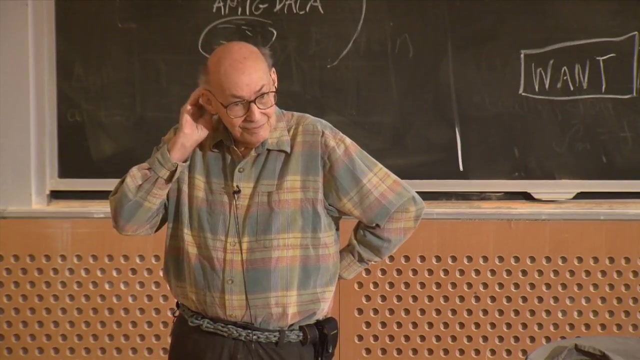 thinking about now. Yeah, also, how do you represent the priority of goals, Because they're almost described as defense machines that turn on all the time. But how do you resolve conflicts? How do you decide which one to go first and which one gets first? 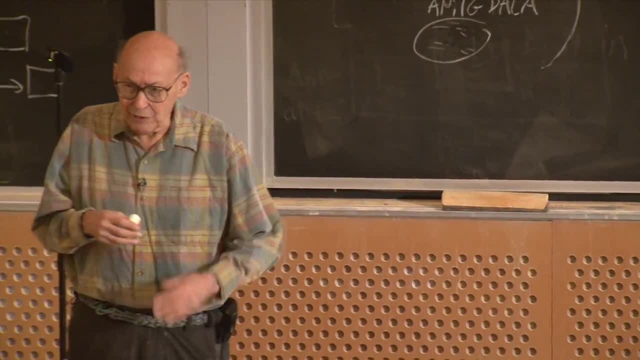 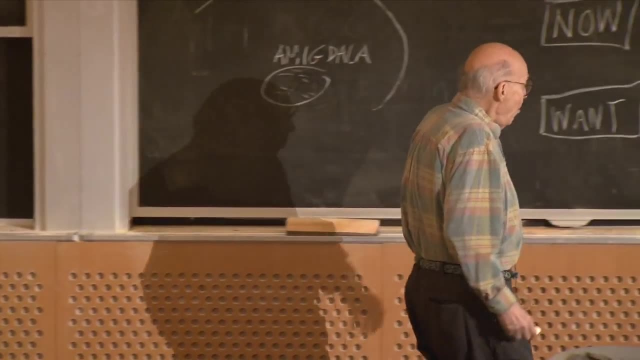 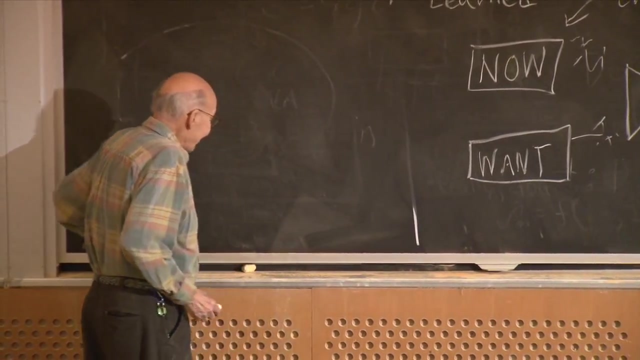 OK, How do you represent the relations of your goals? The standard theory, for which there's no evidence, is that in fact, you used the word hierarchy. So if you ask a naive person, they'll give you a pretty good theory. 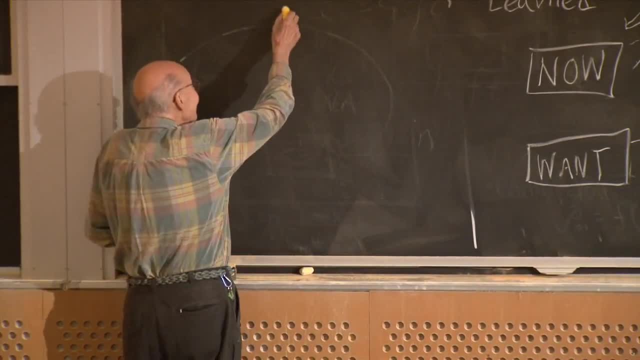 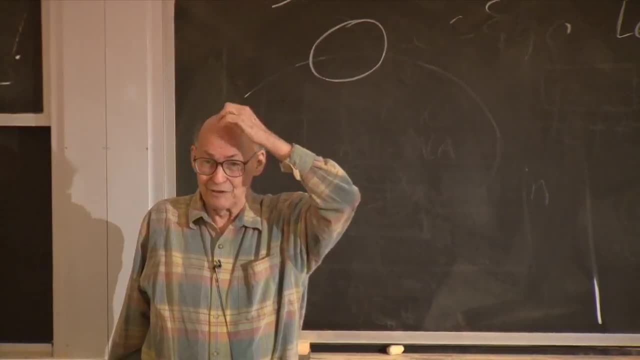 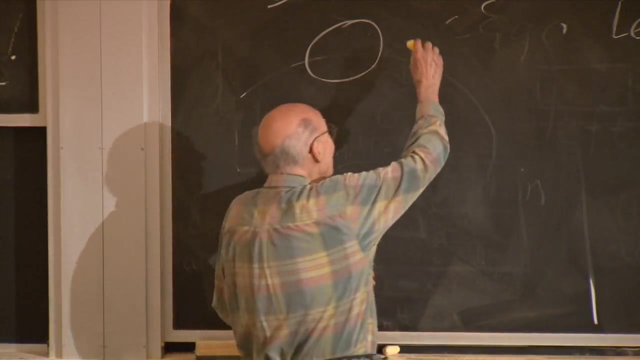 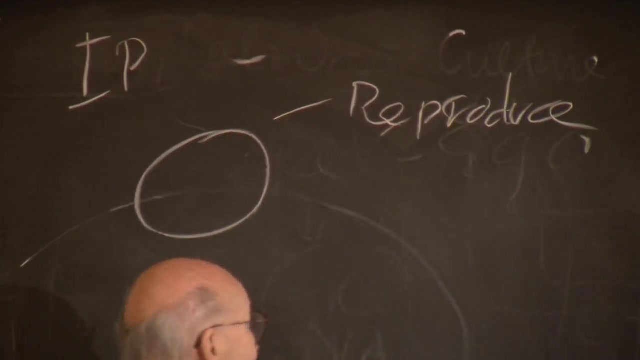 Well, completely wrong, but good. And the standard theory says, well, there's one big goal at the top And you say, what is it? And some people would say, well, maybe it's to reproduce. Darwin could, but didn't argue that. 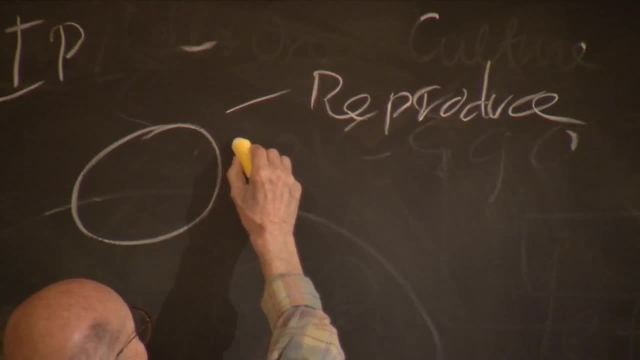 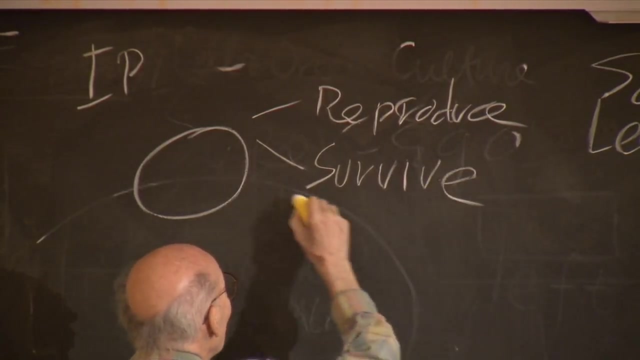 Or Or to survive or something like that. OK, So if you take that one, then it's obvious what the next calls in the hierarchy would be. I'm not saying this is how things work. I don't think it does. 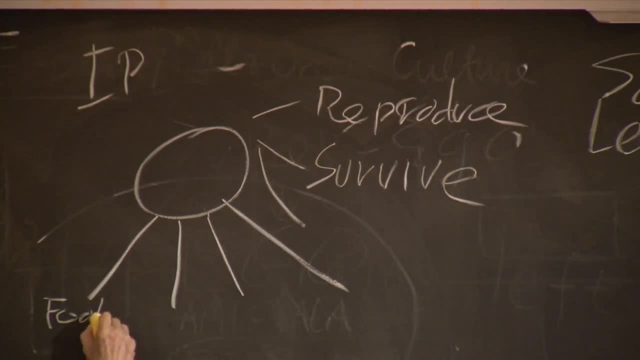 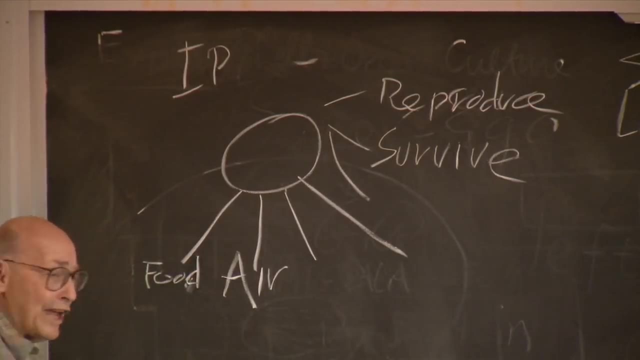 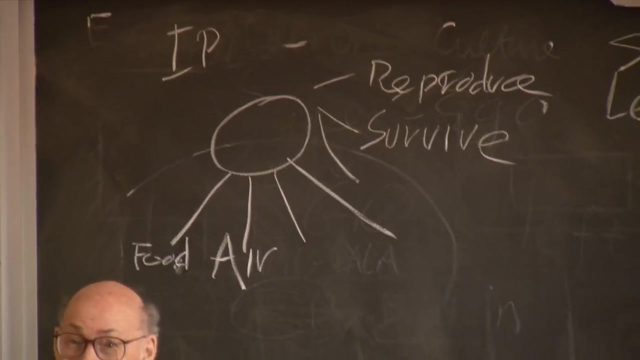 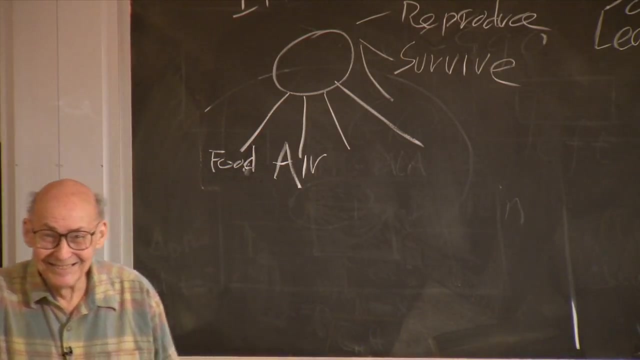 But so there's food and there's air, But air gets very high priority If you put a pillow over somebody. their first priority is to breathe And they don't even think about eating for a long time. So that's very nice. 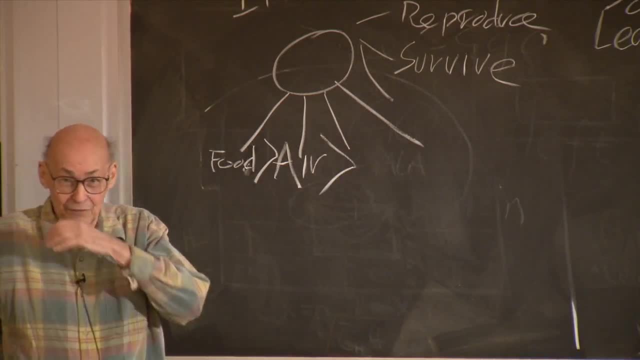 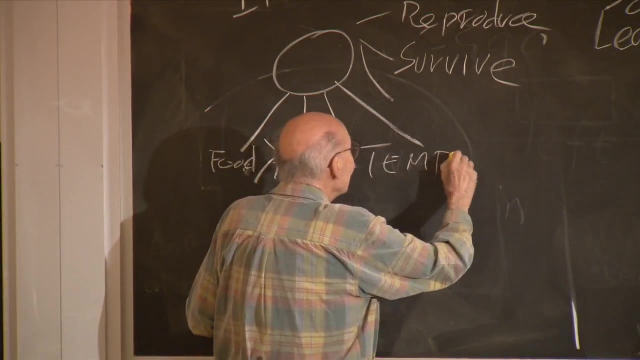 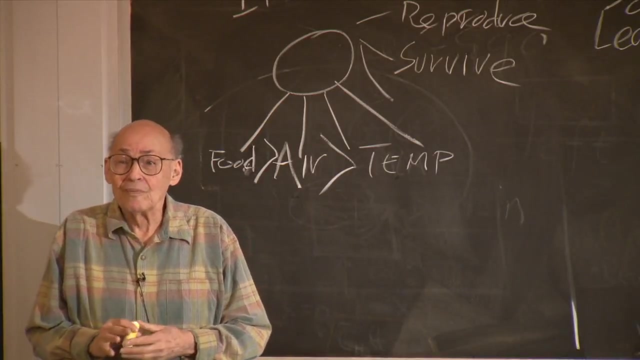 I don't know what comes after that. If you're out in the cold freezing, then OK, And there's temp. The nice thing about air and temp is that if you have those goals, you can satisfy them in parallel, Because in fact you don't need much of a hierarchy. 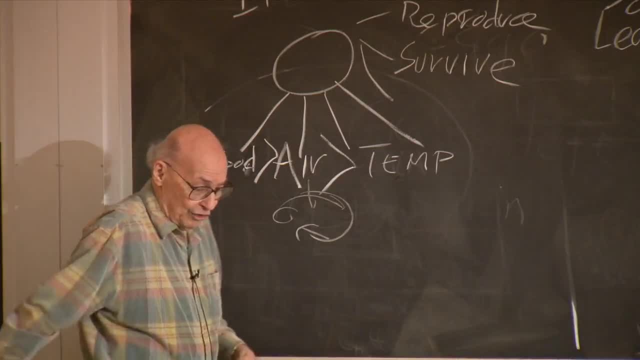 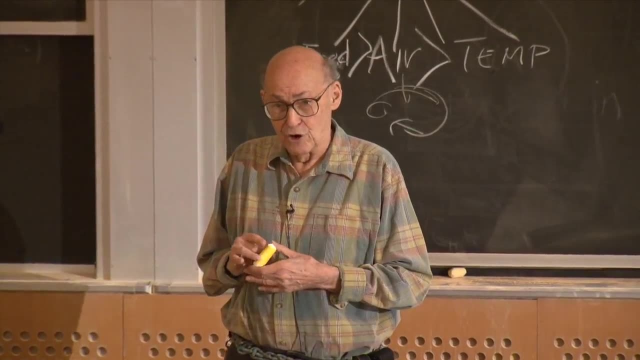 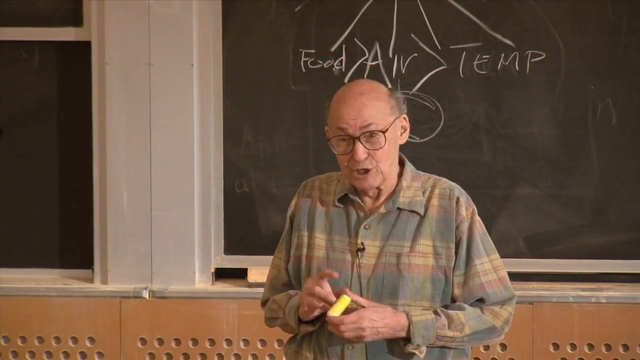 The breathing thing has this servomechanism where, if there's a higher level of CO2 than normal in your blood, then the- what is it? the vagus- Yeah, The vagus nerve or I don't know. They know a lot about which part of the brain gets excited. 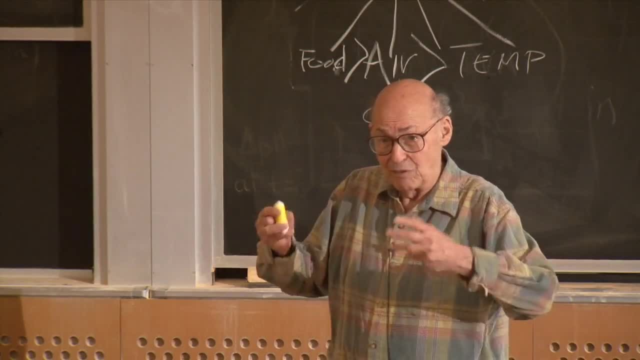 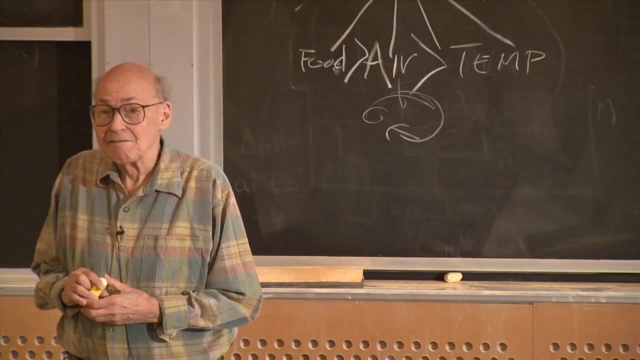 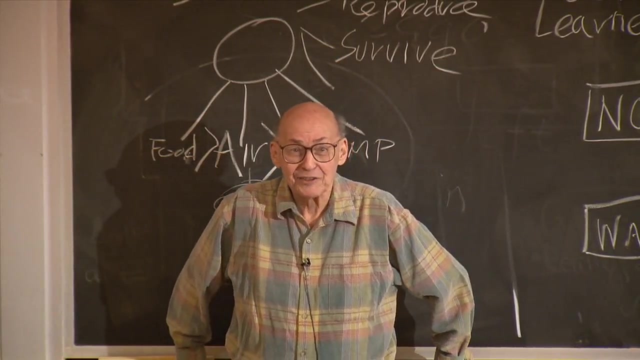 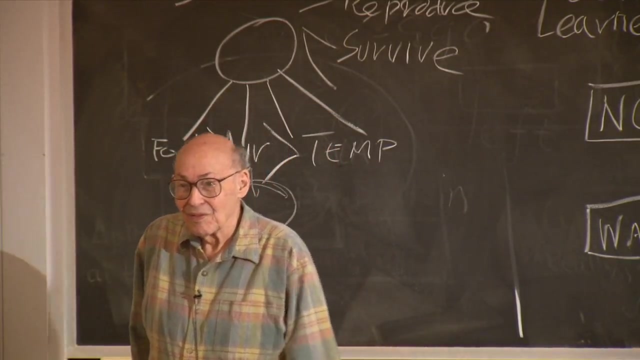 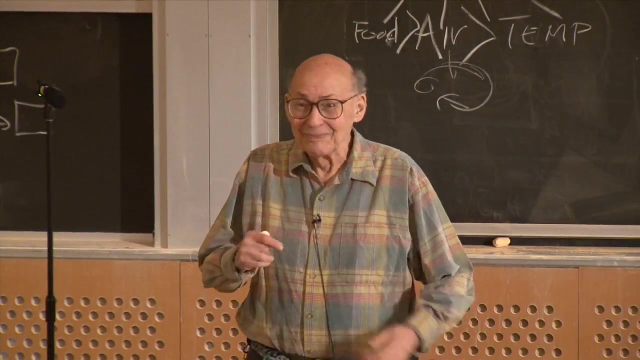 and raises your breathing rate or your heartbeat rate. or My favorite animal is the swordfish, because How many of you know about brown fat? Brown fat is a particular Thing found in invertebrates And it's fat, It's brown, I guess. 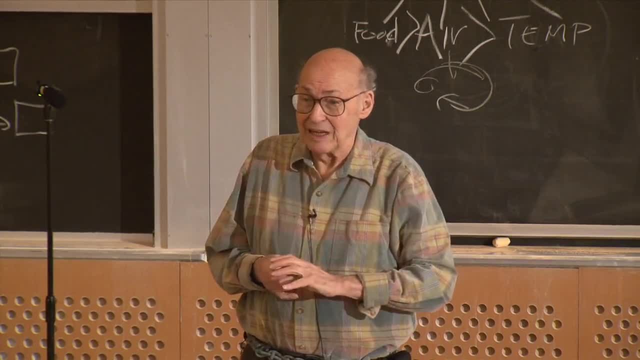 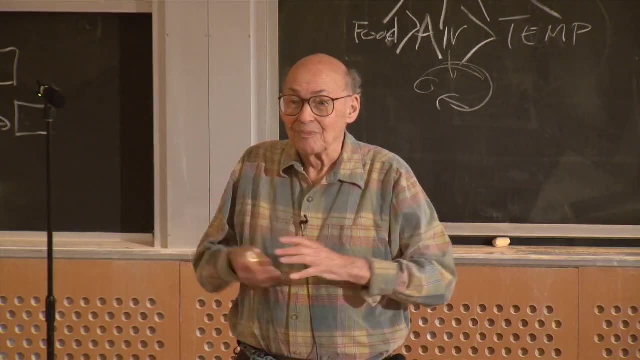 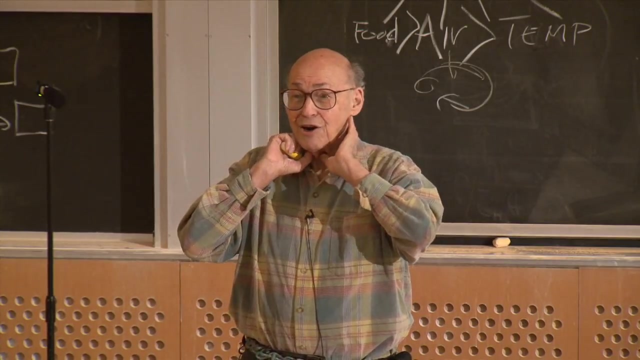 And it has the property that it can be innervated by nerve fibers and they cause it to start burning calories. And the swordfish is normally cold blooded but its carotid arteries have a big organ of brown fat around That. 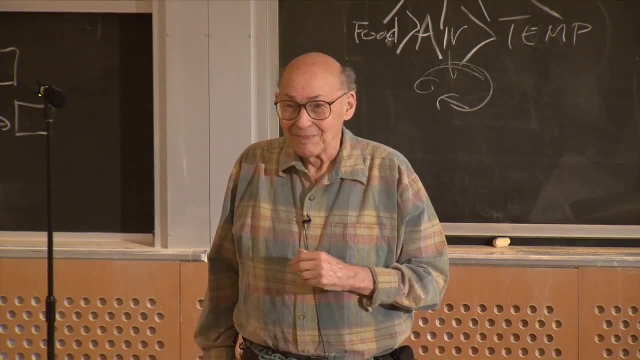 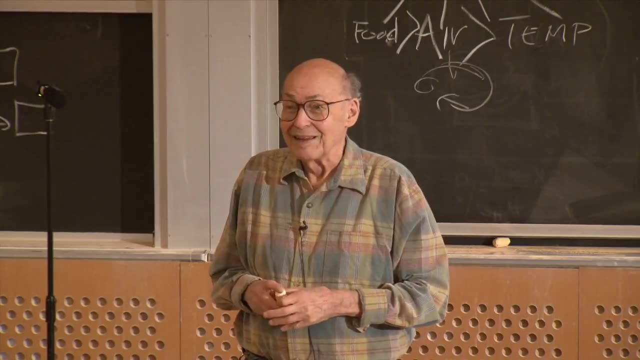 That's what's going on with them, just as the blood comes into the brain And if you turn on the brown fat, it warms the brain and the IQ of the swordfish goes way up And it swims faster and uses better evasive tactics. 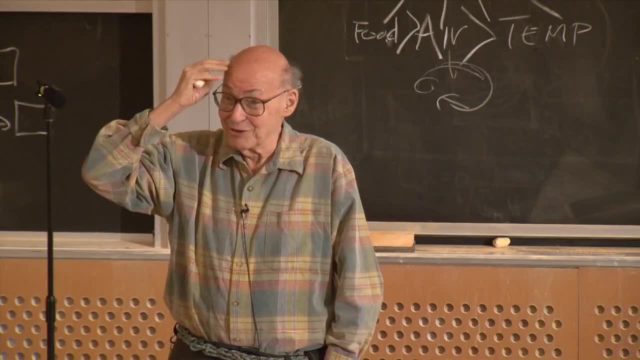 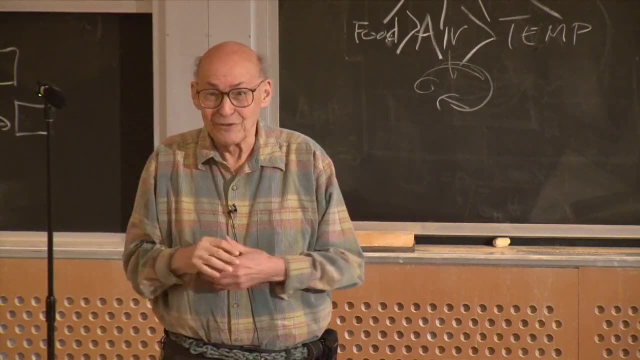 I'm trying to remember. There are a couple of other animals that are known to cold blooded, animals that are known to have a warm blooded brain, that they can. Isn't that a great, Great feature, I wonder. does our brain do a little bit of that? 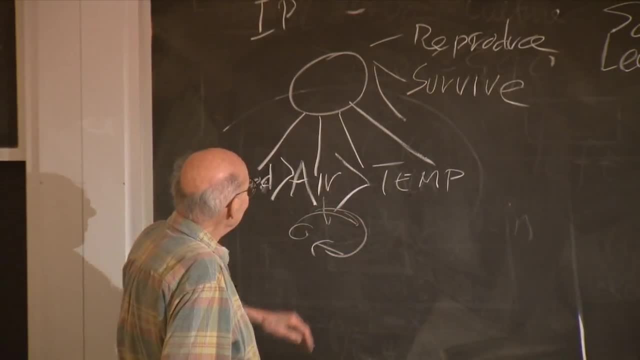 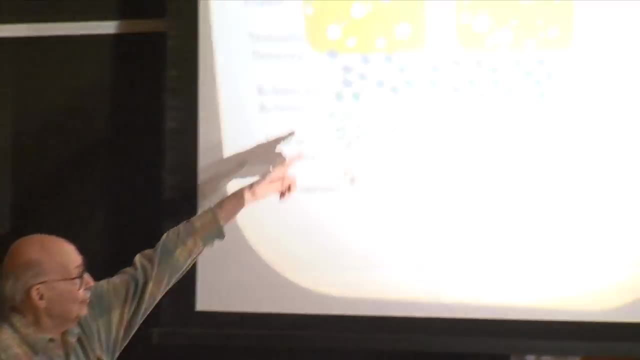 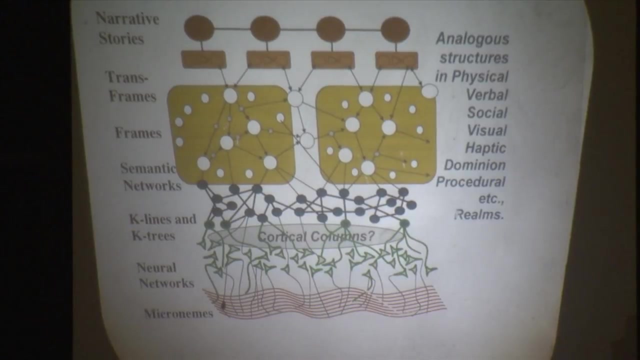 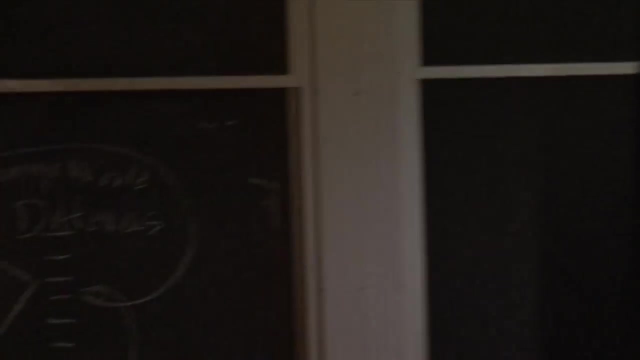 I got lost telling funny stories. So anyway, this K-line idea is very simple. It says that perhaps the way human memory works is that here and there you have big collections of nerve fibers that go somewhere and go to lots of cells. 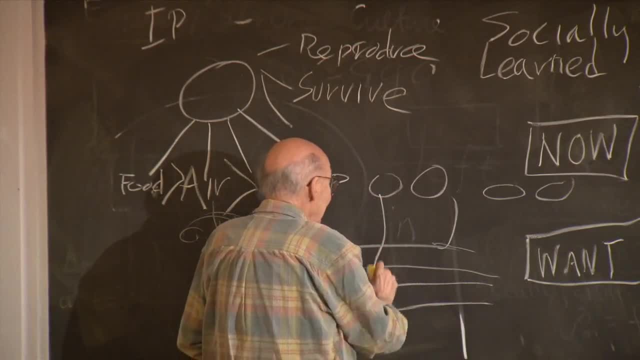 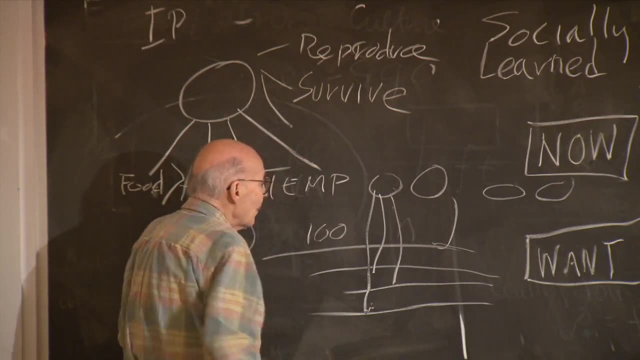 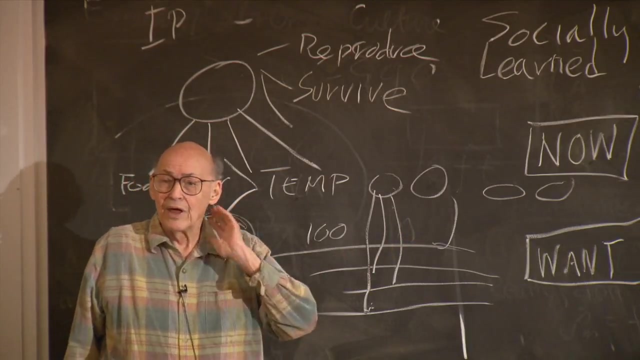 Let's say thousands of these cells and each one is connected to some particular combination. Imagine there's 100 wires here and each of these cells is connected to, say, 10 of those wires. Then how many different wires do you have? 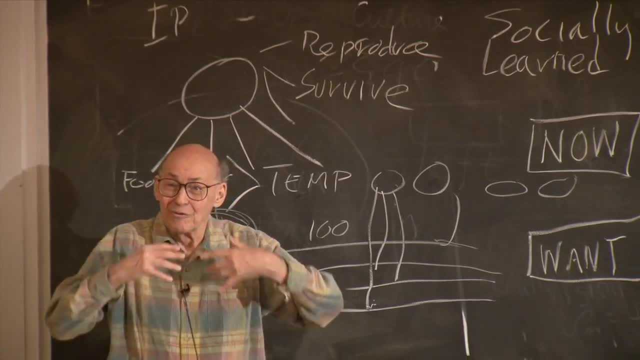 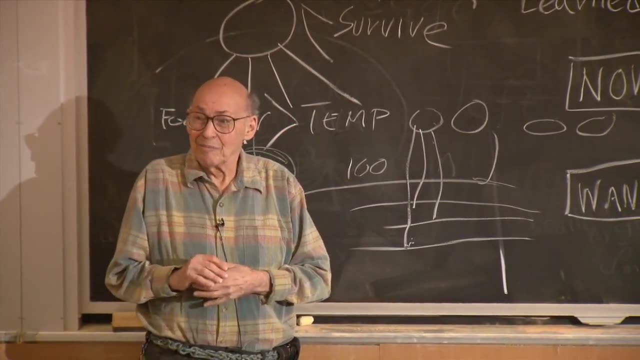 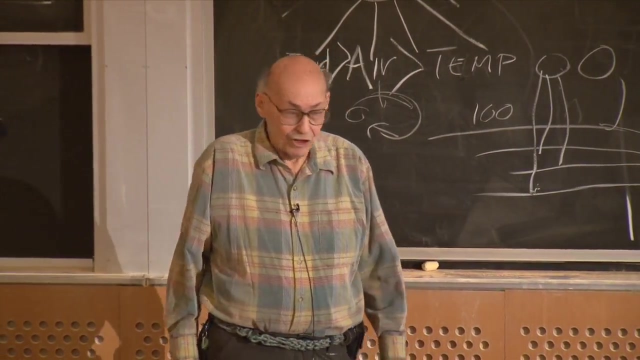 How many different cells could you have for remembering different features of what's on this big bus bar? Well, how many ways are there picking 10 things out of 100? It's about 100 to the 10th power. So here's a simple kind of memory where you have 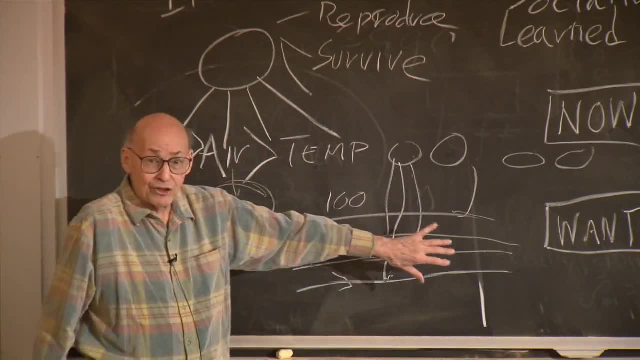 of course it'd be useless unless these bits by themselves have a little, have some correlation with you know, have some correlation with the other. So here's a simple kind of memory where you have. of course it'd be useless unless these bits by themselves have a little, have some correlation with the other. 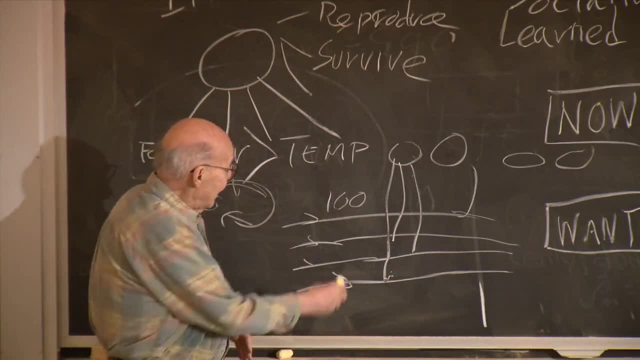 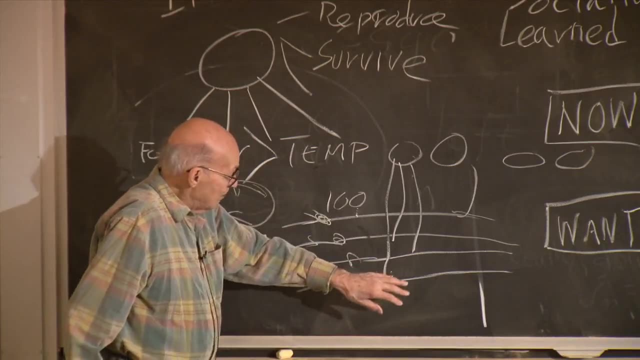 So here's a simple kind of memory where you have. of course it'd be useless unless these bits by themselves have a little, have some correlation with some useful concept, And then, at any particular time, on this particular bunch of fibers in the brain, maybe 20 of these are turned on. 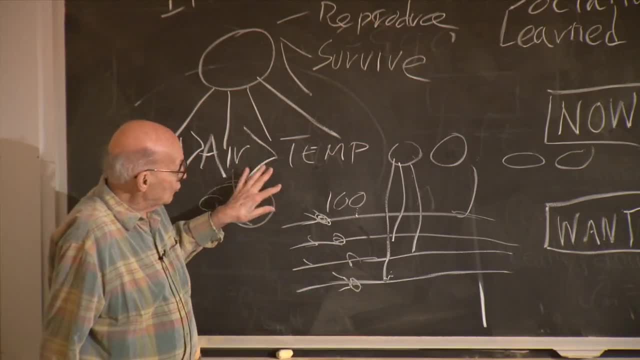 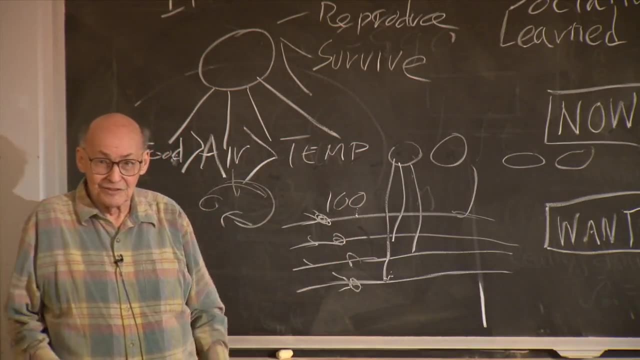 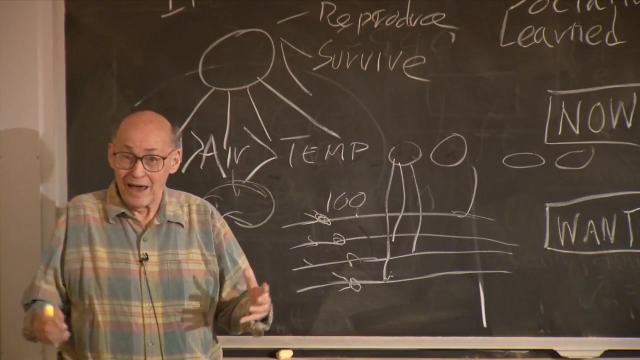 And if something very important has happened, you send a signal to all these cells and say: any of you cells who are seeing more than 10 or 15 of these 20 fibers at this moment should remember that and set themselves to do something. 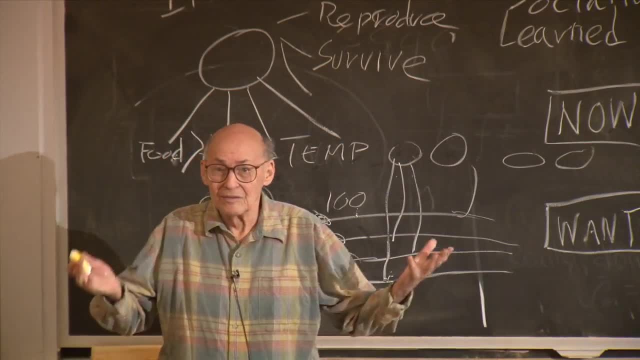 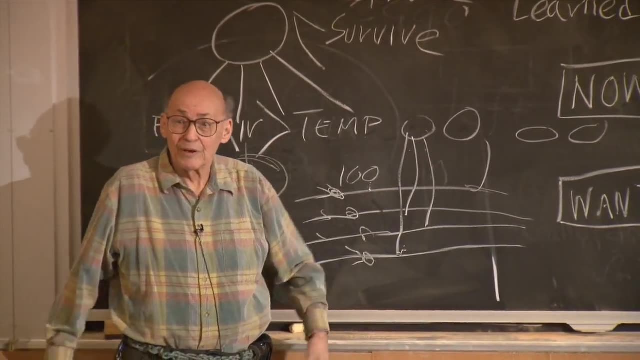 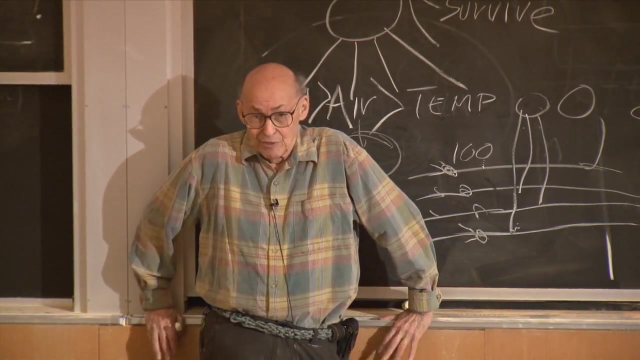 next time you see that pattern, something like that, Something has to decide which of these cells is going to copy at this time, and so forth. So there's a theory of how kind of symbolic memory might work in the brain, And I got this idea from a paper. 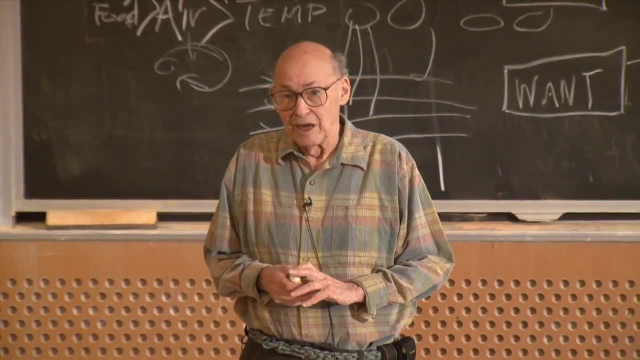 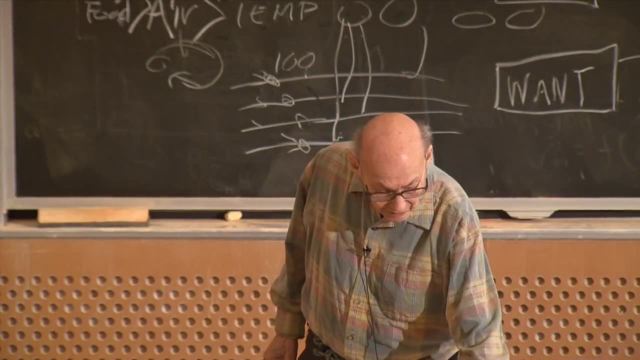 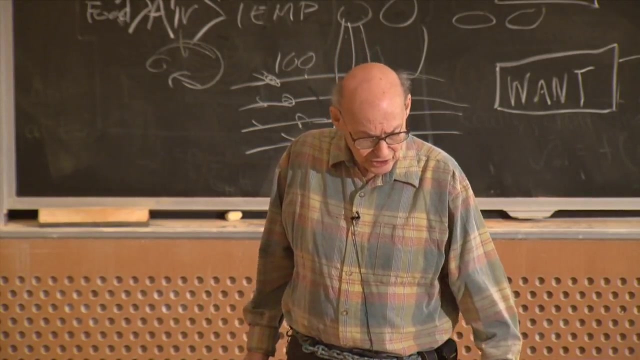 I don't remember what their idea was, but by David Waltz and Jordan Pollack. Pollack is an AI theorist- at Brandeis, I guess- who in recent years has turned into some kind of artist and makes all sorts of beautiful things and simple robots. 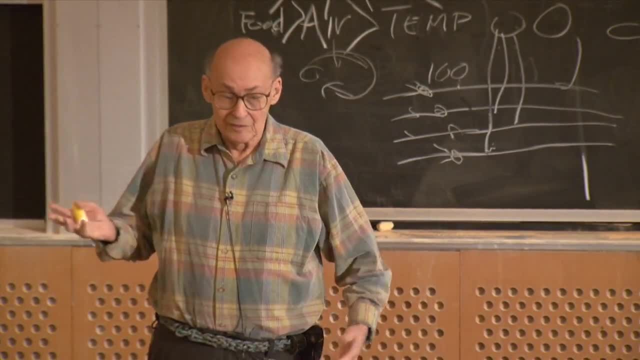 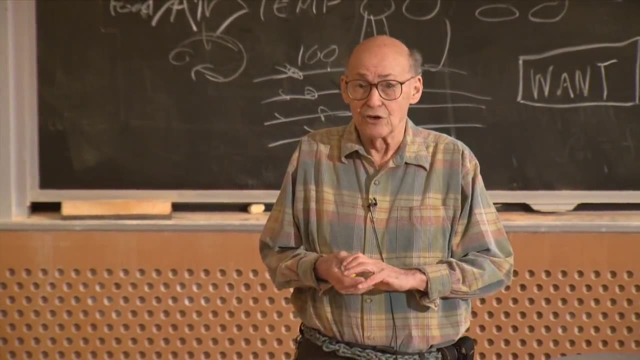 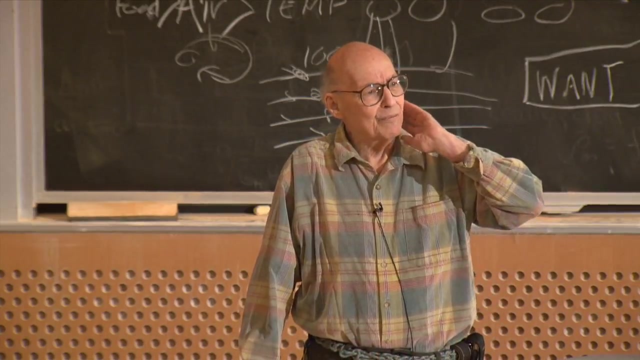 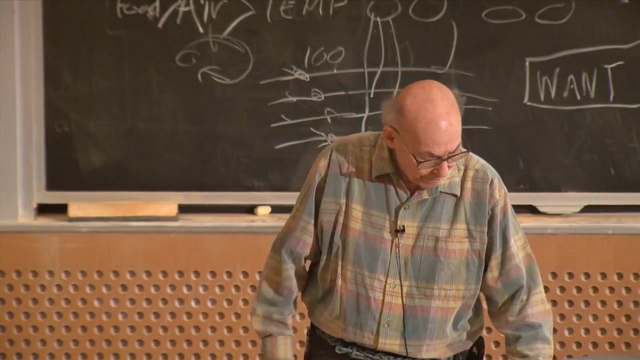 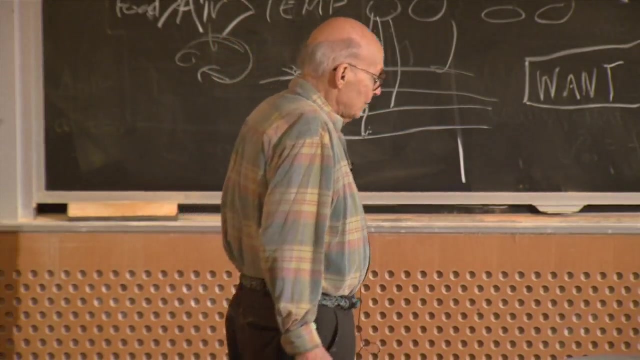 that do this, and that David Waltz searched his web page sometime because he was here for many years as a graduate student and then developed beautiful theories of vision. When did Dave move? Do you remember Pat? Anyway, something like that, But as far as I know. so I made up this theory, which 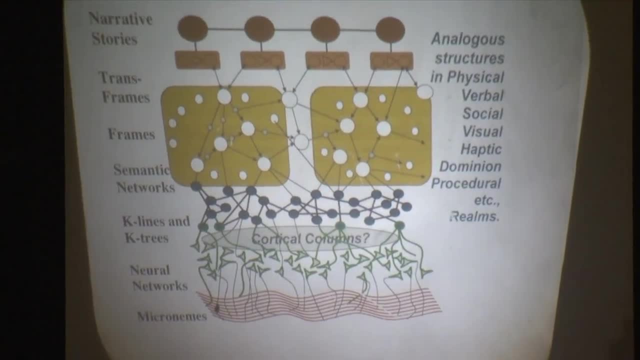 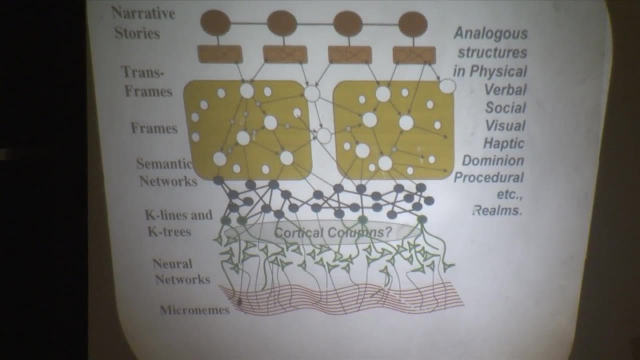 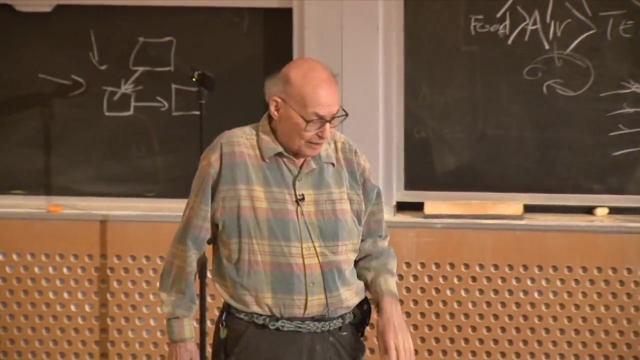 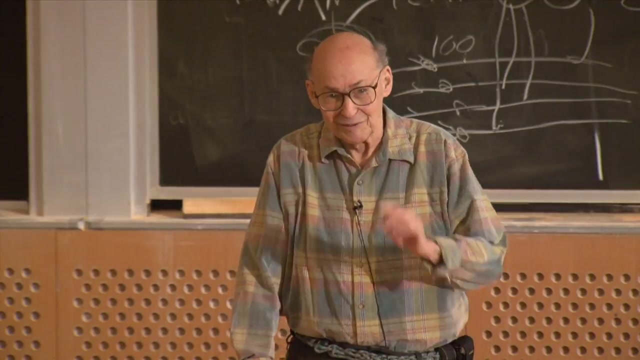 is really copied from Waltz and Pollack, but simplified and neatened up. And then I went on and made other theories based on that, But without them I would have been stuck in some conditioned reflex theory for a long time, I suspect. 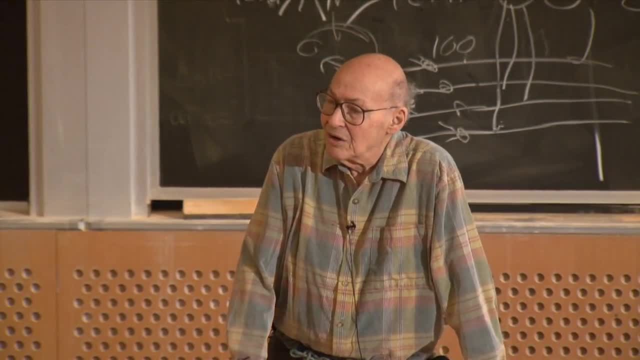 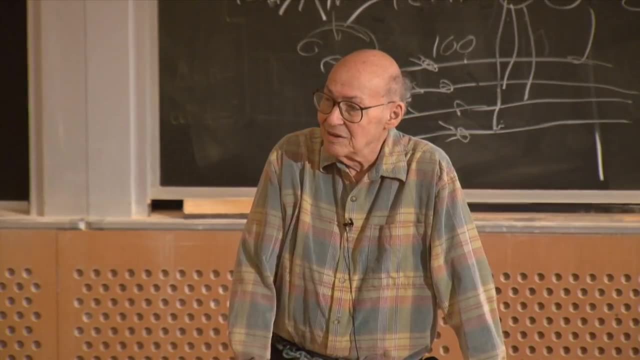 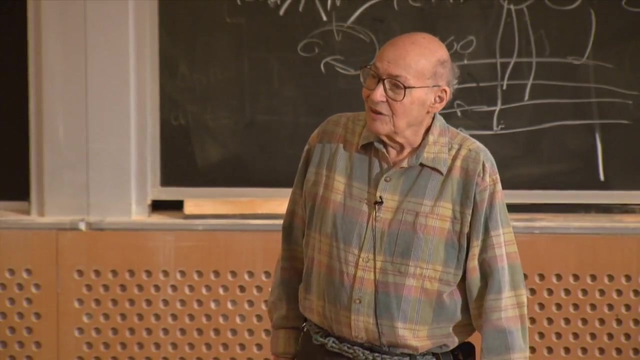 A minute, Yes. So, Professor, you mentioned the role that the amygdala plays in storing the short-term memory And you mentioned that the memories that are stored in there are wiped out. Well, that's a question, Presumably as you grow up your amygdala. 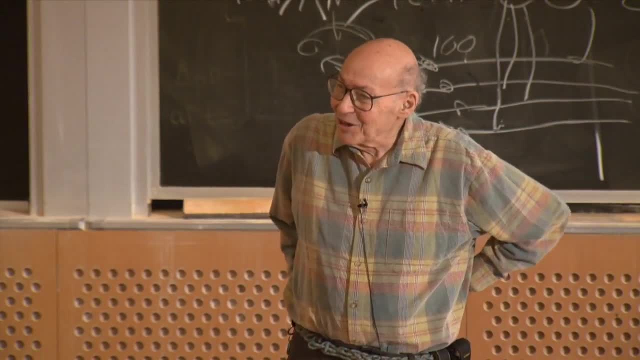 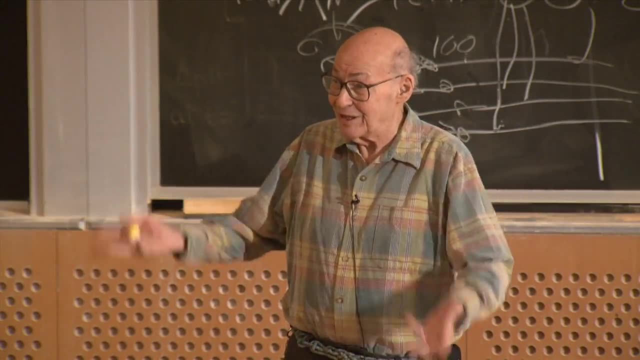 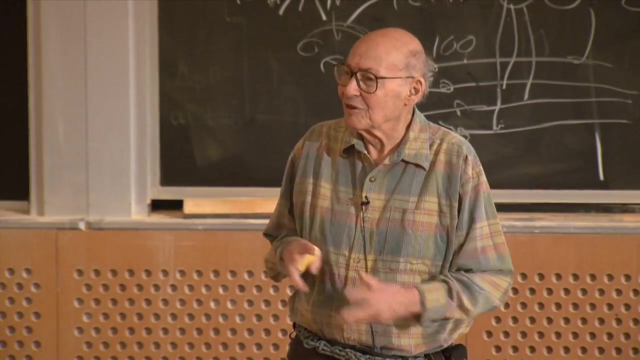 gets better at learning what to recognize, But I've never seen any discussion or theory of how much of your short-term memory is. how do you learn and develop and get better at remembering things that are worth remembering? Oh Sorry, Go ahead. 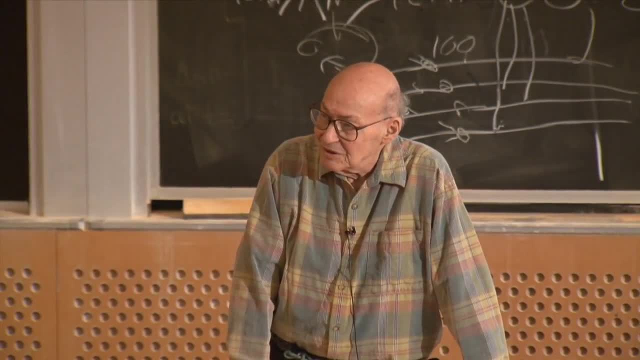 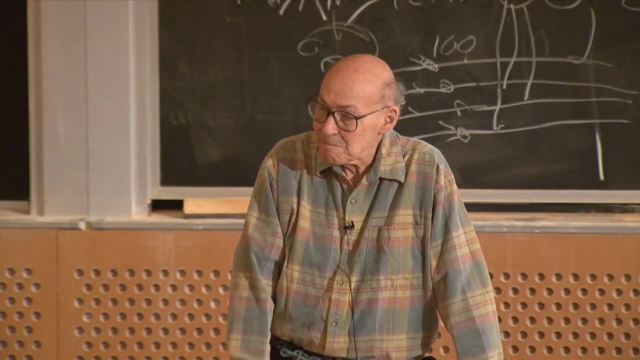 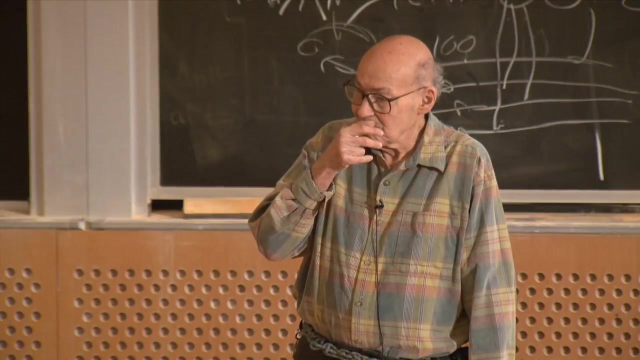 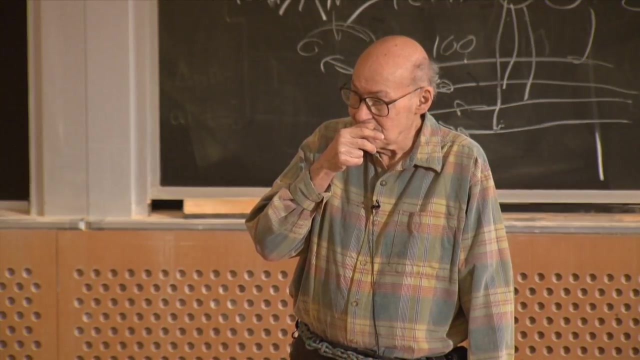 My question is that. my understanding is that. so whatever memories are stored in the amygdala during, whatever is stored in the amygdala is wiped out after you sleep, right? What sort of implications does this have about remembering dreams, Because my understanding is that after you have a lucid dream? 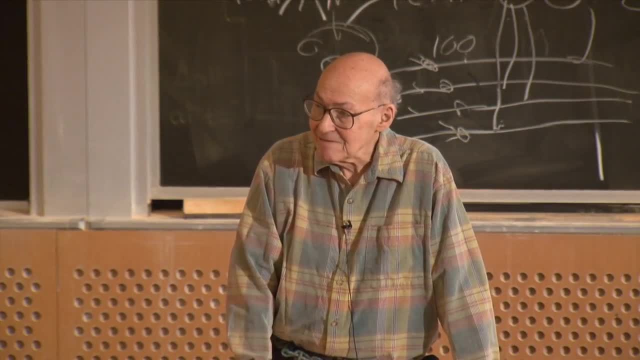 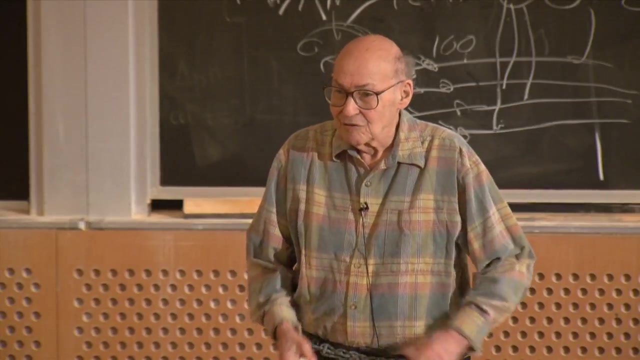 you tend to forget, And the memories of the dream are wiped out after a certain point later on in the day. So what sort of implications does it have on the ability of people to remember dreams that they have? Good question, There have been some theories, but I 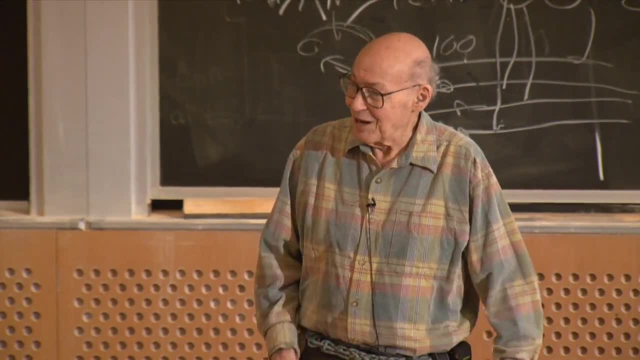 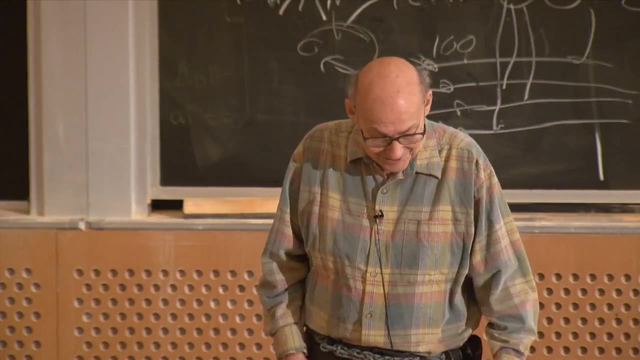 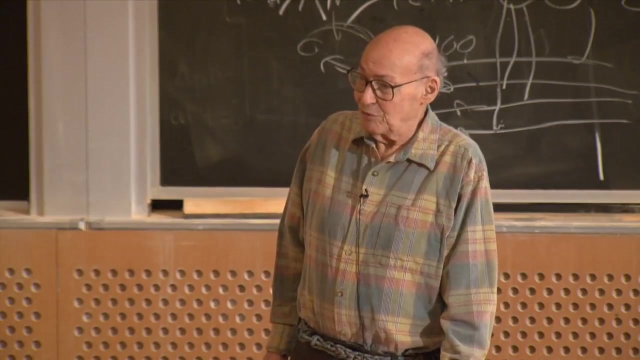 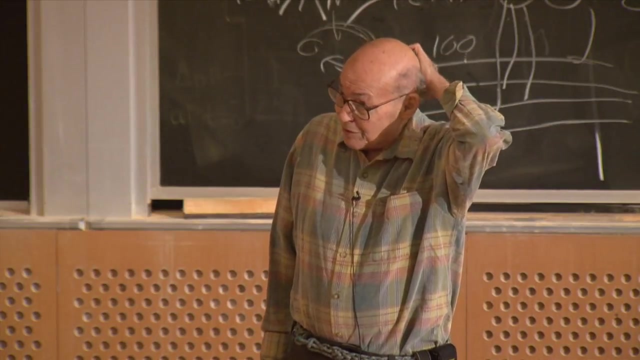 think I mentioned Freud's theory, which is that you're not remembering anything When you wake up. you make up the dream, And I think that's surely completely wrong. But Freud made it up because he was mad at Jung. Jung had a theory that people have telepathic connections. 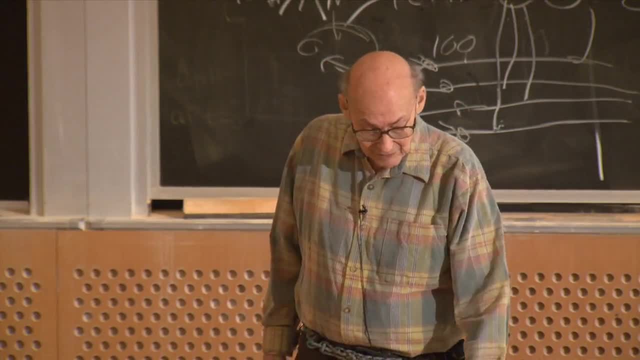 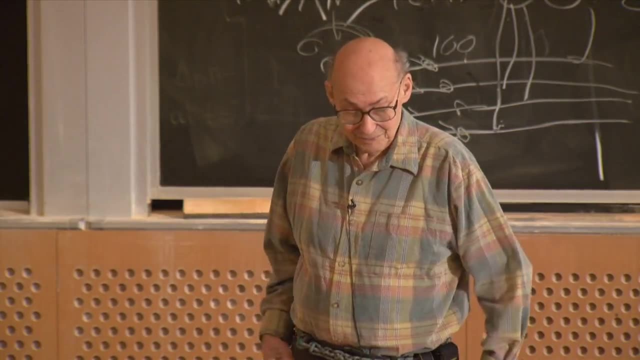 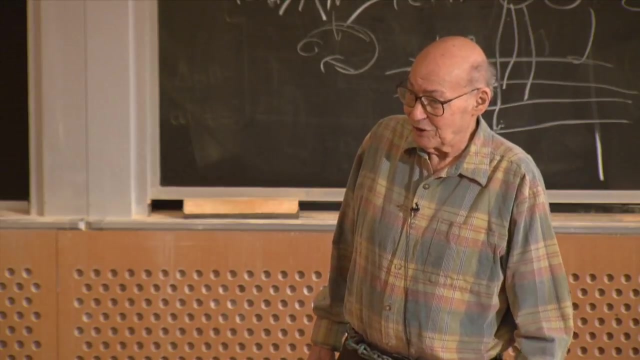 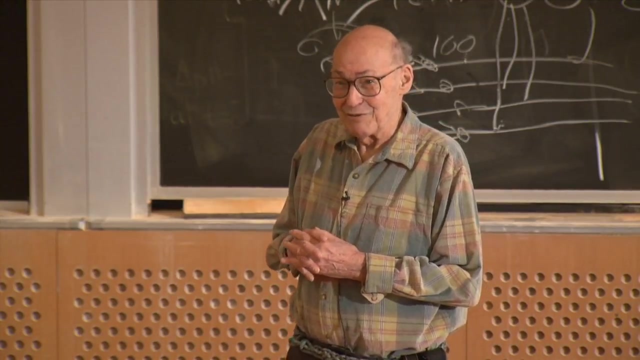 with other people And so he had been Freud's student or disciple for some years and then he went mystical And Freud went up the wall, because Jung was obviously very smart and imaginative. I'm trying to think if I've had a very good student who 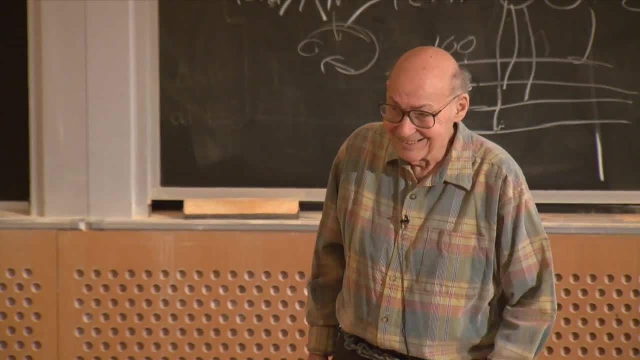 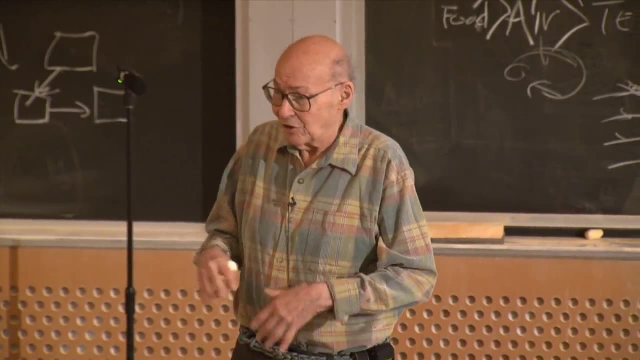 turned mystical, but one or two, but not like that. Anyway, that's a great question. And when I said things hang around in the amygdala for 20 minutes, that's not true. It's not true. It's not true. 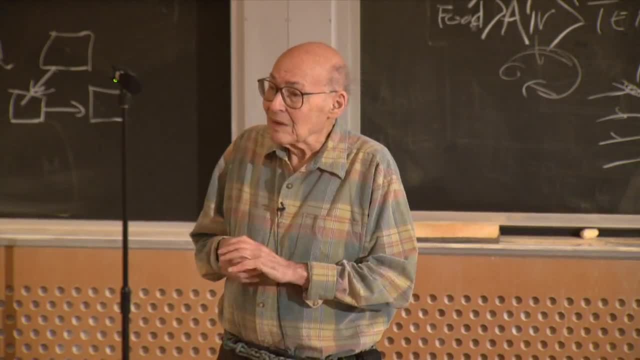 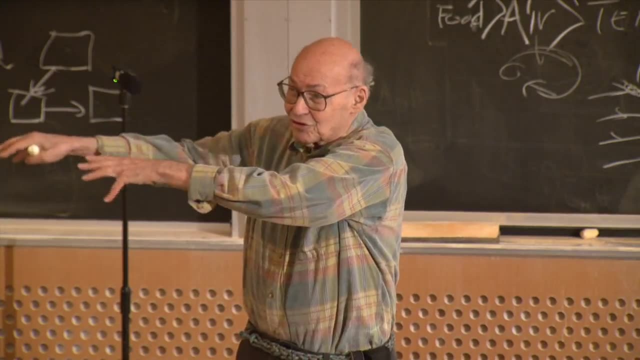 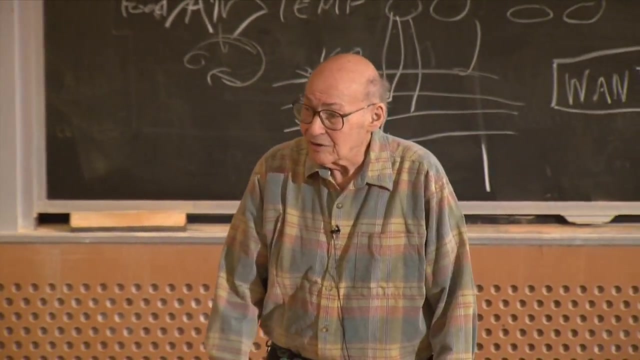 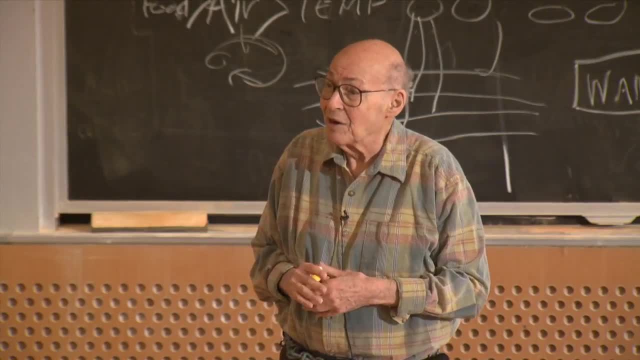 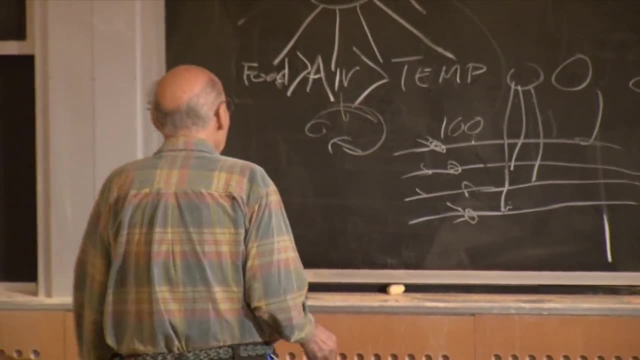 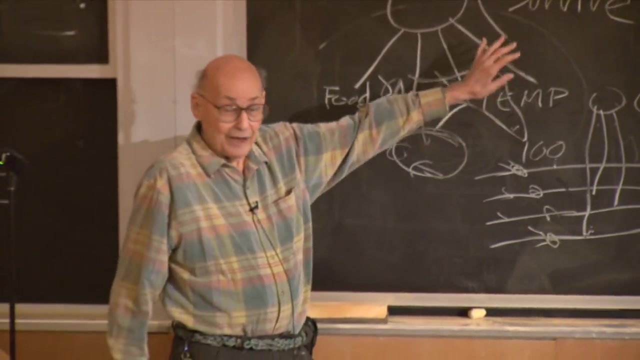 or to copy it in some way into the other parts of the brain. it must still be in the amygdala or somewhere. So, in fact, maybe, Maybe there's the amygdala and some other parts of the brain that haven't been identified that contain. 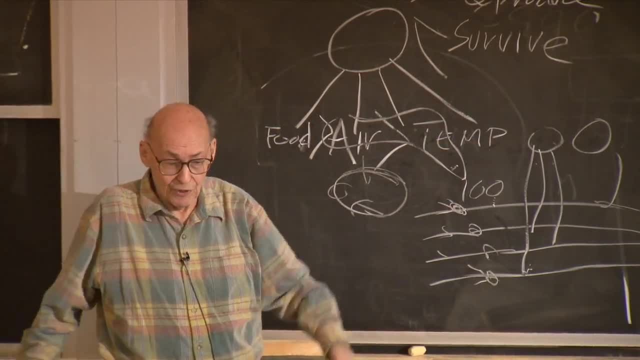 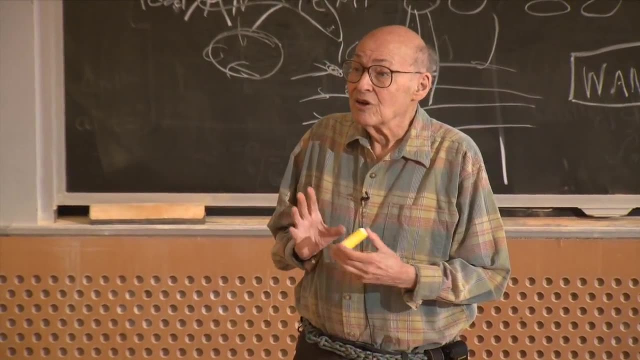 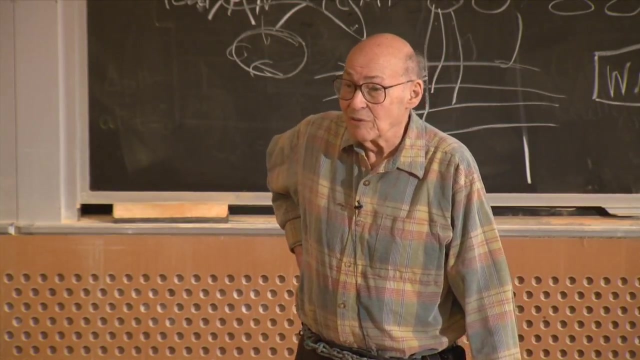 slightly different copies of the memories for a longer time, and so forth. So who knows where and how they work? Maybe the language centers remember paragraphs of things that you've heard or said for some time, and so forth. I don't think it's true. 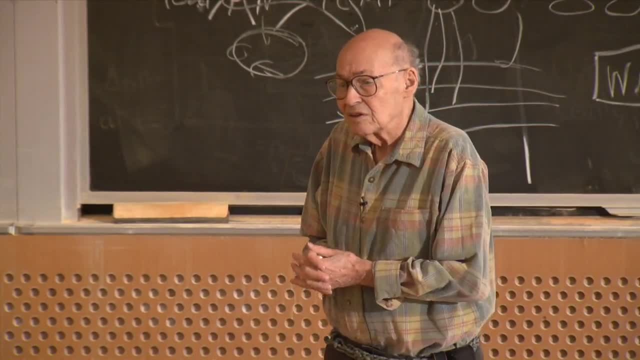 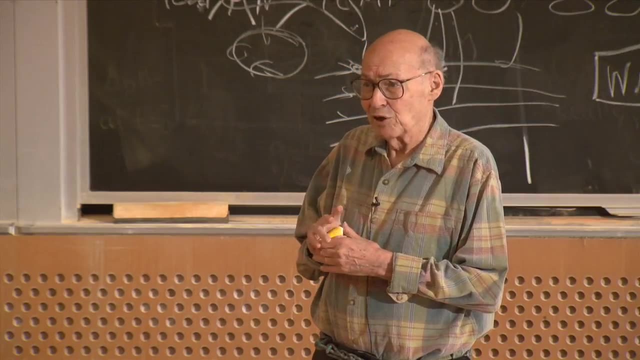 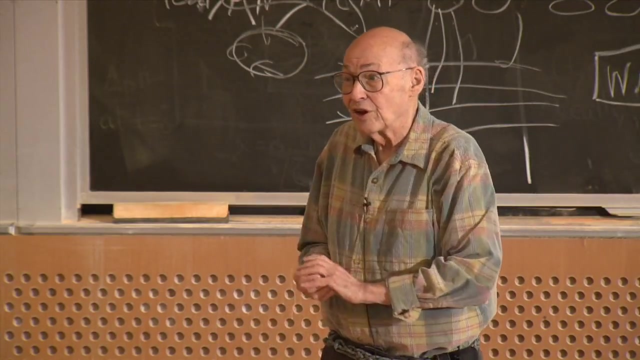 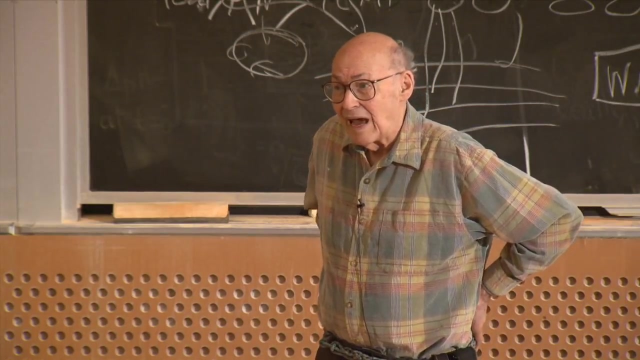 I don't think anybody really knows much about it. They're very sure about the amygdala, because injuring the amygdala or injecting Novocaine into a blood vessel that goes there has such a dramatic effect on you just can't remember anything for that short period of half hour or so. 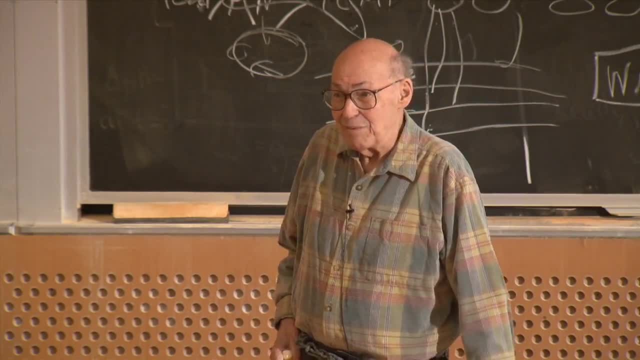 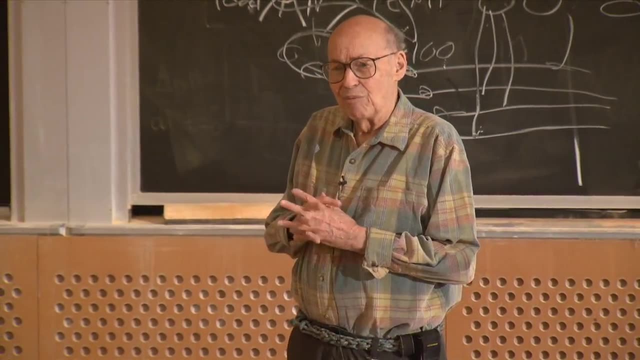 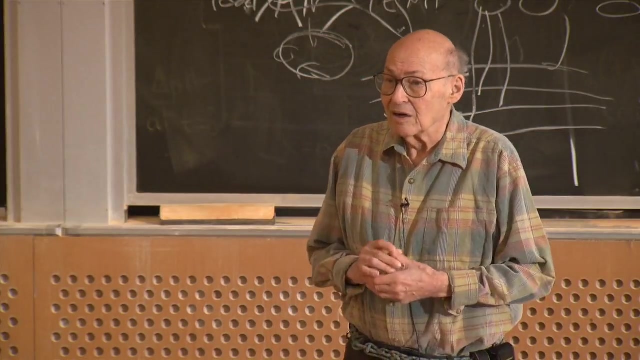 But there must be lots of other. Maybe memories are stored in 10 different ways, in 10 different parts of the brain. Who knows? One problem that I think I mentioned is that, although a great deal has been learned about the brain from modern scanning, 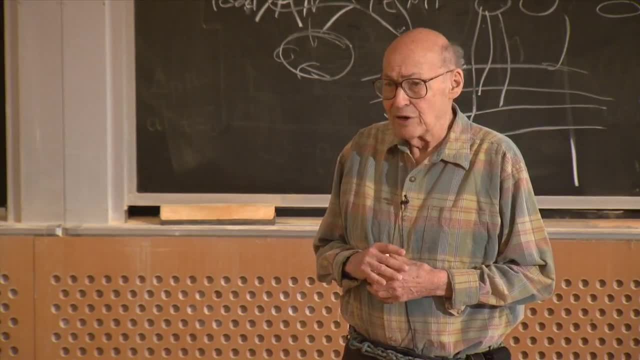 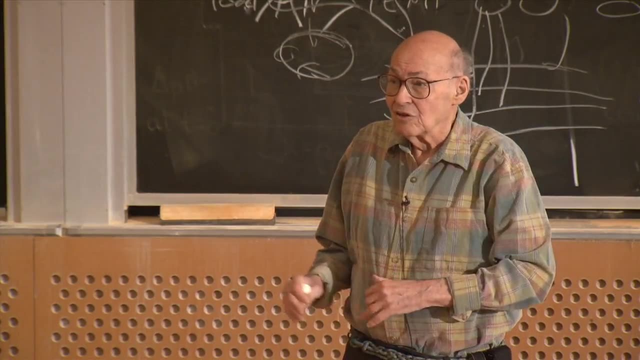 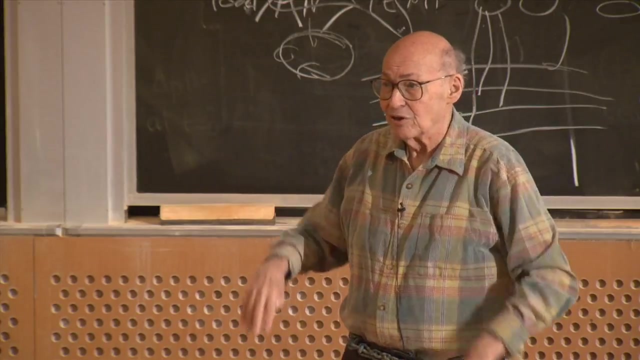 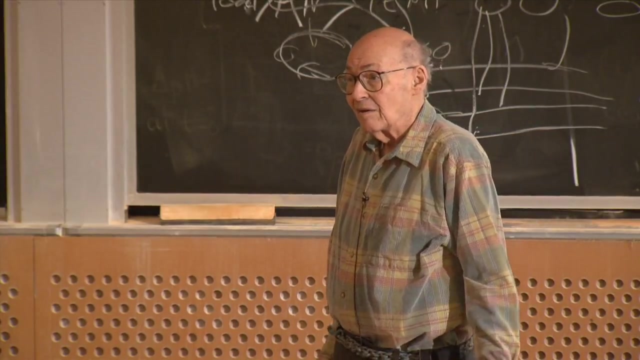 techniques. almost every result that people talk about is obtained by turning up the contrast so that most of the brain is dark And nerve centers that are highly active show up in your. You've all seen these pictures which show three or four places in the brain lighting up. 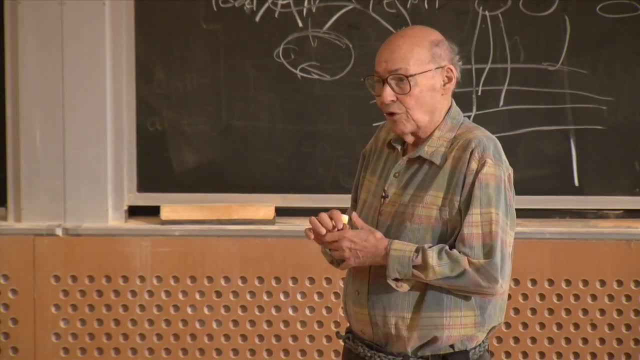 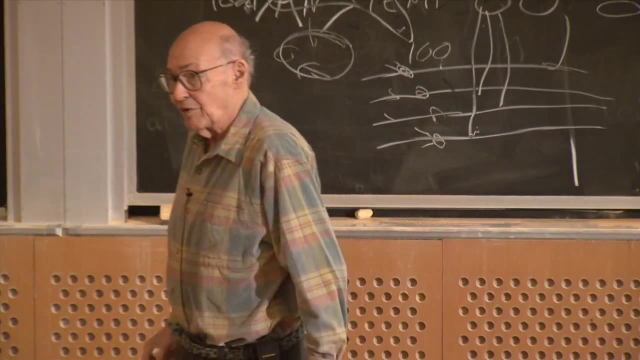 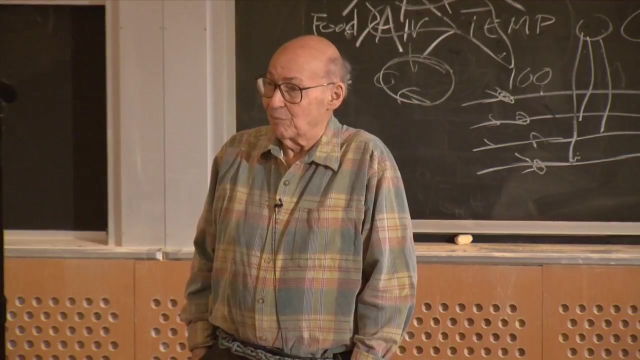 Well, there's a good chance that for any particular event, there might be 10 or 20 places that have just increased a little bit. And when they turn up the contrast, all that evidence is lost because those regions which are all black or whatever, 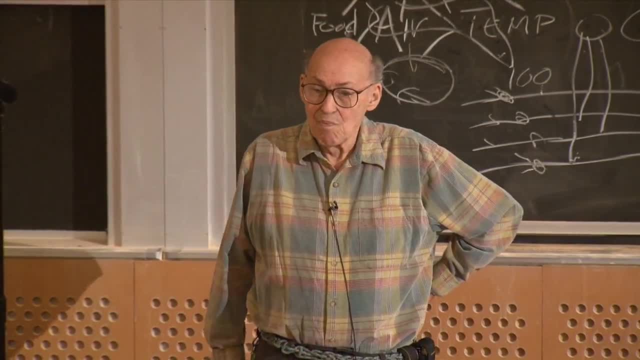 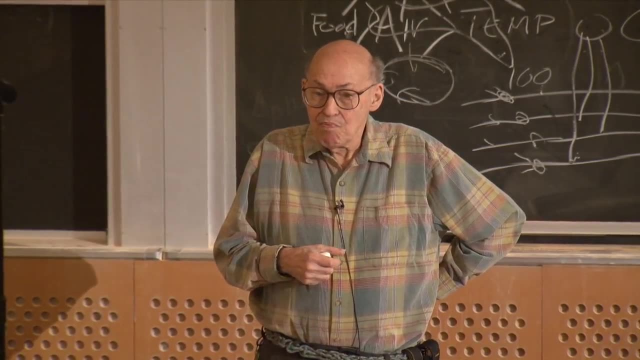 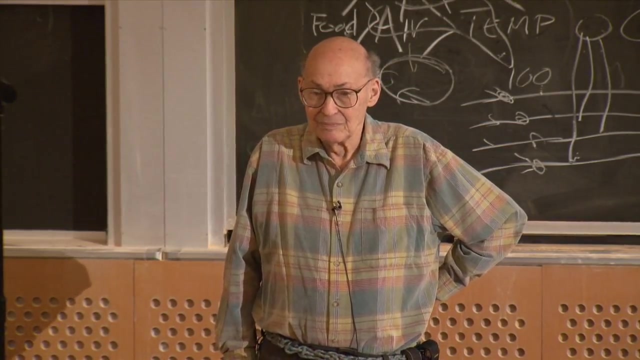 Anyway, Yeah, I'm not an expert on that, But I would go as far as to say that probably if they have a finding that where there are no specific areas, so you have a pretty uniform picture of the changes in metabolism, then you don't make theories. 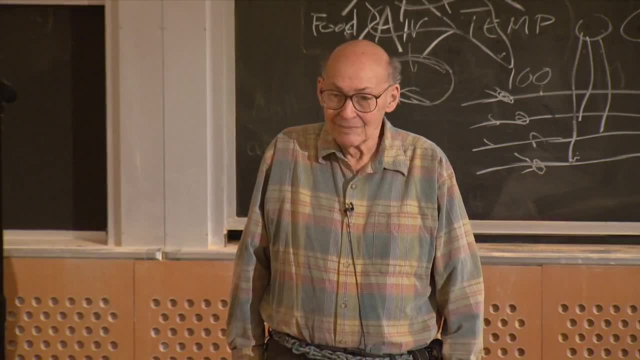 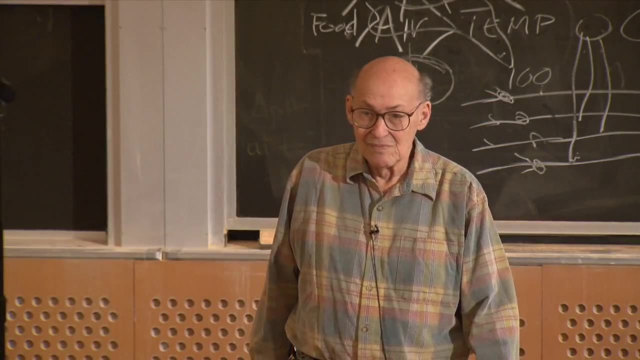 or you don't publish that result because you don't have any clear areas where the point that and then nobody knows that. OK, that particular thing was actually exciting to the whole of the brain. That's just a guess. Yeah, it could be that some things involve. 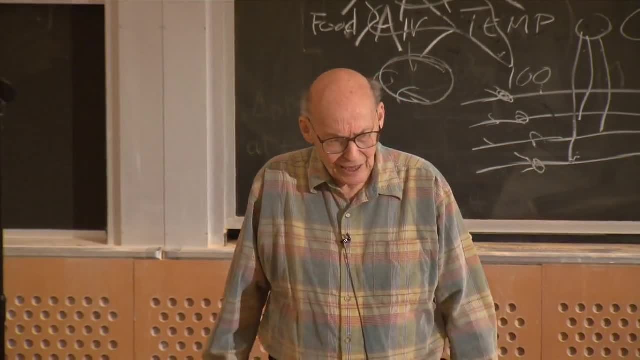 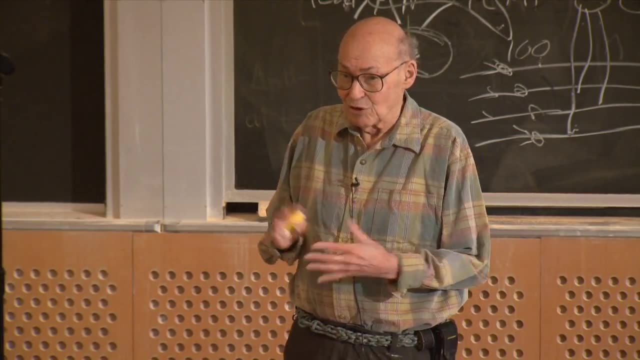 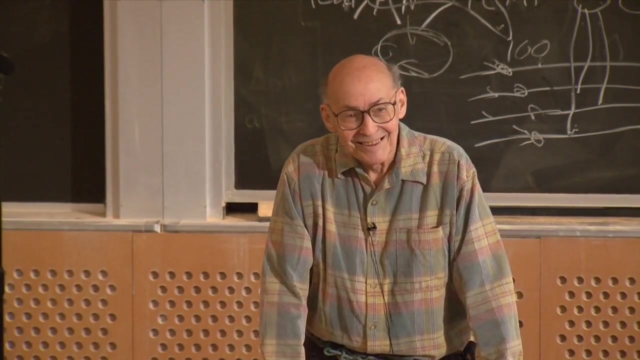 very large amounts of brain, But I'm inclined to doubt it. Probably you want to turn a lot of things off most of the time so they don't fill up with random garbage. Who knows? Yes, Just want to follow up on that. 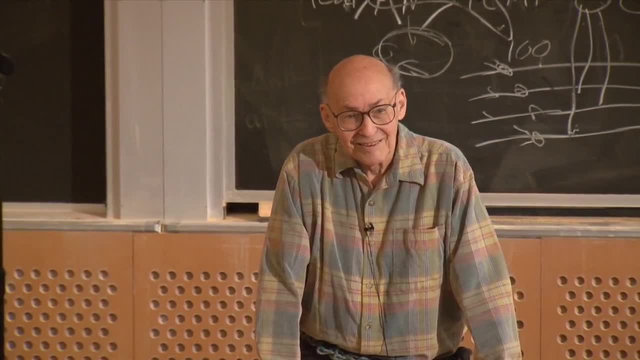 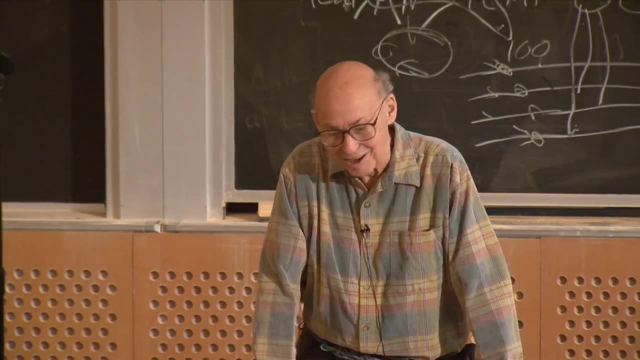 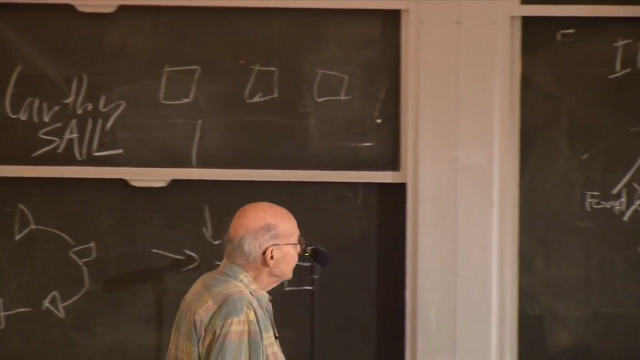 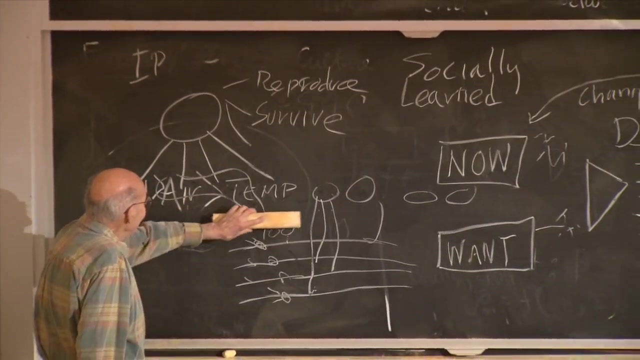 Why do you think that? Do you think that hierarchy of goals is naive? And what specific features of goals do you think that structure doesn't achieve? I didn't finish that, did I? She's asking. I started to say what's the hierarchy of goals? 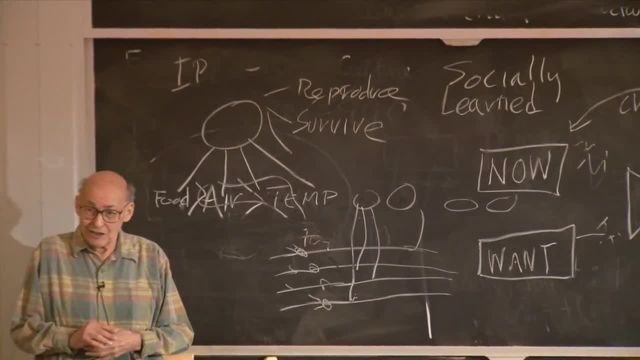 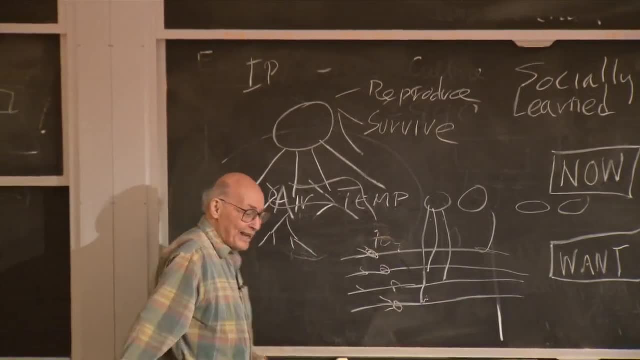 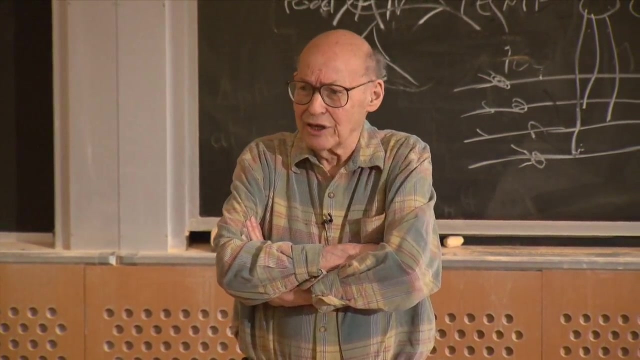 But it looks like I got stuck on the well-defined instinctive goals that you need to stay alive And I guess my answer is: I don't have any good theories of how you do that At any time when you're talking to somebody. 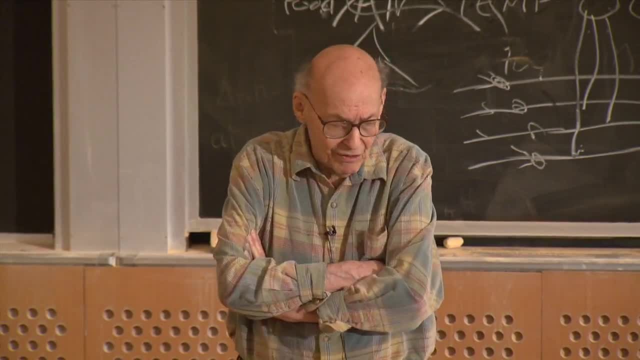 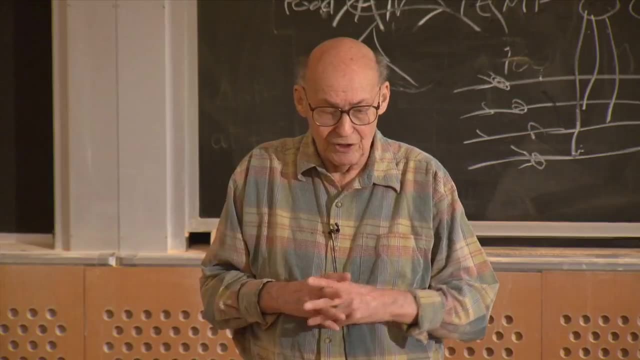 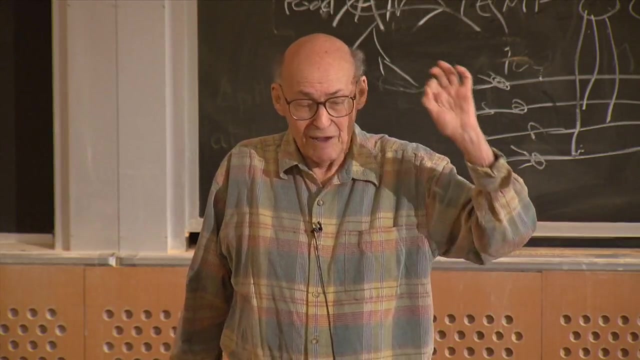 you usually have a couple of very clear goals like. I want to explain this. I want this other person to understand this. for this reason I'm having trouble. Maybe I have to get his or her attention by, and then you get a sub-goal of doing some social thing. 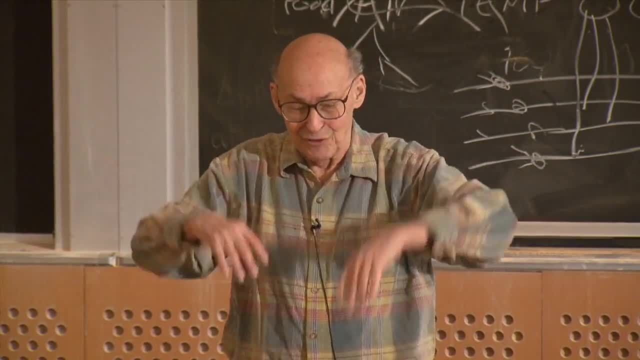 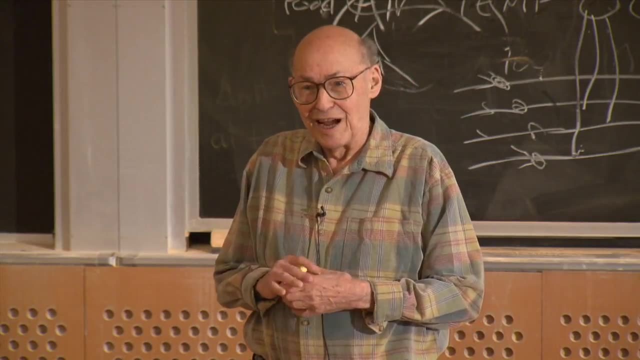 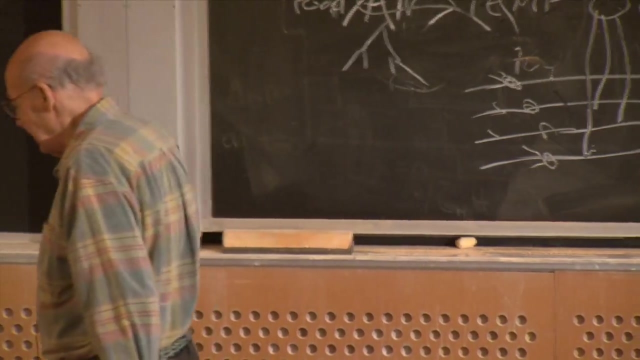 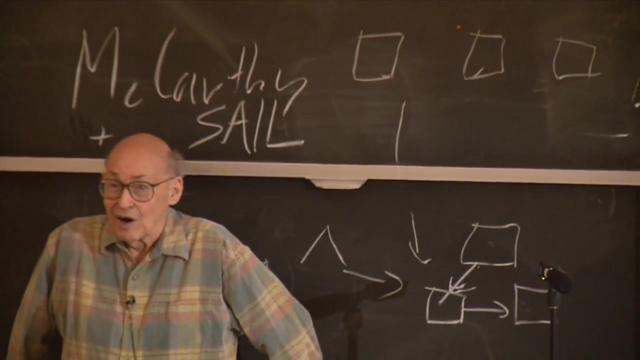 to convince them to listen to you and all sorts of things. But I just don't have a nice picture. When you're writing an AI program, you usually have goals and sub-goals in a very clear, clear arrangement, like the theorem-proving programs. 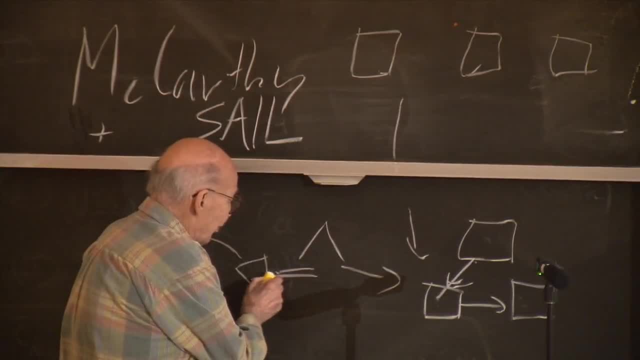 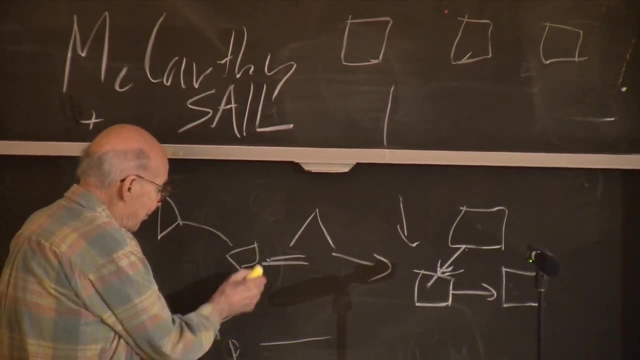 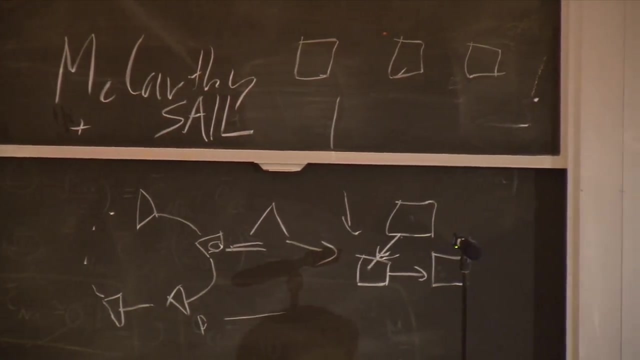 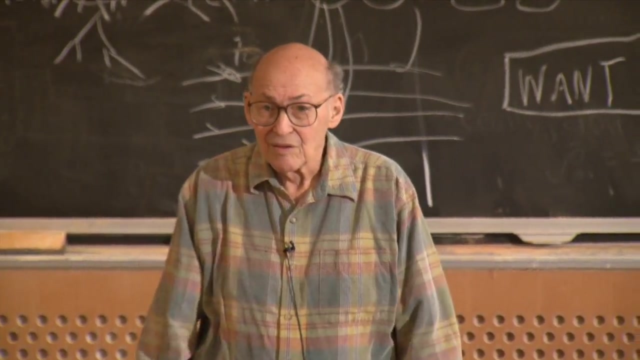 are wonderful because you've proved some kind of expression. but the particular theorem you are trying to prove has another condition which is different from this condition, And people have gone quite far in making models of um, something like theorem-proving, where the world is very simple. 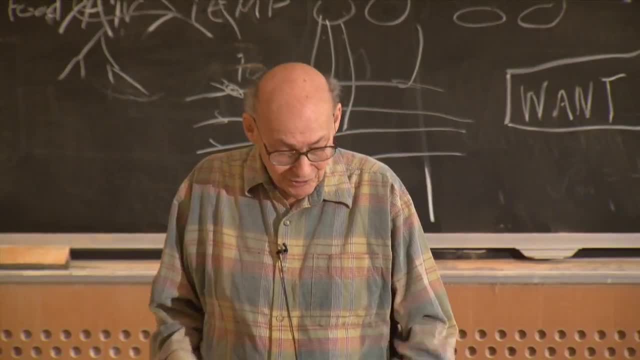 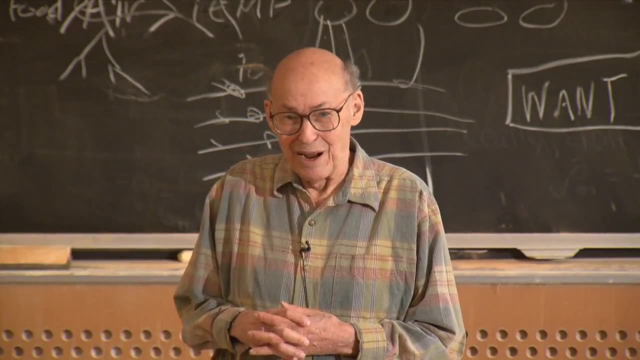 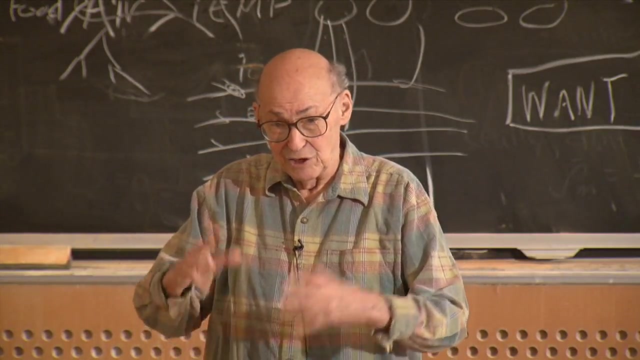 If you're proving something in geometry or group theory or a little fragment of mathematics, then there are only five or 10 assumptions hanging around, And so you could actually plan a little bit of exhaustive search to go three or four levels, And then you would do something like in a chess program of 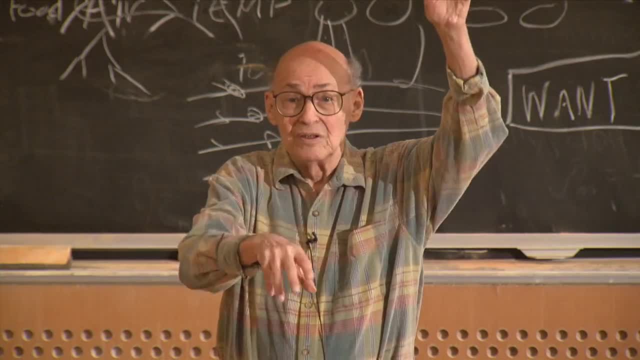 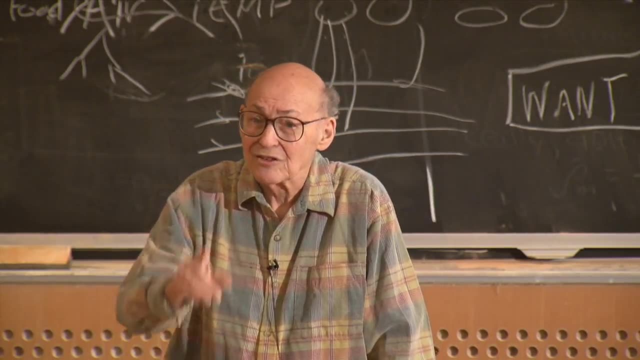 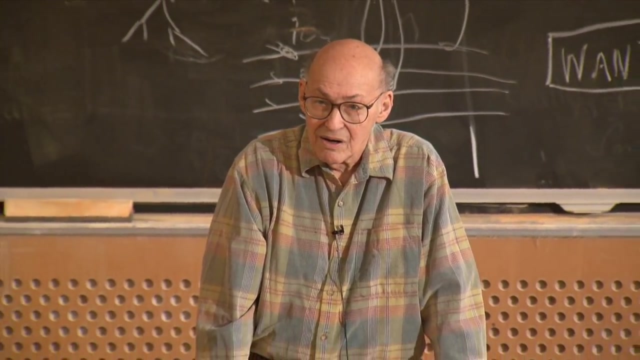 over time, discovering it never pays to explore a tree that has this feature because of whatever. Yes, Are goals relevant Like do we always have goals, or is it just like something like when I play chess, maybe I have a goal? 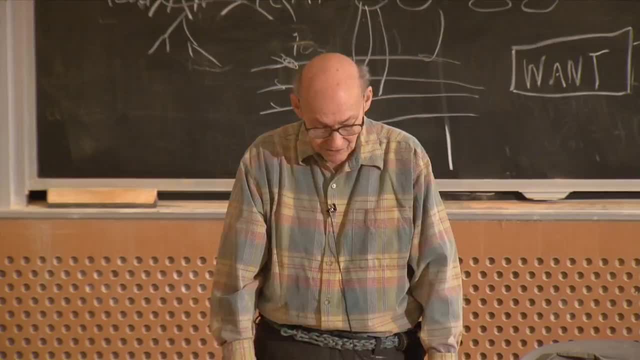 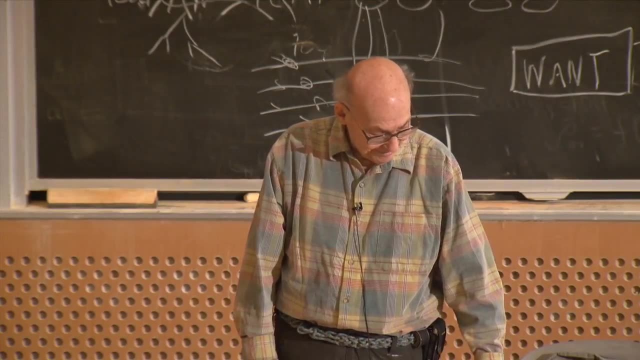 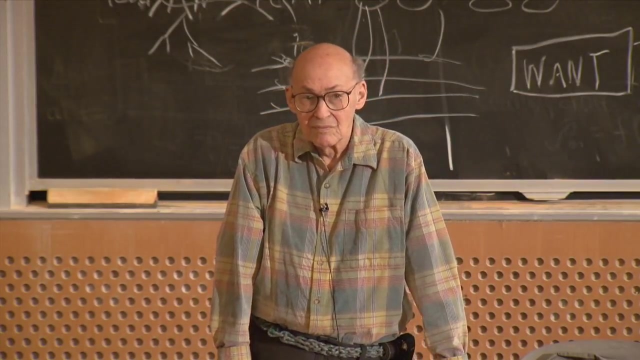 but why should I have a goal Like? why isn't that? like maybe I don't know- that goal of reproducing is greater At some points of my life? or like I don't know, why are goals important? 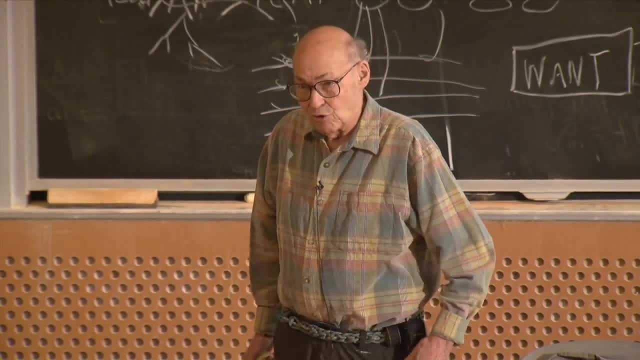 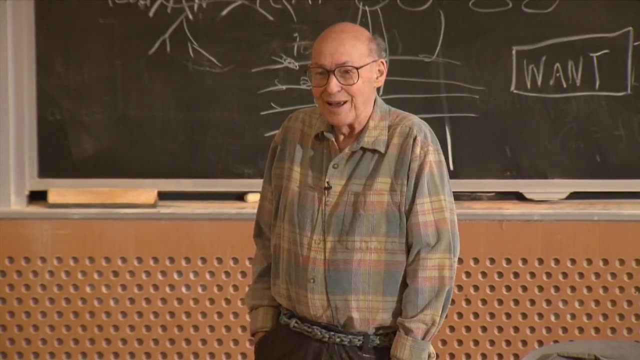 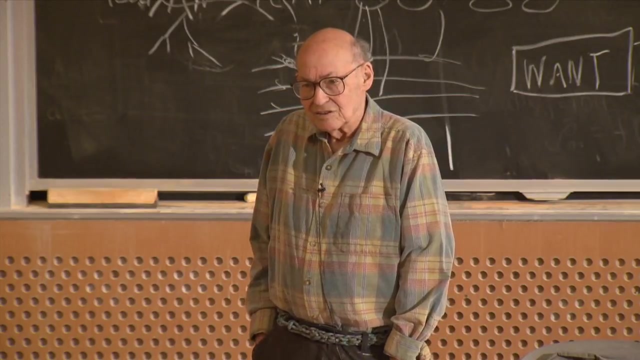 Well, the survival goals are important, because if you crossed a street without looking, you could do that about 20 times before you're dead. So why are there? uh, well, Just only the survival goals are important. Yeah, Yeah. 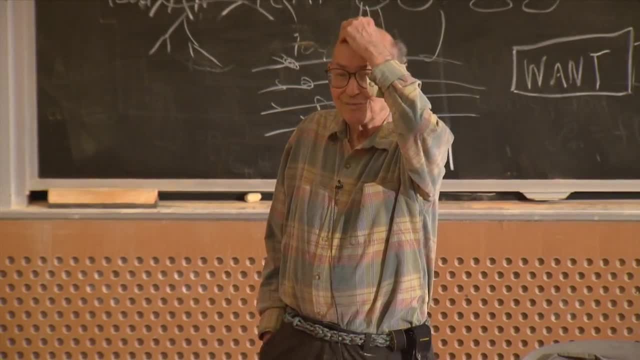 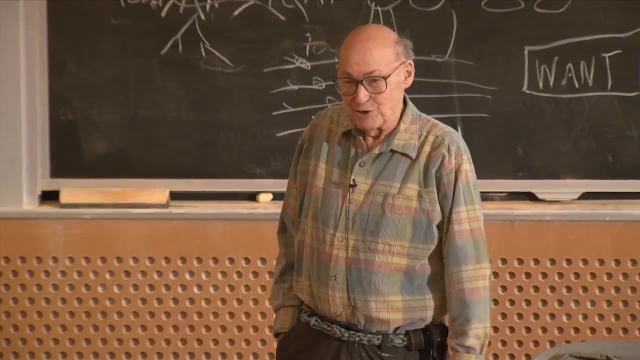 Yeah, Yeah, Yeah, Yeah, Yeah. Well, if you don't make a living, you'll starve. So now you have to. if you've committed yourself to being a mathematician, now you have to be a good mathematician, or else you'll. 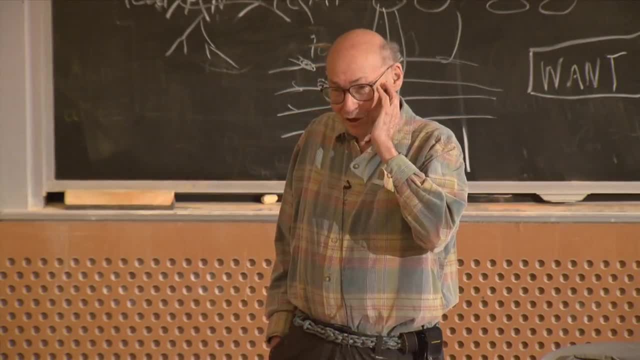 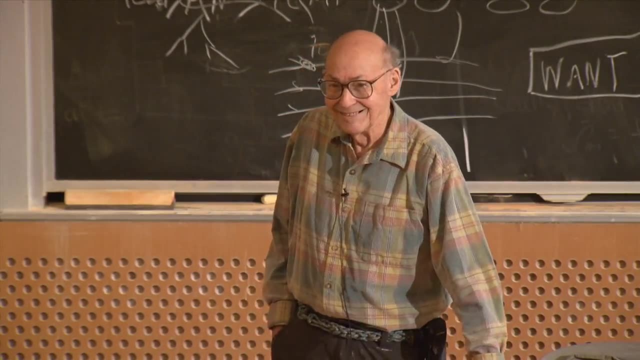 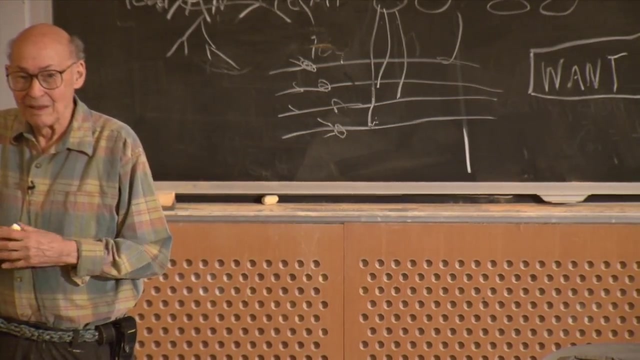 starve and so forth. I was a pretty good mathematician. only, my goal is: I had to be the best mathematician, so I quit. You don't want to have a goal you can't achieve? Yeah, but is that part of the intelligence play? 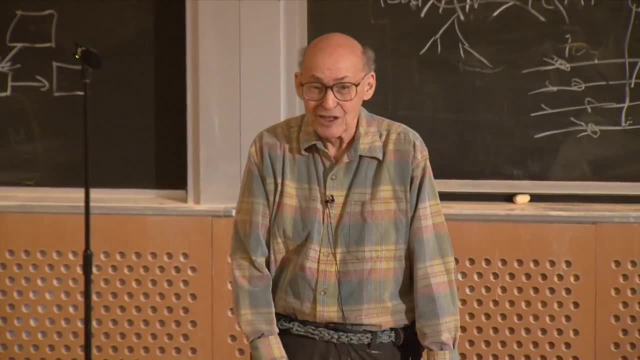 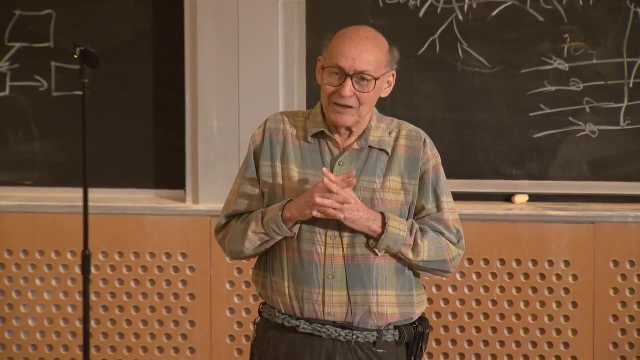 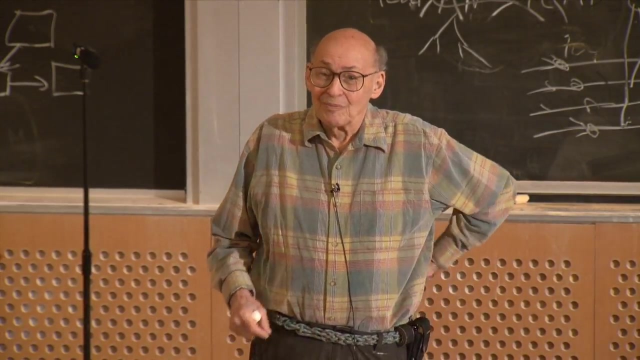 Well, a lot of people do have one, So it eats up a lot of their time and they're wasting it. I'm not sure what the question is. How do you make a? I think the feature of humans is that there's sort of general purpose. 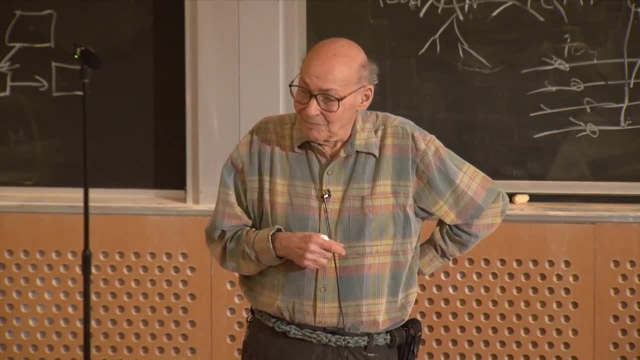 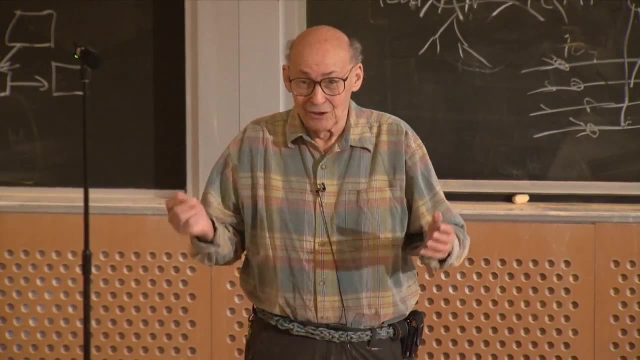 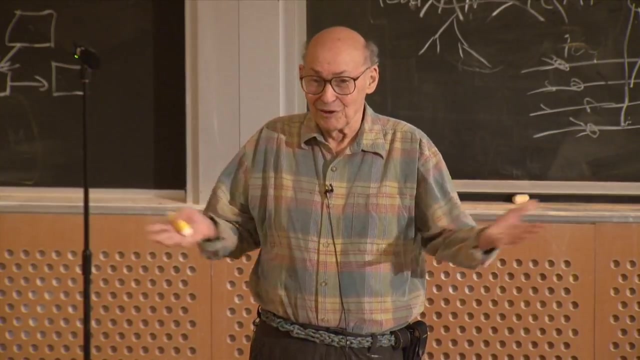 So there are a lot of things people do which are bad things to do. You can't justify them. You could think of people as part of a huge search process And as a species or a genetic system. it pays to have a few crazy ones every now and then. 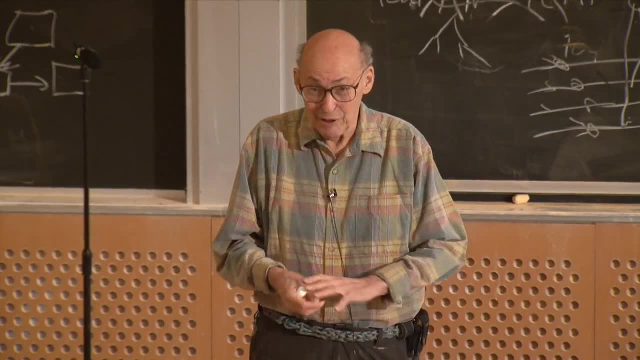 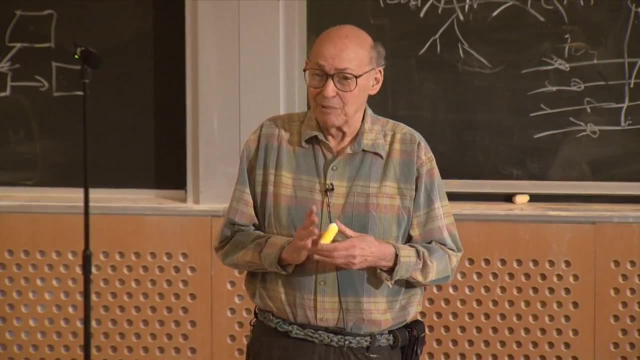 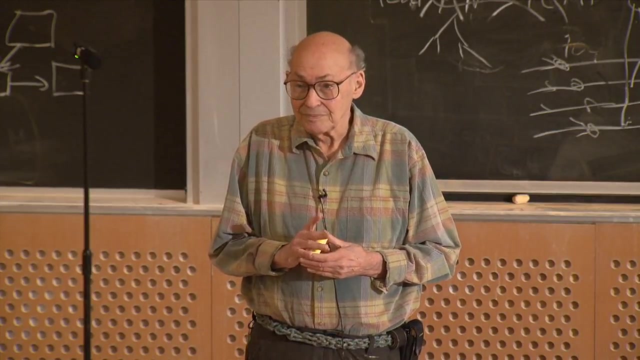 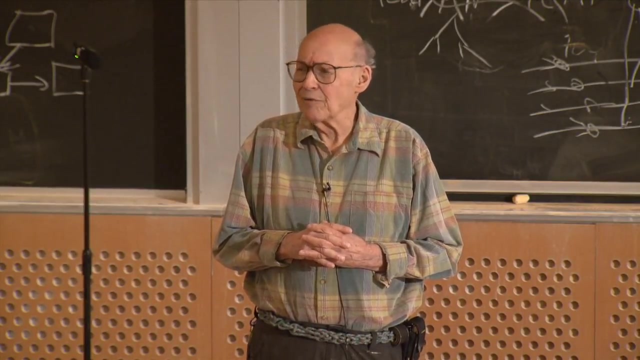 because if the environment suddenly changes, maybe they'll be the only ones who survive. William Calvin's question: how come people evolved intelligence so rapidly in 5 million years? That's a good question, And he attributes it partly to 10,, 5 or how many periods. 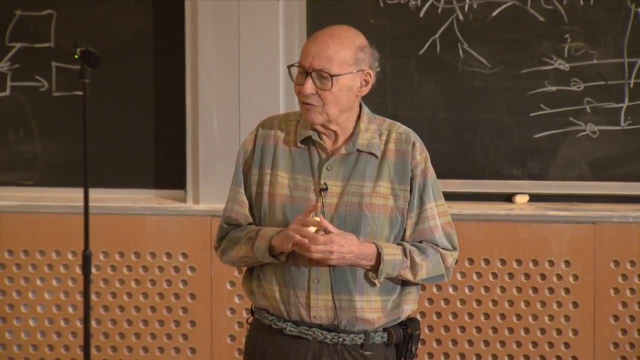 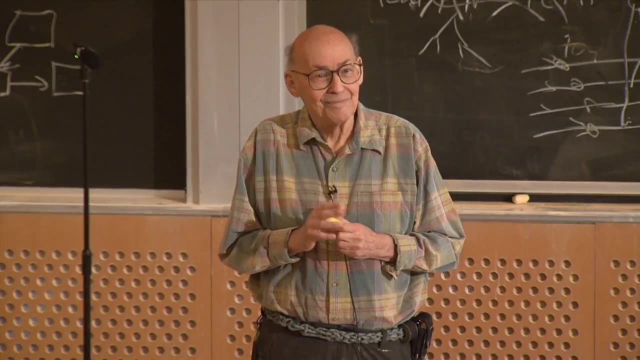 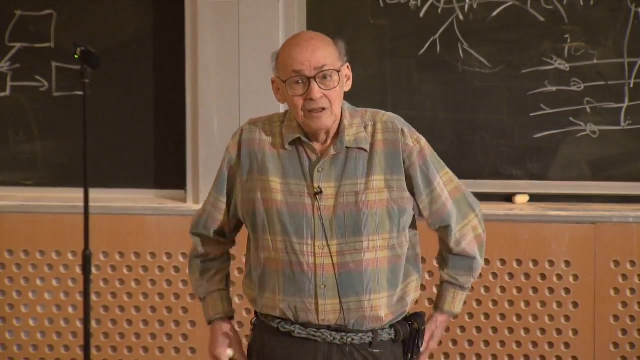 of global cooling were there. It's about six or seven ice ages in the last. Anybody know the history of the Earth. Anyway, some evidence use- at least used to be. I haven't paid any attention- is that the Space nozzle is wheeling water on footprints. I don't really know much about that So I don't have complete problems of that. Senators said: if you like, you'll be able to have one in 5 million years. But that doesn't have to be taught and it won't. 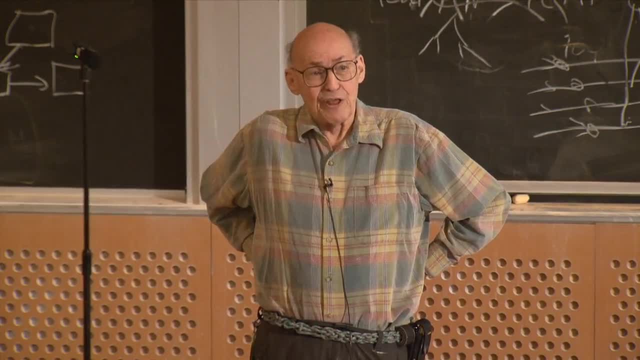 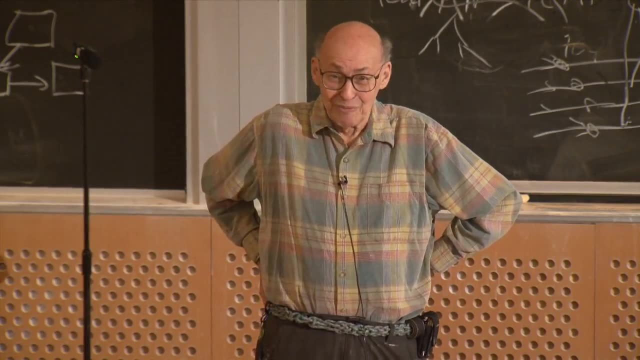 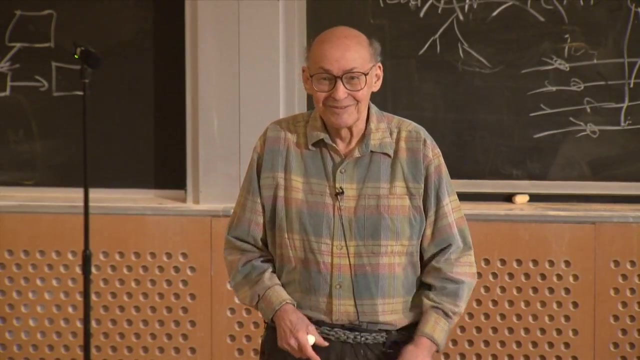 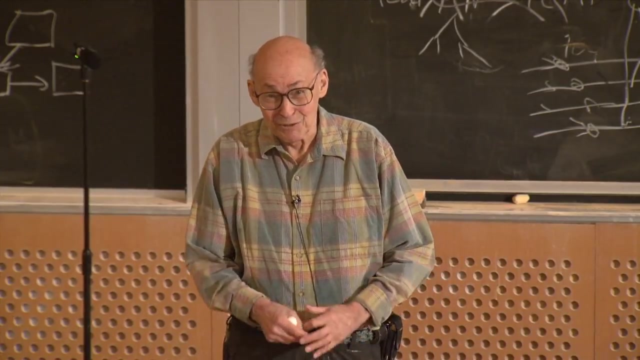 human populations got down to maybe just tens of thousands several times in the last million years, And so only the really different ones managed to pull through. Might be the ones who had all sorts of useless abilities. Yes, So you're talking about learning MARVIN MINSKY- The ones who ate the others which 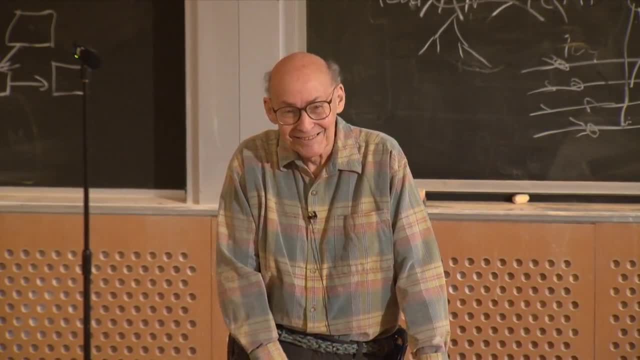 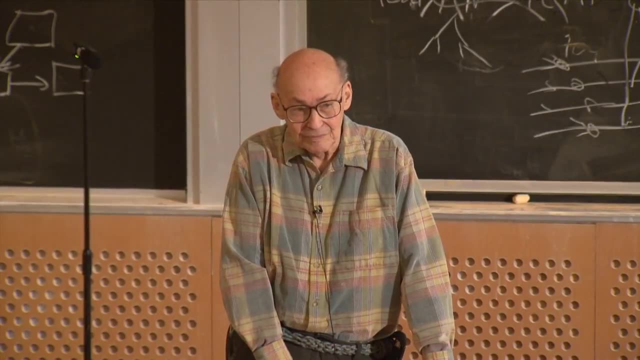 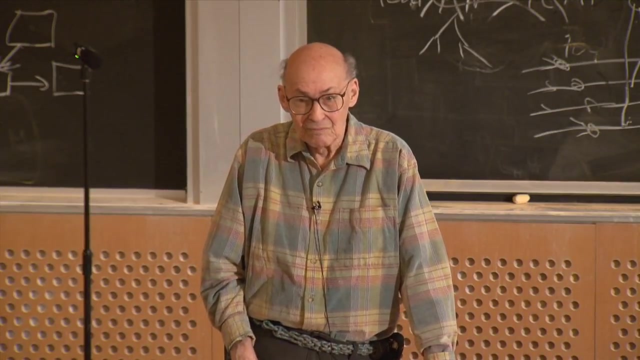 would have been punished. before that Go ahead, You were talking about representing the K-lines and everything like having some lines and then activating some of these features. So, in the case of learning, would we change some of these connections? And if this is the case, how would this? 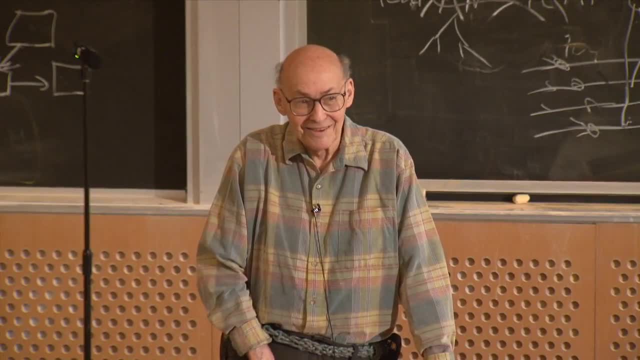 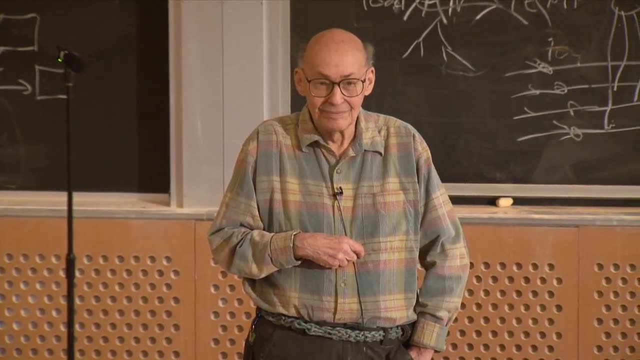 affect the higher-order objects like frames and everything. If we change something that's really the low representation, will this affect a lot? Wouldn't the whole system break because some sub-procedure is going to be able to return from it? MARVIN MINSKY- That's great. 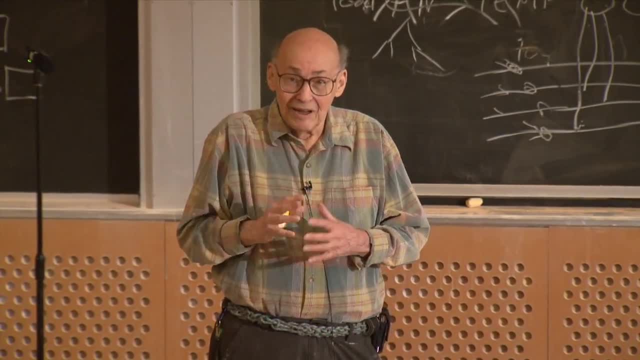 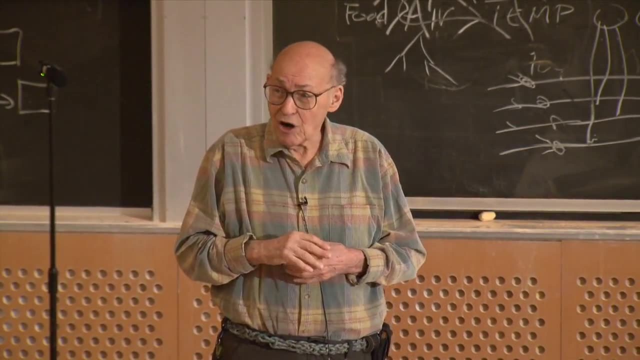 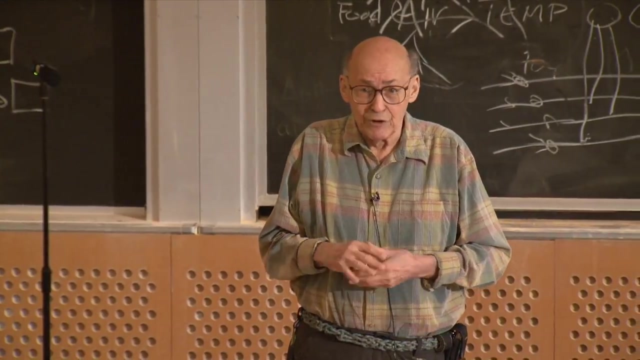 That's another question I can't begin to answer, Namely when you learn something- let's take the extreme form- Do you start a new representation or you modify an old one? OK, that's a choice. If you modify an old one, can you do that without losing? 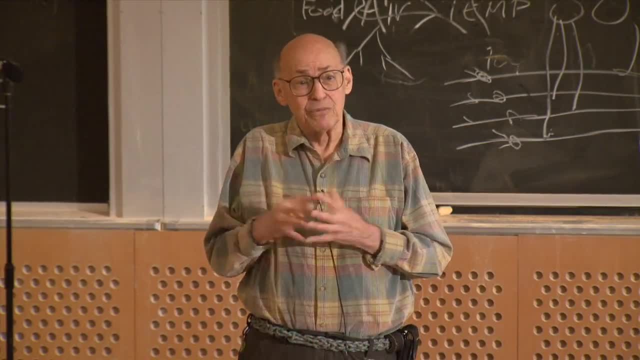 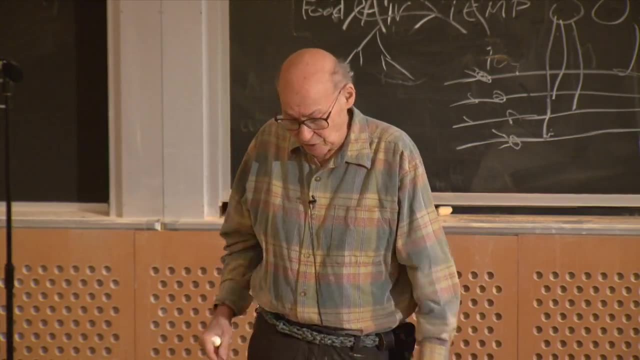 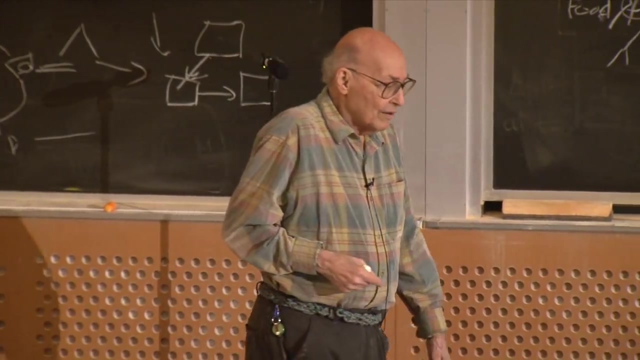 the previous version. So, for example, if I grow up- MARVIN MINSKY- If I grow up monolingually, which I did, so I learned English. and then I can't remember why, but for some reason, around fourth grade somebody tried to teach. 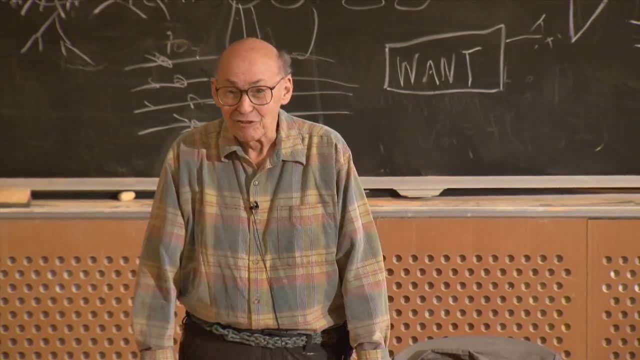 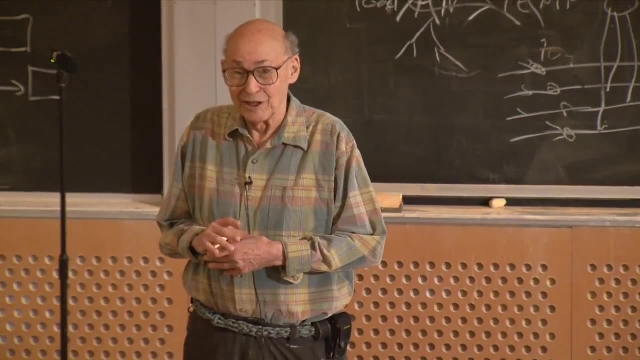 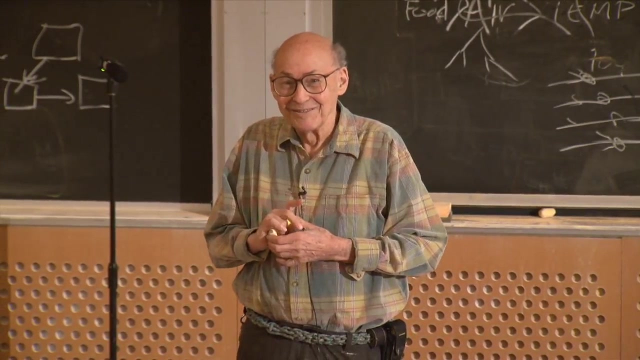 some teacher tried to teach us German, And so for each German word, I tried very hard to find the equivalent English word. And OK, MARVIN MINSKY- Figure out how to move your mouth so that it comes out German, which actually for many words. 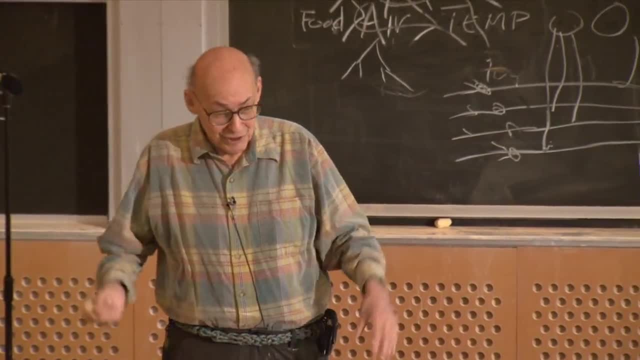 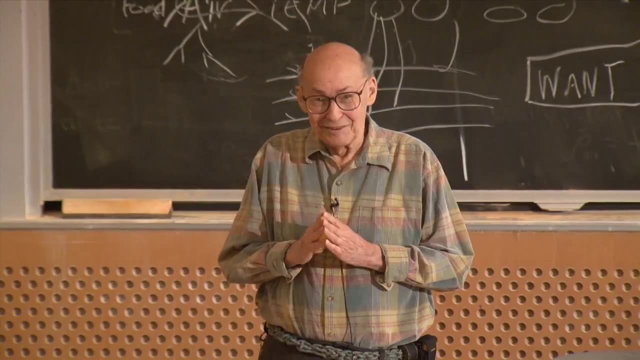 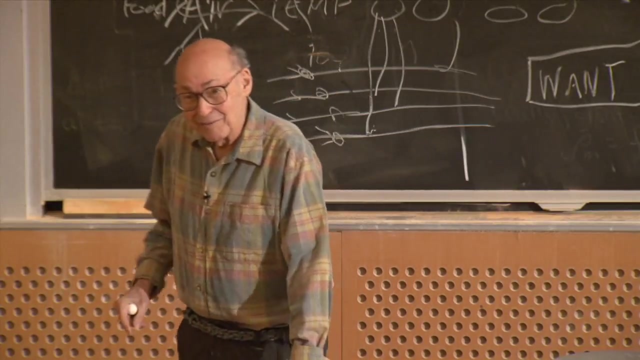 works fine, because English is a mixture of German and other things, And for many words it doesn't. So that was a bad idea, And if I had gotten very good at it, I could have lost some English. Anyway, that's a great set of questions. 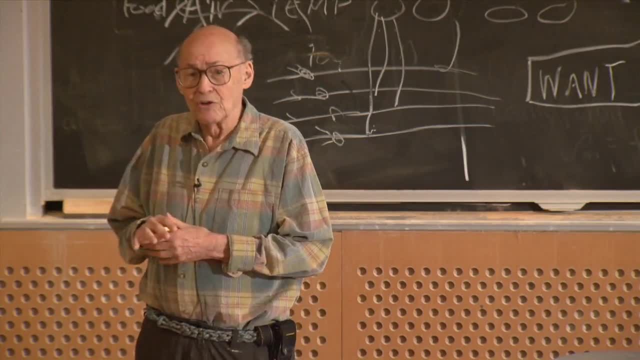 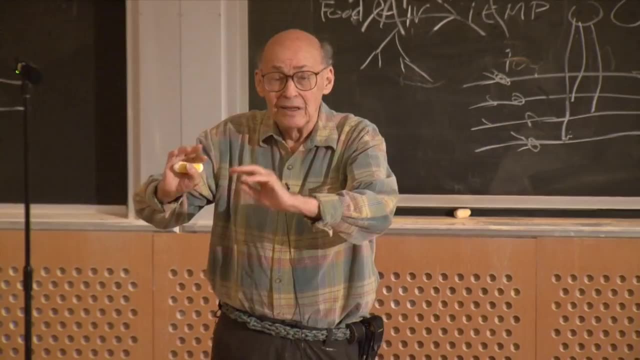 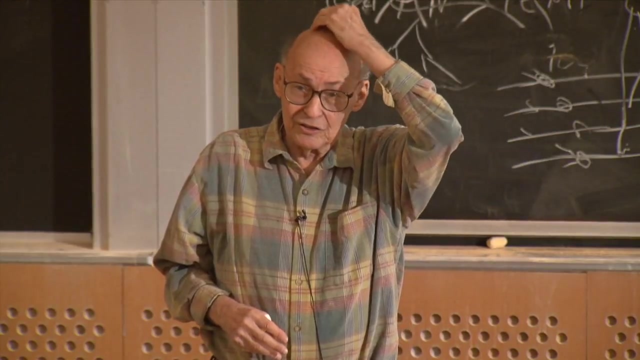 When do you make new? MARVIN MINSKY- Make new memories. When do you modify old ones? And the hard one is: if you can't modify an old one, how do you make a copy? that's different. And there's a section called in Society of Mind. 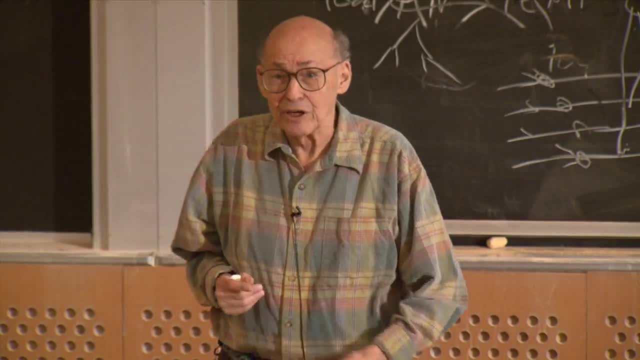 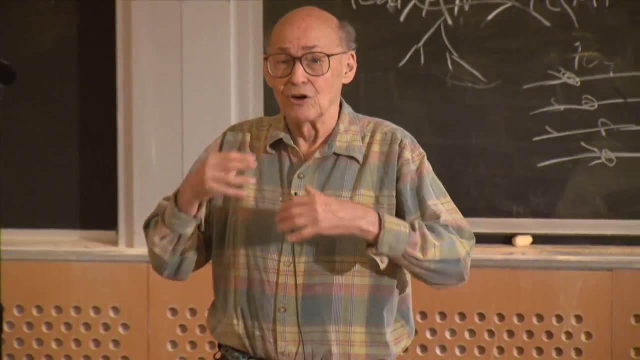 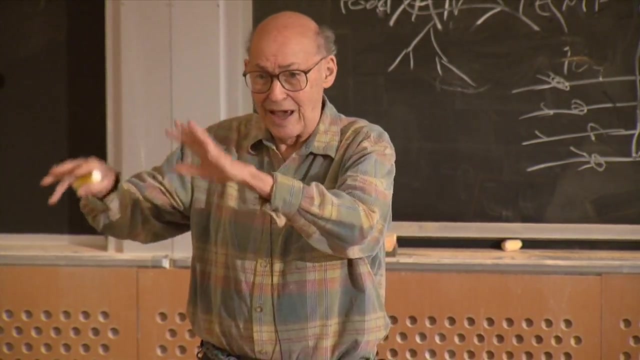 about how we do that in language, by paraphrasing what someone said, Or MARVIN MINSKY- You say something in your own head and you misunderstand it. I'm doing that all the time. I say such and such is a this or that. 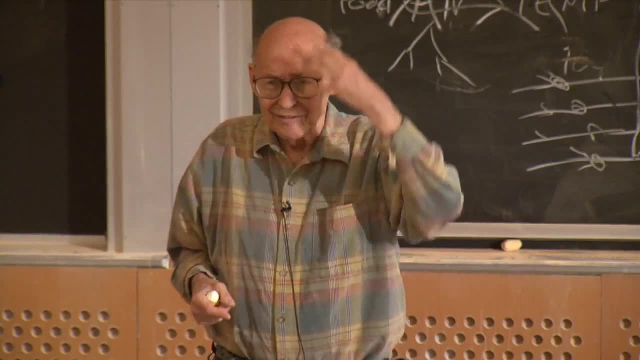 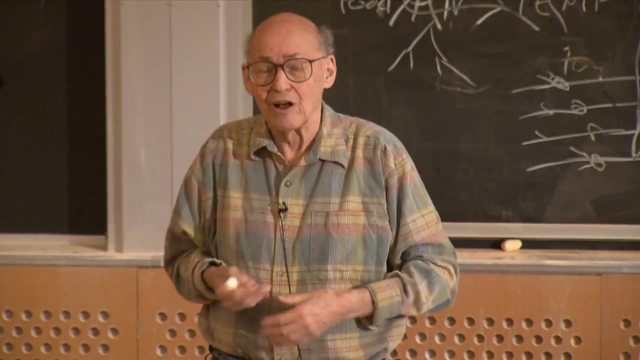 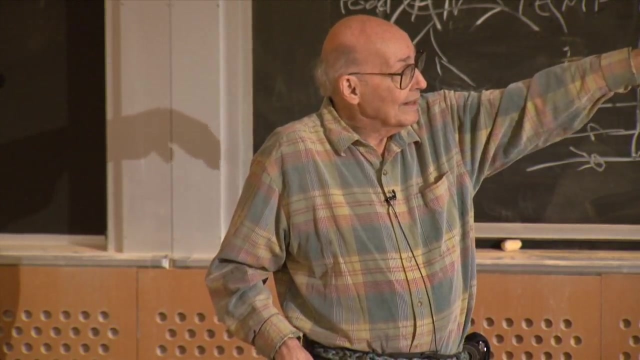 And then it's as though somebody else had said that and I have something. No, that's wrong. He meant this. So when you're talking to yourself, you're actually converting some mysterious inarticulate representation to speech, And then you're running it through your brain. 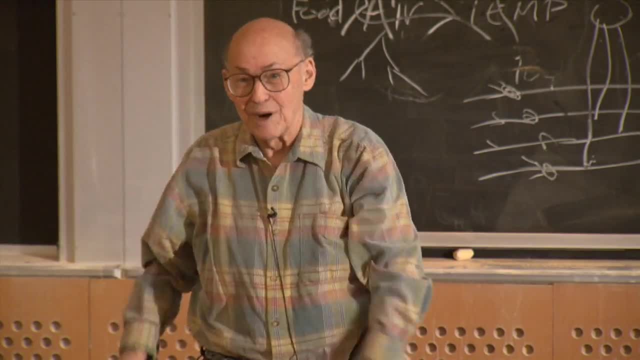 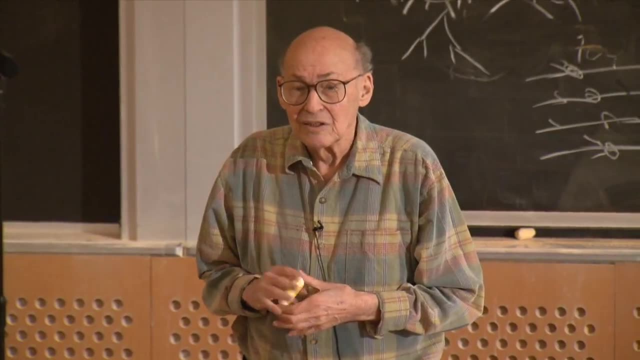 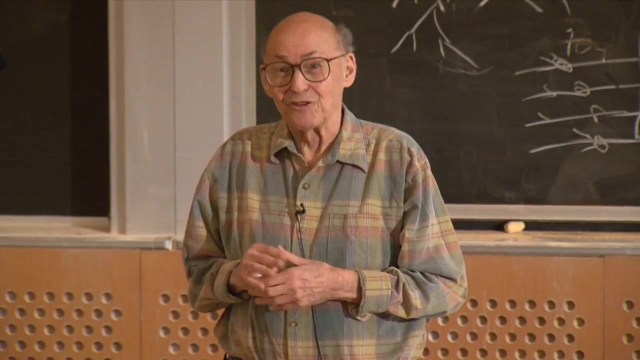 and listening to it and converting the speech back to a new representation. So I think the wonderful thing about language is it's not just for expressing. It may be. how come the only animal that thinks the way we do is the only animal that talks the way we do? 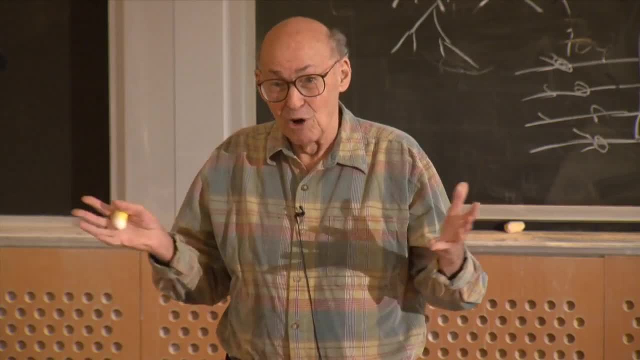 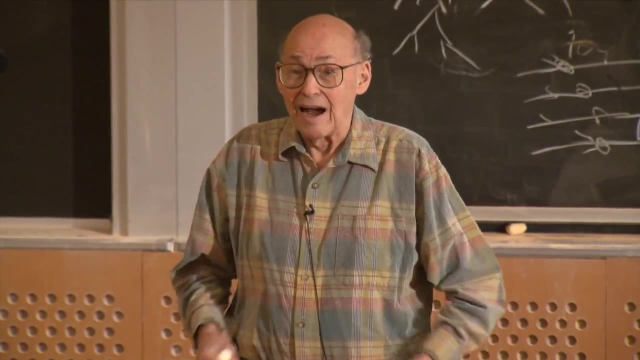 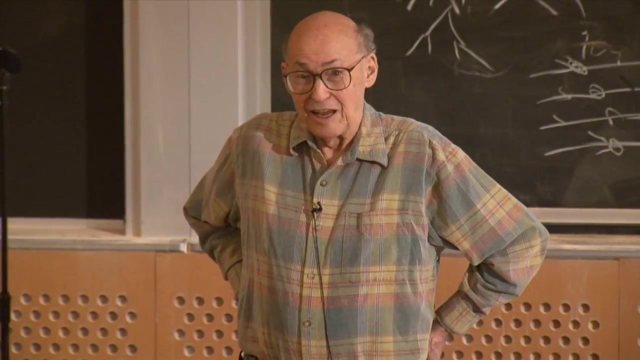 Who knows, Maybe whales? MARVIN MINSKY- Yeah, Yeah, But nobody has decoded them to do something like that. But that's a question: How do you copy a memory to make a new version? And the answer is: you can ask anyone. 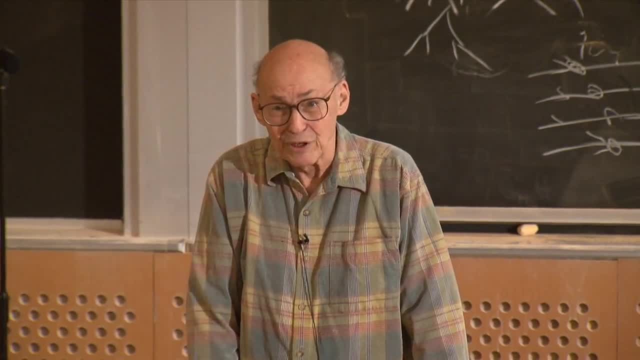 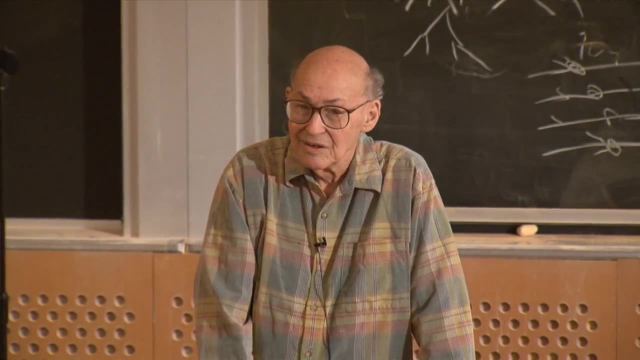 and they'll say: I don't know, Why aren't there five theories of that? Yeah, I don't know if that's true, but I believe there is a sort of objective map between words in language Like, for example: 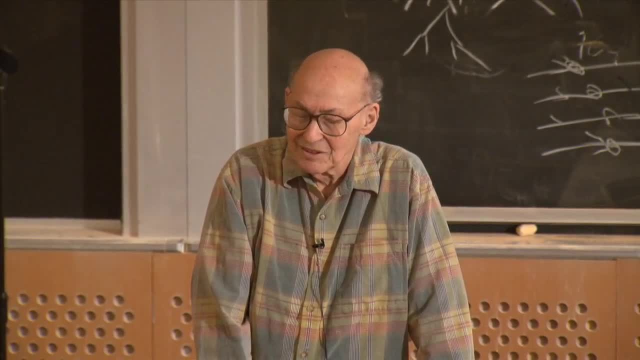 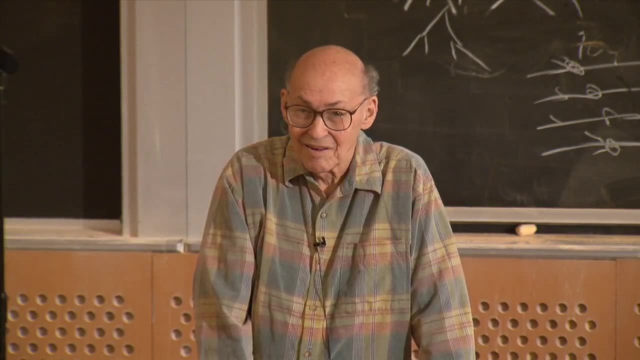 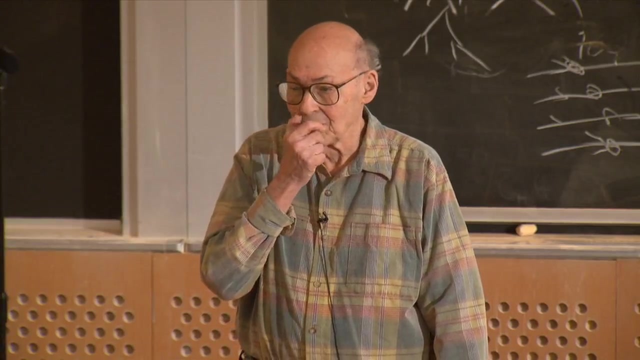 So, for example, if I have a table, I say like in Portuguese, And there's a sort of objective map, even for colors, which is sort of weird because you're kind of dividing all the colors into chunks of colors. 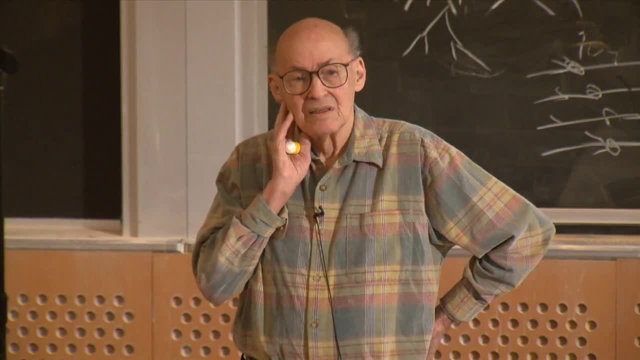 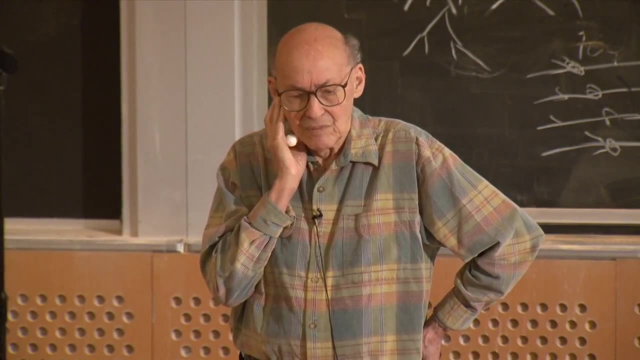 And even, I believe, for words, languages that were not formed, like MARVIN MINSKY- Oh yeah, With the same ancestry, I don't know. For me, it seems that there's some sort of objective map between words. 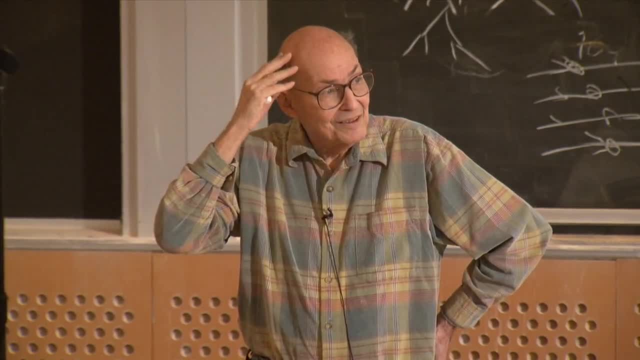 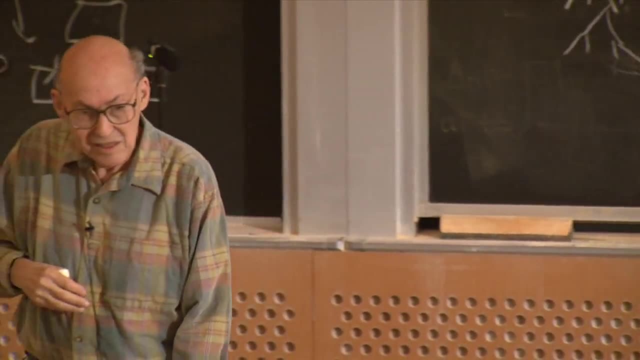 MARVIN MINSKY- Well, there are certain things that are just sort of naturally more useful to talk about, And so a lot of languages tend to have words for the same thing. Like languages will have a word. that means table, But if there's some culture that doesn't have tables, 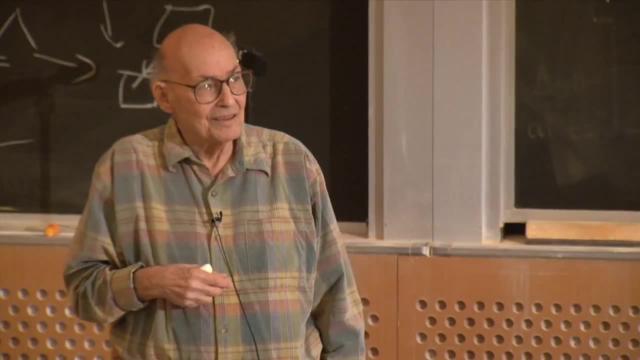 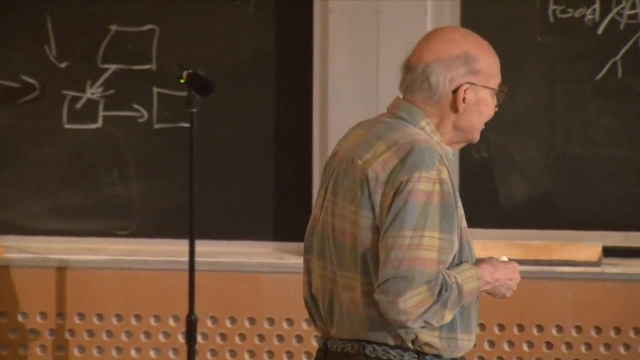 then they probably wouldn't have any single word for table. And regarding the colors thing, there have actually been some interesting studies done on that, Like they've done color naming surveys with lots of writers in the world, And it turns out that different languages partition the color. 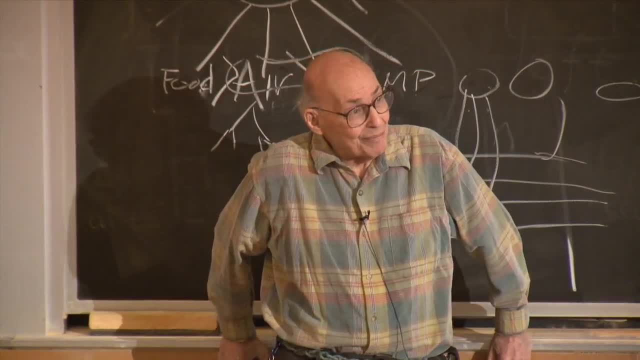 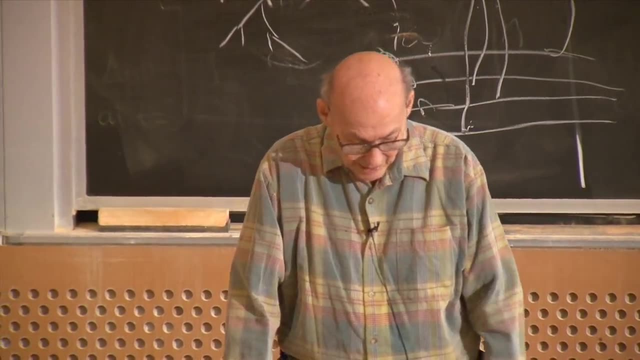 space differently. MARVIN MINSKY- I was just going to ask if anybody knows They tend to do it similarly- is using it for the way that people perceive colors, The way that they divide up the space based on the number of words that they have, is actually? 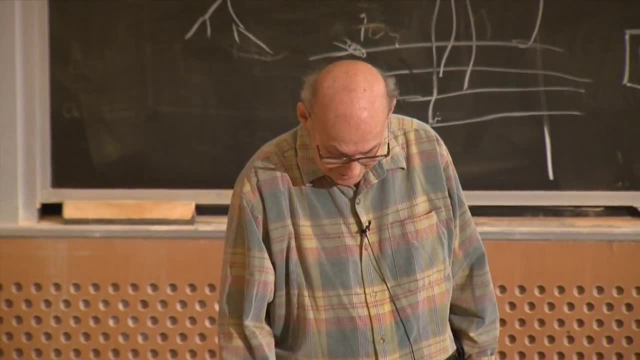 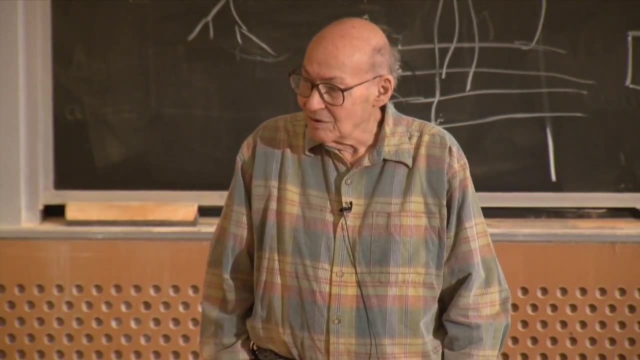 maximizing the similarity of things with the same name and the difference between things with the same name. MARVIN MINSKY- Yes, Like Dara Floroditsky did some of the interesting studies on that. MARVIN MINSKY- Right. 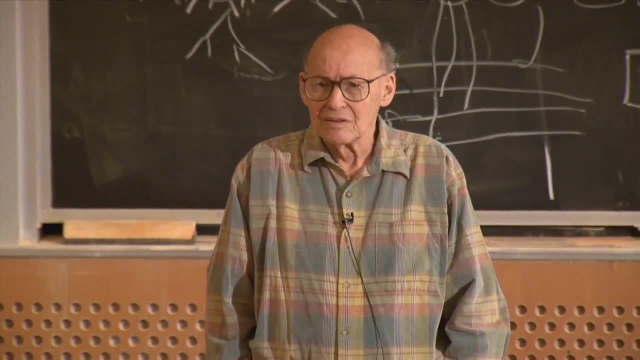 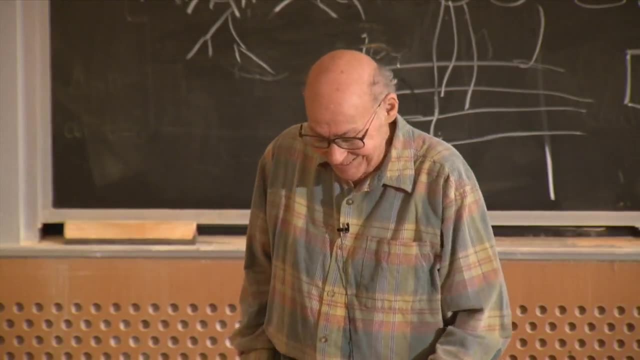 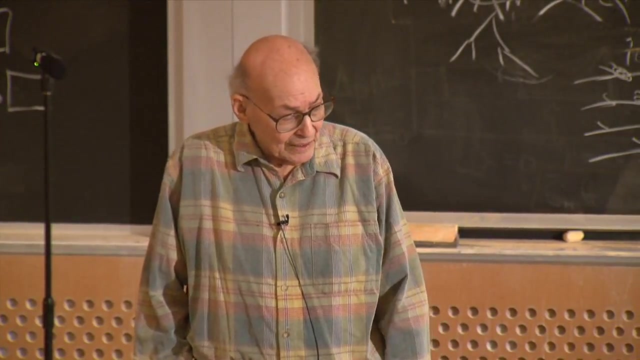 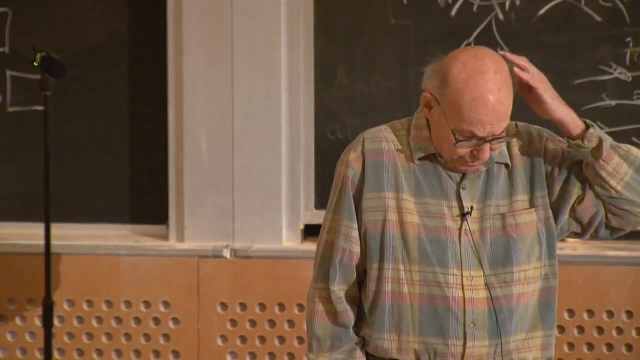 I'm trying to remember when children use colors. Let's see, I had a daughter- who have still, I must say- And she suddenly started color words and had six or seven of them in just a couple of days And she sort of got interested in that. 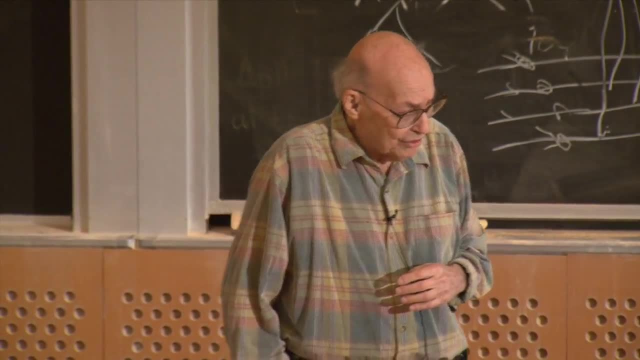 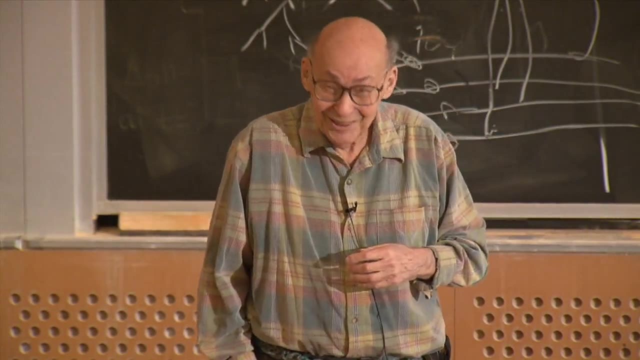 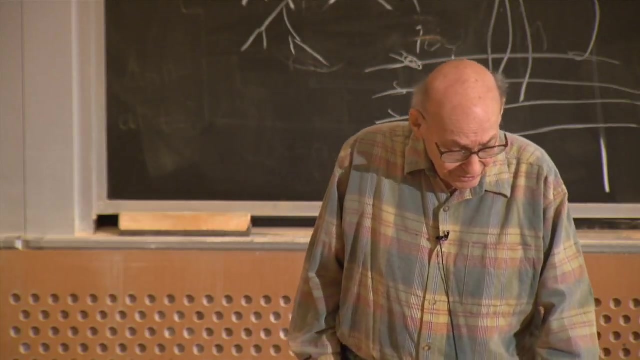 And so suddenly I said: oh my gosh, This is what Maria Montessori calls a. I forget what she called it. What's this moment when the child is open to being taught? So I said: this is her chance to learn a lot of new color names. 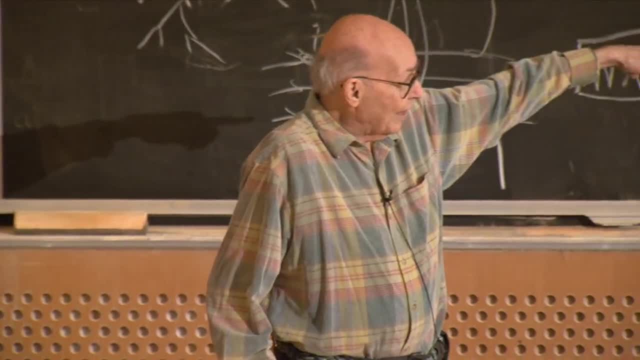 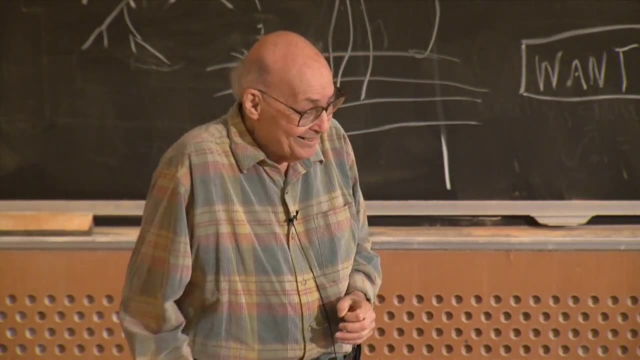 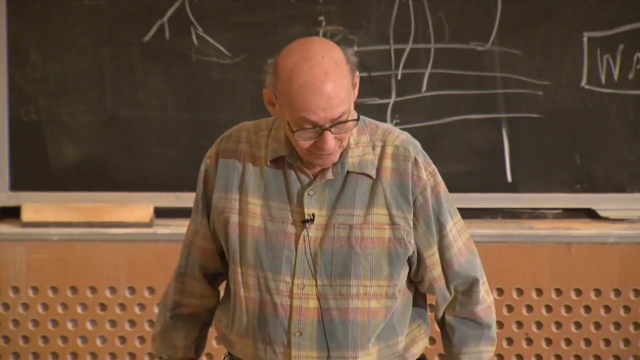 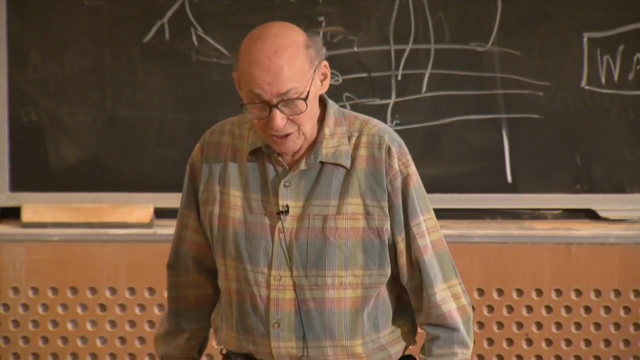 So I said: and what about this? I said that's aqua, And she said that's blue green, And I said: no, this is aqua, And she refused. So that was that. So some months later she learned some more color names. 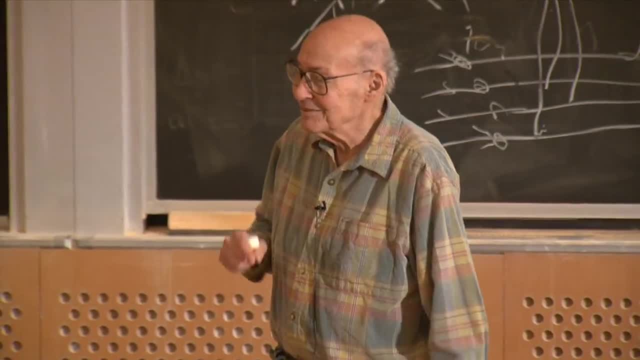 But it wasn't the same. MARVIN MINSKY- When she was saying blue green, was that because somebody had taught her blue green, Or it was because she was combining these two colors? MARVIN MINSKY- I think she was combining it. 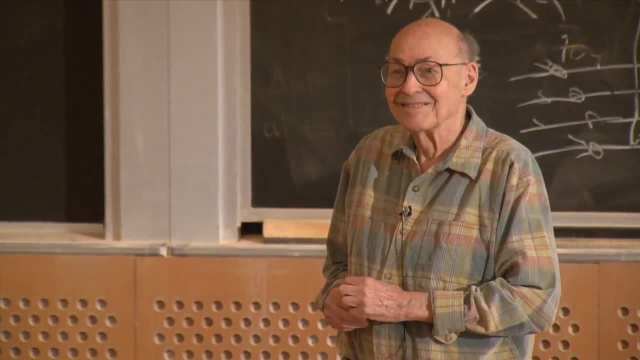 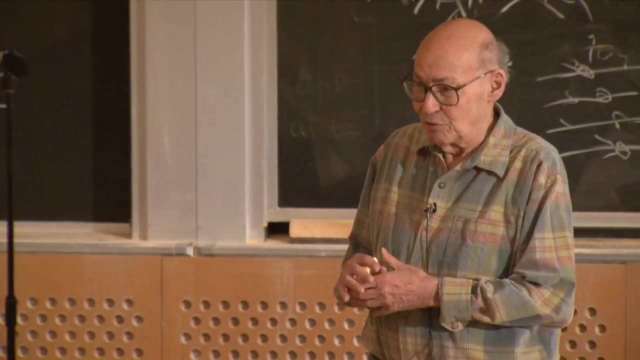 Do you remember? Yeah, I think she was combining it, because it looked a little blue and a little green. MARVIN MINSKY- Mm-hmm, So she had a concept that there were certain building blocks of colors. MARVIN MINSKY- It looked like she. 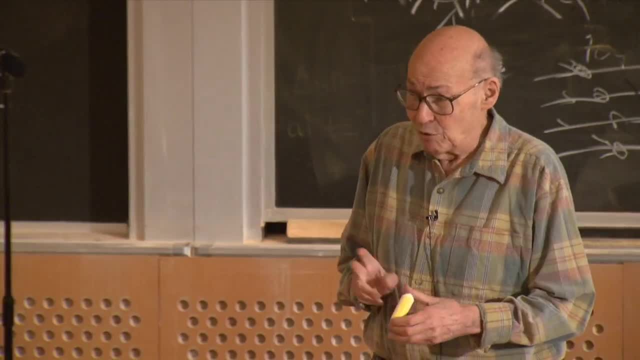 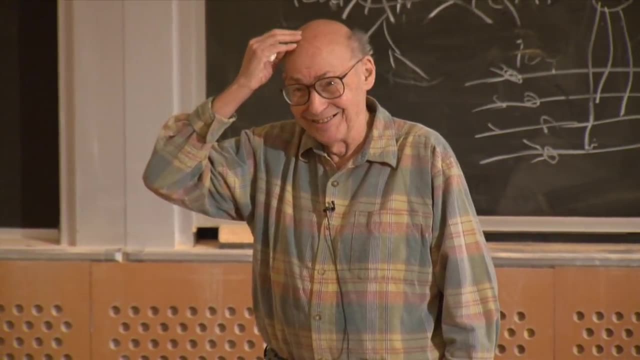 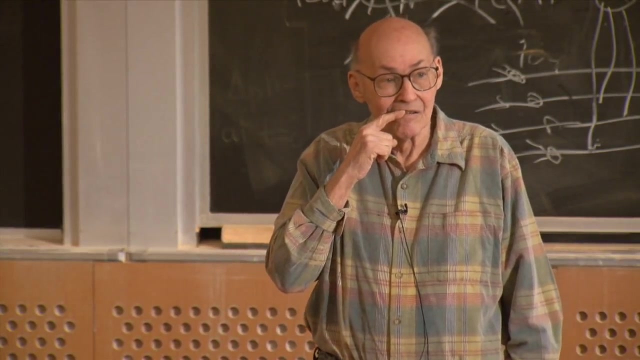 wouldn't accept a new one. Ella And I always wondered if I was 15 minutes too late. When does the Montessori door shut, Sort of. similarly, there's studies done on different languages with how well people distinguish different colors. So in Russian there's a different word that means light. 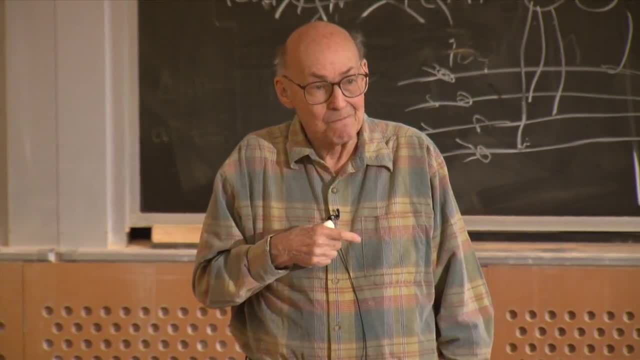 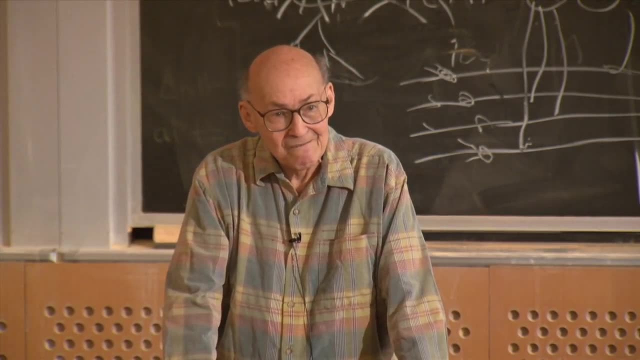 Blue and dark blue. So Russians are better at distinguishing different shades of blue than, say, Americans. And there's also a lot of languages that don't have distinct words from blue and green, And native speakers of those languages have trouble distinguishing blue and green. 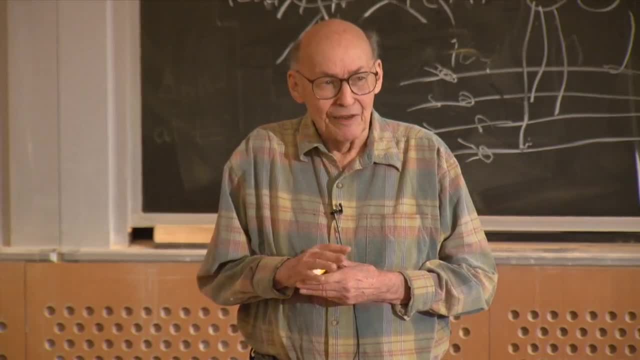 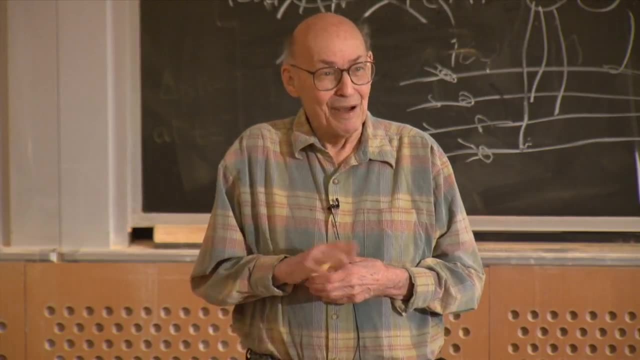 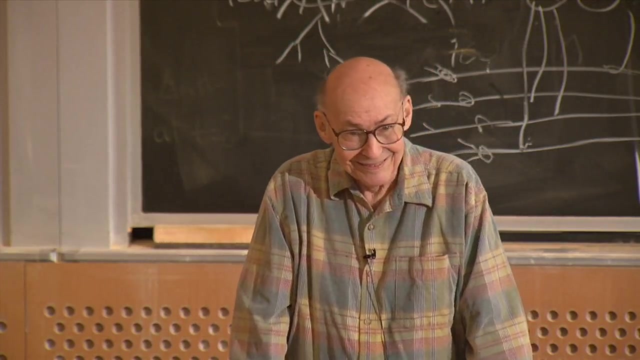 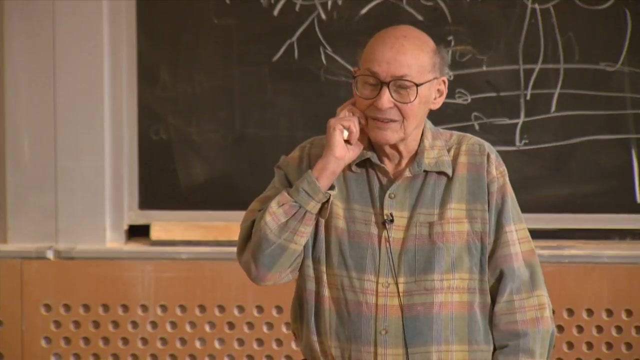 MARVIN MINSKY- So that gives me a great idea. If I could have found some unfamiliar objects and colored them aqua, that might have fooled her. MARVIN MINSKY- There must be a branch of psychology that worries about, because there. 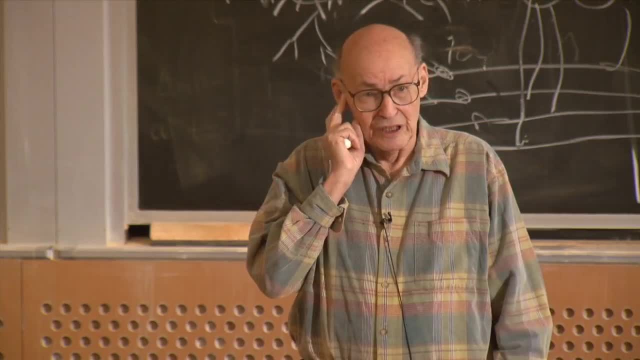 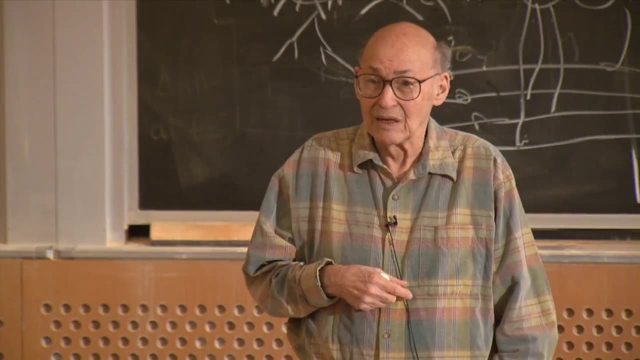 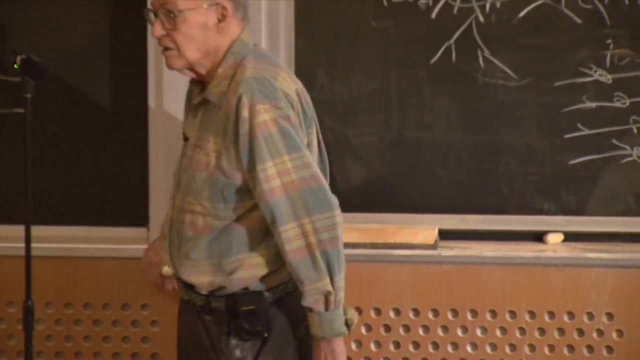 must be names for sounds too, And certainly a lot's known about ages at which children can't get new phonemes. Yes, A story in memory and language. So I'm bilingual. Maybe other bilingual people in the room The audience could confirm this. 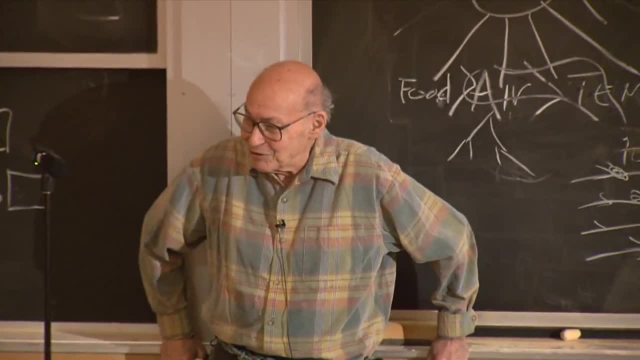 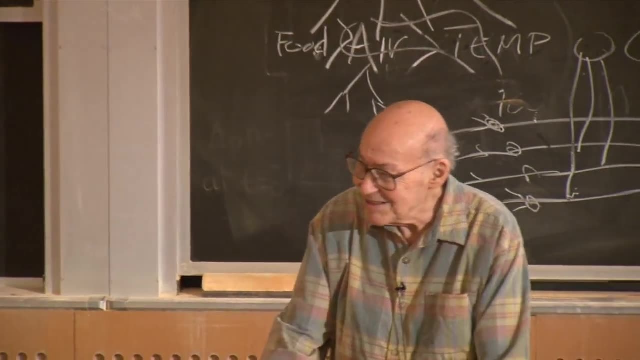 MARVIN MINSKY- I didn't know that. What's your other language, French? MARVIN MINSKY- For heaven's sake, I've known Henry for 20-odd years, So one thing that can happen is you can be talking with another bilingual person. 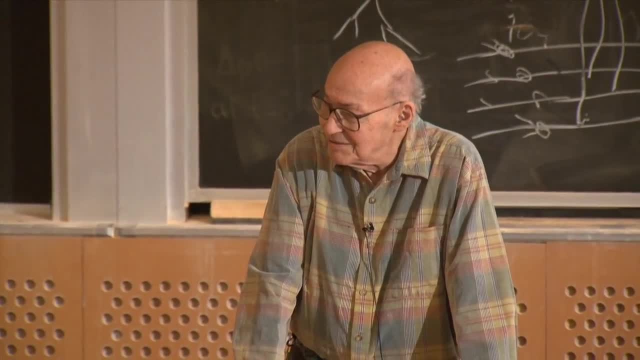 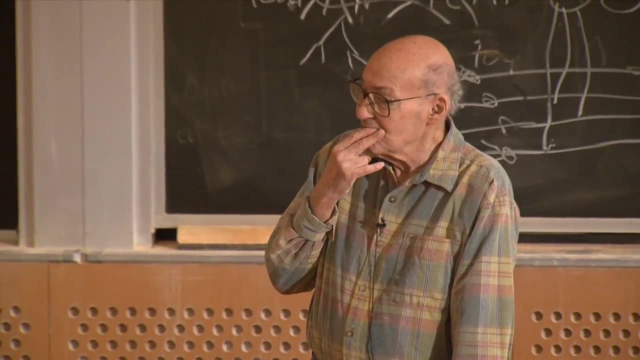 And so I can be talking with someone who also both speaks French and English. And then, like a week later, I'll remember every detail about a complicated conversation. We were working on this project And we needed this and all this stuff. 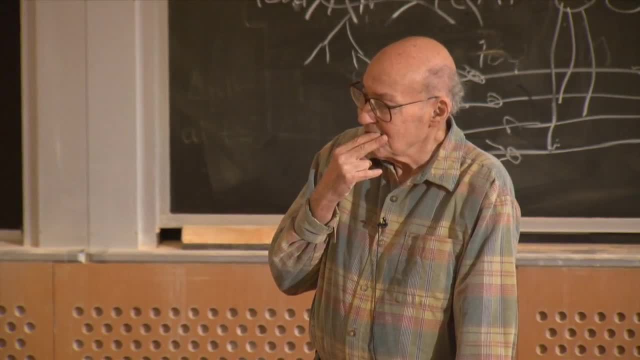 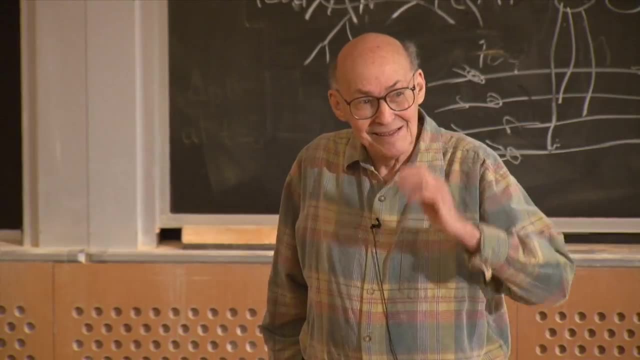 I remember every detail, except which language we had the conversation. MARVIN MINSKY- Yeah, my entire family is bilingual And we sort of generally speak a mix of Russian and English all the time. So I can never remember even what language I was speaking at the time. 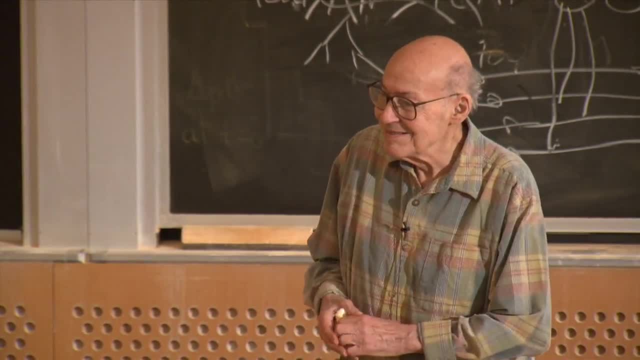 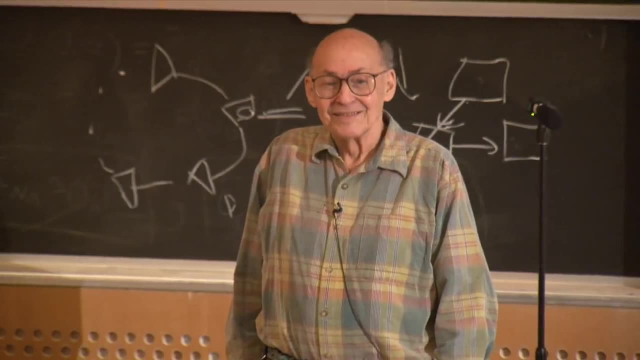 Yeah, that mystifies me, Because if we start in a language, how could I forget what language it is? MARVIN MINSKY- Well, I think there is a very simple answer to that one: You have a language that's neither English or French. 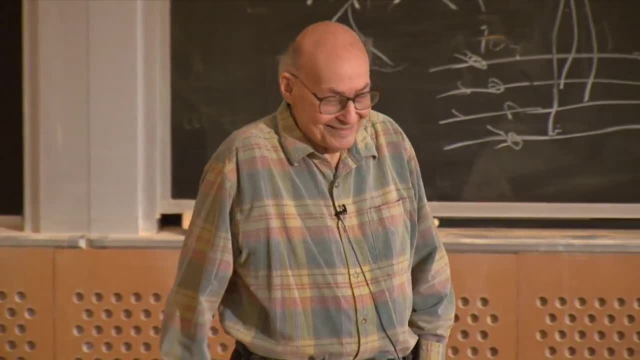 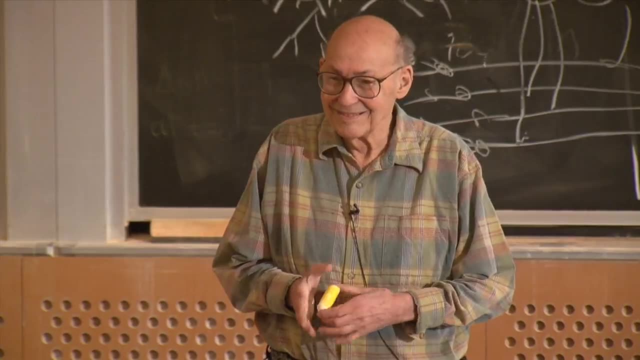 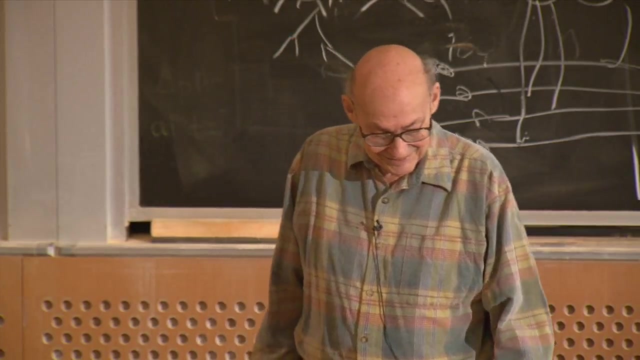 And you just have a very simple like tag going there And then you just, whenever you want to express something in English or French, you just encode, decode, encode, whatever is the word that those thoughts that you were having, MARVIN MINSKY-. Well, that's the question. 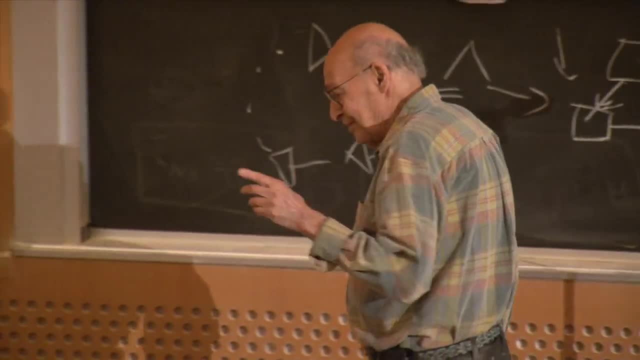 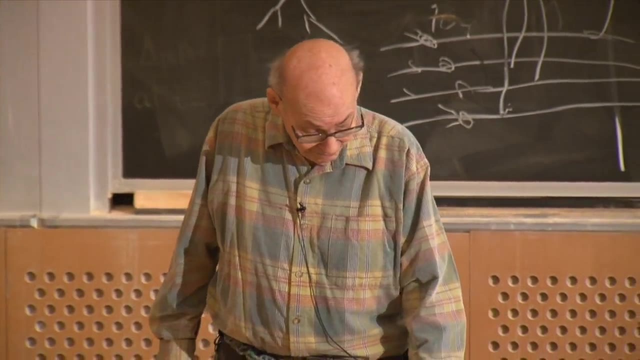 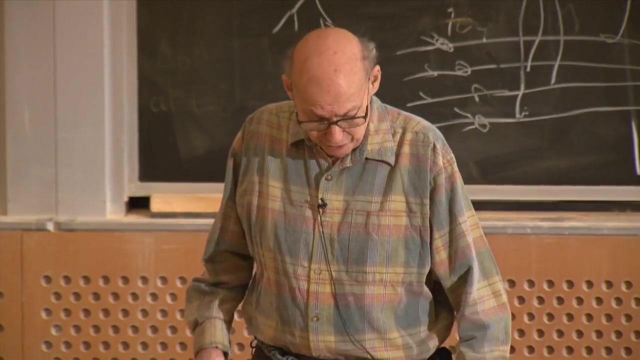 What is that language, Or do you have any thoughts on that? I don't know. You remind me. I think I mentioned this, But I was once at a meeting in Yerevan, Armenia, And there was a translator who was practically real time. 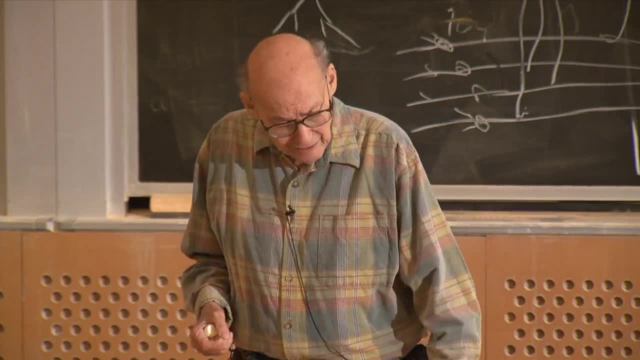 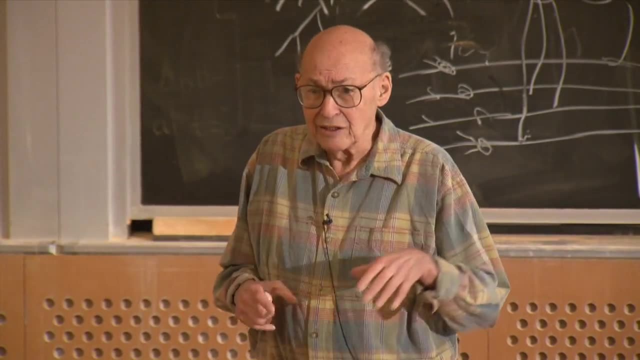 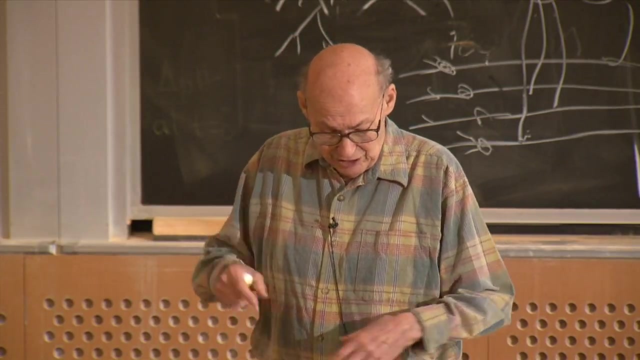 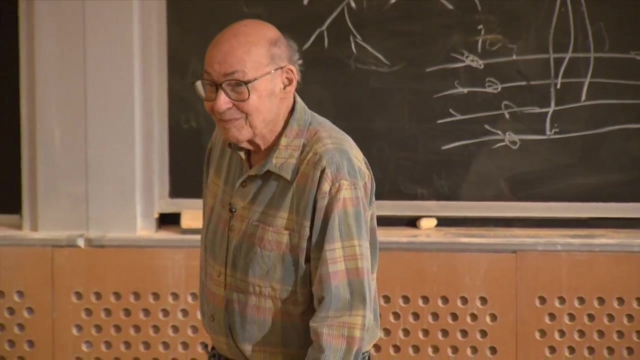 And Francis Crick was talking And at some point the translator switched And he started translating from English to English And Crick would say something And the translator would translate it into English. Very well, I thought Wasn't quite the same words. 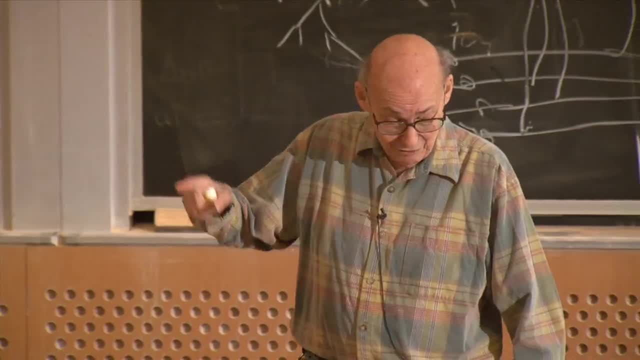 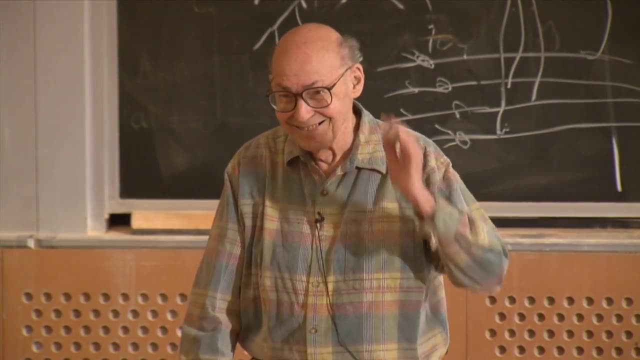 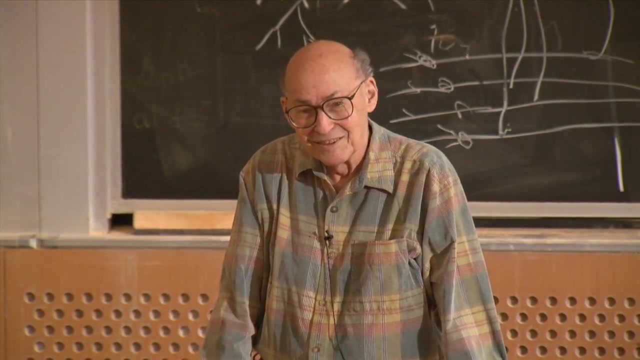 And after a while somebody asked him why he was doing that And he said he didn't realize he had switched. Do you think that could happen to you? I suppose MARVIN MINSKY-. Yeah, I think that there are other ways of like on translation. 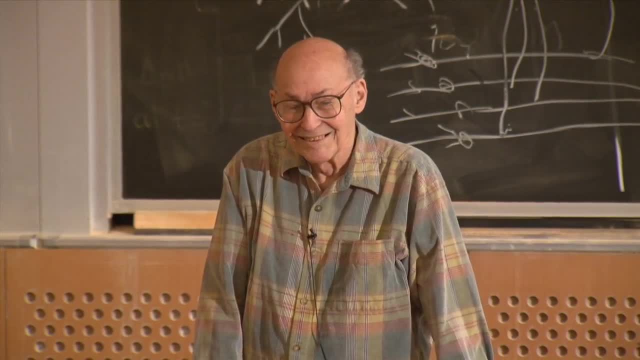 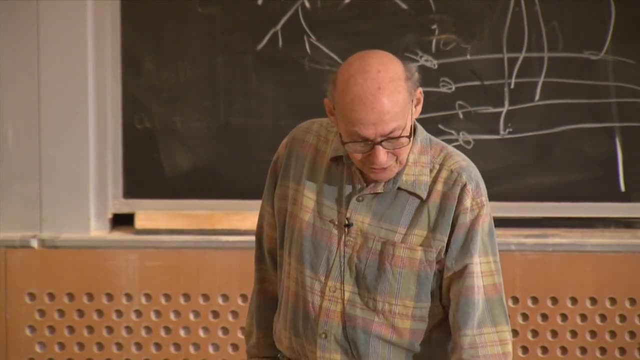 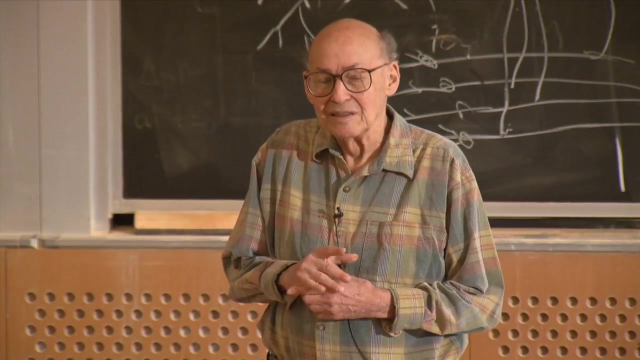 Transmitting ideas and learning, I don't know, maybe like arts or music besides the language, that can be really helpful. MARVIN MINSKY- I don't think there's anything nearly like language. But art is pretty good, But it's so ambiguous. 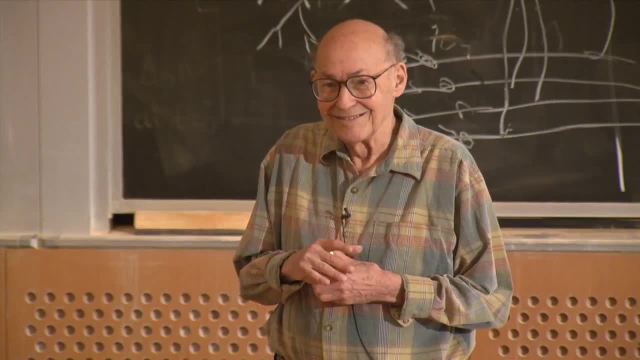 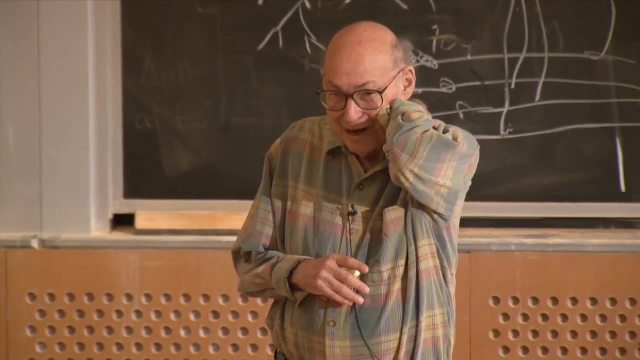 Cartoons. they're awfully good. How about Lisp? MARVIN MINSKY- What? How about Lisp? MARVIN MINSKY- Lisp? Yeah, that was a good one. MARVIN MINSKY- Oh right. 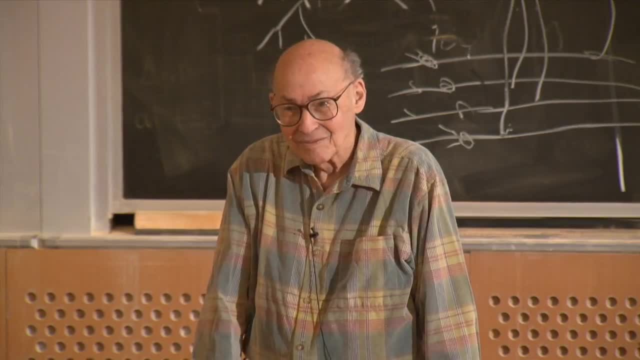 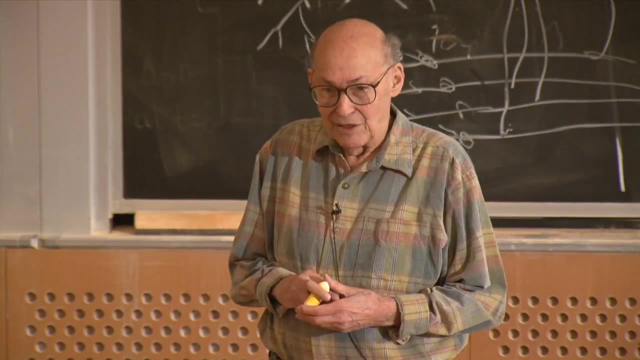 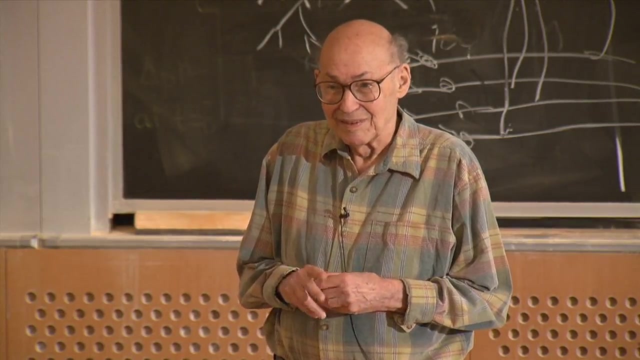 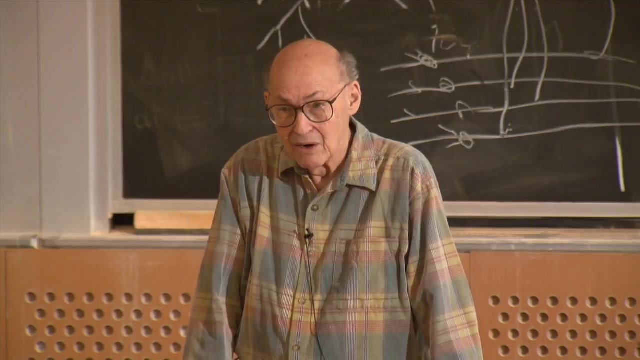 OK, MARVIN MINSKY- Programming languages. Yes, why is mathematics so hard? I wonder if the habit of using a single letter for every variable might be might make it easy and hard. It's hard, Who knows? But yes, you have great questions. 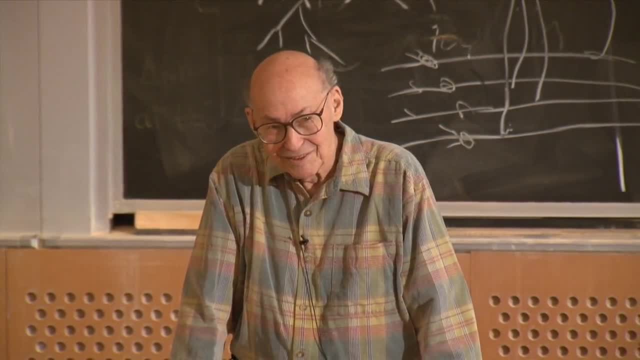 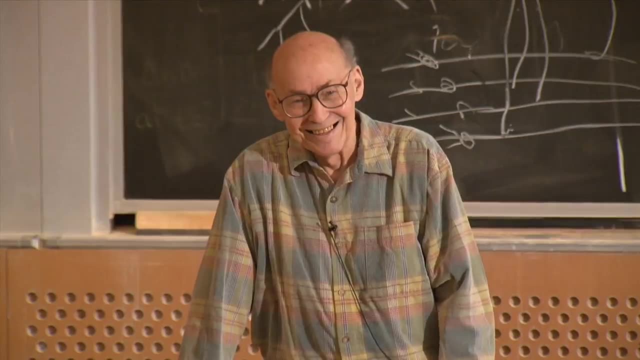 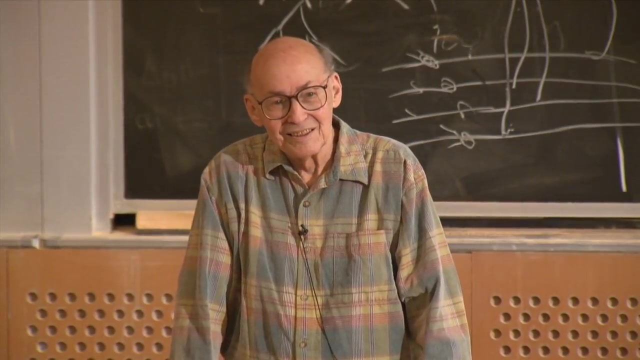 So last year you mentioned why mathematics is hard. I thought about it. MARVIN MINSKY- Say it again. Last year you mentioned that mathematics is hard And I thought about it and I do feel like there's an extreme lack of representations of ideas. 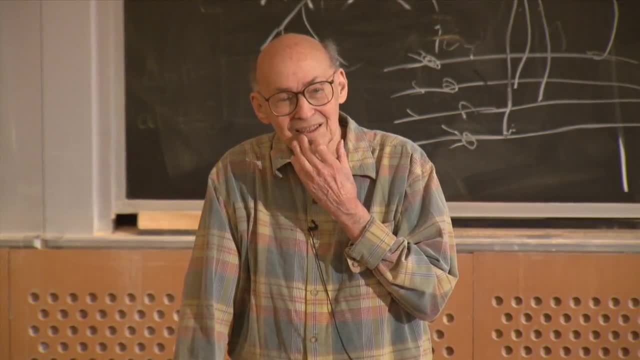 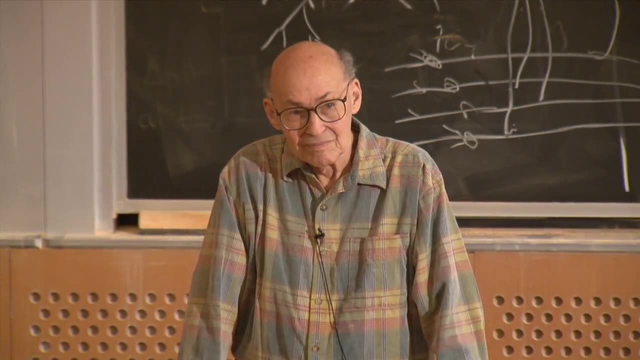 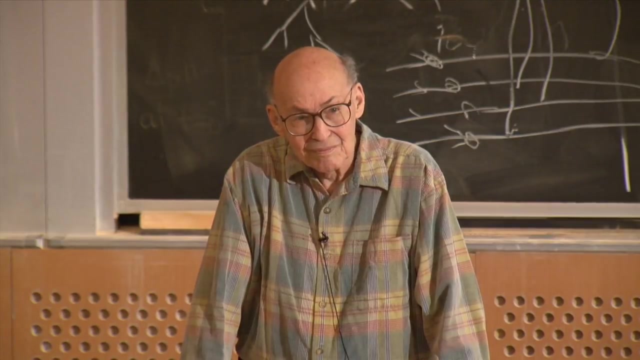 Solving a problem, you need to identify so many things And there's so many processes that you like have to apply to them without having a name for any of them, for like classification. Well, you have induction and deduction. 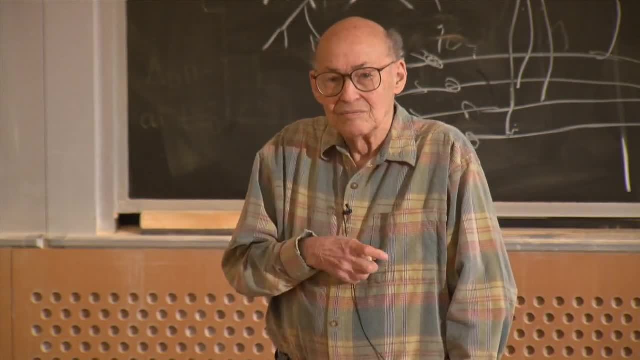 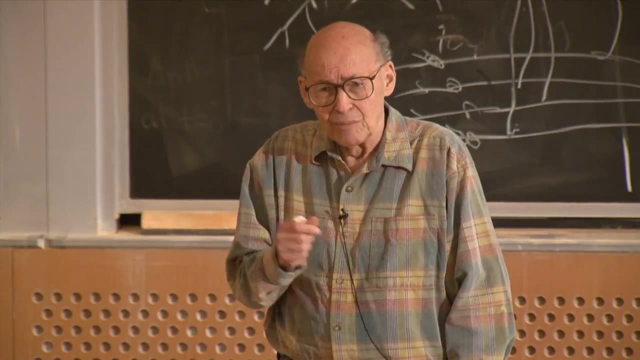 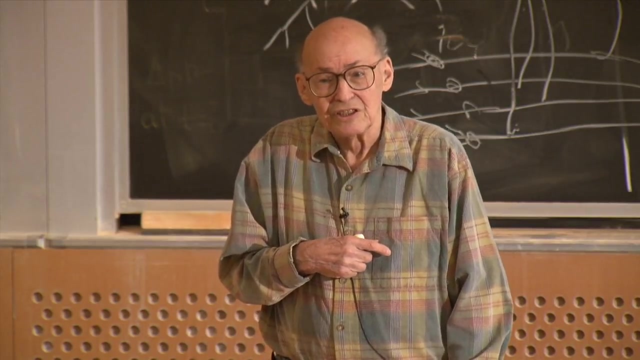 That's about it And contradiction. like MARVIN MINSKY- Yes, and you have this. One feature of mathematics is completely unredundant representations. I wonder if there's some way to fix that or change it. It's isn't that. 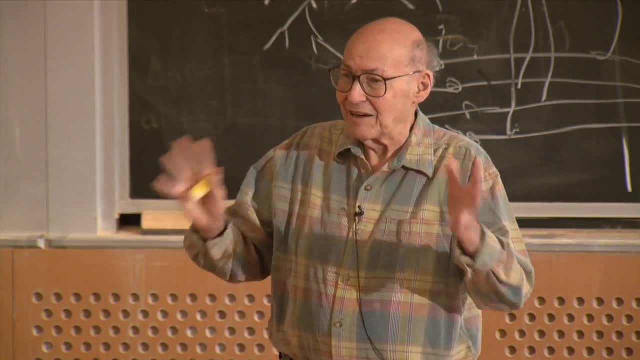 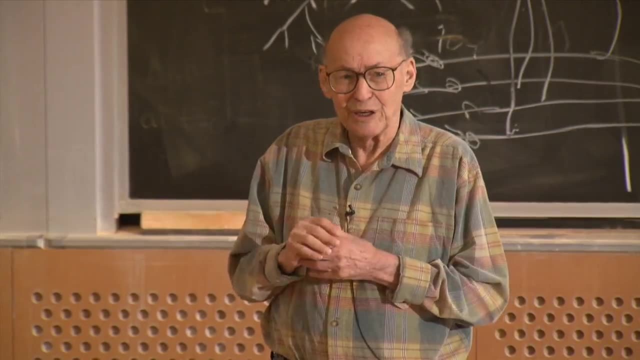 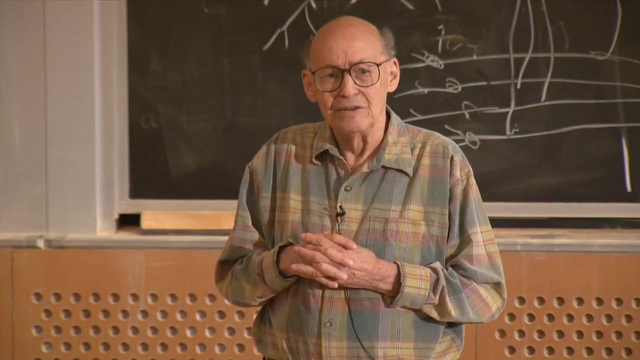 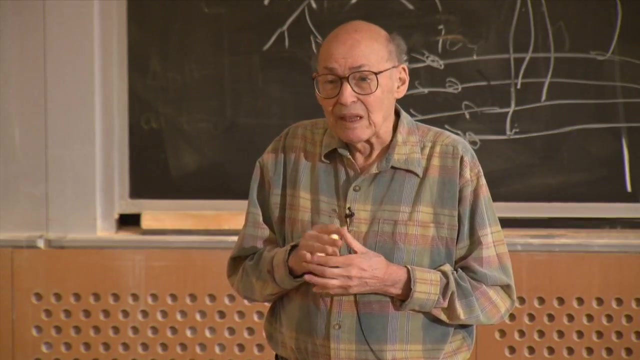 MARVIN MINSKY- Yeah, I mean, what other activity do we have where there's absolutely no redundancy at all in a mathematical experience? So for some people it's delightful And other people it's very hard. I mentioned Licklider who in programming he would 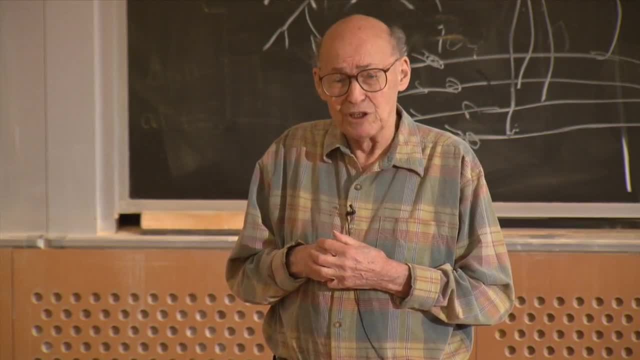 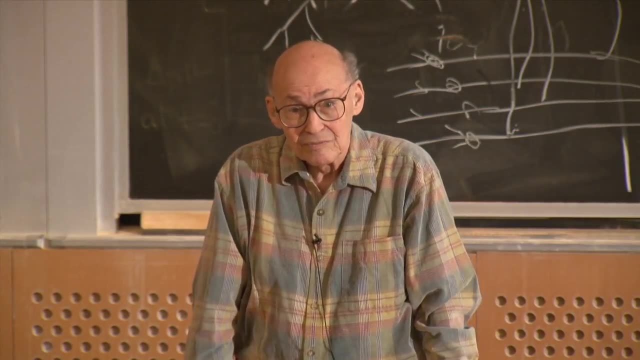 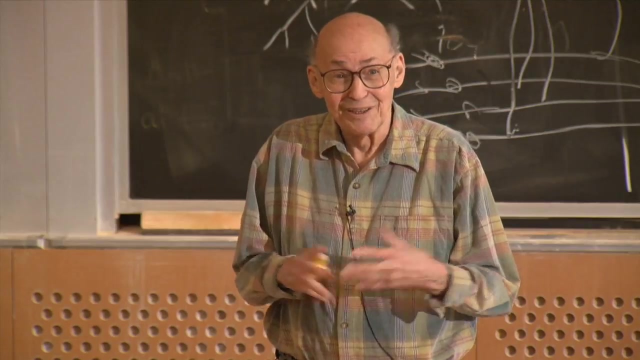 have very long variable names. Sometimes they'd even be sentences, like the register in which I put the result of: And the great thing was you could read those programs. They looked sort of stupid, but he didn't have to make. he didn't have to. what do you call notes? 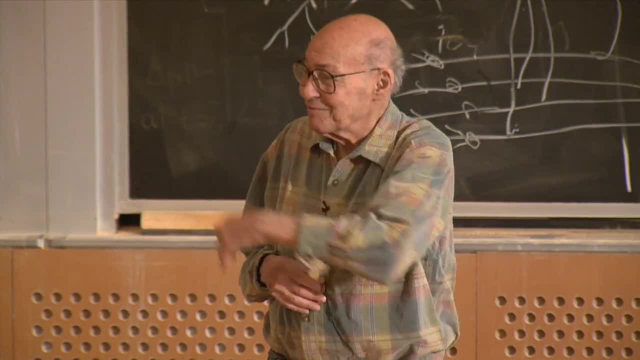 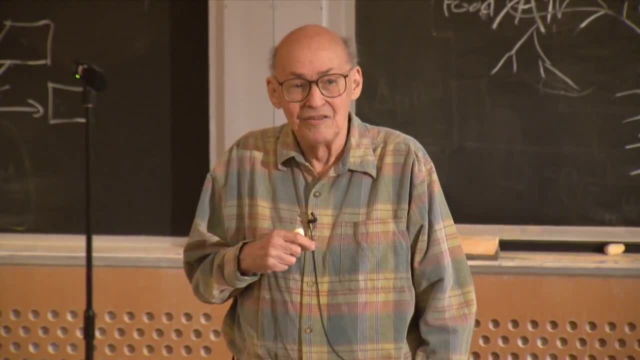 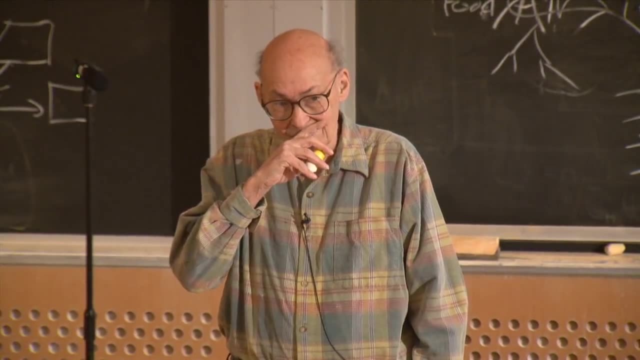 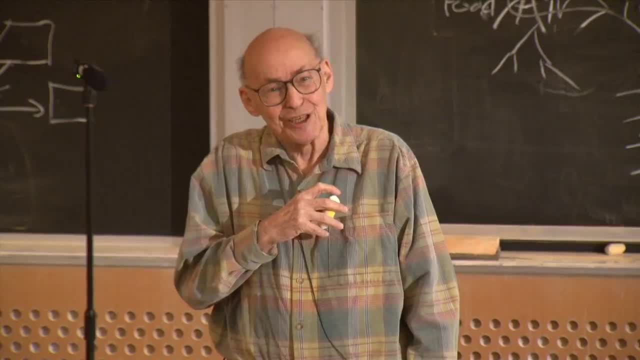 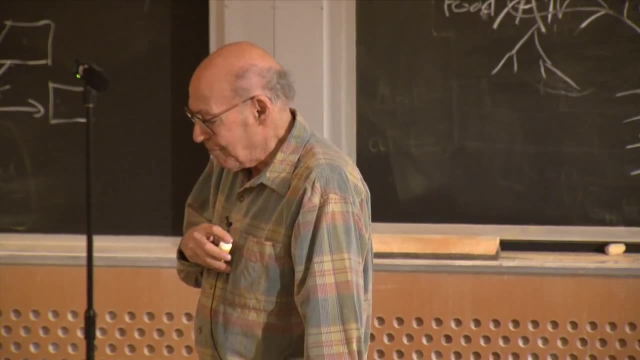 MARVIN MINSKY-. Uh huh, What kind of math do you like? Do you do topology? I like topology. I like topology, MARVIN MINSKY- I love topology. That was I once was tutoring a high school student who. 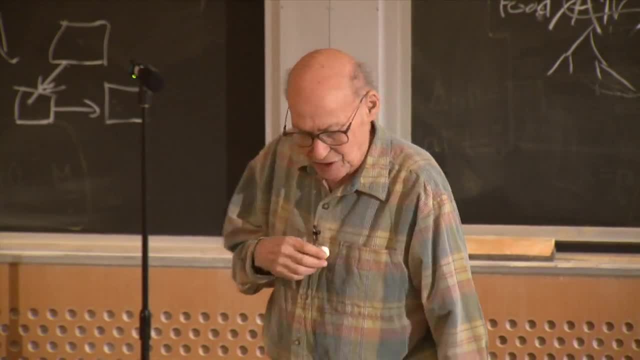 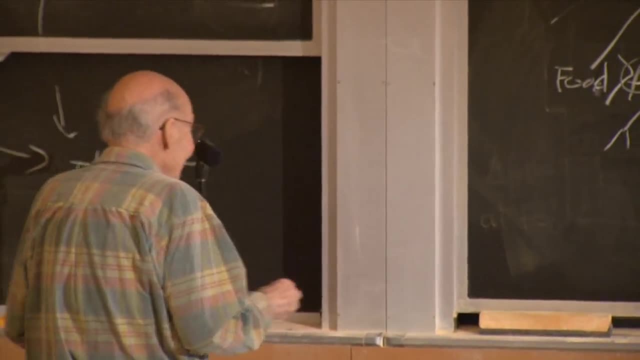 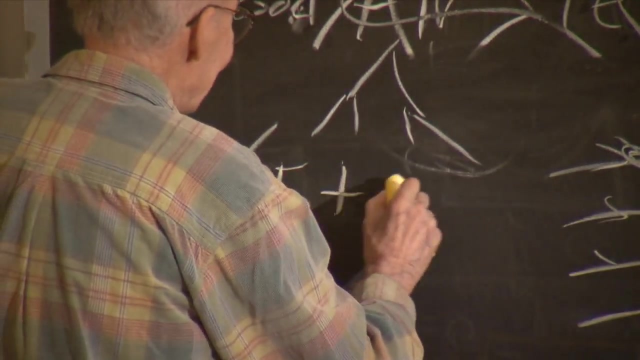 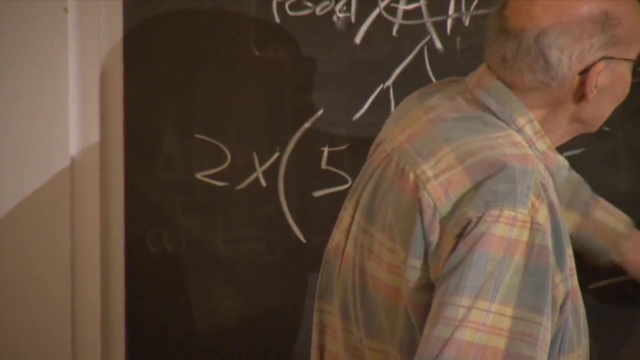 couldn't do algebra. I'm a- I don't know if I made it- mentioned this, And it turned out he didn't know how to use parentheses, So he would have an expression, stuff like that. But if there were something in there, 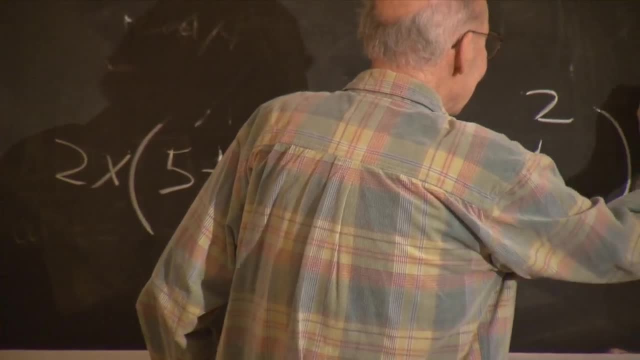 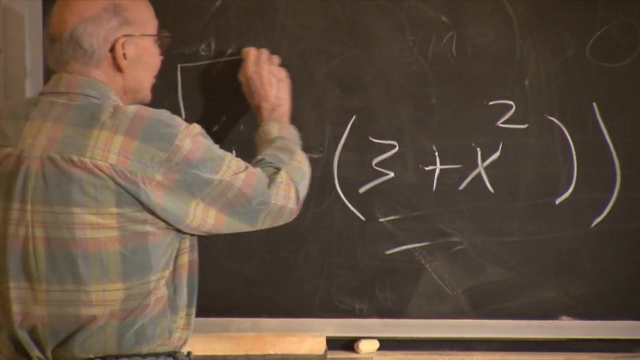 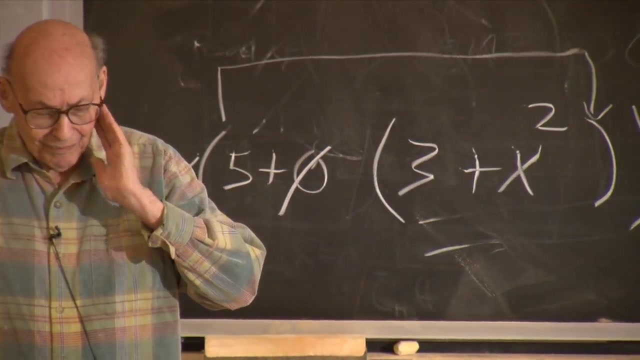 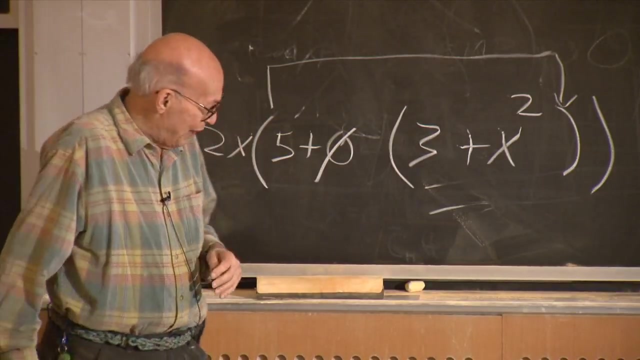 he didn't know what that meant because he knew sometimes he would. he didn't know how to match them, So I couldn't figure out why. And I asked: how come? And he said maybe I was sick the day they explained. parentheses. 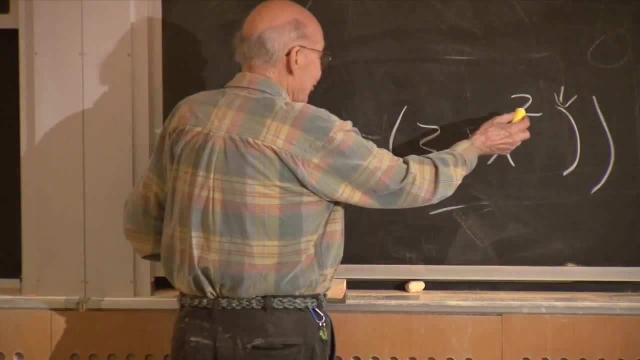 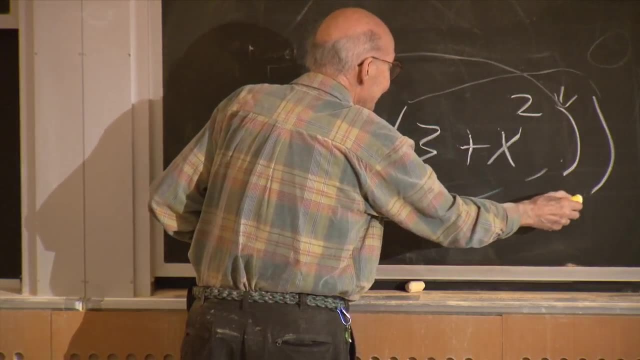 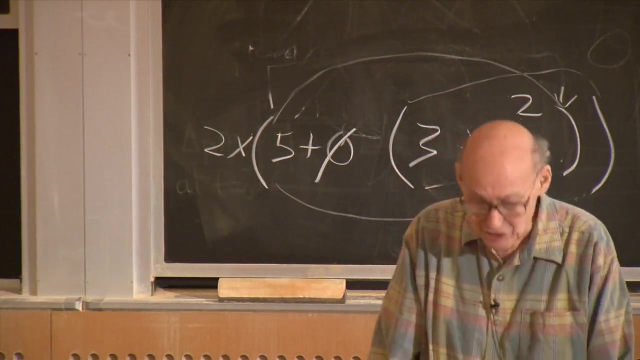 And so I gave him little exercises like make them into eggs. And you see, if you make this into an egg then this egg won't work. And the funny thing was he got that in five minutes and then he didn't have any trouble with algebra the rest. 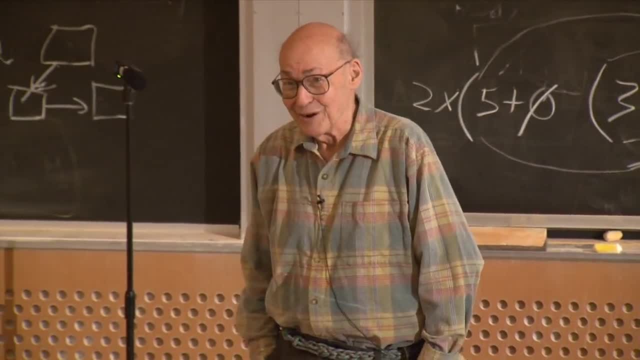 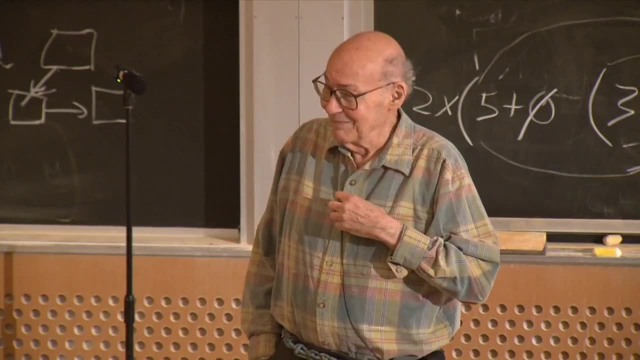 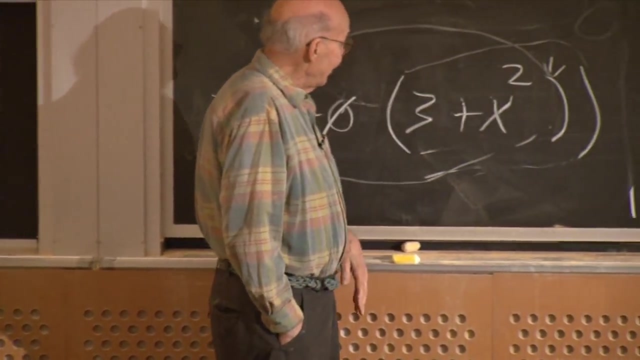 Can you imagine, I wonder. I've never done much tutoring, but if you can find the bug like that it must be great fun. But I bet it doesn't happen very often. That was so funny I couldn't imagine, not, you know. 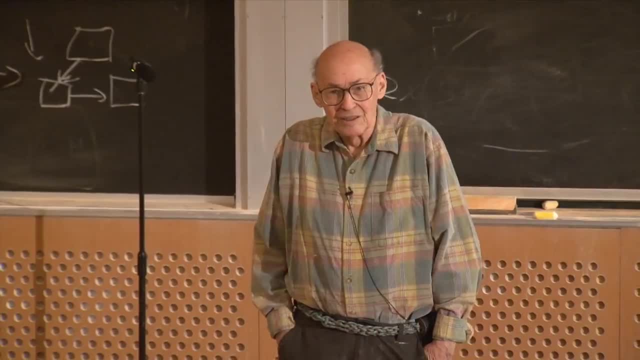 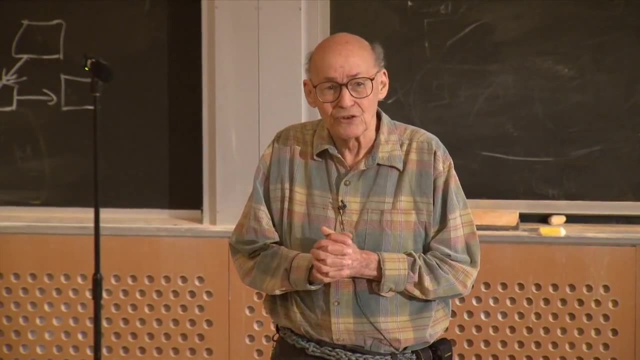 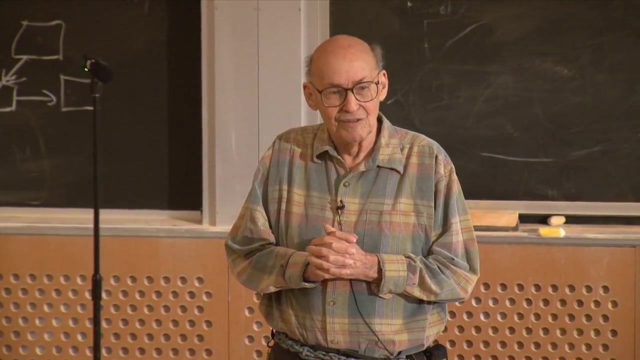 So if you don't have language, there must be. Well, why are some people so much better at math than others? It's just that they've not understood. It's just that they've not understood about five things. I feel like they have a set of things. 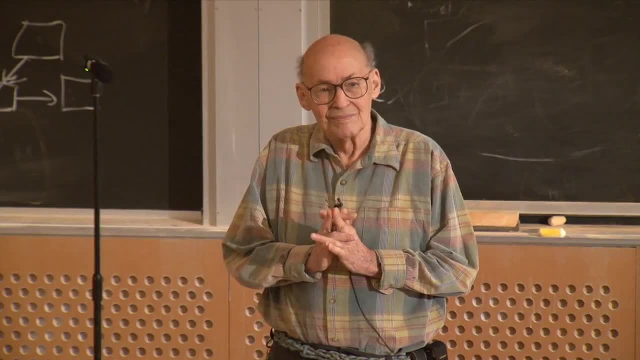 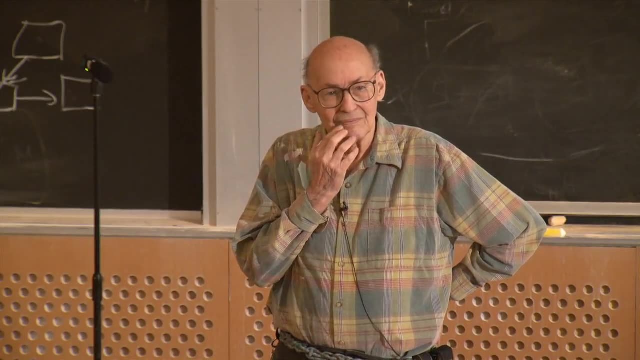 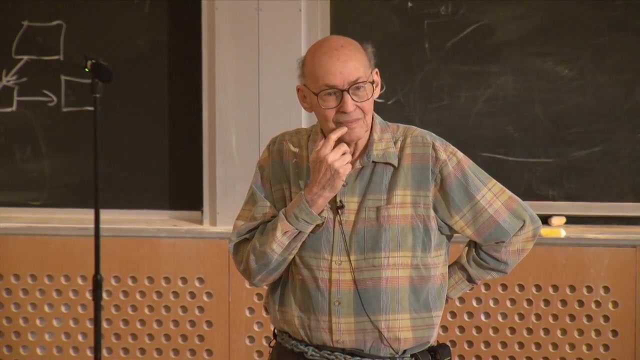 they know to go to when they face a problem. So well, that's kind of similar to your Feynman story, But I feel like they know exactly. They have names for concepts of ways of solving problems. So they look at a problem and they're like: 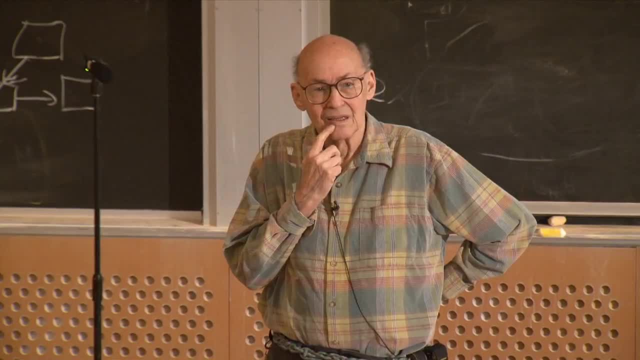 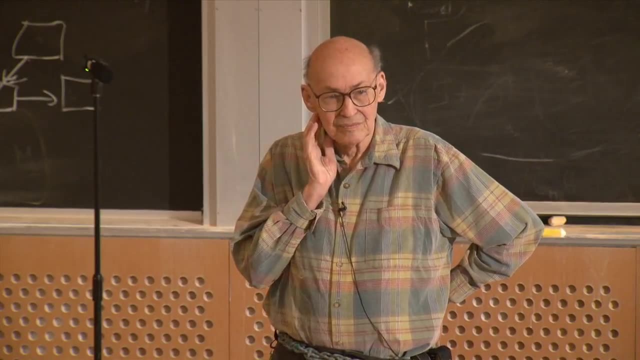 I'm going to try this approach And then, if it doesn't work, I know this other approach. I'll just try it, Instead of looking at the problem and you think: OK, so what possible thing, what possible method can I use? 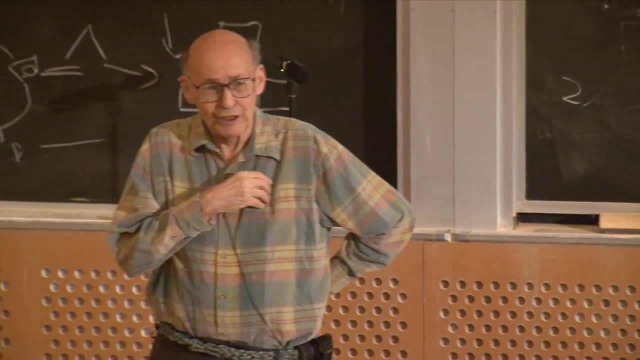 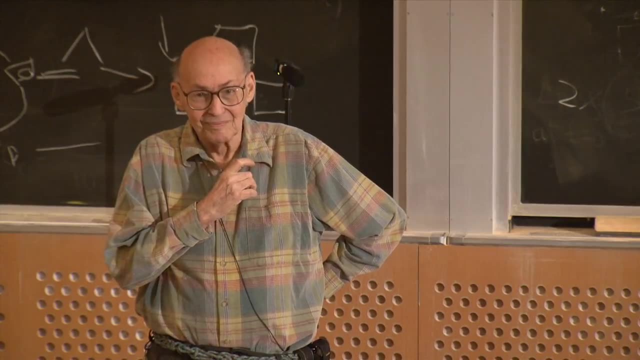 Oh, names for methods. So do you have public names or are they secret names? I feel like they're secret names. They're just stored Because they can't explain it to other people. They can't be like this problem. there are a few of them. 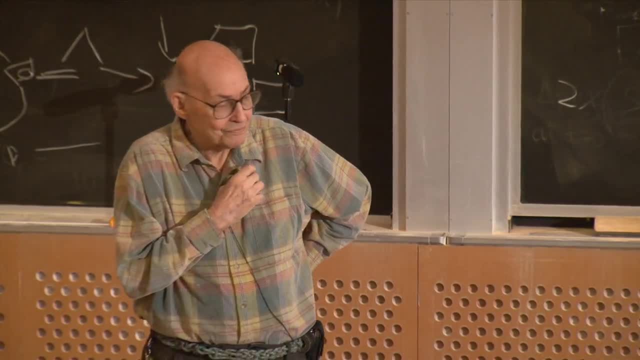 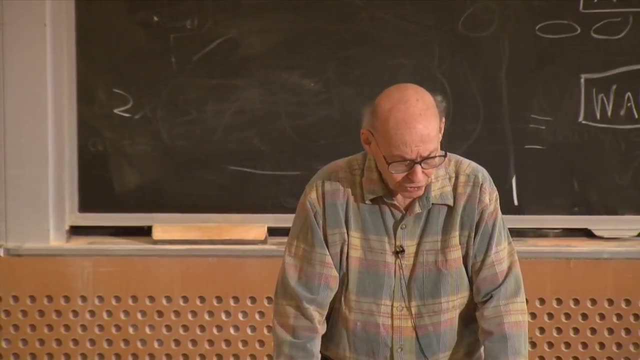 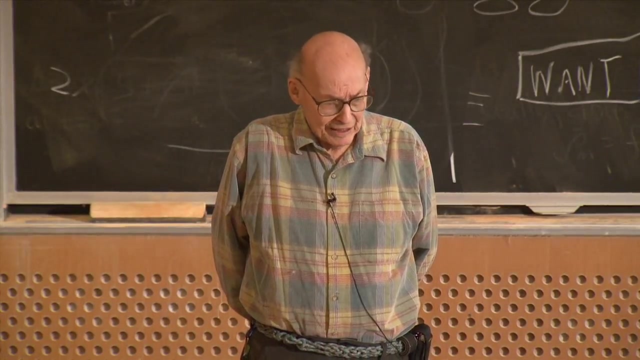 And then this one, This problem and that problem. They generally they have the general same method, although they're greater than that. I had a friend who was a composer And she had all sorts of sounds And they were filed away on tapes. 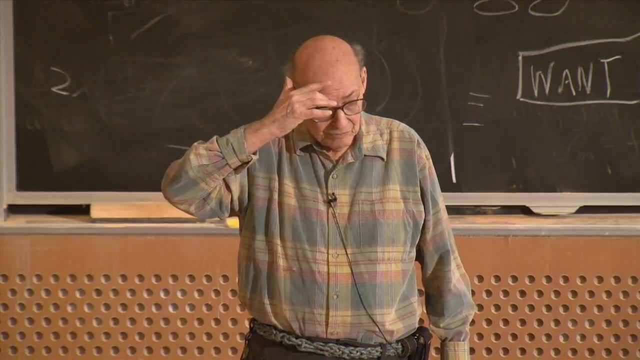 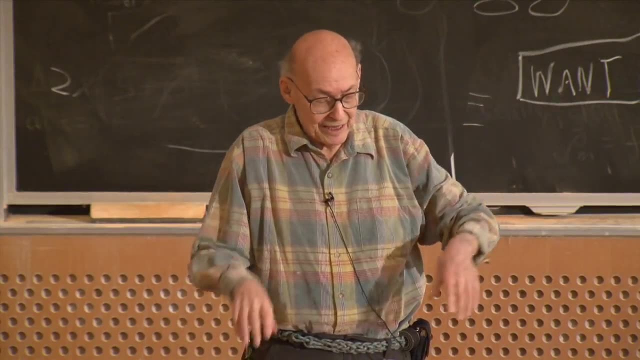 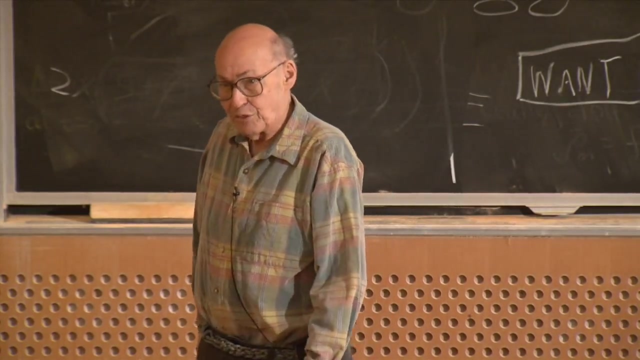 And the tapes had little symbols on them And if she needed a sound she would go to the closet and pull out the right tape and it had more symbols written on the reel And she'd get this thing which might be a thunderstorm or a bird or something. 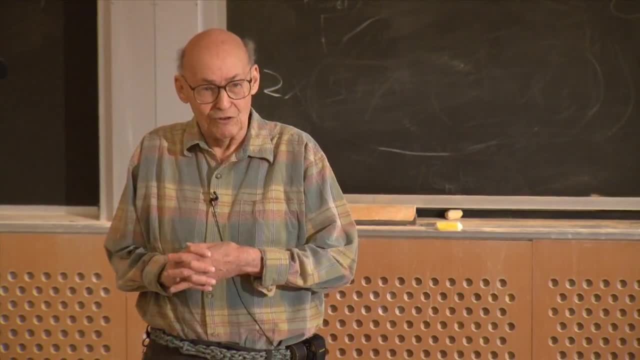 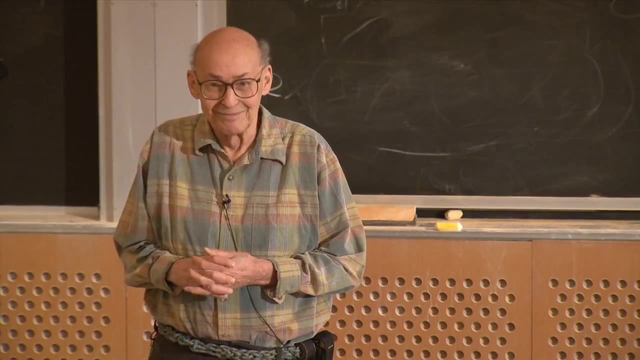 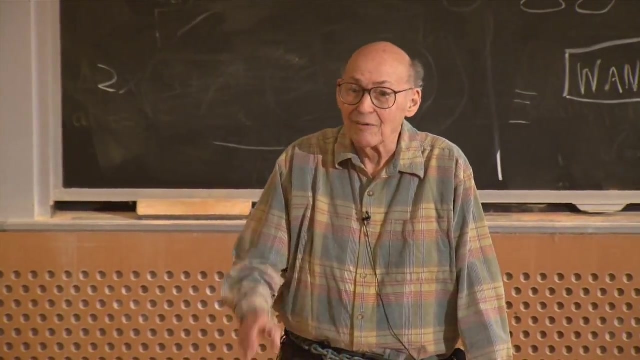 So I asked her what was her notation for these sounds, And she giggled and said: I can't tell you. It's too embarrassing. I never found out, But she had developed some code for sounds. Yeah, So I would say that they. 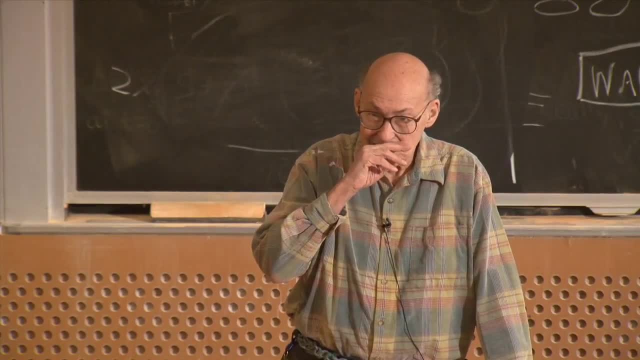 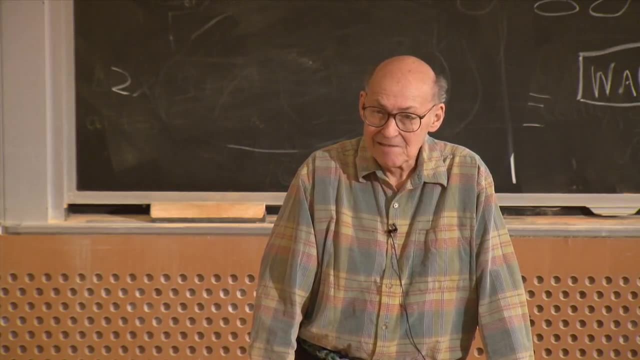 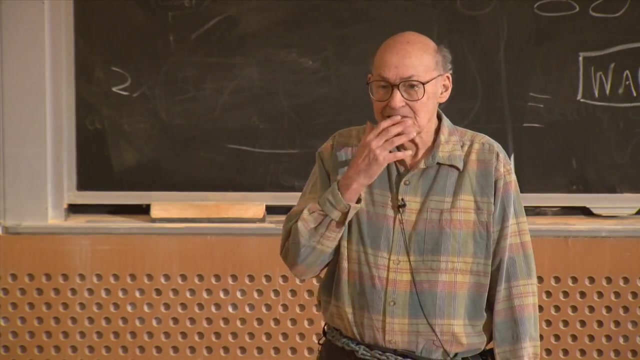 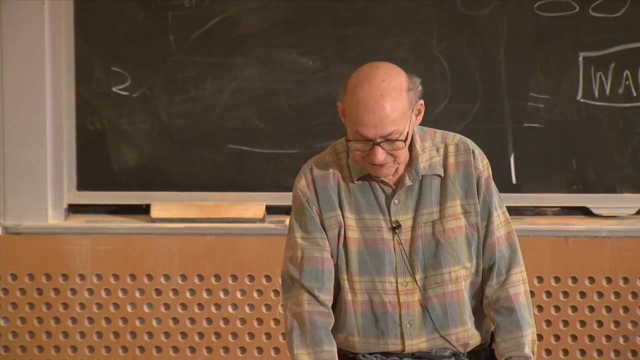 have some optimal representation of things. that math requires symbols or patterns of solutions And their representation is optimal. And if you're good at math it doesn't mean that you're good at playing music, Because when you play music well, you have maybe a good representation of the sounds. 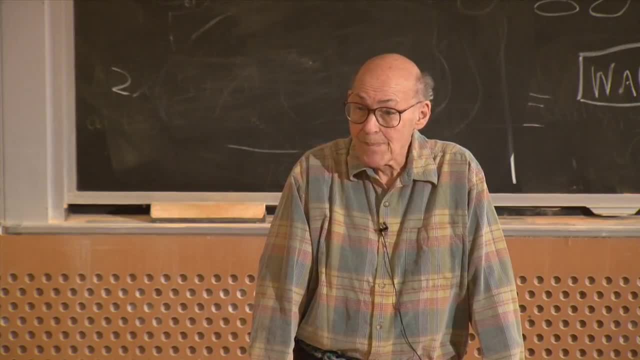 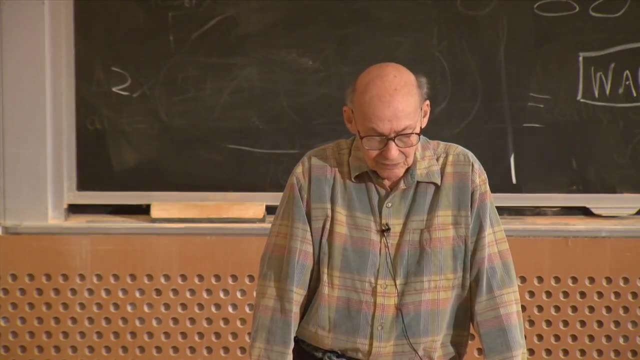 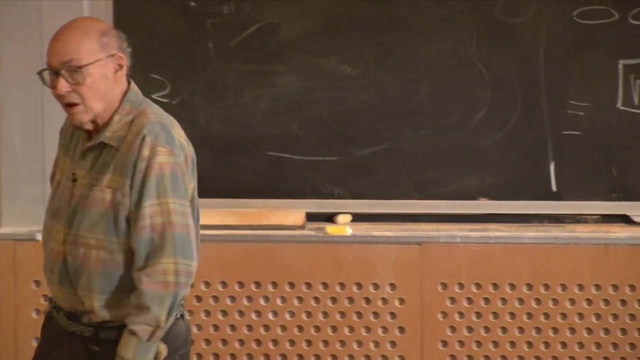 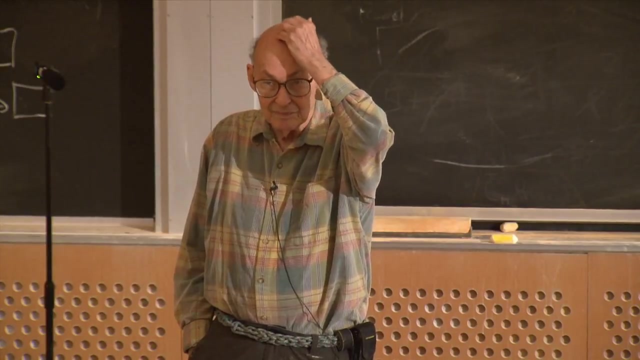 And so it's just being optimal. Yeah, So you can access like: oh, so I have these solutions, these patterns of solutions that I need to. I don't know, I need to solve this math problem I have, I don't know, by induction. 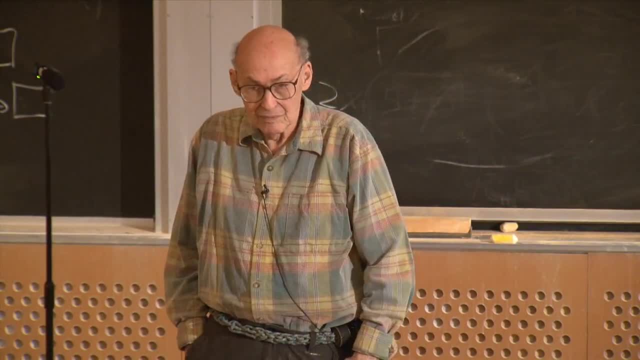 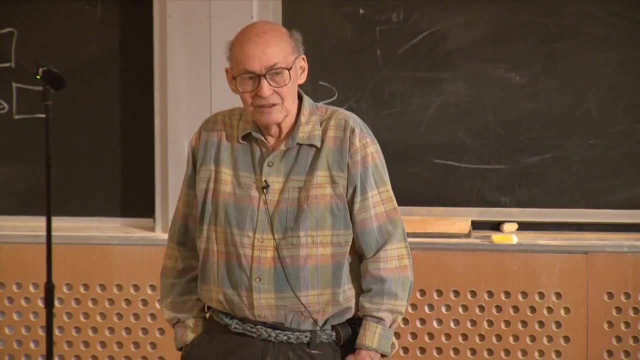 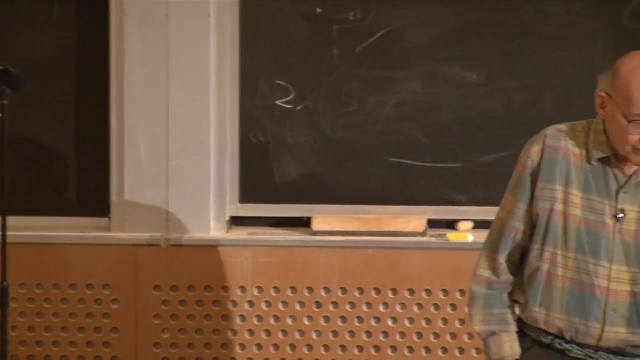 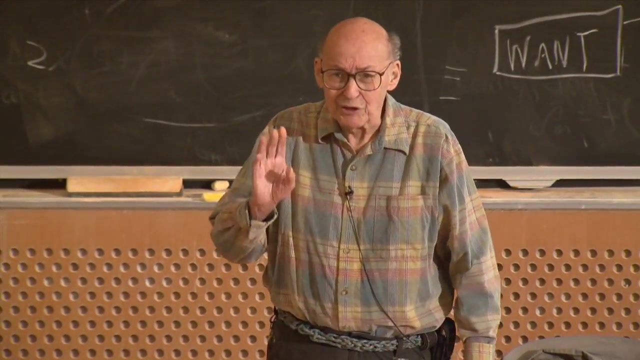 or by a contradiction And in his brain or somebody that knows a lot. the person can access it very fast. So the representation itself is very well defined, So you can access it. That's an interesting whole, Remember. let me interrupt. 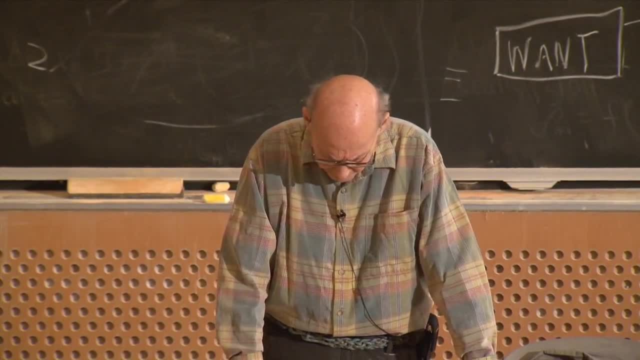 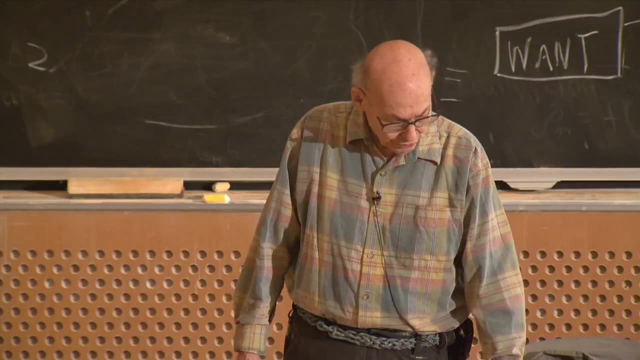 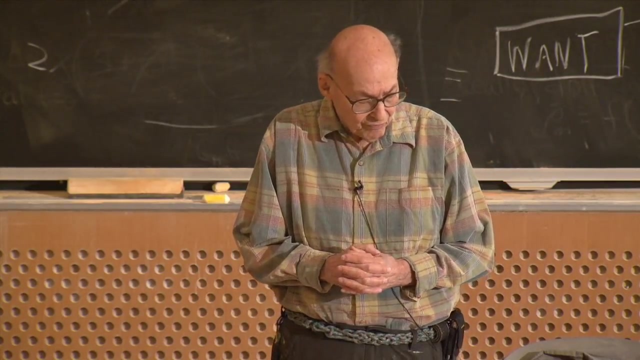 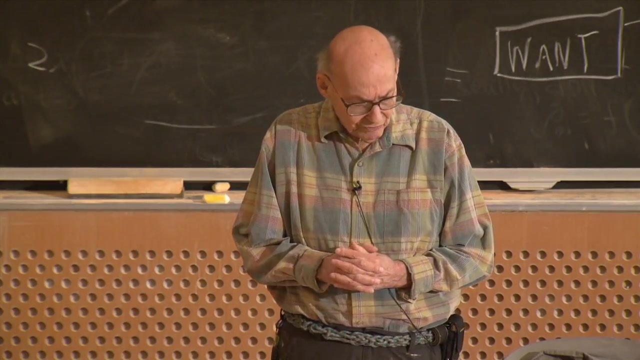 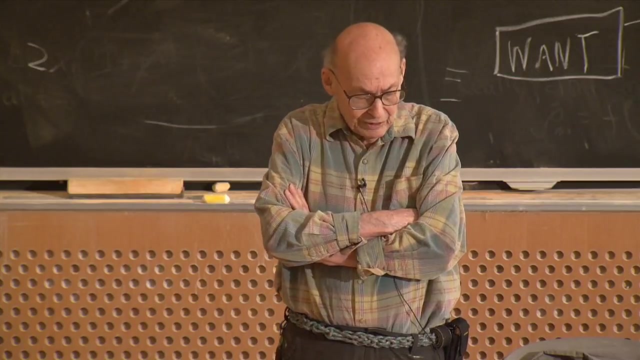 I was once in some class, math class, And it was about n-dimensional vector spaces, And some student asked: well, how do you imagine an n-dimensional vector space? And there's two stories, So, and the instructor, who I forget, who fought for a while. 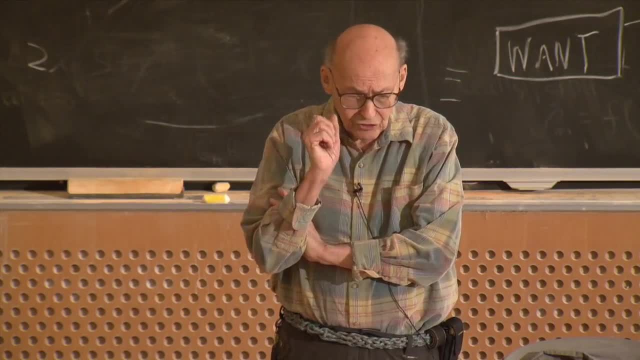 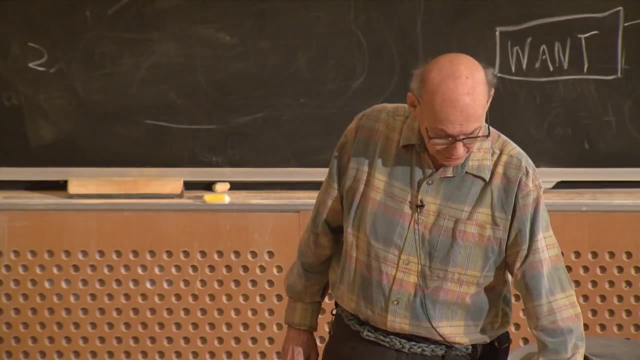 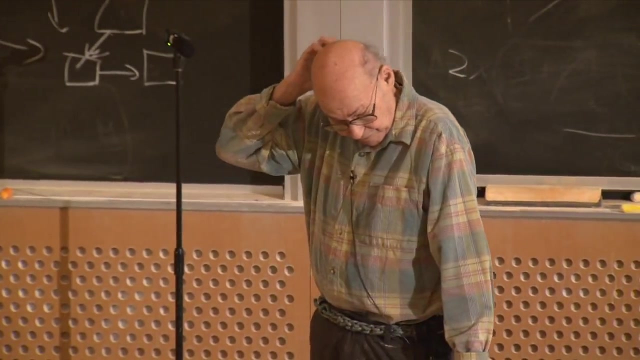 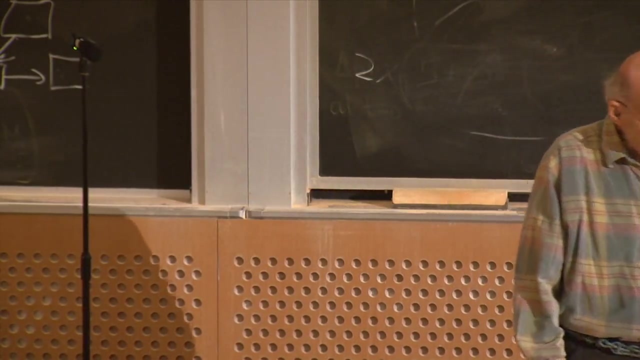 And then he said: oh, it's very simple, Just pick a particular n. So, Yeah, Yeah, Yeah, Yeah, Yeah, That was completely useless. So then next time- and I was a disciple of a mathematician at Harvard named Andrew Gleason, who was a wonderful man. 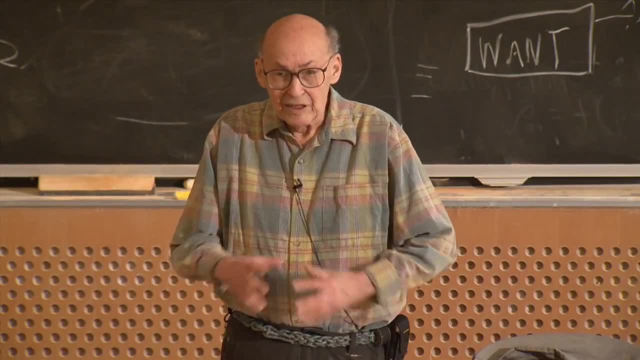 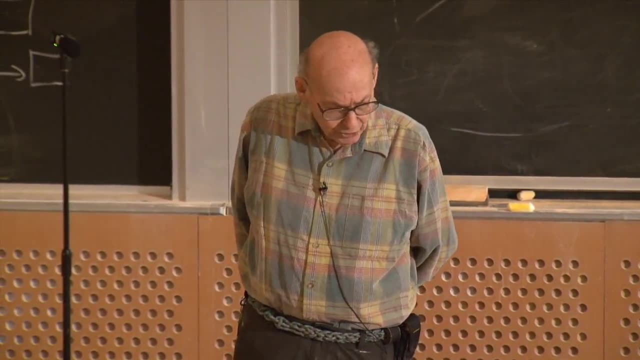 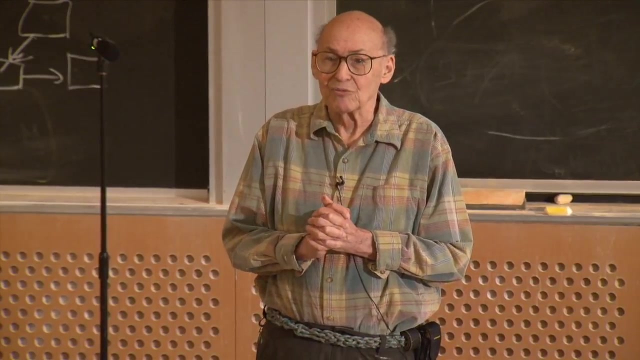 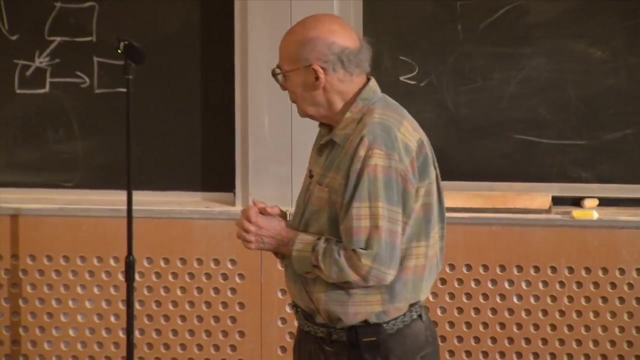 only a couple of years older than me, But he had won the Putnam three times first prize. And I said: what would you tell a student who wanted to understand an n-dimensional vector space what it means? And he said, well, you should give him five or six ways. 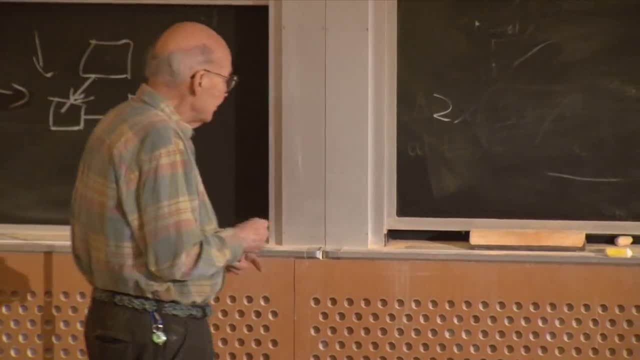 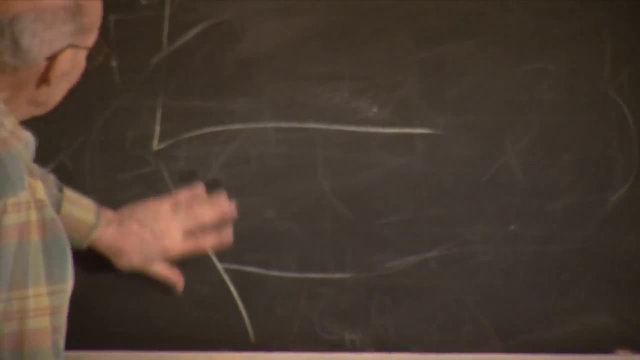 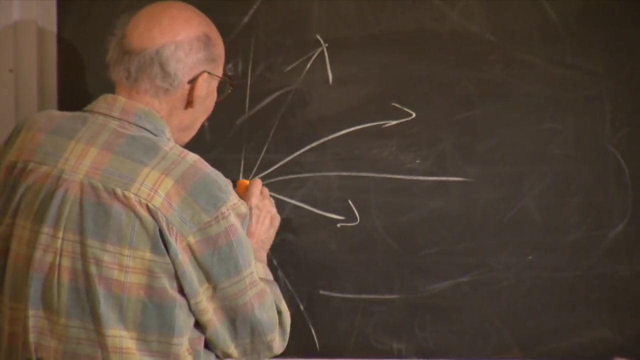 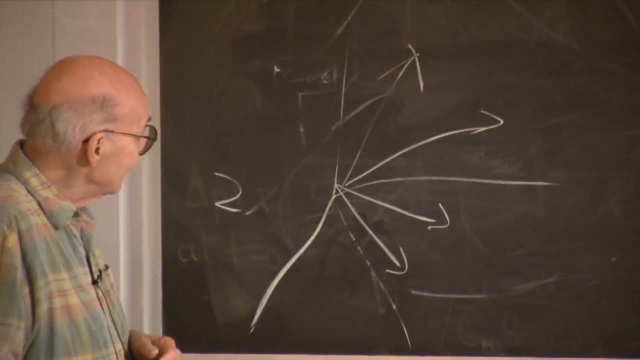 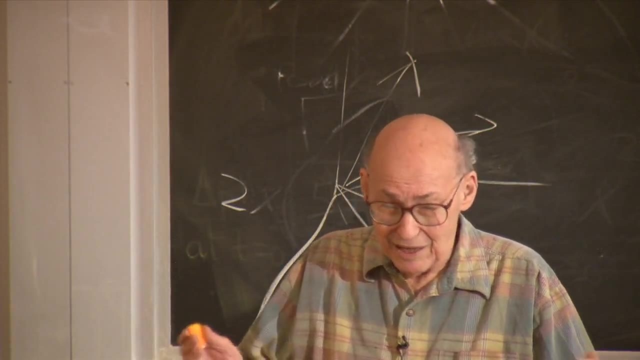 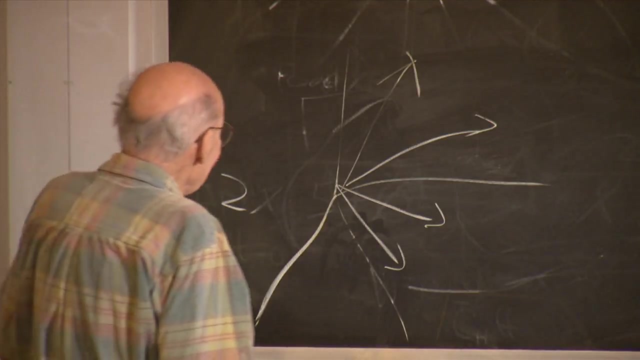 to all the others, just like that. And then he added: and you should make the sum, And if there's an infinite number, you should have the sum of the squares of their lengths converge to a finite value. And then he said: or you should think of it. 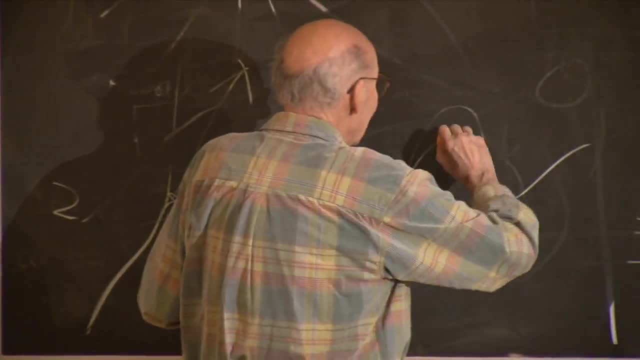 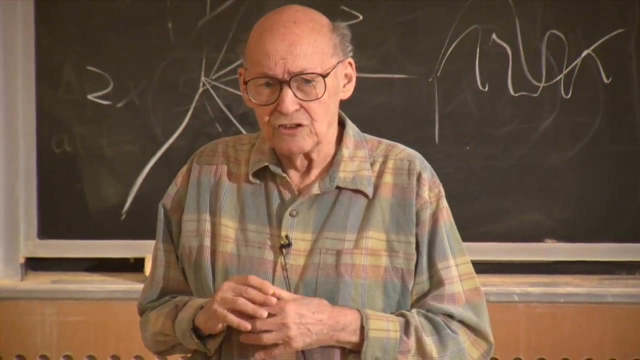 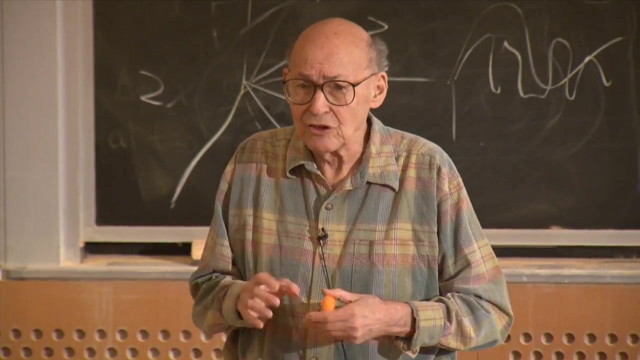 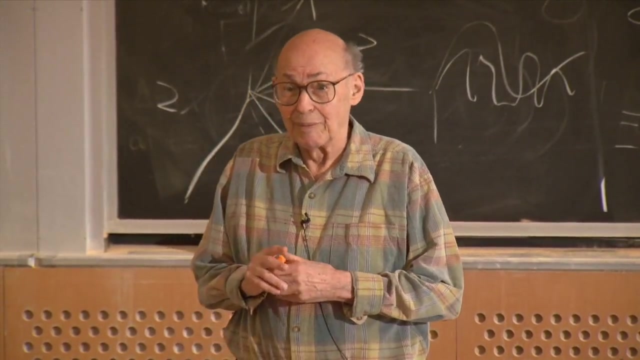 as a Fourier series with things of different frequencies. And then he said: or you should think of an object in a topological space, and each dimension is finding the boundary of the last one. And he went on for about six or seven And 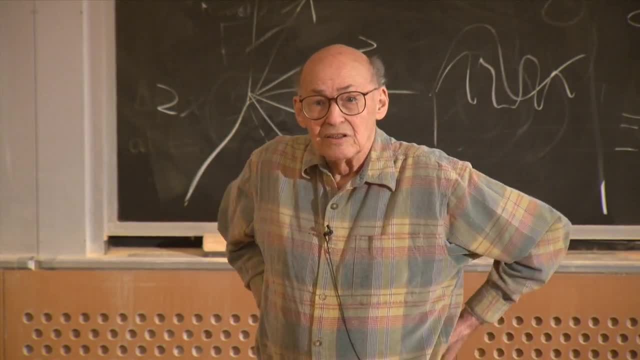 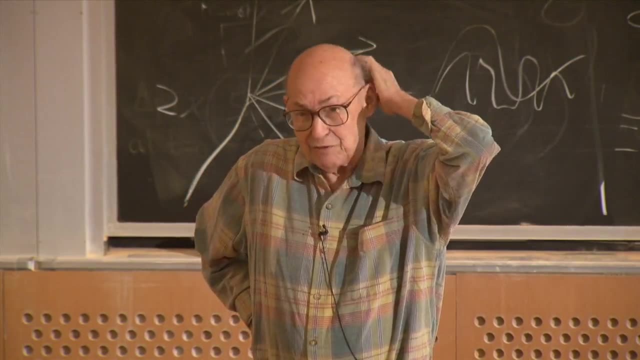 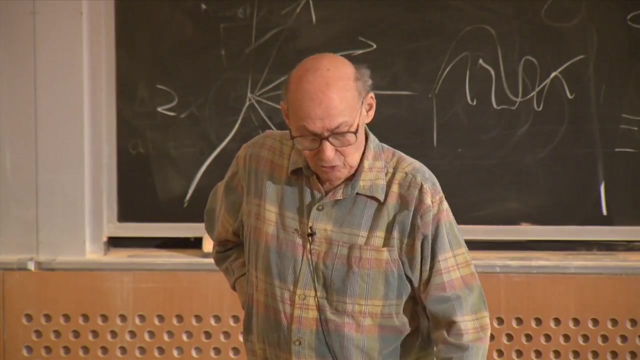 That was a great idea. That is well have seven completely different ways. And I remember I once had the same conversation with Richard Feynman And I said: well, how did you do that? And he said: well, when I grew up, I always, whatever it was. 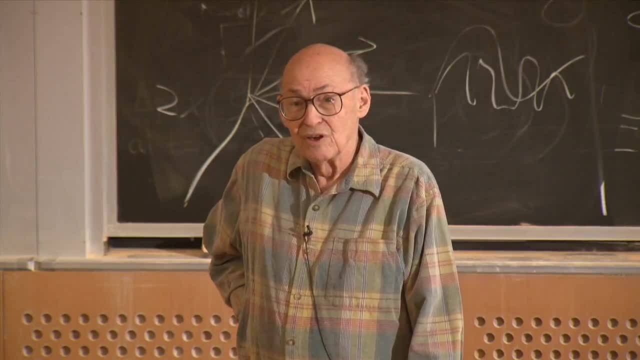 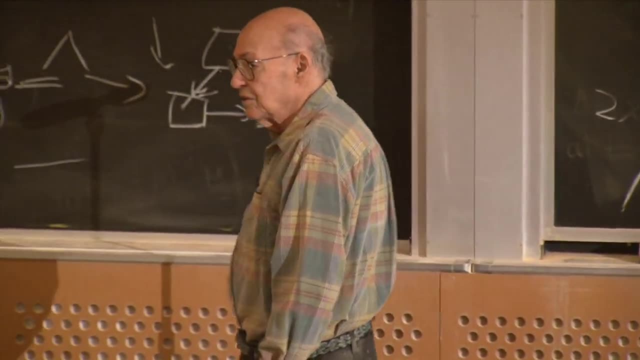 I always thought of three or four representations, So if one of them didn't work, another one would: What, Yeah? so my idea for somebody who wanted to: if you asked them about how to understand multiple dimension spaces, would say: read Flatland. 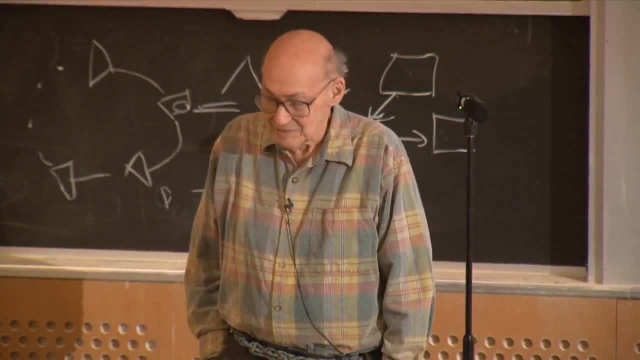 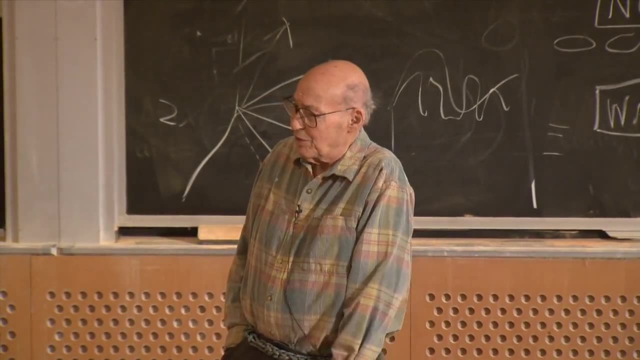 Read Flatland, Because that would give you the analogy right. Once you have that analogy, then you could. it would be easy to extend it to other dimensions. Oh good, Has anybody written a 4D Flatland where you make fun of the 3D people who? 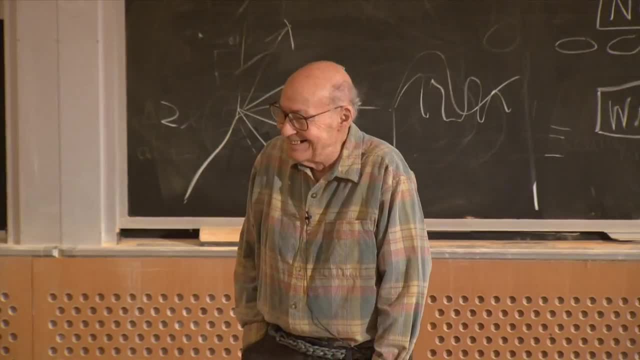 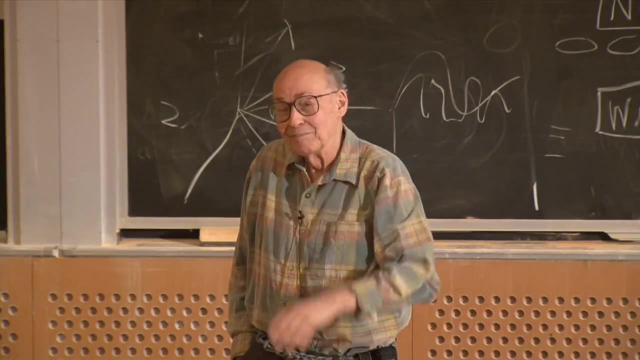 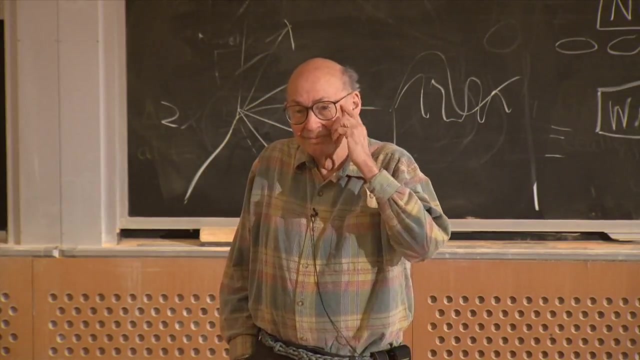 they can't get out of a paper bag And so like there will be some events that maybe will prove that. So, for example, in my case, when I do a lot of math, I when I try to talk to people, it's very hard. 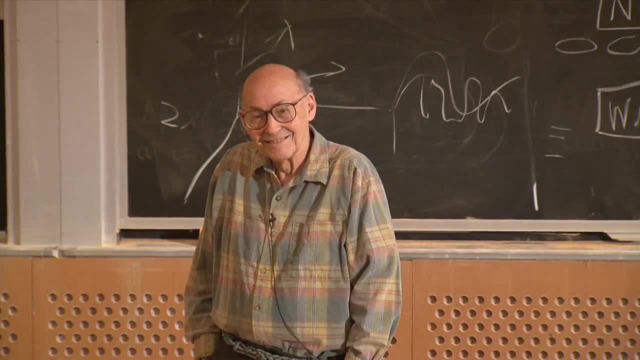 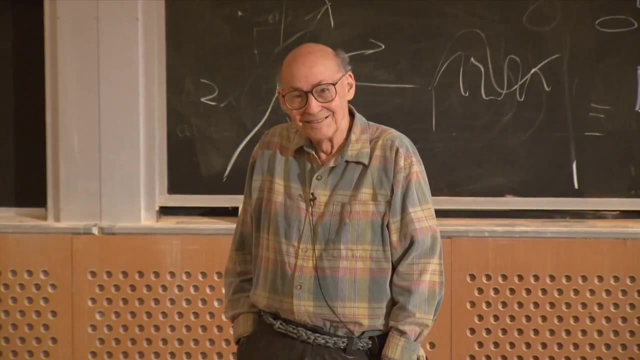 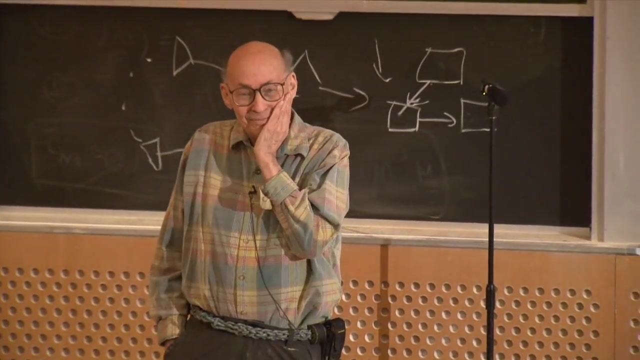 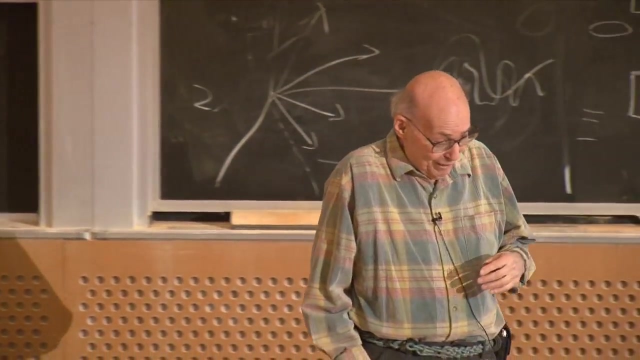 And like maybe I'm my representation of, like solving problems in math, And people tend to get better in math if they, Because they are optimizing their representation of math, And that would be the case. I think I understand the problem. 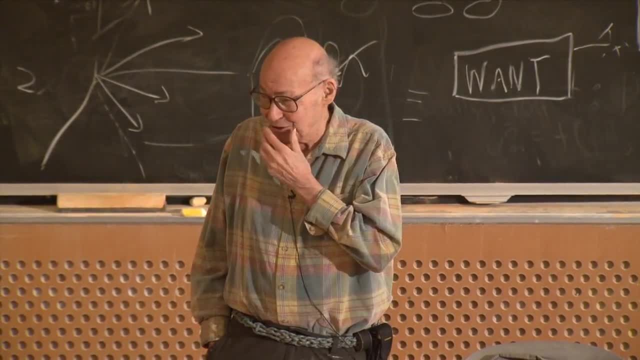 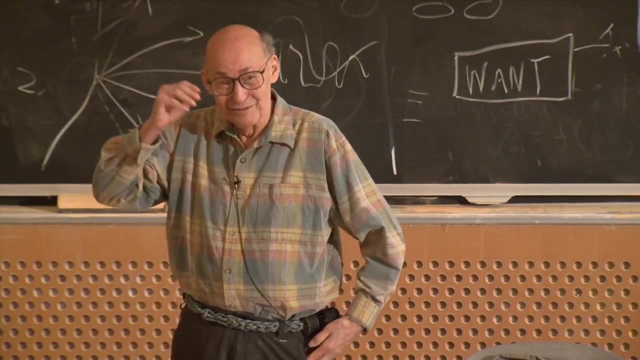 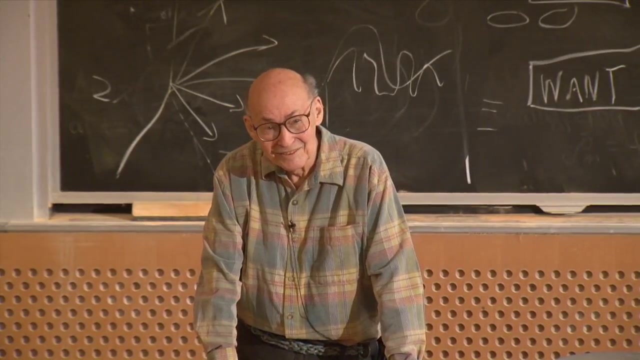 But I don't think I have any friends left who are not mathematicians. That's what happens if you live in this place long enough. Yeah, I feel like. So that's one way they're doing better. I feel like the other way they're doing better is they. 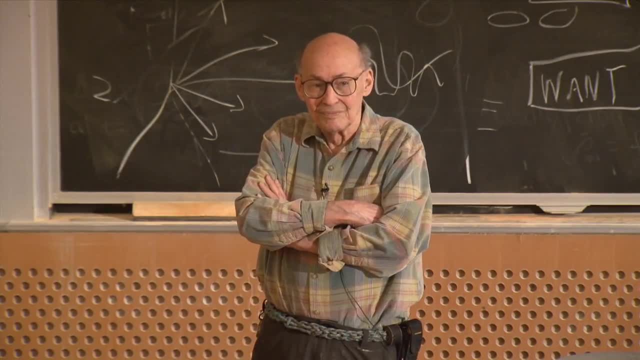 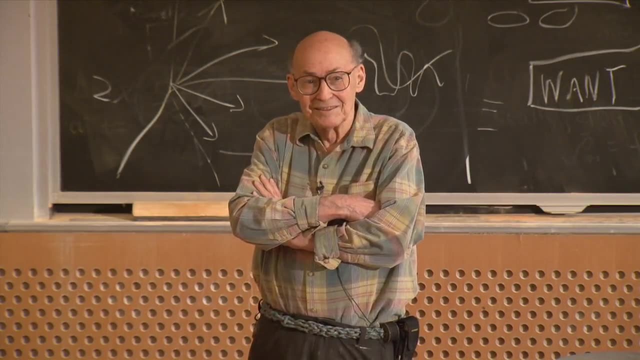 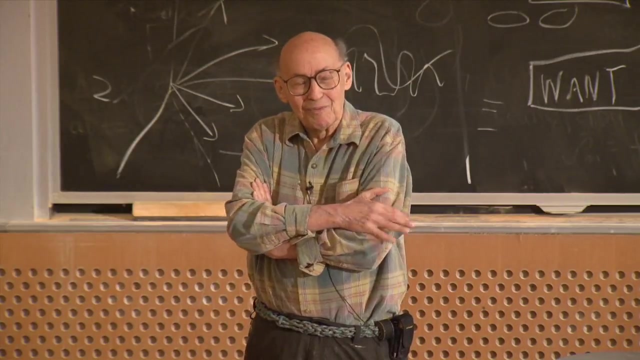 you know they like objectify things that we don't objectify Like it's, it's, it's like the. you know learning how to learn better idea. Learning how to learn better, to learn better, Like. so it's one thing to like know what the. 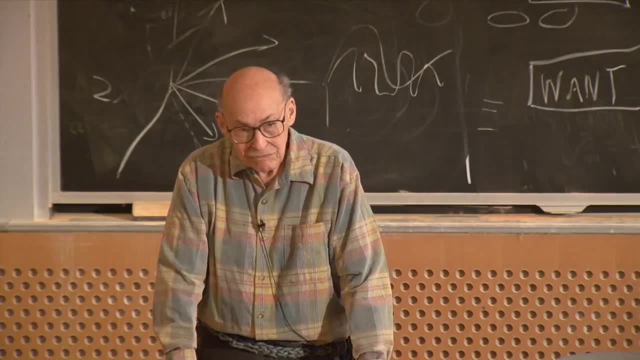 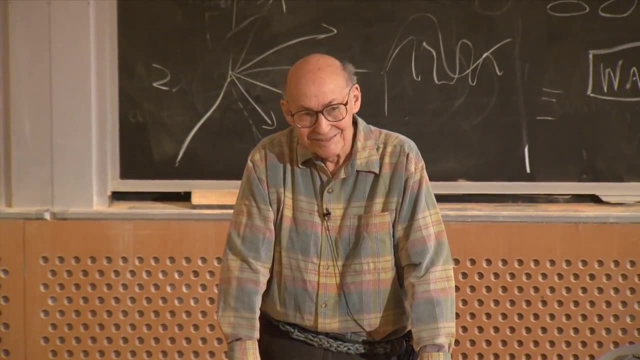 what the right representation is. We're predicting the problem with like the right method. It's another thing to like optimize that process. So like, what process did I use like in finding that representation? And then they make that into a concept. 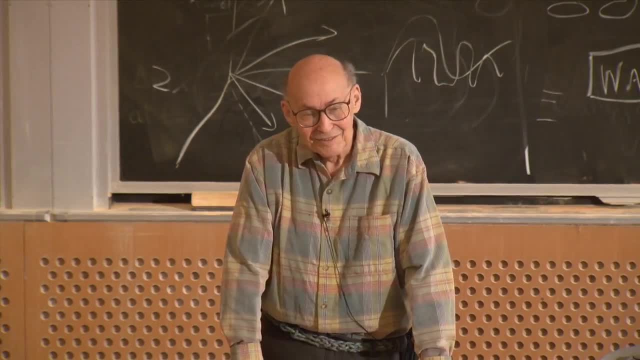 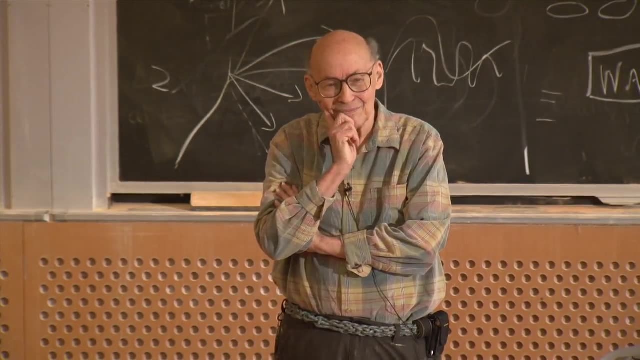 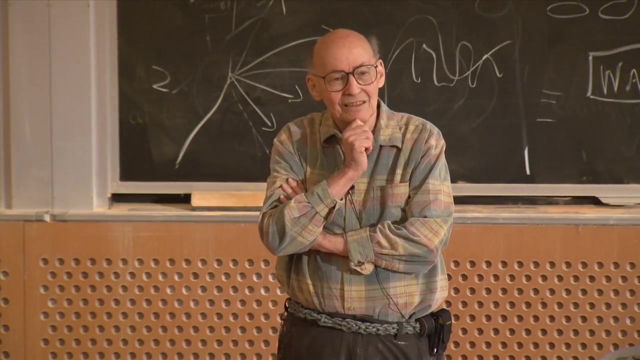 And then they have a lot of this kind of concepts. Have you ever helped somebody to learn better? Yeah, What did you tell them? So she, she had trouble with you know she had trouble with basically like true truth tables. 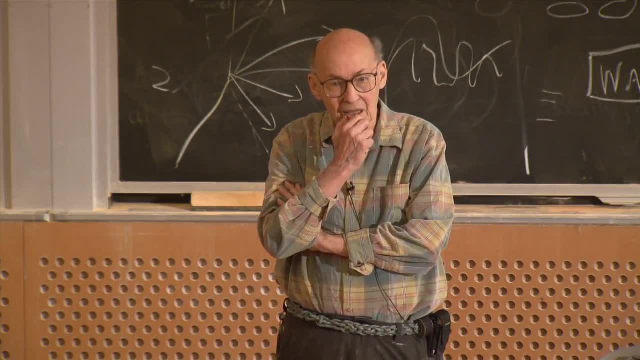 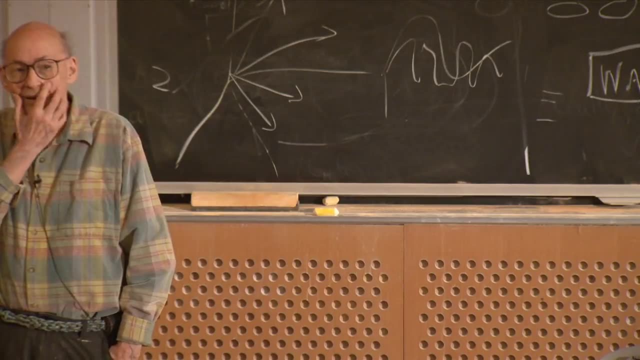 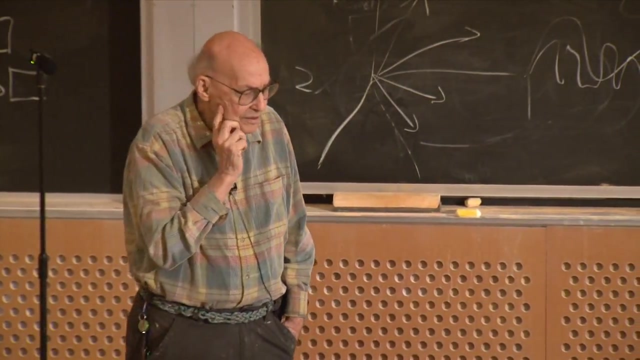 something like that: Uh-huh, Like and more and stuff like that. So she like her, her way of seeing the problem is to make a chart And I forgot what I told her. I told her to kind of like map simple problems. 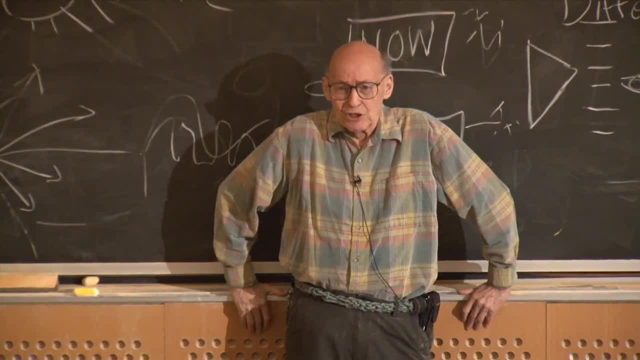 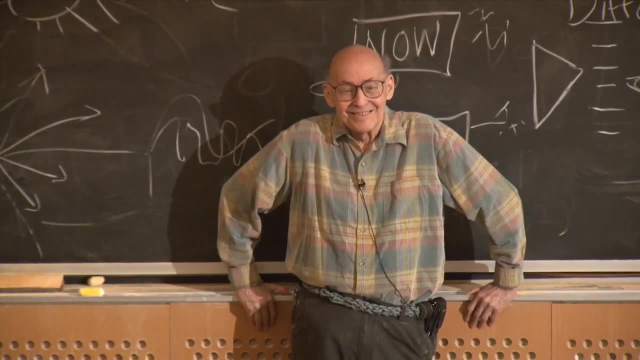 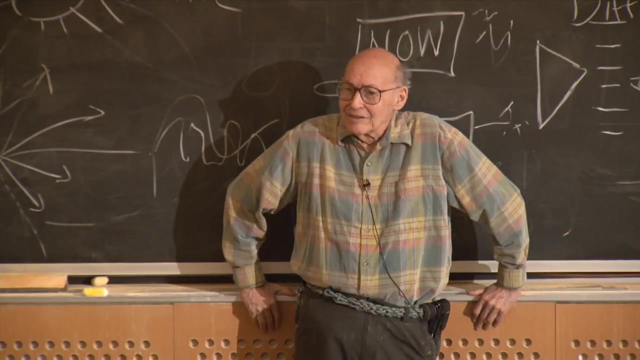 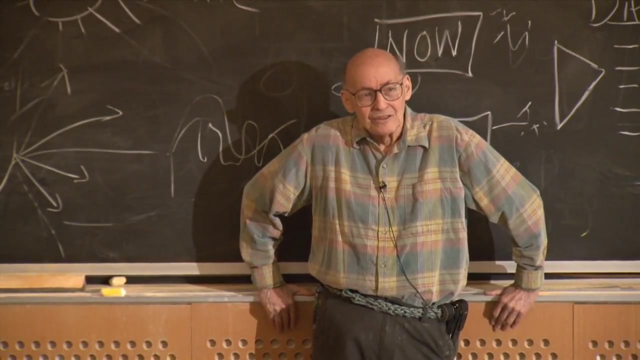 You know, maybe most people don't, you know, don't have, don't have the word representation in their, in their language. Is there any place in grade school where you, where you actually talk about what's your representation of acceleration? 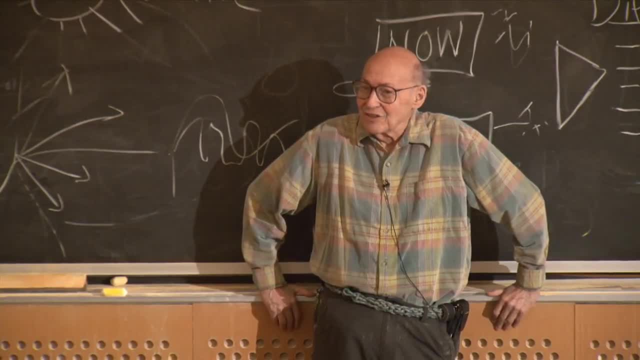 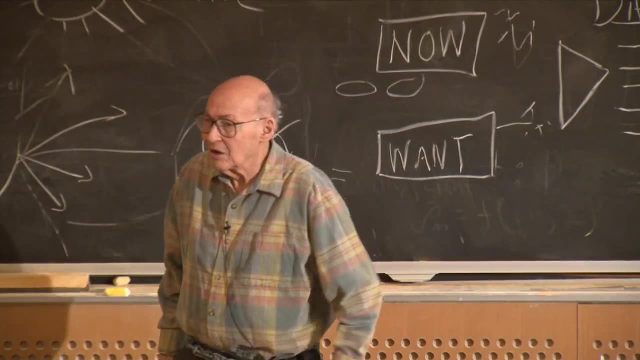 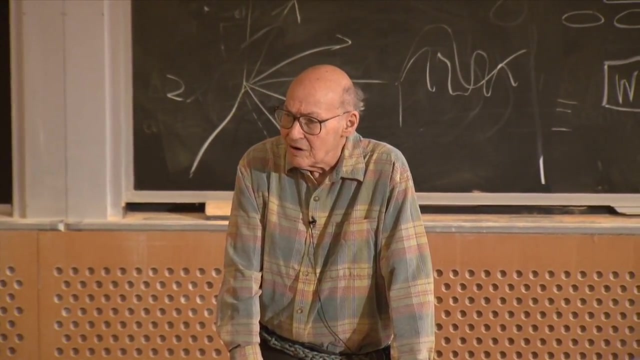 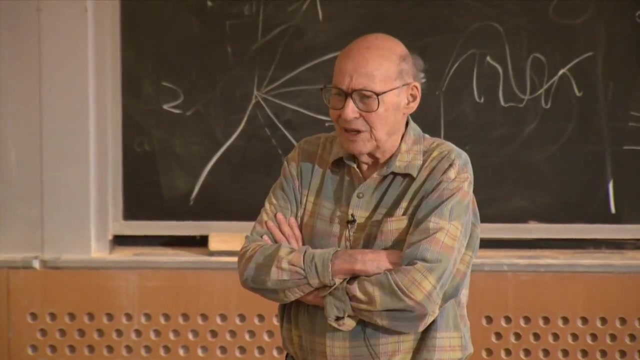 Is: do we teach that word as part of any subject? Parts Here, Here, Uh, Drawing some vase or something like that that will ask you to represent it. MARVIN MINSKYI- Yes, But it's hard to get out of. yeah, OK. 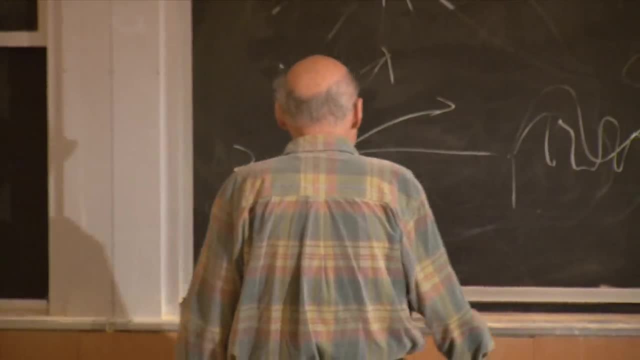 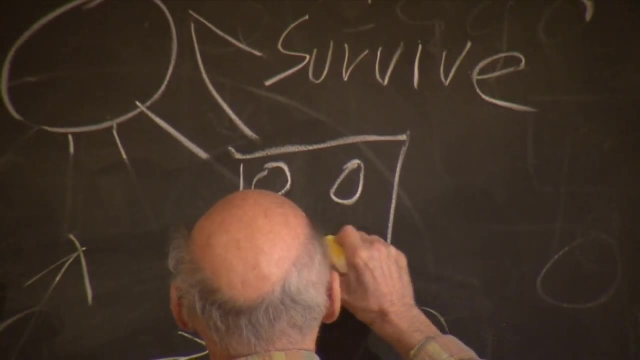 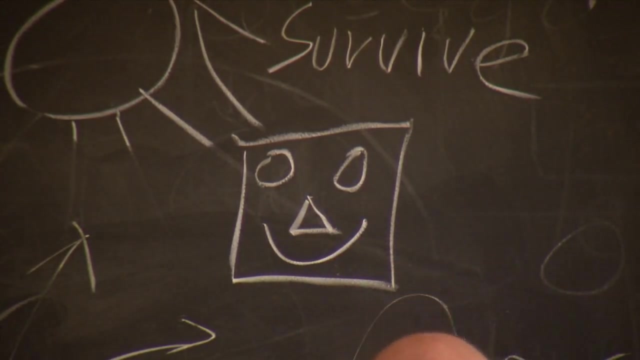 So they're radically different representations of. Maybe that's MARVIN MINSKYI- Yes, I don't know. If you have an idea that there's something maybe to correct the picture. MARVIN MINSKYI- Tinker toys. 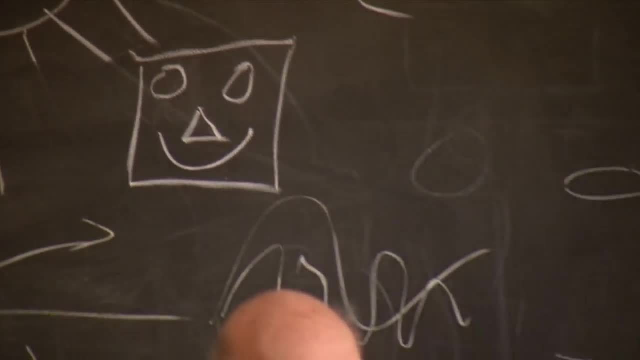 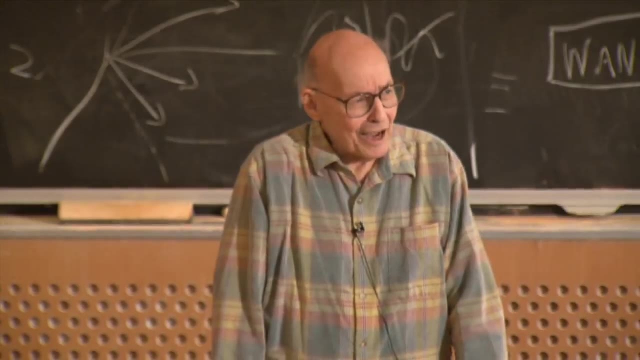 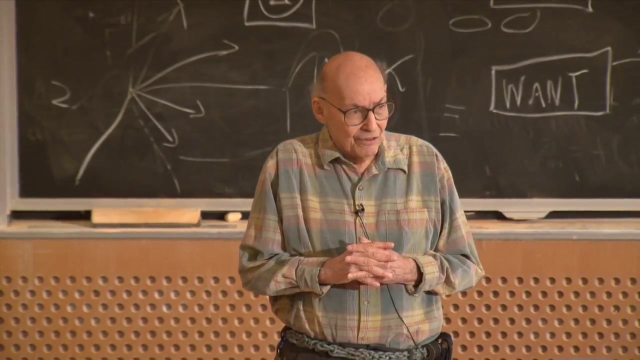 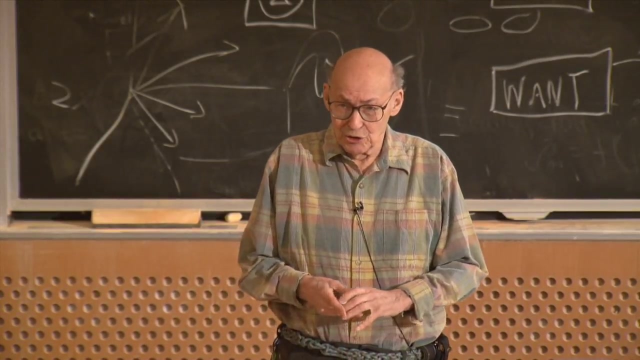 Tinker toy. Yes, that's to represent physical structures as tinker toys. Yeah, I wrote a little article complaining about the popularity of LEGO as opposed to tinker toys- MARVIN MINSKYI- Tinker toy- Because the children who grow up with LEGO 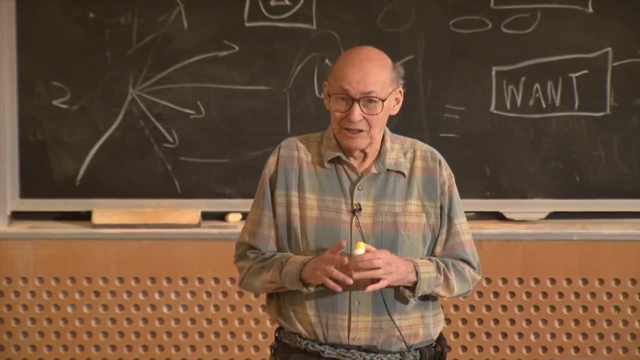 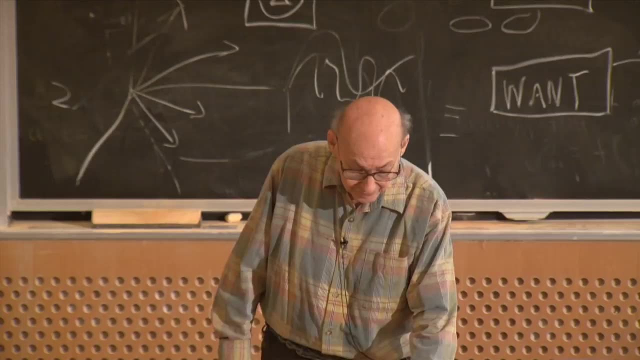 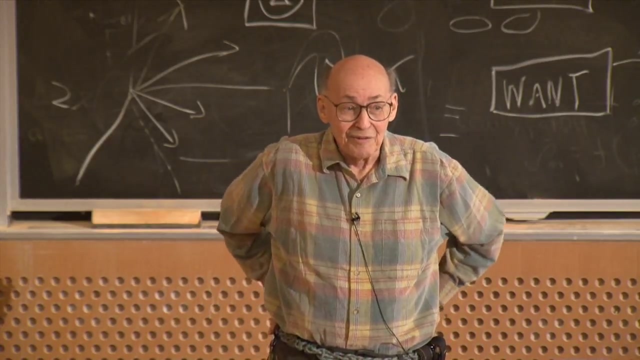 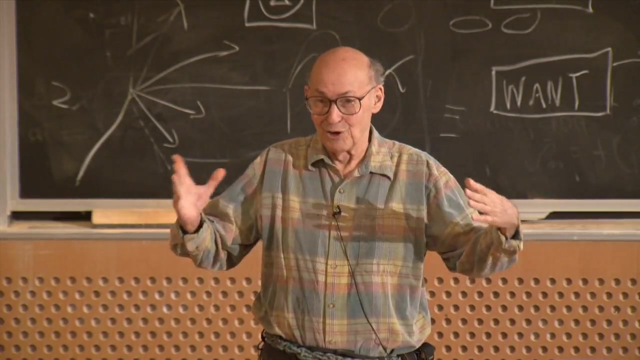 can't understand how to make something strong by making a triangle. So I sort of had the conjecture that, although those people could build all sorts of wonderful houses and things, they ended up deficient in having the most important of all: architecture. MARVIN MINSKYI- Yeah, 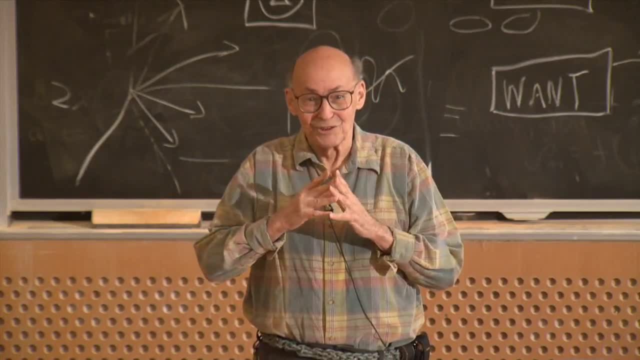 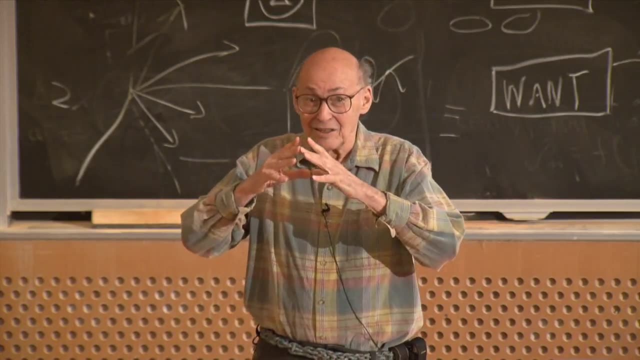 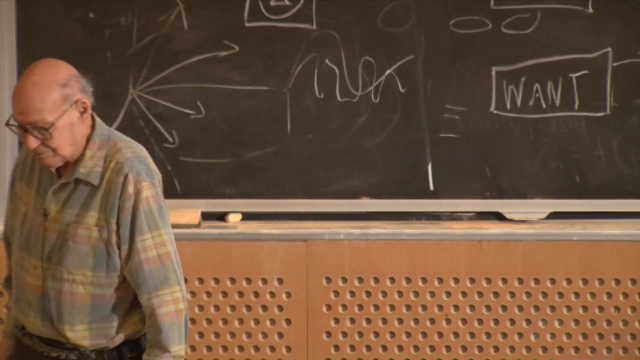 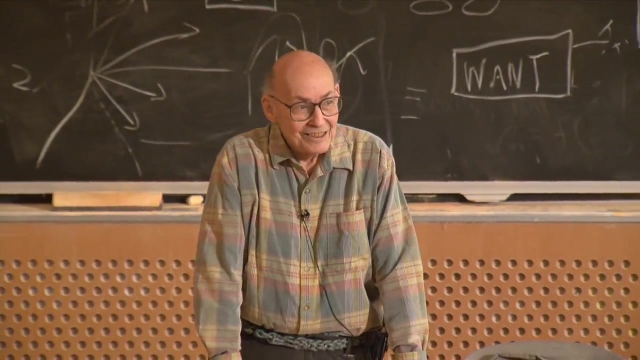 And they're not really architectural concepts. A triangle is infinitely strong because I mean, you can't alter a triangle without breaking it, whereas I don't know what That's a run-on sentence I can't finish. This explains the deterioration of society. 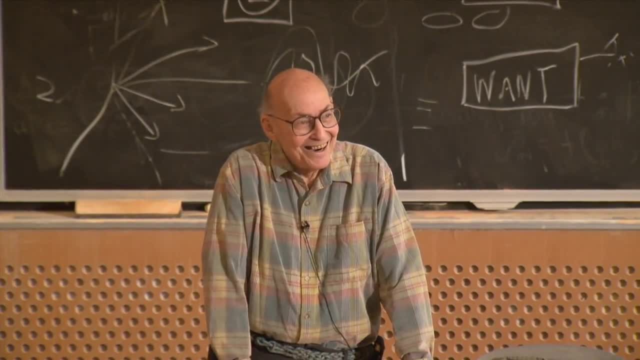 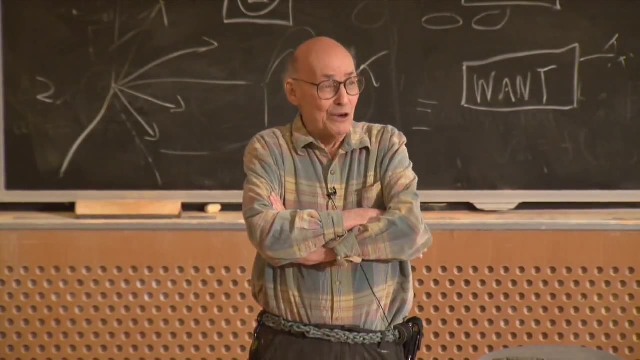 Marvin, We don't have a, We don't have tinker toys and we don't have chemistry sets with chemicals that make explosives out of them. MARVIN MINSKYI- You have to go to terrorist school to get a good education. 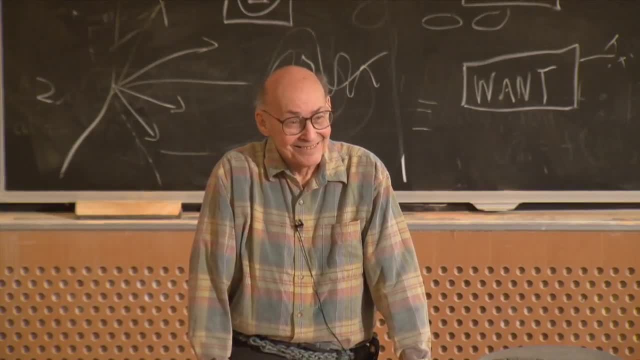 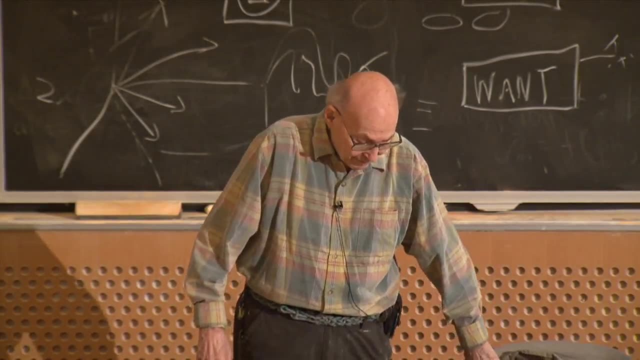 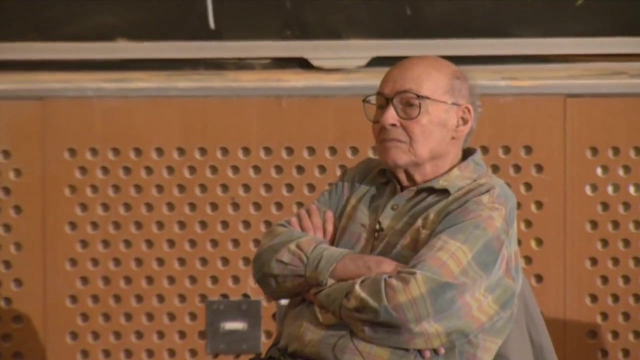 So actually, in this conversation about being good at things and learning how to learn better, I think that a point that sort of relates to this idea of tinker sets and playing around with things. I think that it's not enough to simply come up. 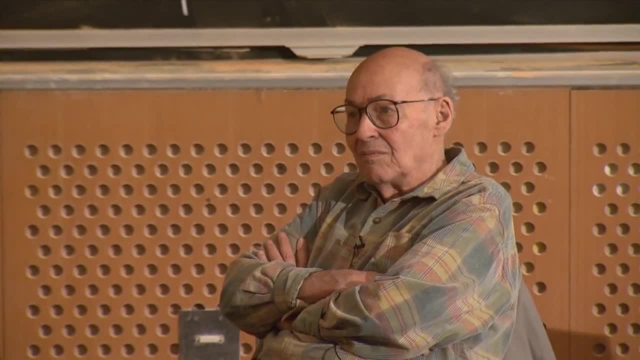 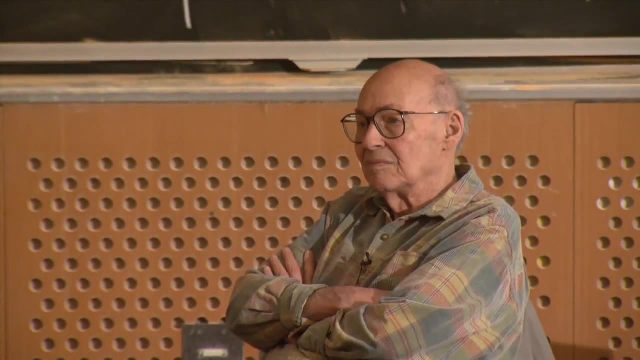 You have to really come up with the best representations of a concept. In order to actually be good at something, whether it's music or speaking a new language, you have to not only understand it conceptually, but you actually have to gain a certain amount of fluency. 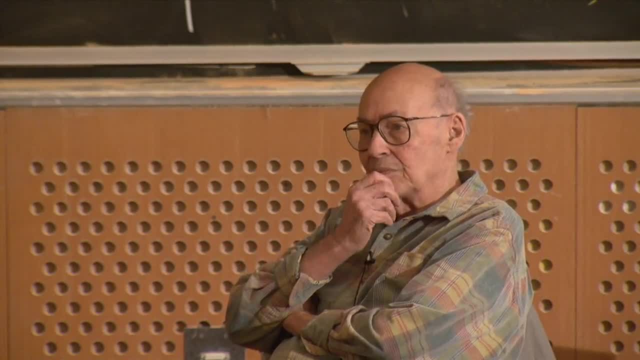 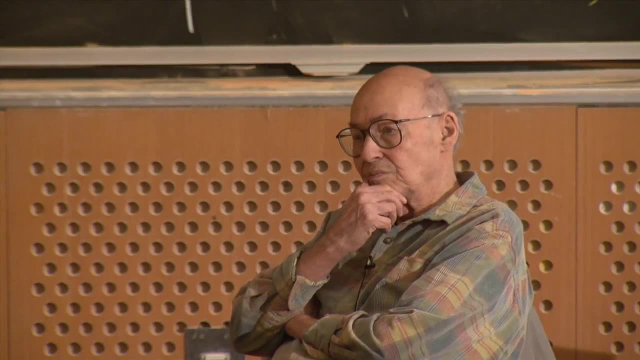 And to gain fluency, you do have to play around with the thing a lot, whether it's turning it around in your mind or practicing it physically. So in the case of math, it's like: yeah, you can come up with all these different representations. 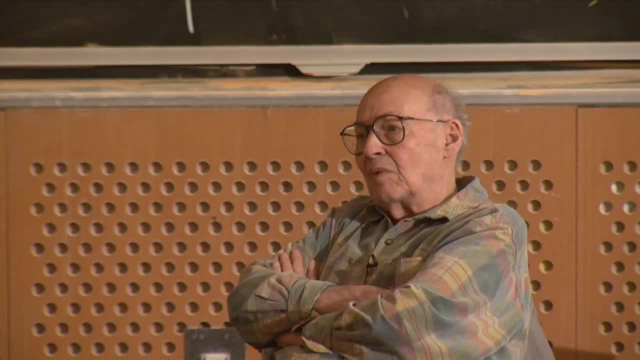 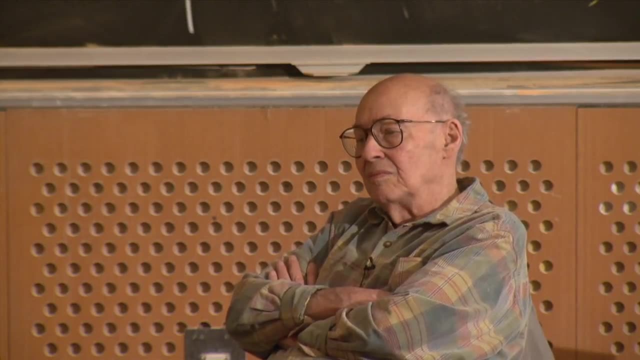 of it. And that's the first thing. The first step is understanding it. It's great once you understand it, But just because you understand the concept, like on the conceptual level, it doesn't mean that you can actually know when to use it. 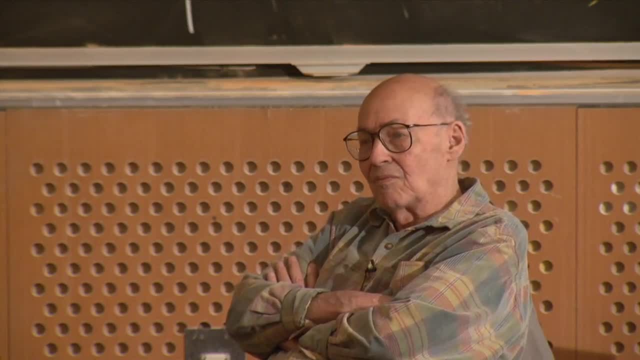 or know how to use it when you're solving a problem, And similarly for music, like, say: I guess I'm mostly talking in the case of improvisational music, when I'm trying to speak something with the music. So I have something that I want to say. 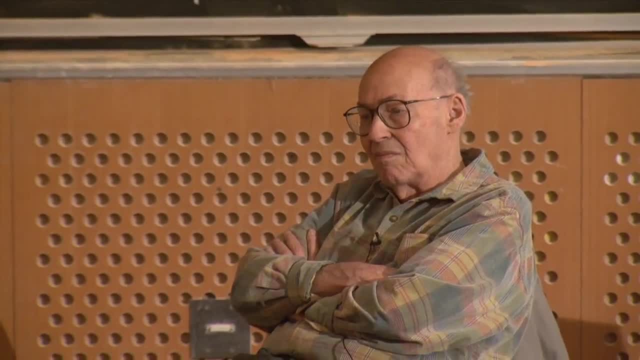 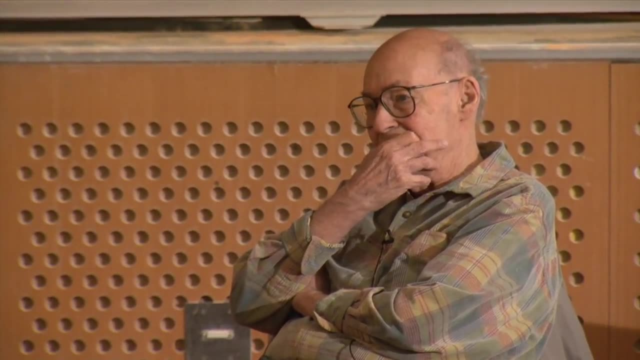 And maybe it's something that's sort of low level. I'm trying to resolve one chord, to get to some sort of cadence. Now I can have multiple ways of resolving the chord And in order to do this, I have a vocabulary. 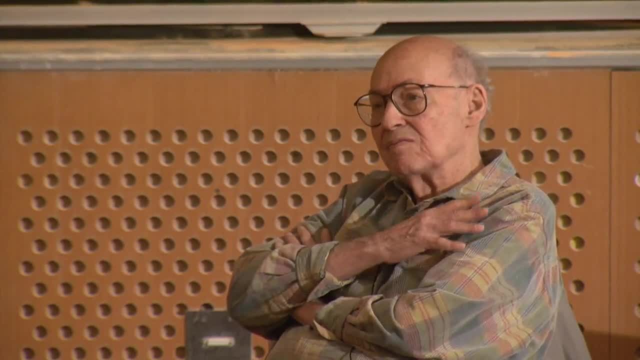 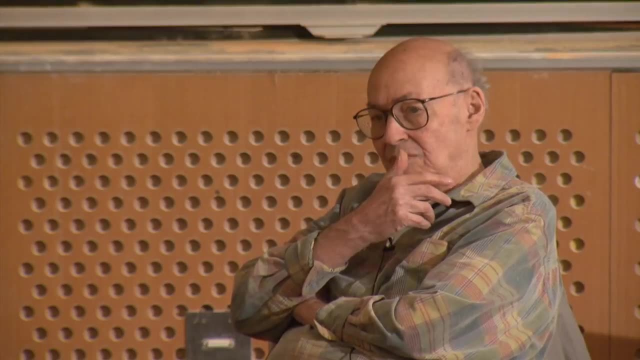 of the different ways, And if one way doesn't occur to me when I'm playing the piece, I can try another way. But the important thing is that I have some way that I can resolve it in real time, or else my piece is never going to come out. 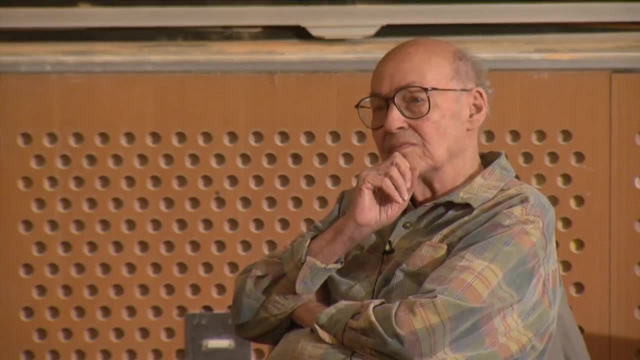 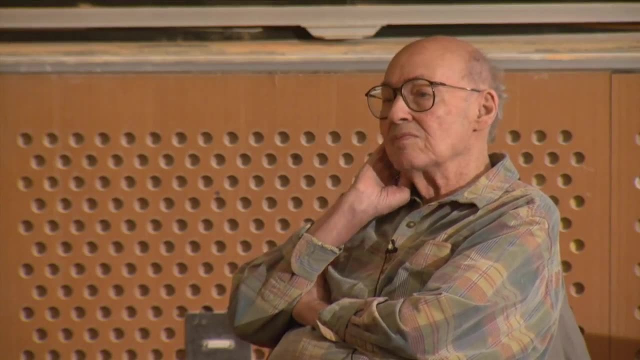 And then same thing about learning different languages or speaking different languages. In order to be able to speak or to express ourselves, we have to have not only understanding of the language, of the structure, but the immediacy of being able to access it. 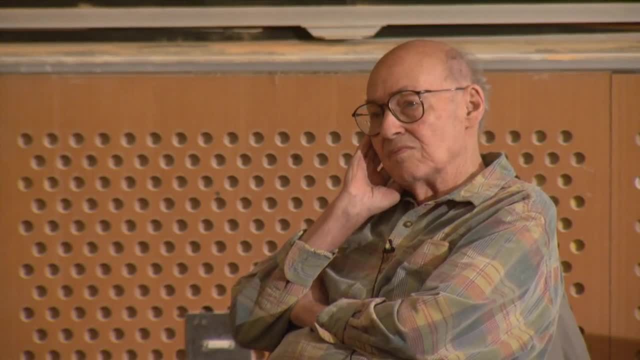 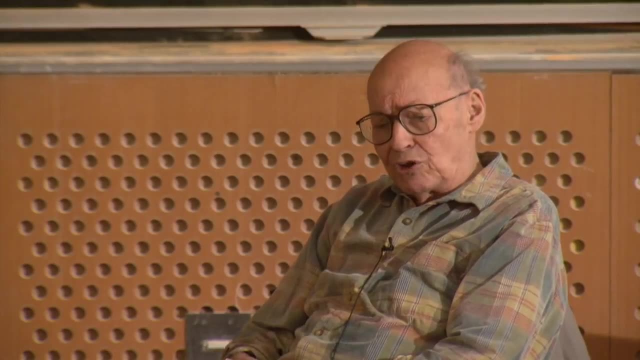 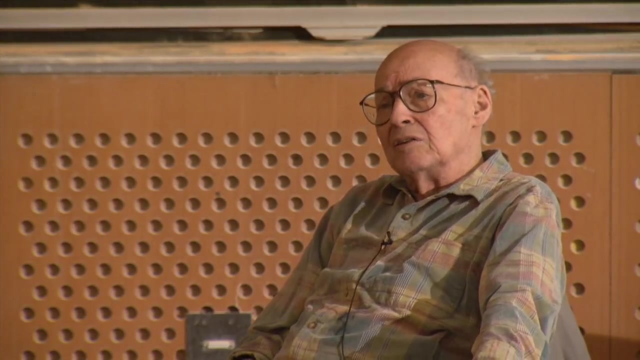 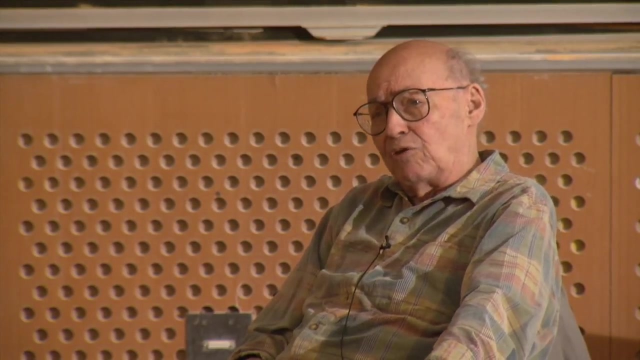 And that comes with practice, with tinkering, what have you? Well, maybe that goes in several directions. One thing about where in our educational system do we in grade school is there a place where you emphasize having several representations? Because I can't think clearly right now. 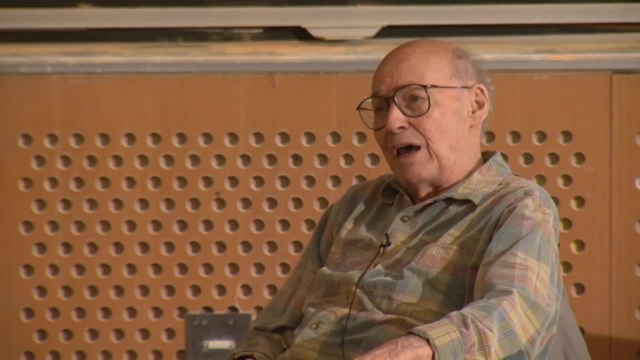 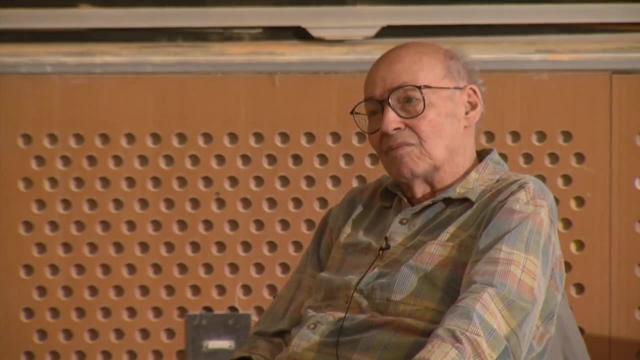 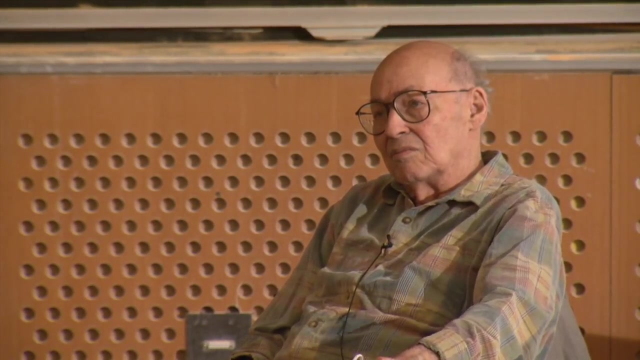 But it seems to me that you're usually trying to tell them the one best way And There's like: A, there's the idea of the one best way And B, there's the idea of reinforcing similar, the same process over and over again. 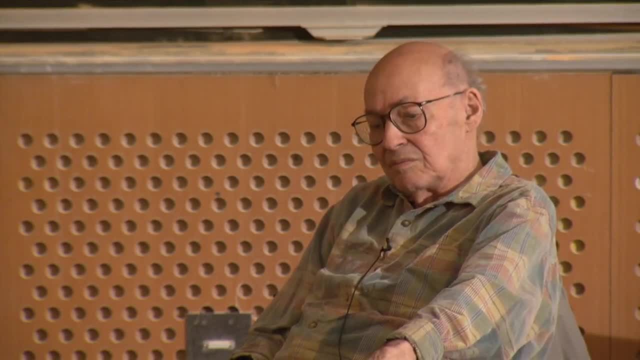 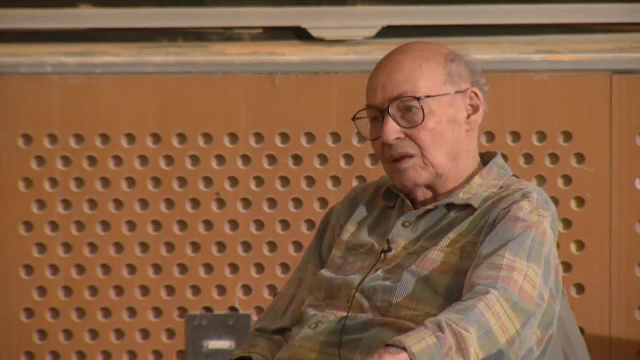 So when you learn math, it's like you learn this technique And you reinforce the technique by doing a bunch of homework problems that are essentially like repetitions of the same thing, Whereas I think a better way of doing it well, two better ways. 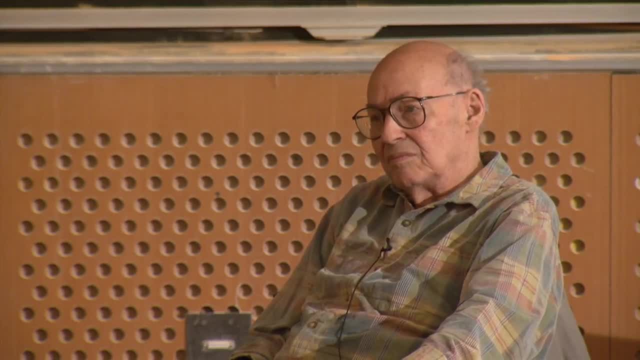 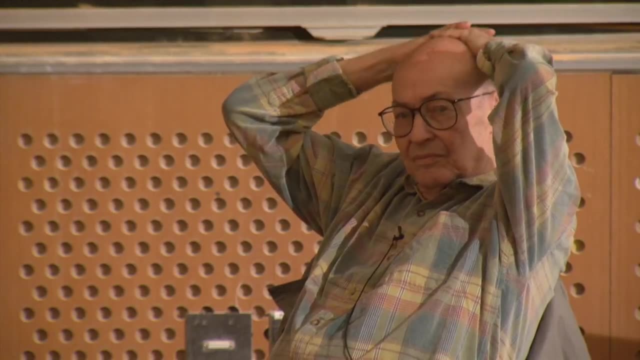 A: you have multiple representations And two: you create problems where you make people like traverse paths differently, And different people may have different solutions And each time you solve the problem you may have a different solution, But the idea is you lay out like a whole network of paths. 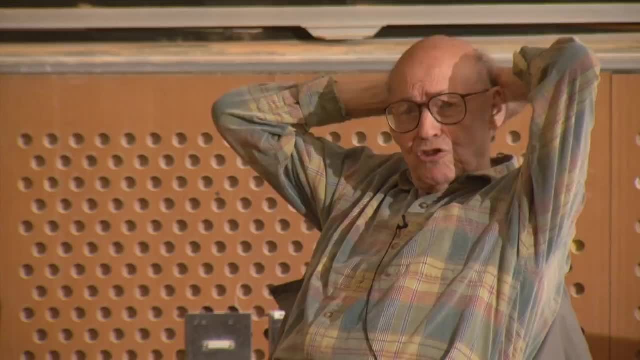 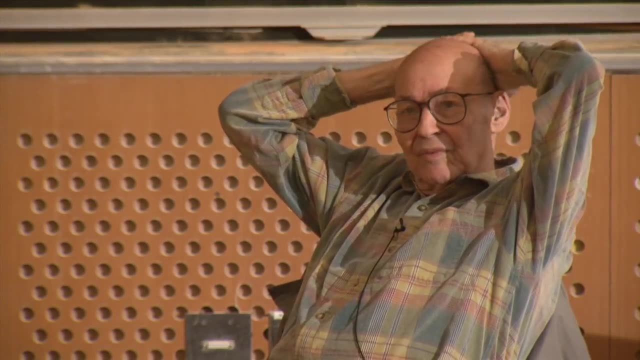 in your head to solve any given type of problem. So where in grade school do you ask children to solve the same problem, Problem three ways? Can anybody think of? Is that part of the education? What It's the closest thing I can come up with. 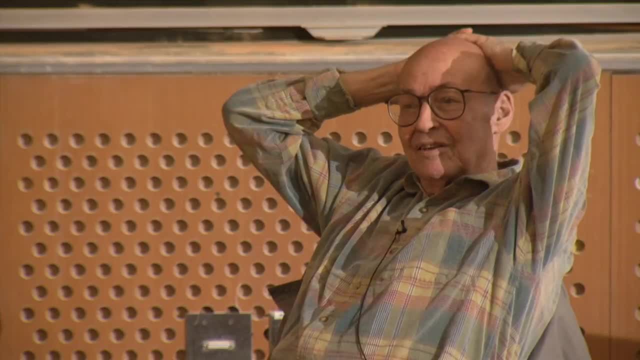 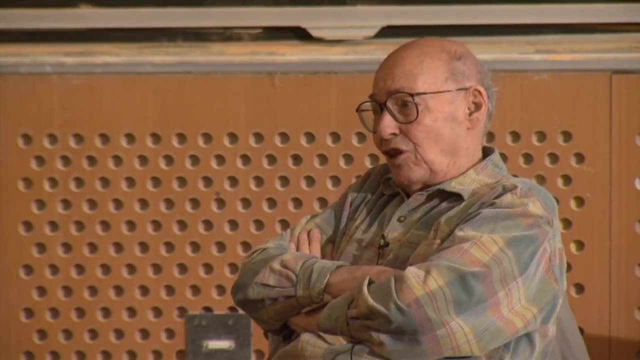 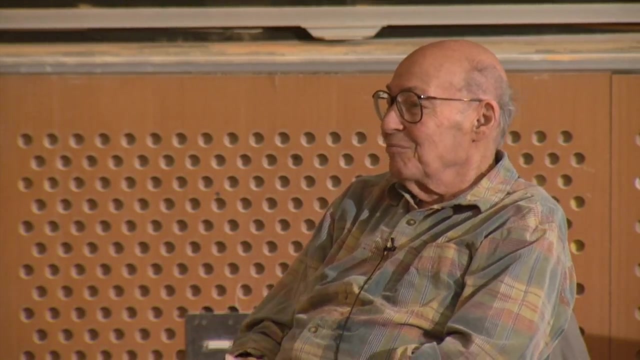 With fractions. What about literature class? They ask you for interpretations of novels. Yes, Yes, I bet there are things that happen in literature that don't happen anywhere else in the curriculum, But they probably don't have most children. don't transfer it. 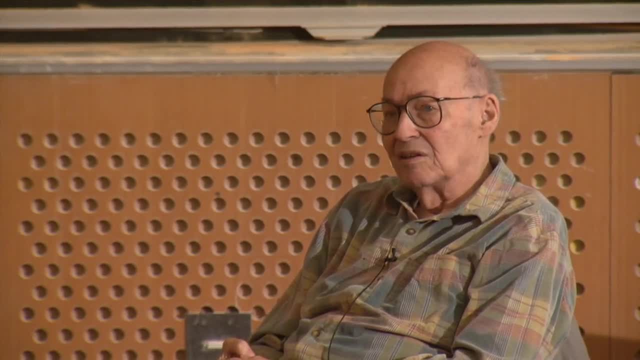 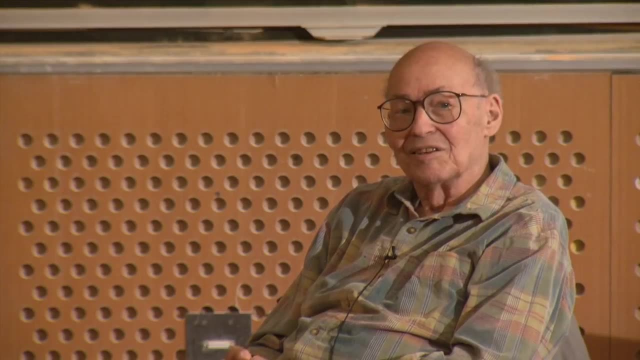 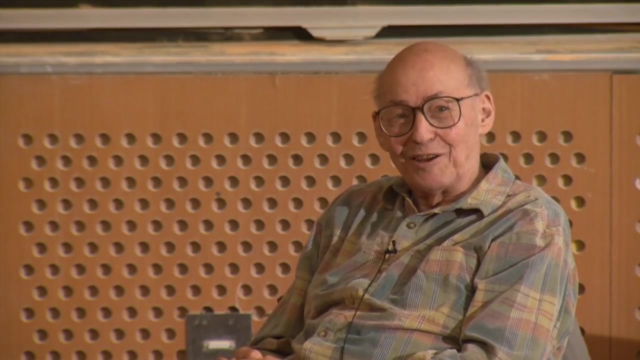 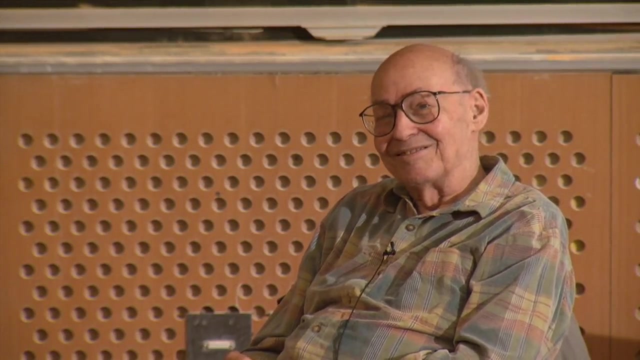 Well, when I was in China and learning math, when we try to find areas of certain geometric shapes, we always do it multiple times, like multiple ways In topology. whatever it is, you just make it into triangles or simplexes. So that's a very strange subject. 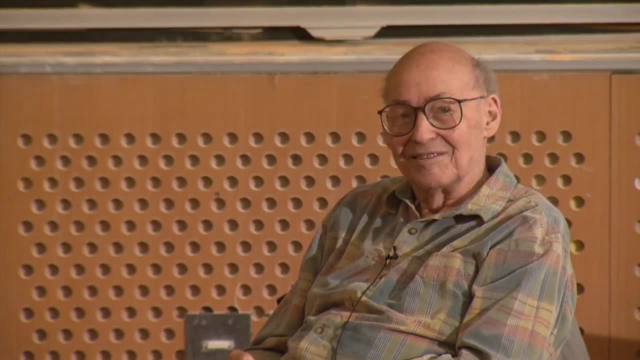 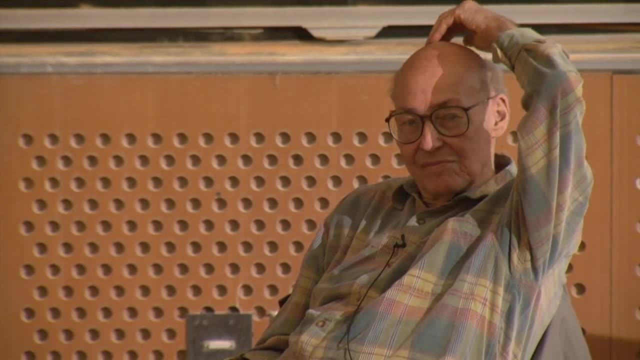 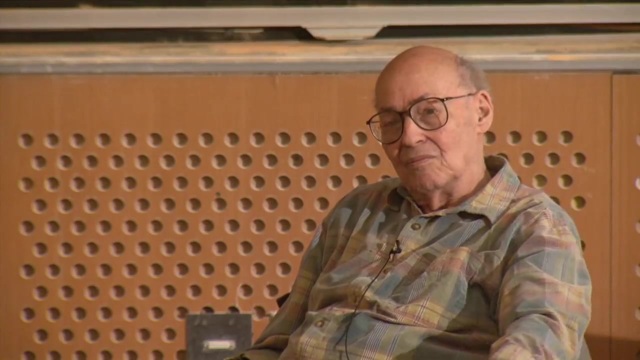 Maybe one reason why topology is so nice is because you can think about it. You can think about it as logical concepts like cosets, You know, if you count all the different points, stuff like that, And then you can imagine it as like a picture. 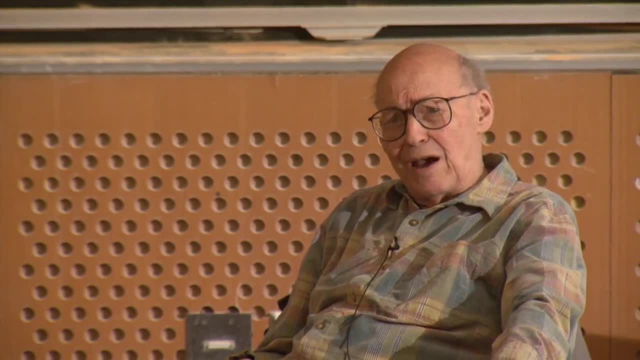 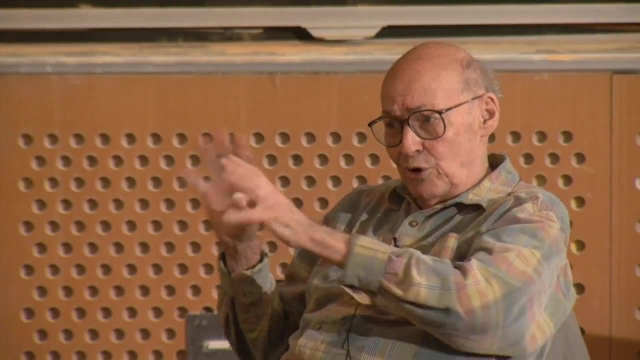 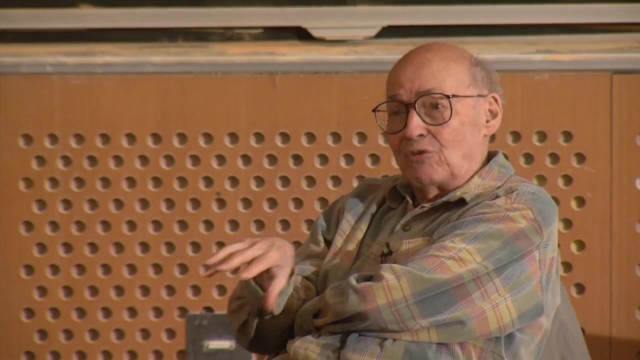 Cosets. Where in real life do you have duality? That's a nice feature of a lot of mathematics. There's whatever you're doing. in some fields there's a dual way where you look at the space of the functions on the objects rather than the objects. 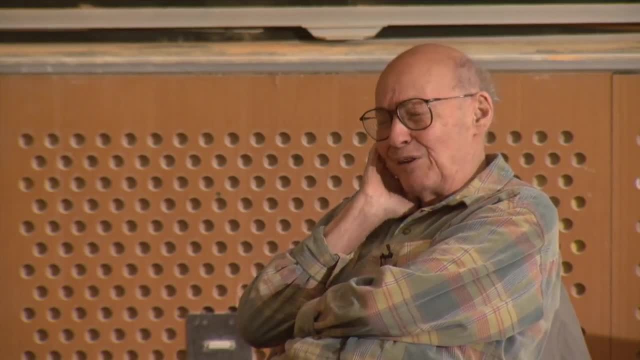 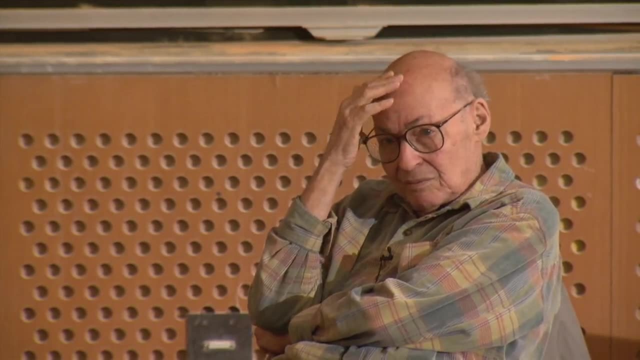 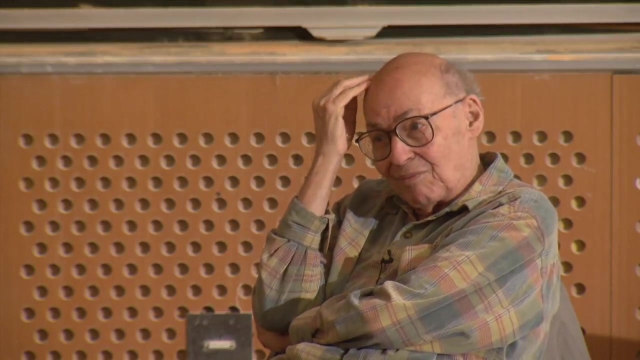 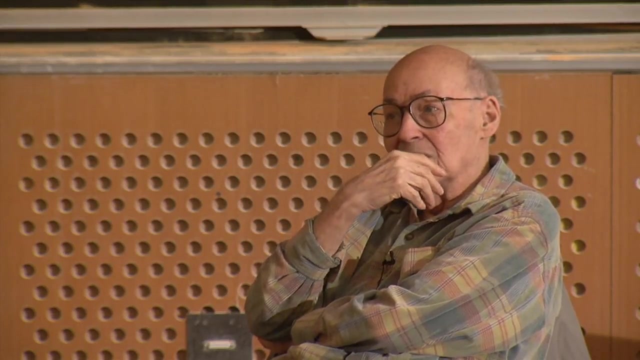 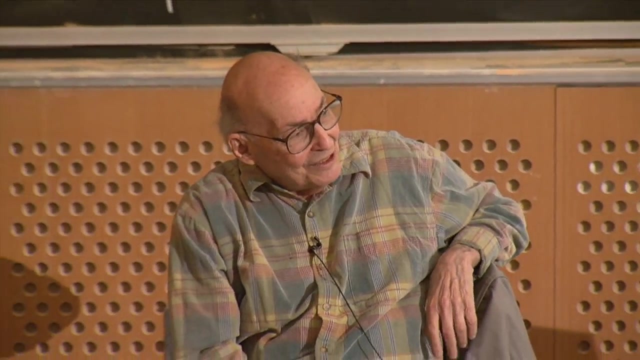 I can't think of any. Where is that in the loop? Is there anything like that in real life? Because in mathematics a lot of problems suddenly become much easier in their dual form. You just change everything. I've been facing one way. 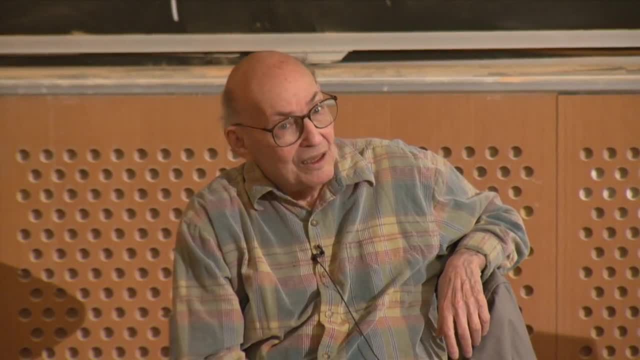 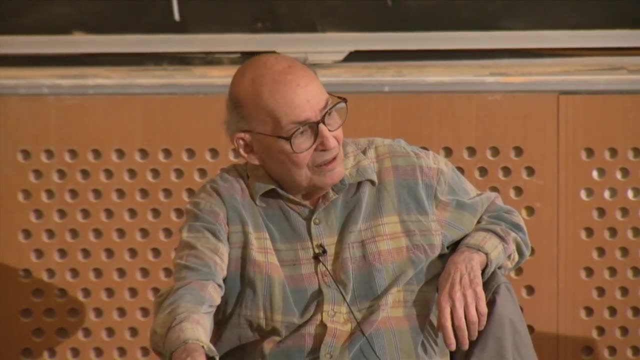 I was just, I guess, a couple of points. You said: why is it difficult? Whenever I've struggled, I think it's because it's constructive And you have to hold a lot in your head. You hold the entire structure of almost a field. 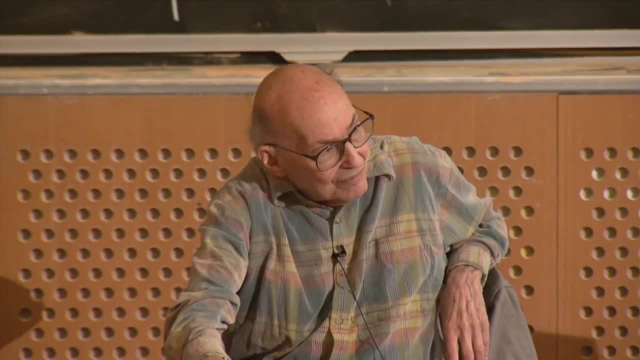 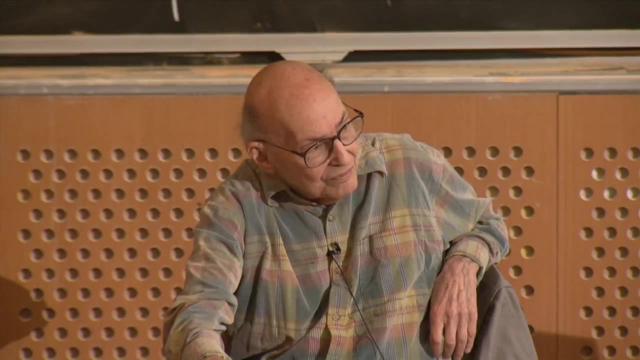 Because if you're learning algebraic topology, you're holding all of algebra and all of that most of journey. So sometimes it becomes It's difficult if you haven't abstracted at the right level. And what I found- I think my advisor was just really good. 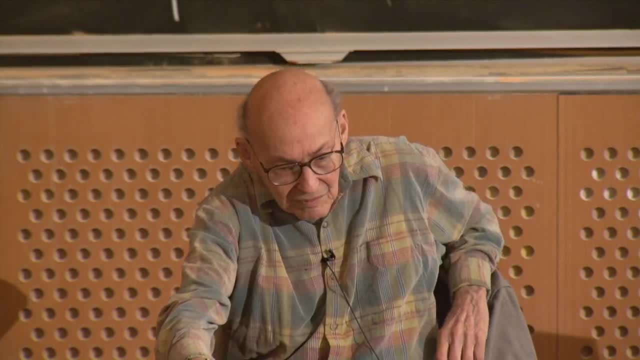 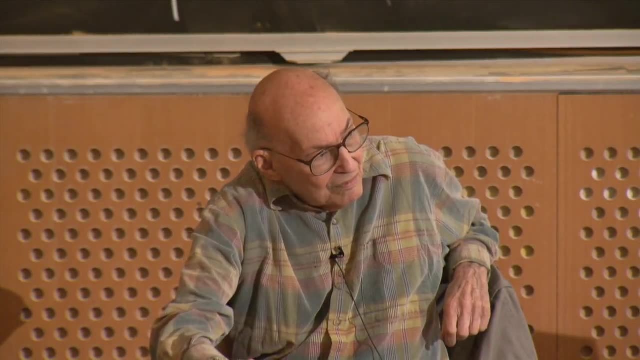 Many times he said two things. He says: really good mathematicians are really good at making analogies in mathematics And I was studying algebraic geometry. And he says: and really good, algebraic geometers can boil everything down to linear algebra. 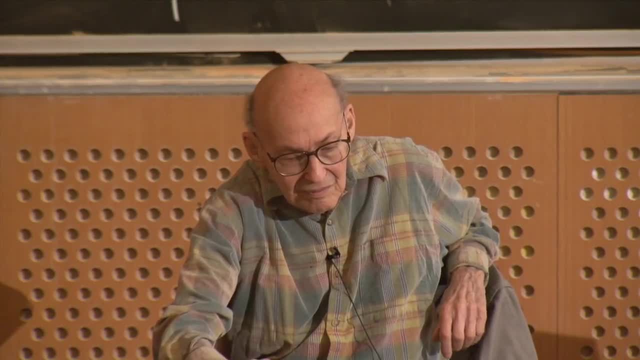 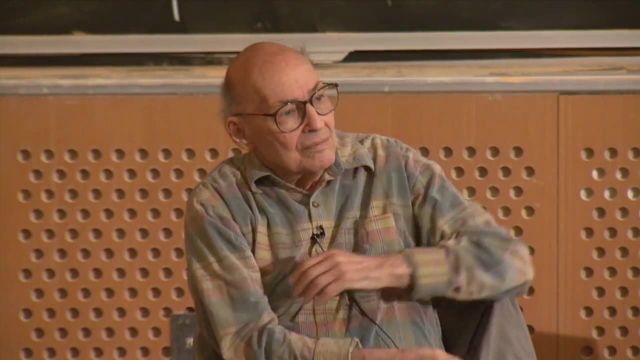 So he says: and you can only do that if you abstract at the right level, And he never gave techniques of doing that. But why do you think the difficulty is in that I'm talking so much about? I mean, an analogy is a relationship. 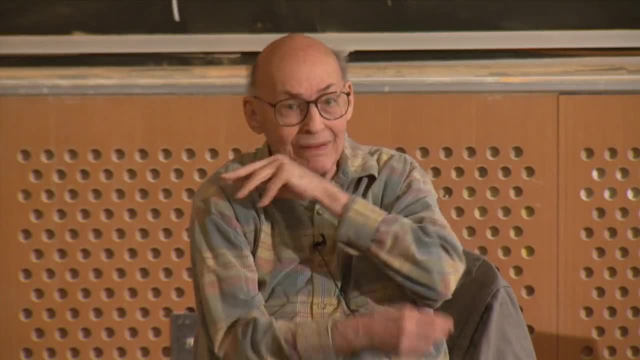 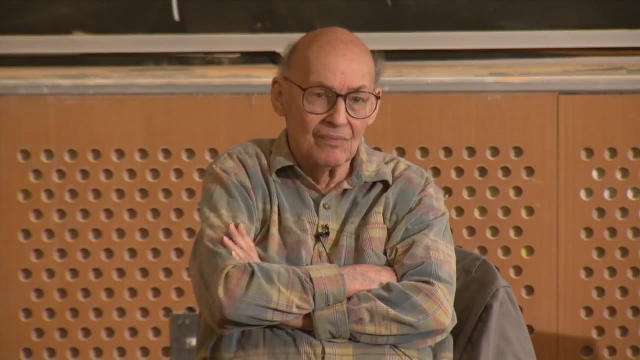 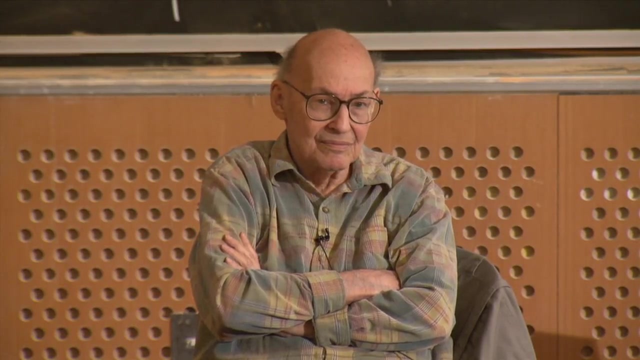 between two objects And if you're good at making analogies, you're a level beyond, a level above just looking at objects. You're looking at relationships of objects And, regarding the practicing thing, I mean, it's still related to representations. 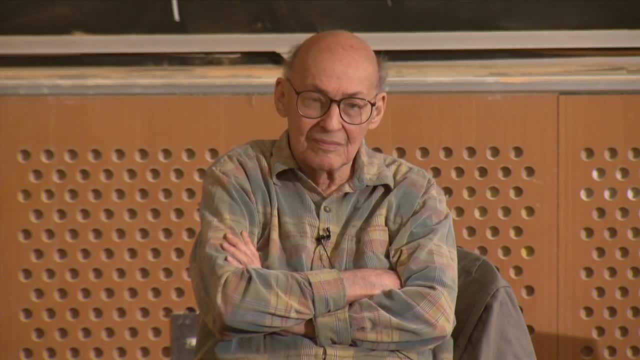 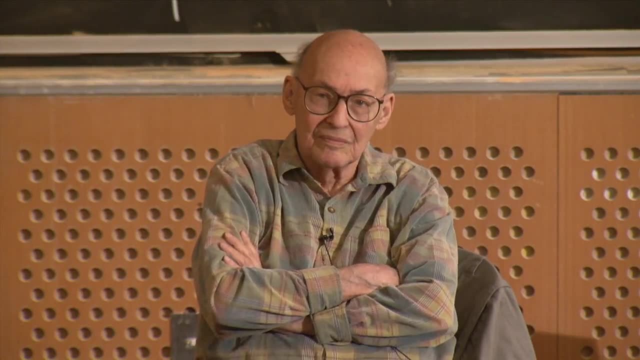 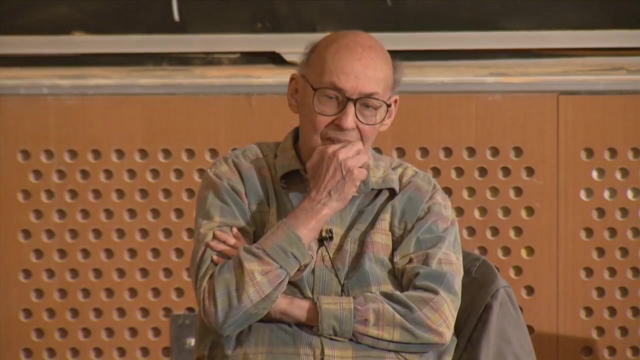 Because at each practice you're learning something new about like this type of thing, This type of problem, that make you better at identifying them in the future. And it's not like numerous practices- The number of practices doesn't matter to your ability of solving problems. 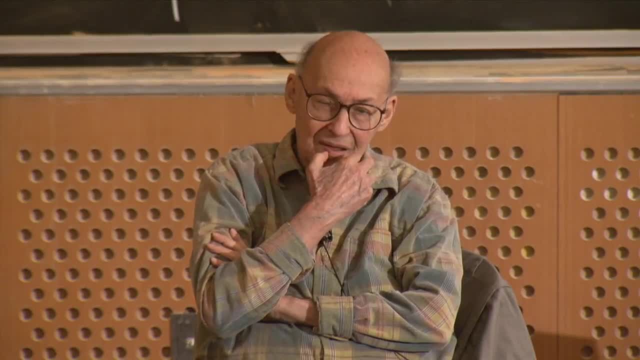 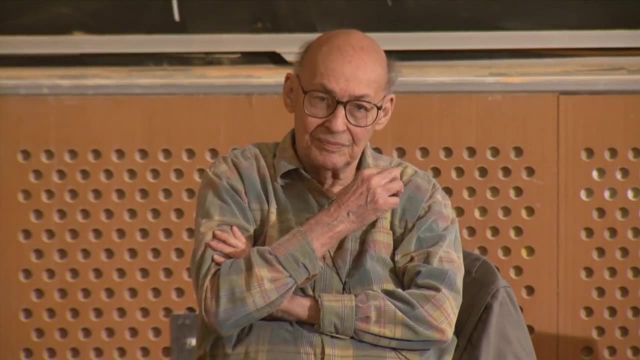 It's what you learn from each practice, If you can do a thing. once I have a friend who basically told me how to do math. It's like you look at a problem, you solve it once You go back and you think about how. 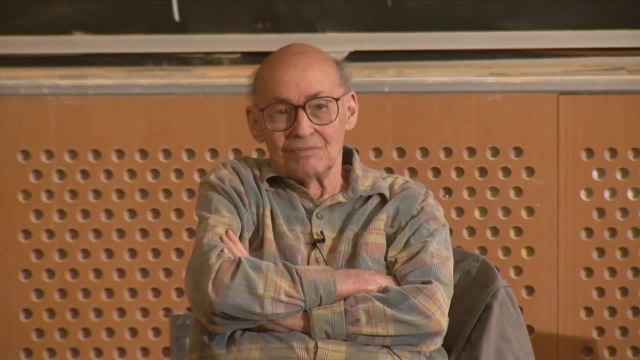 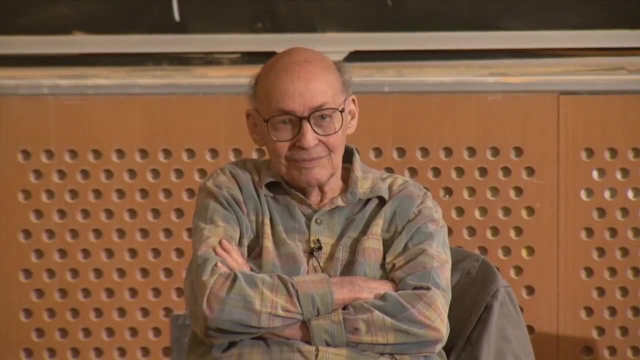 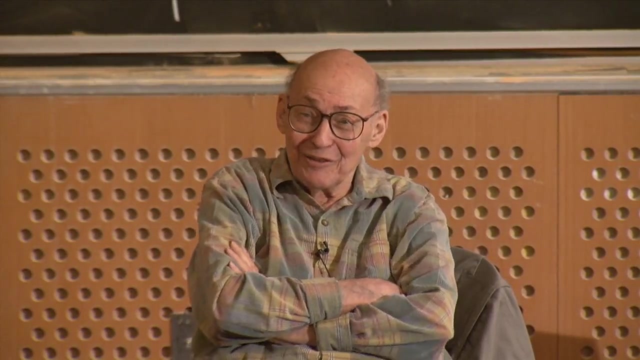 you solved it, like what's the process you used to solve it. So a good problem is, make up another problem like this: Yeah, That's essentially what you were learning when you were practicing. It's probably too hard to grade. You can't teach things. you can't grade in the modern 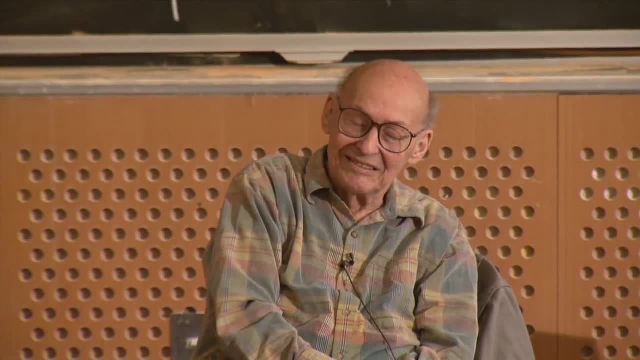 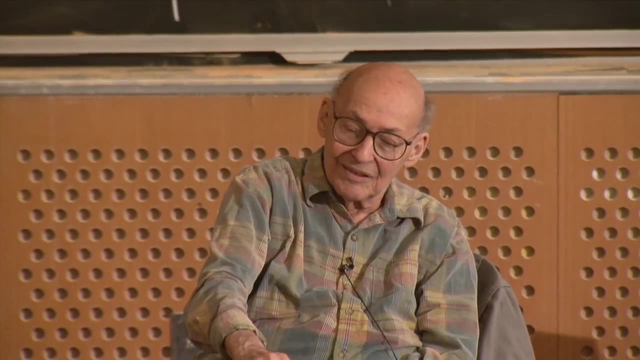 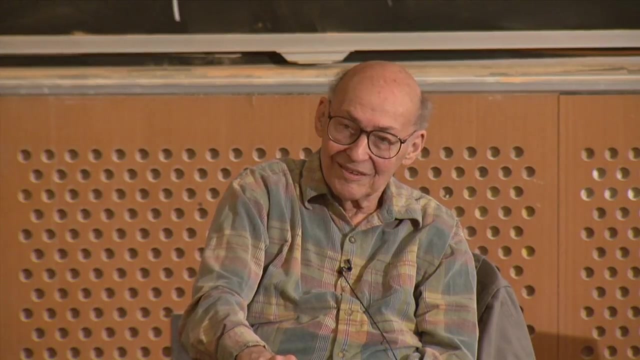 Yes, So I would believe that math is too abstract, And so it's difficult to go from one representation to another, And that would be the problem. I can't learn a new concept without having a concept that's very near that concept. that's very similar. 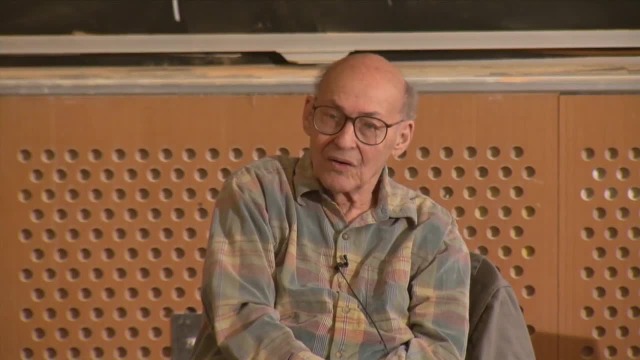 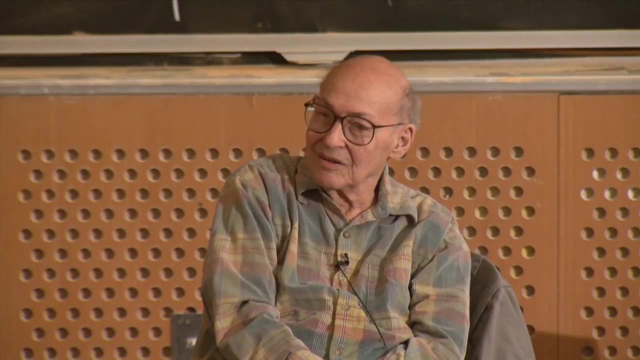 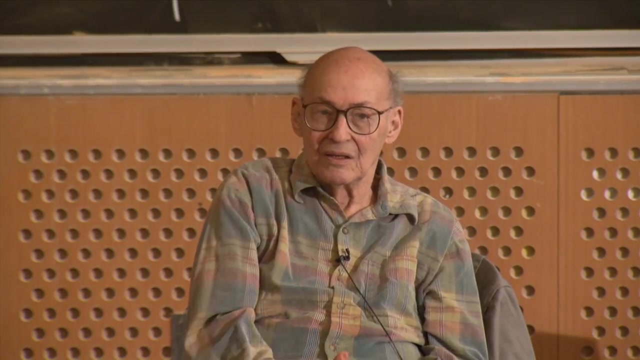 So it's just that if I don't have good representations of a lot of things, it's difficult to put a new representation. So when I learn topology I should know analysis, And then I can go from there to there, because the representation is very close. 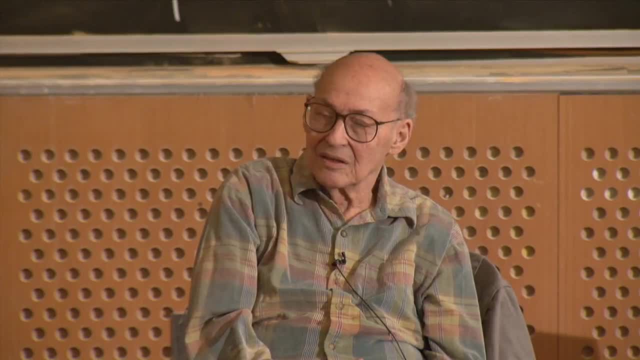 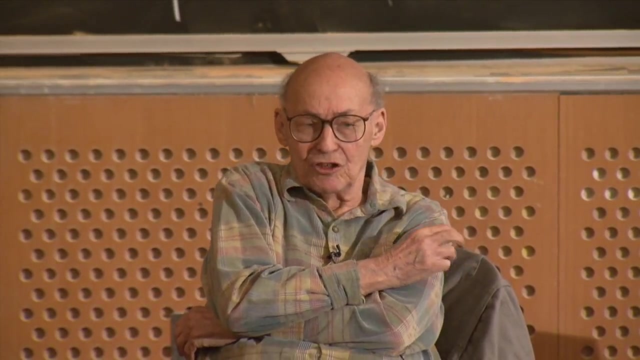 Yeah, And so people that are good at math, maybe they have a lot of representation, So it's easier to add a new representation of a thing because it's like both. Certainly would be nice to know Like in the same of vectors. 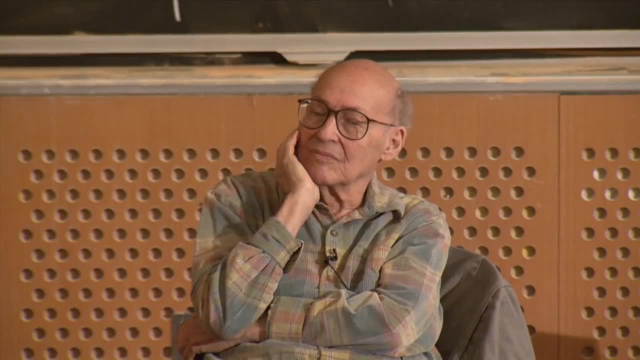 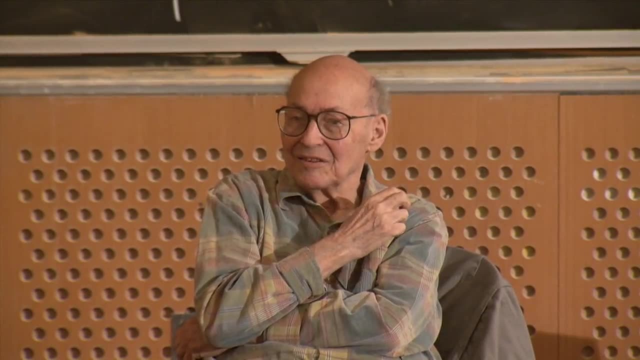 I already have the concept of like I don't know the perpendicular lines, And so just adding more lines. it's easy, but like, just I don't know great, I don't know any dimensional thing. It's very abstract. 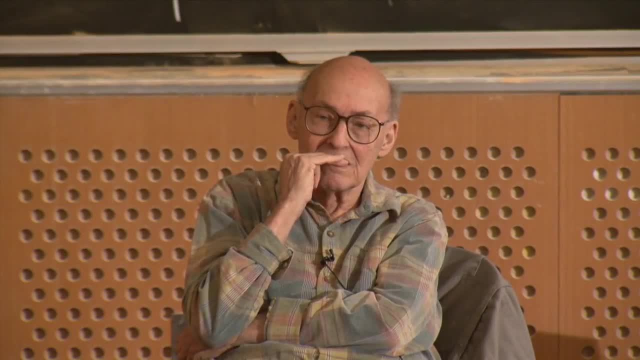 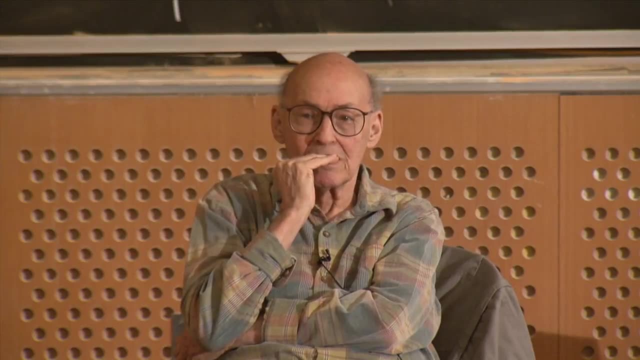 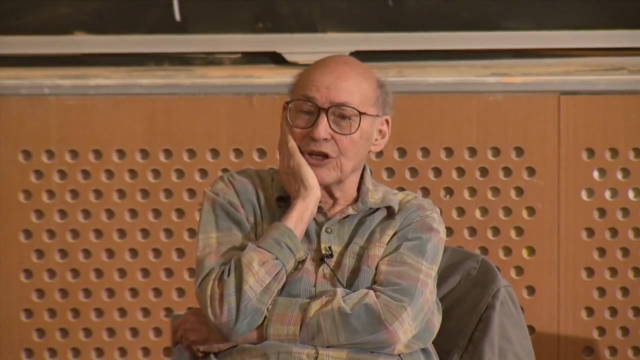 I don't have any other representation that's close by that concept. It's just that I need a lot of concepts and representations And then I need, like, one that's close by- Yes, Between the vectors and the Fourier, they're so different. 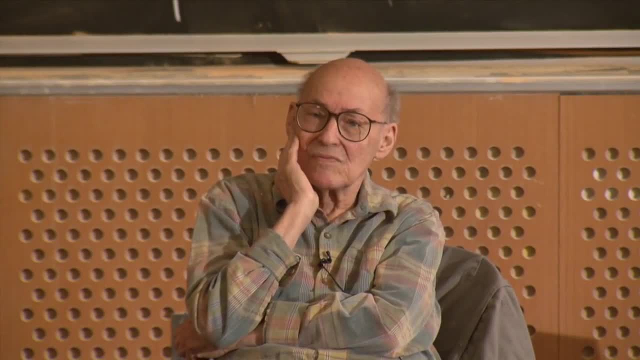 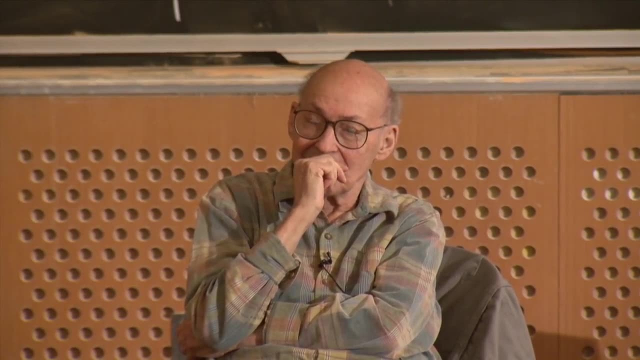 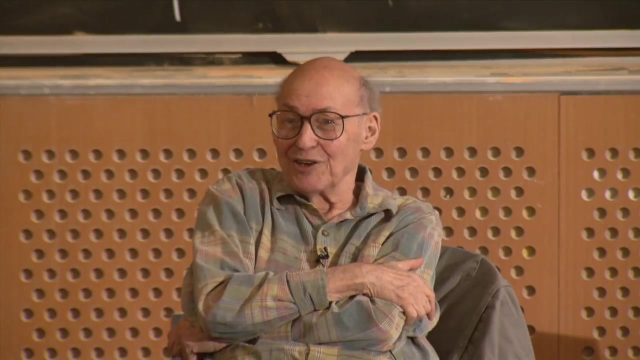 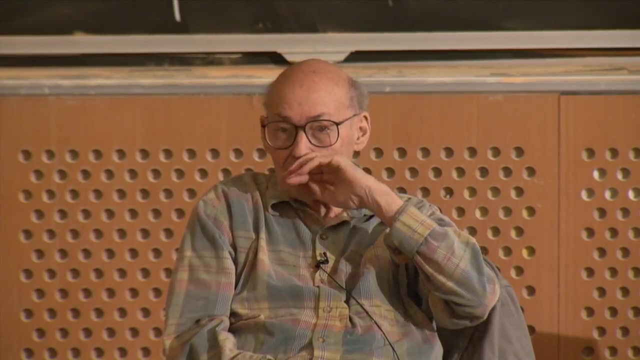 What would be in between those two? The Fourier is built by other kind of concepts. I don't think there are any Actually. square waves- Probably square waves are easier to understand than sines and cosines, but they're not continuous. 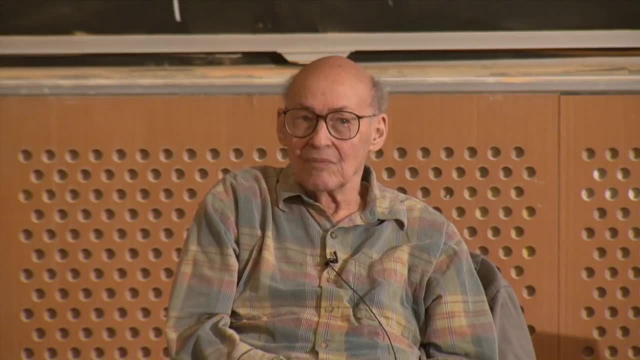 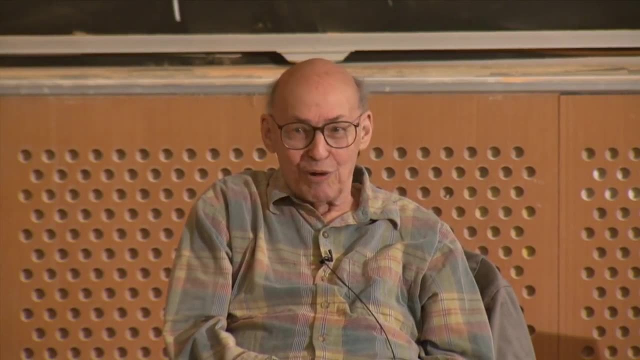 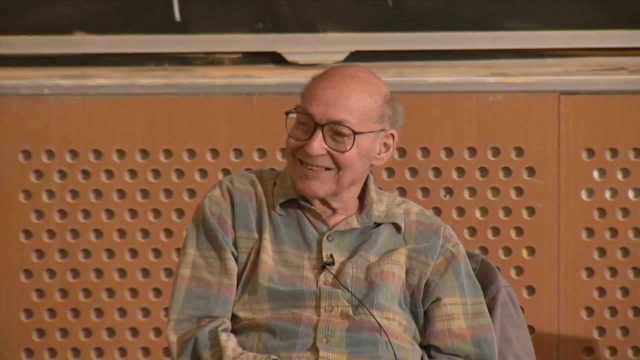 I mean not differentiable. I don't think there are any. I don't think there are any. Who has a problem to solve? I'd like to comment on the- I think- Xiaoxiao's- comment on having lots of practice. 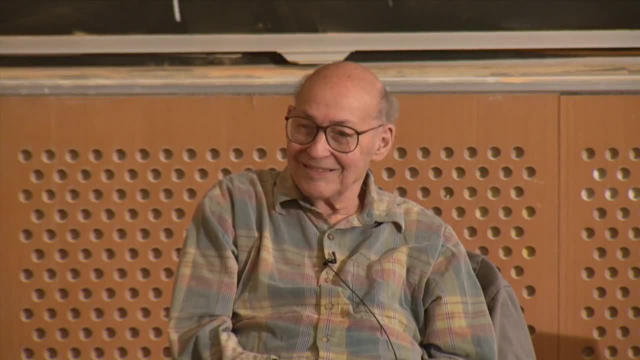 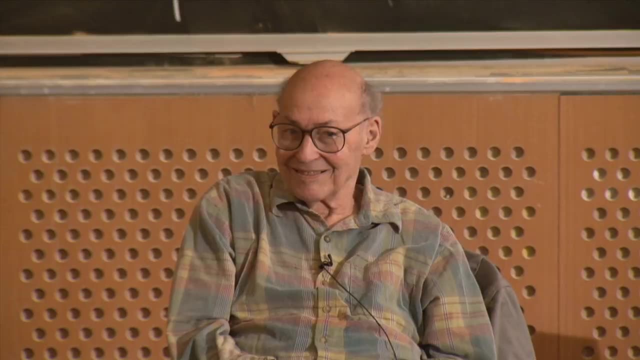 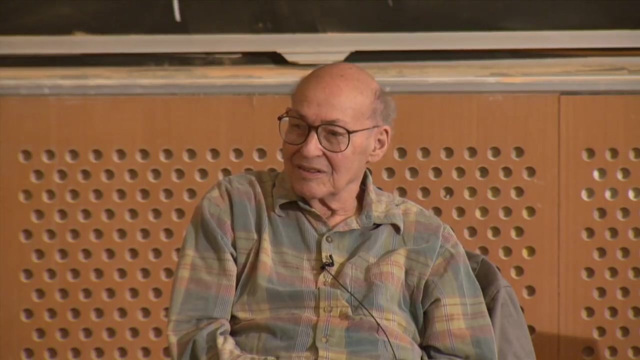 And I don't think that actually so much outflows like the representational view or well, I don't know what's going on there. I think it's a little bit more logical. but if you have new representations, if you assume that they're symbolic representations, 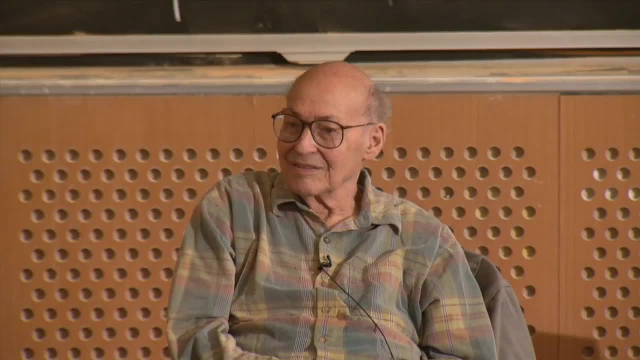 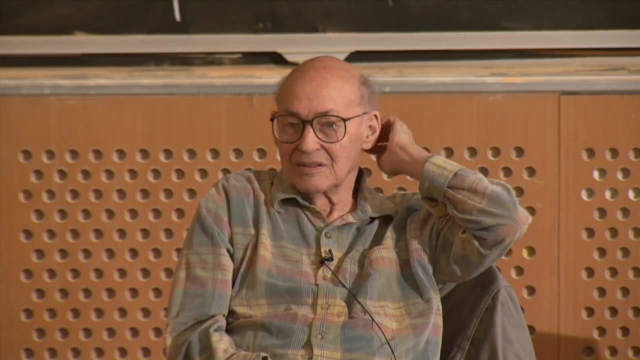 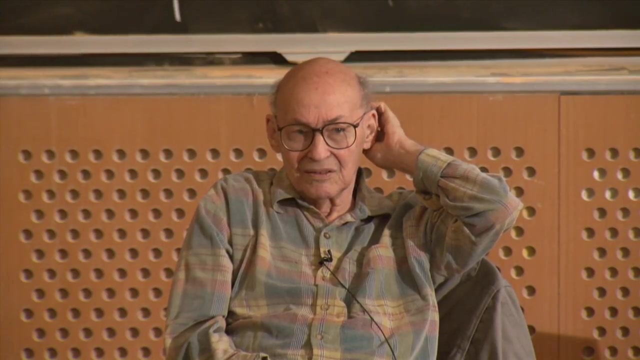 in this sense they are kind of degenerative things. You can combine them and you can make a lot of stuff, But usually when you learn something new, like if you learn the rule, there's going to be exceptions. So when you repeat things- one of the reasons for that- 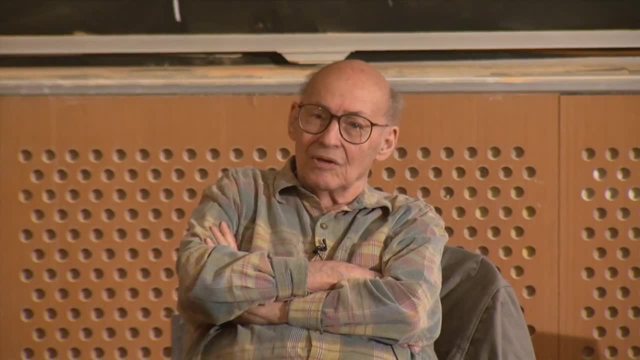 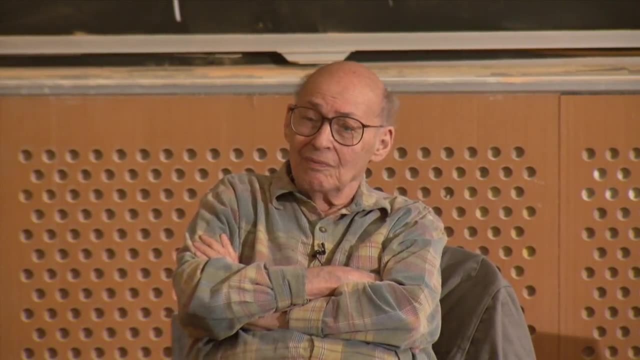 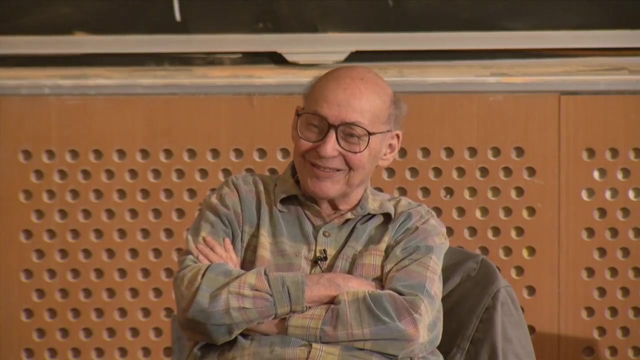 might be to find out bugs. You might have to do the same thing after. Well, now, when you practice a little piece of music by repeating, do you change your representation or do you just repeat and hope it gets better? So I think there's a difference between. 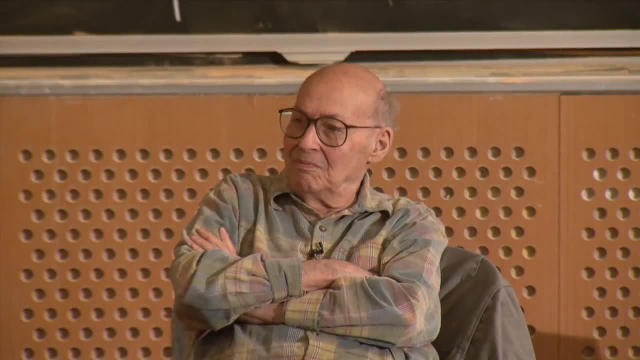 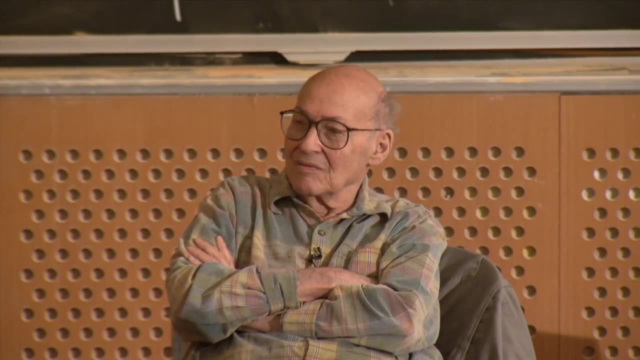 OK, so there's practice in this sense of traditional classical music practice, And then there's the idea of like tinker practice, if you will. I think that the type of practice that I'm advocating is the type of practice where you're actually sort of turning. 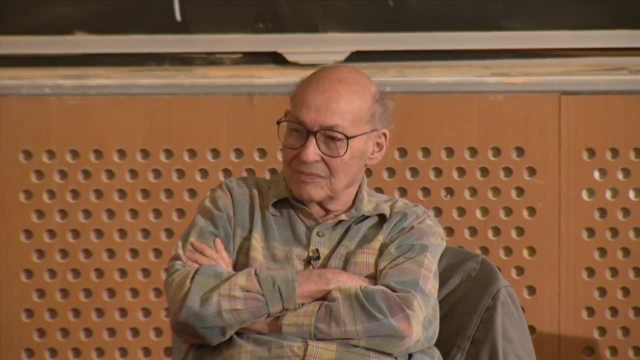 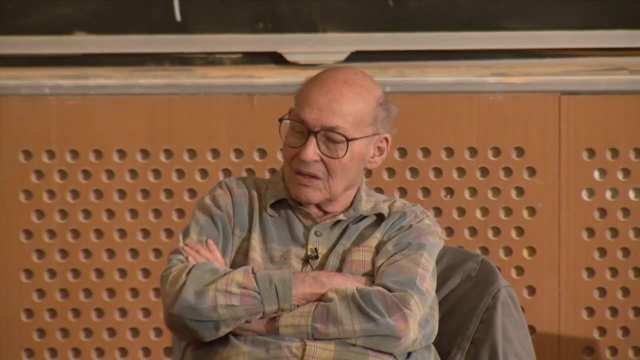 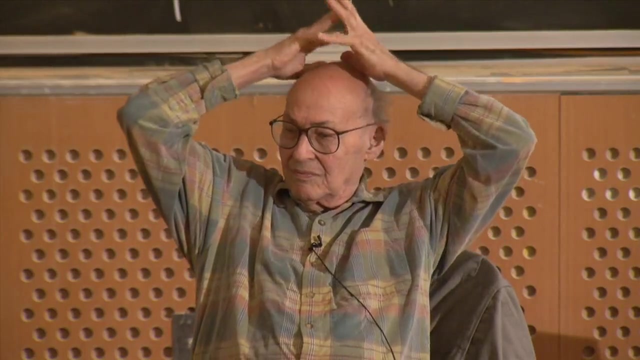 around the concept or the thing, the object in your head, so that you're looking at it from many different perspectives and connecting it to many different things, which is actually conducive to expanding your representation, connecting it to different concepts, like all the good things that help us remember it. 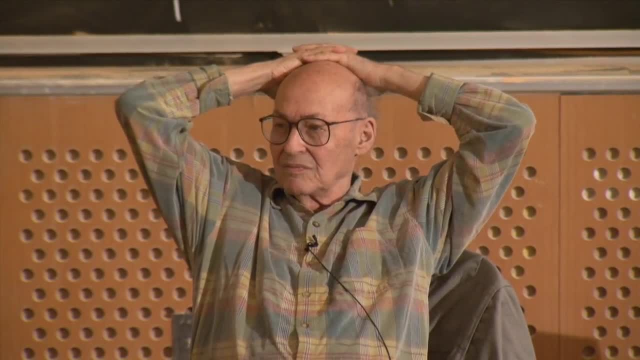 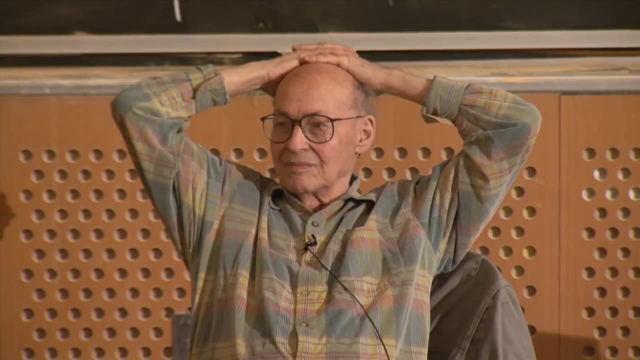 and better use it. This is very different from the classical music practice which, like having been a classical pianist for 18 years, like it's not a really good way of doing things. Well, I was wondering is there? has there been any studies? 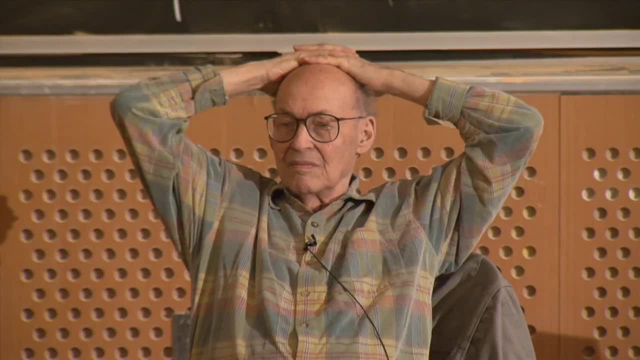 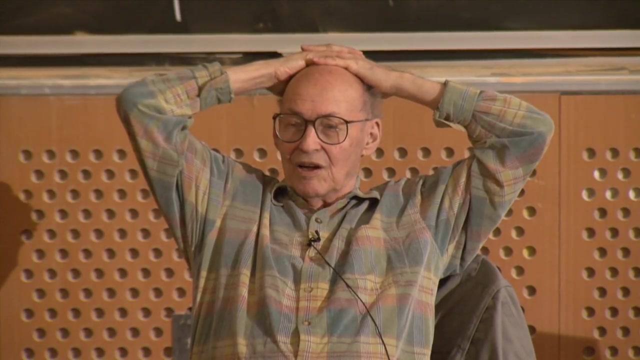 of children? or have there been any children who have just played piano or some keyboard instrument or their lives, and then they suddenly have something where, when you press it, where you can control the volume? A theremin, Yeah, yeah, yeah. 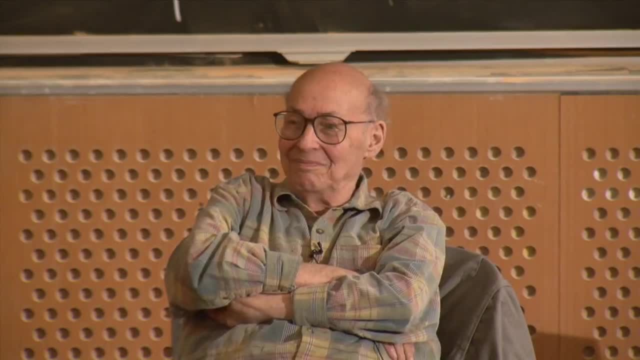 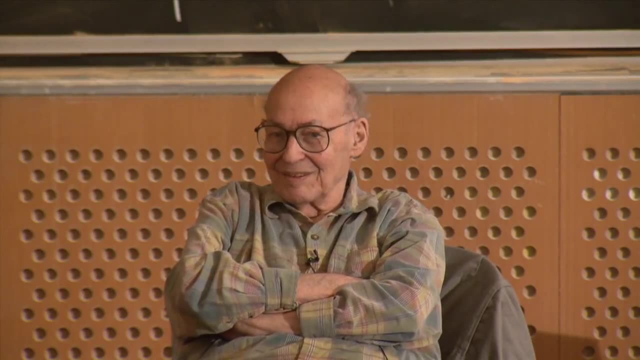 But if the child were very suddenly to learn a completely new dimension? that's the dynamics, and how would it react to that? So I don't know if there are any such cases, But I would suspect that you would go to a suitably 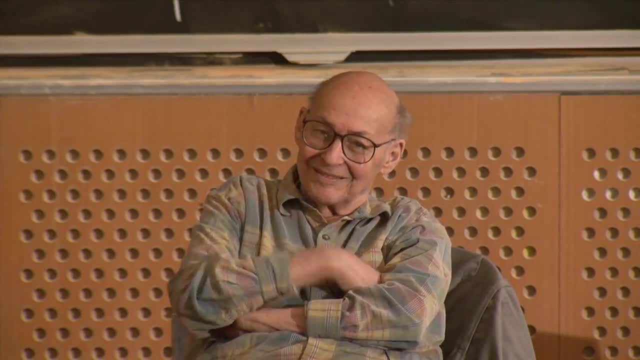 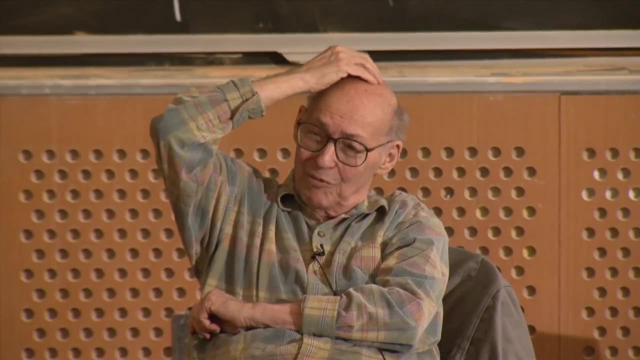 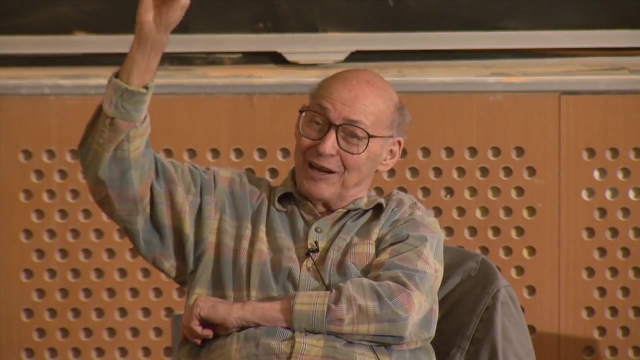 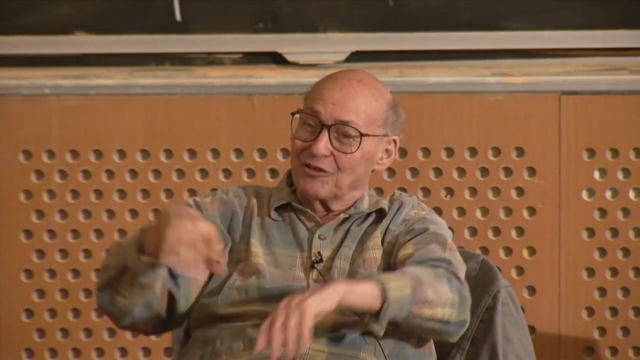 backward place even nowadays and find some children who don't have much. There was a nice period in the Media Lab when we were building, building three-dimensional theremins for pen of Penn and Teller- because he's quite a good musician- and making gadgets so he could wave his hands. 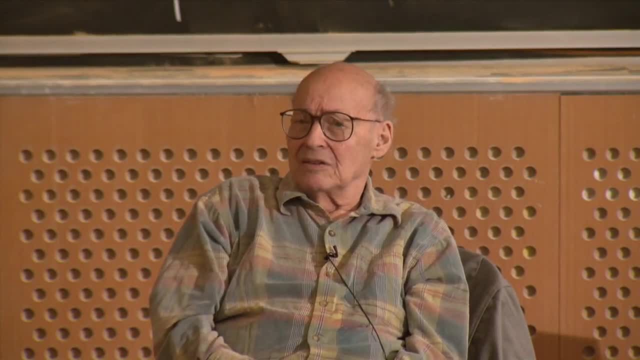 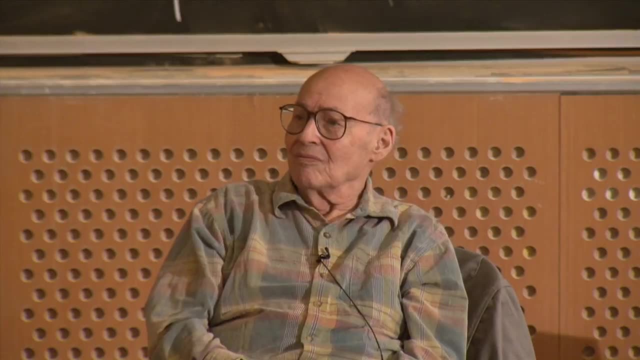 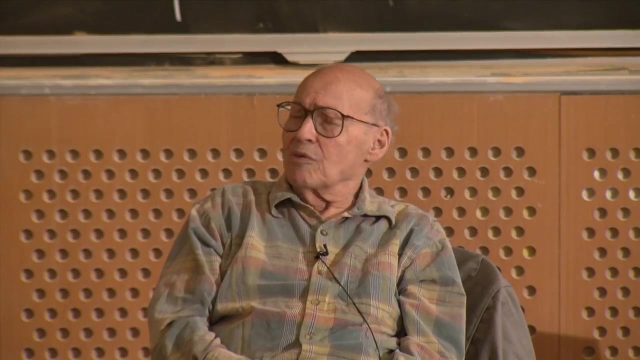 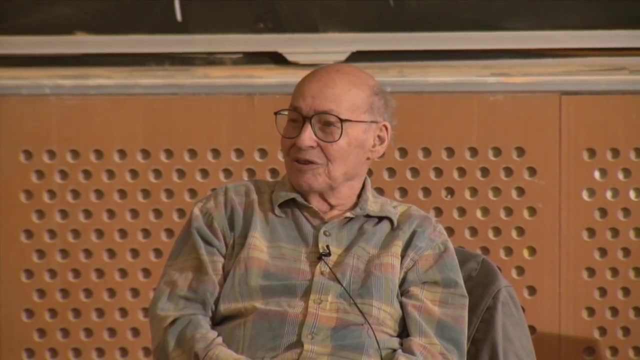 But I wonder, in classical music there ought to be some very short pieces that come in 10 variations, because we make children learn, you know fairly long pieces where it's just repeating. There could be a valentarian instance which is like 32 or 33, like really short pieces. 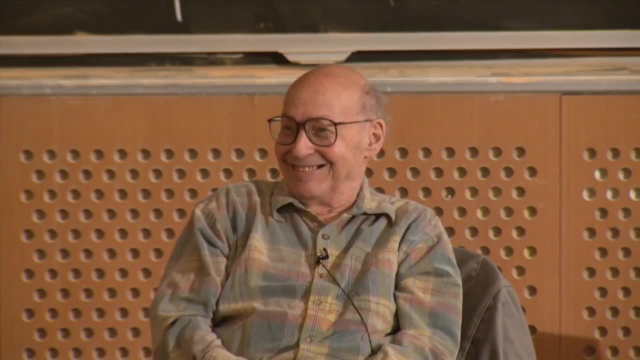 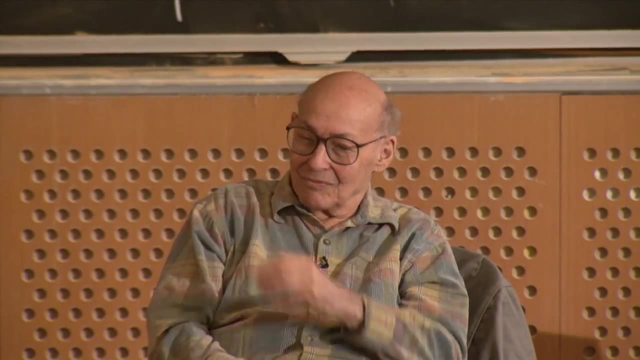 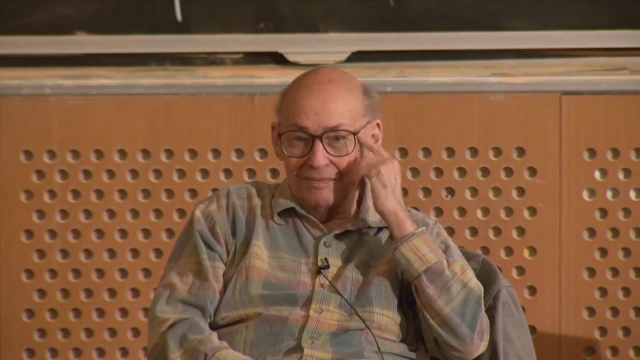 Well, but only eight people in the world can play it. But I guess the thing with classical music is that it kind of just makes you learn this one thing and you learn it by repeating it over and over, whereas in something like jazz that's more improvisational. 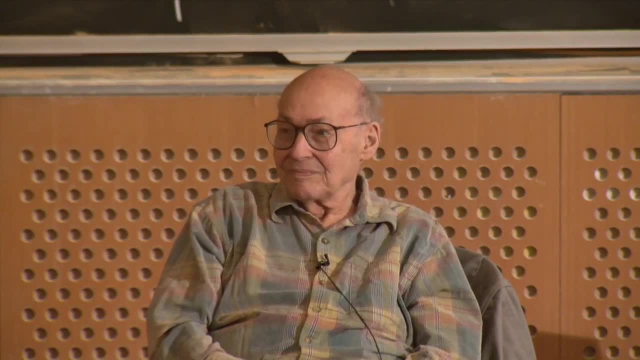 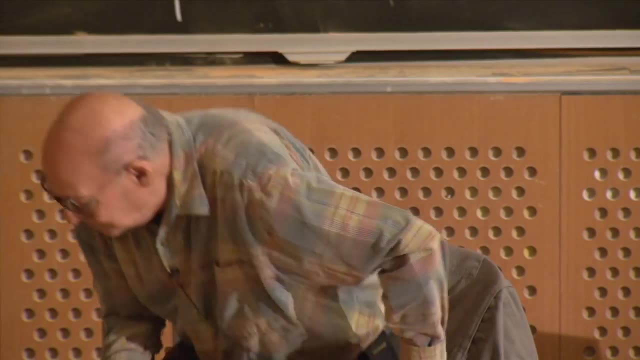 it's like you have a template and each time you go through it you can traverse a different path through it, But even more like classical classical music, where you're playing the same thing each time. I think that there's still like a good way of doing it. 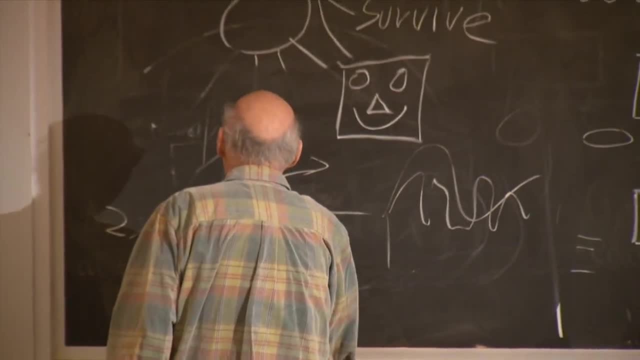 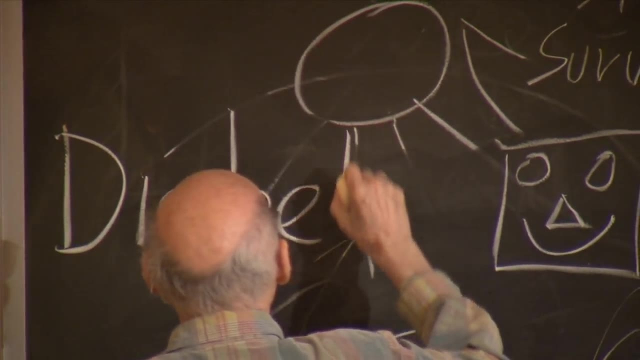 and a not so good way, The good way being, like, each time you practice it you subtly vary it somehow, Like you change the expression a bit, you play it faster, slower things like that, And I guess this goes back to the whole like: 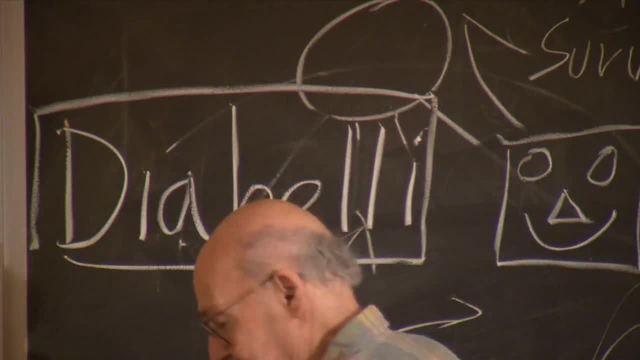 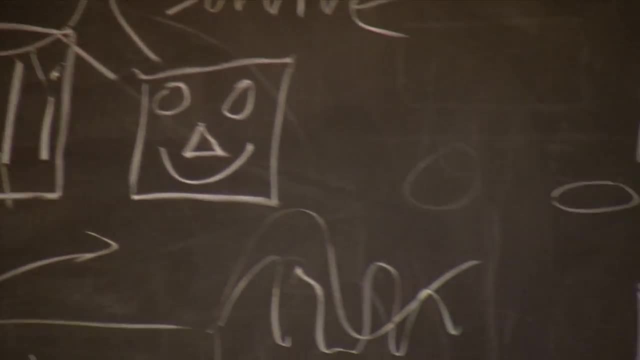 it's like each time you reinforce an idea, like simply repeating it well, like in the beginning, like it might help you familiarize yourself with the idea, but if you repeat it and vary it slightly each time to like, look at different dimensions of it, 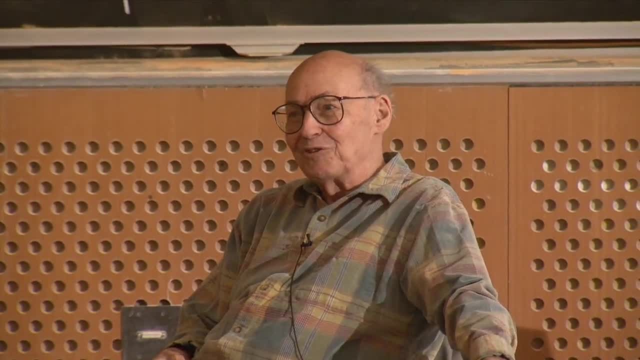 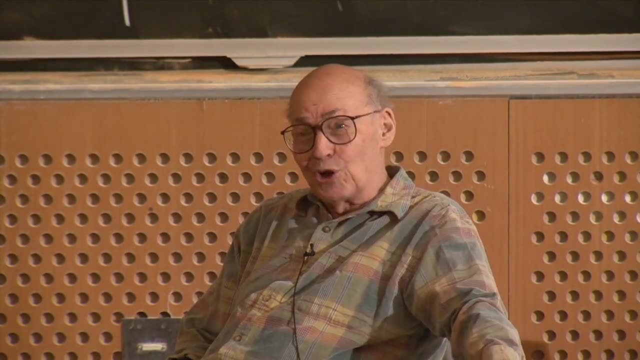 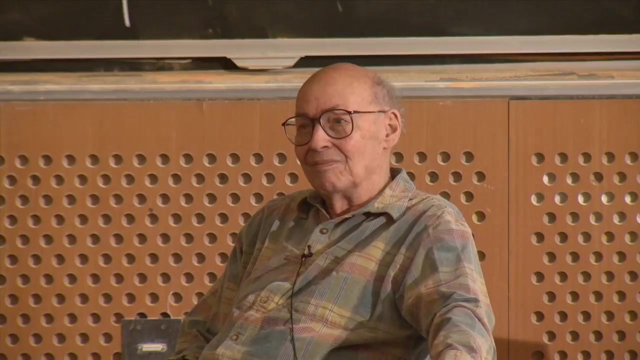 then you learn it better. How many of you know that piece, Beethoven's Diabella? Well, you should Google it up and listen to it. It has 32.. Is it 32?? I think it's 32, and then there's the original theme. 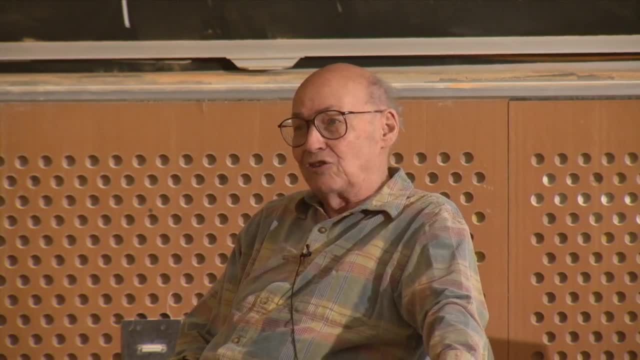 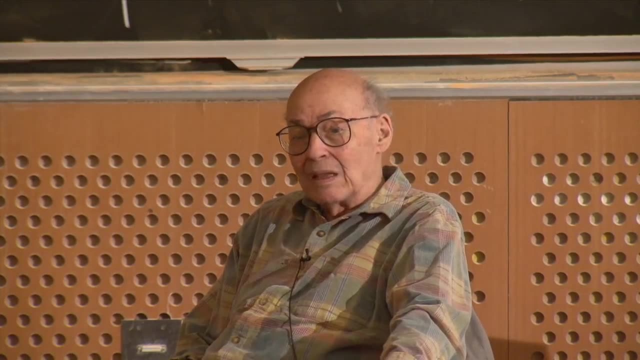 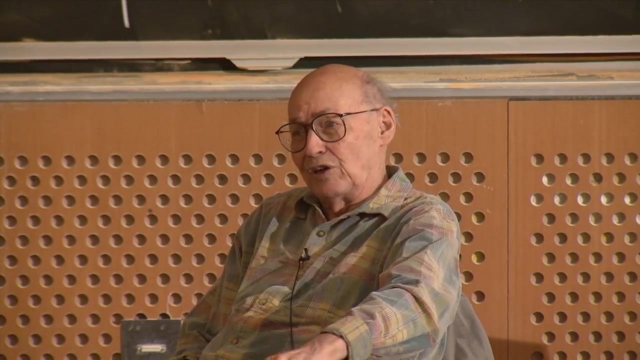 so it's like 33 total. maybe The one I like is the next to last, which is The Fugue. So that'll give you another view of classical music, because the pieces are fairly short and they all have some ideas in common.